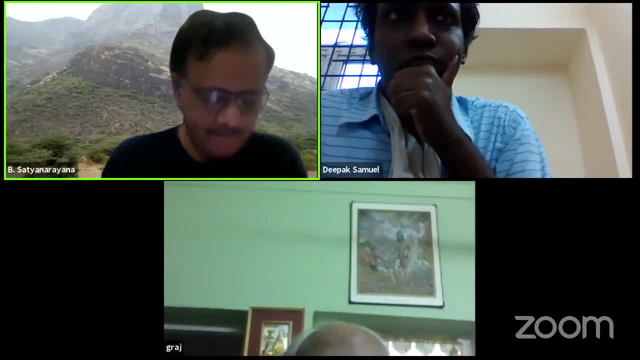 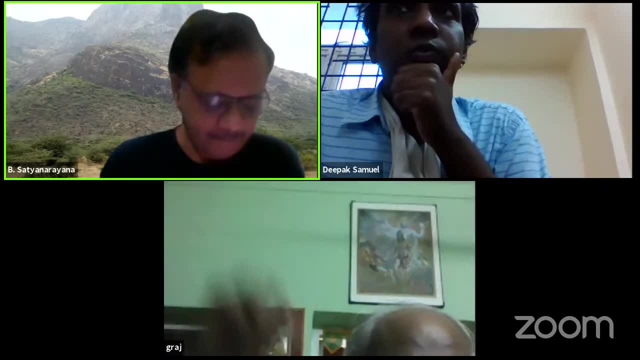 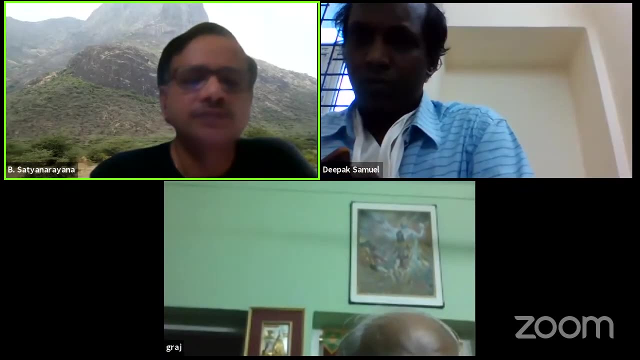 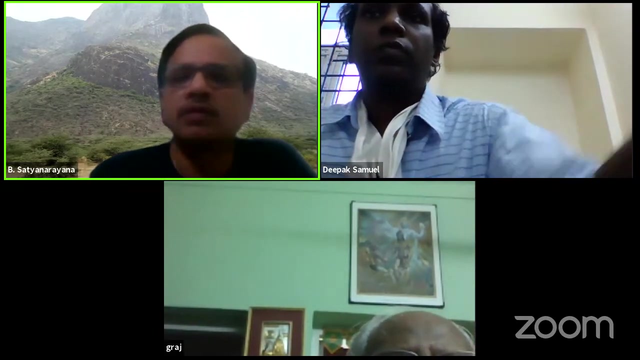 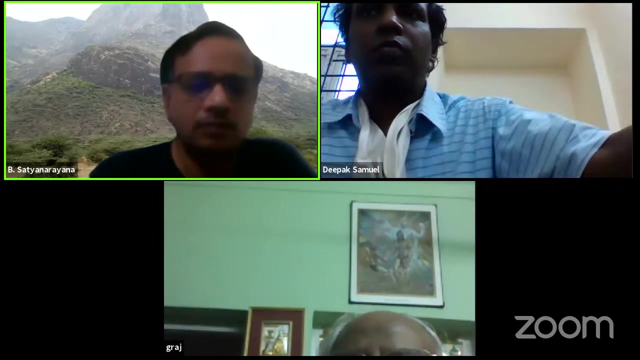 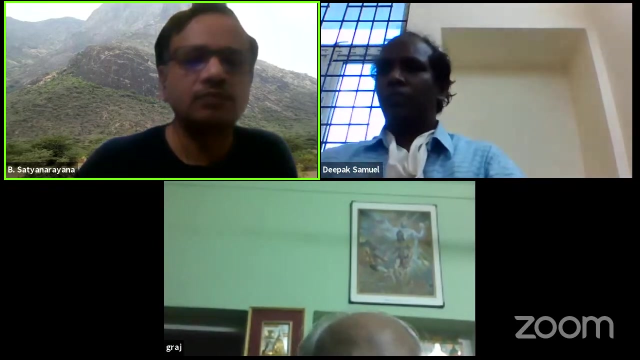 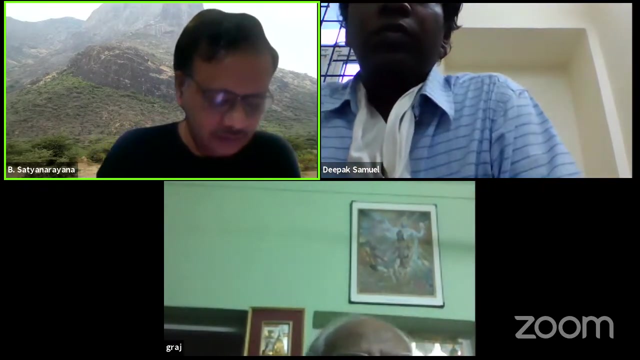 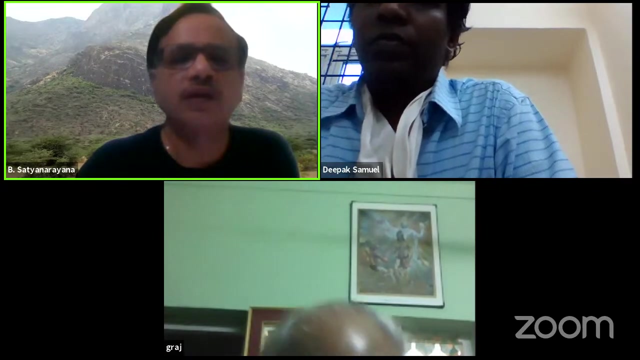 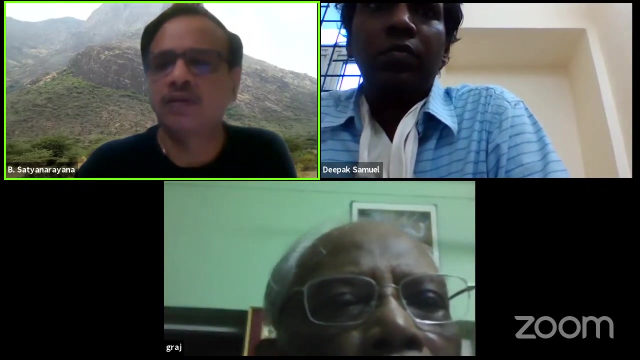 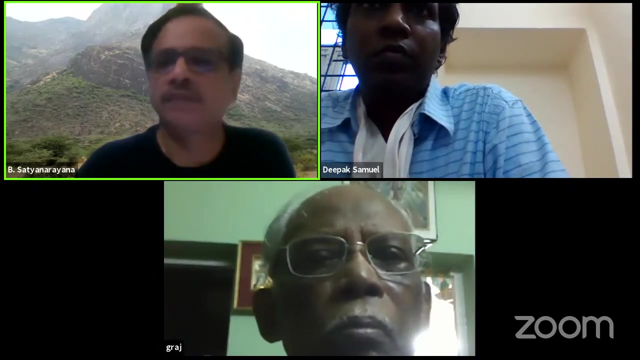 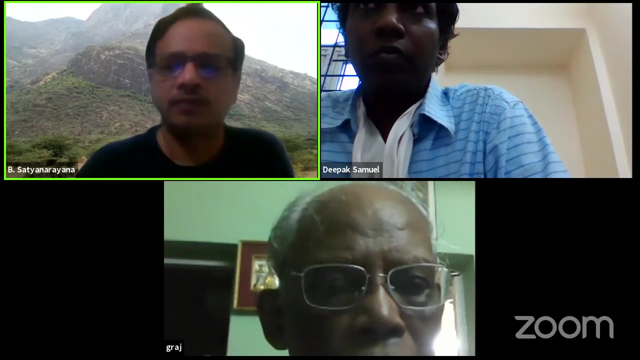 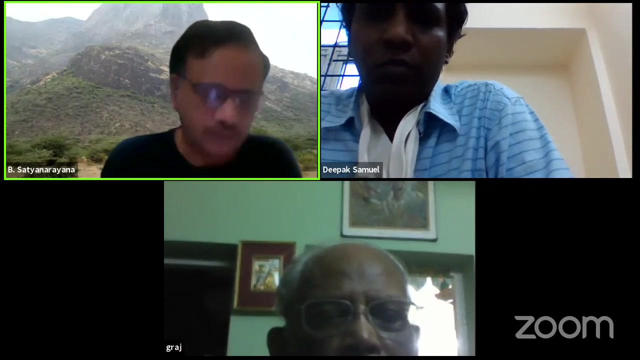 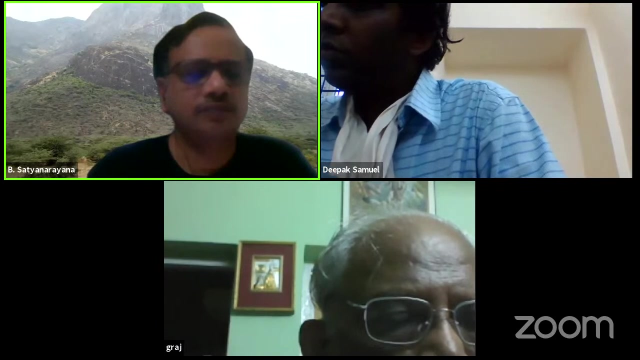 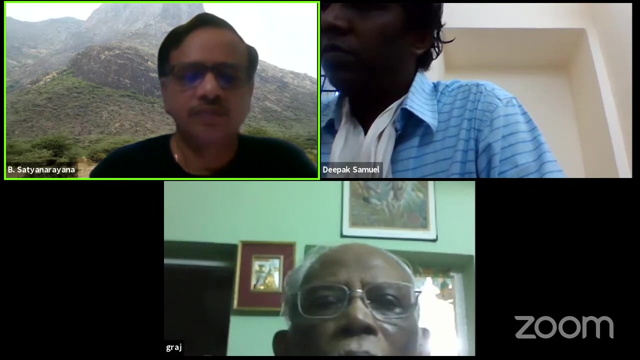 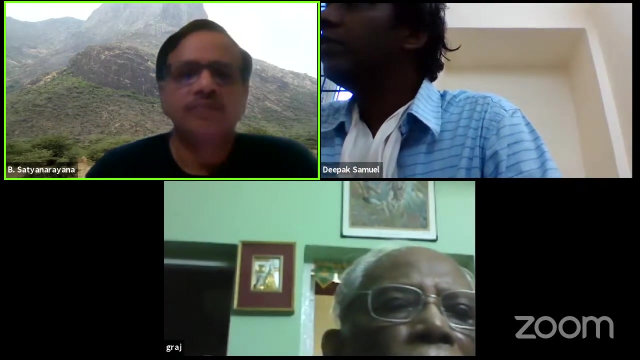 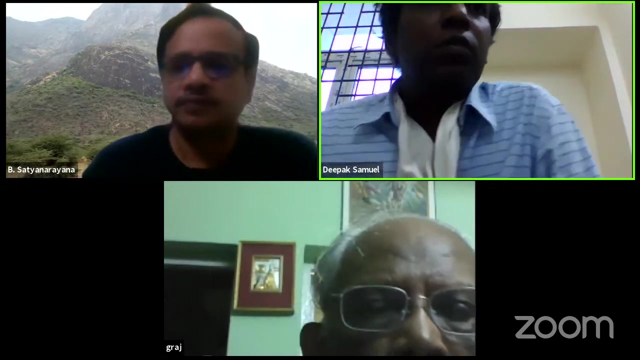 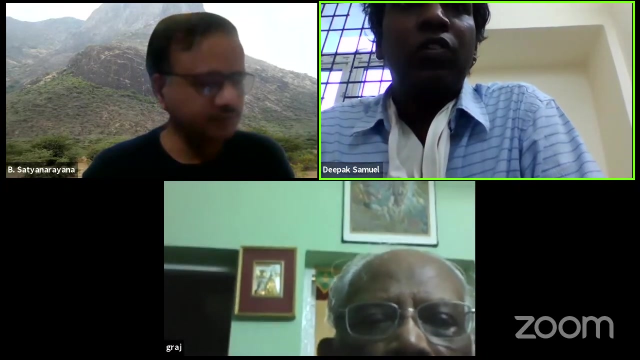 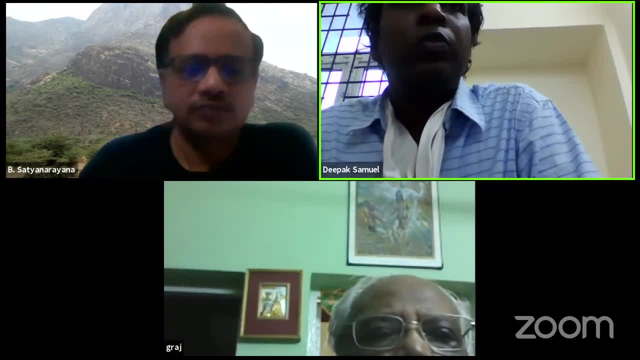 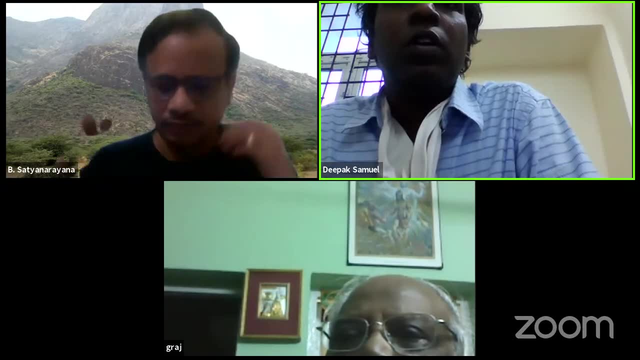 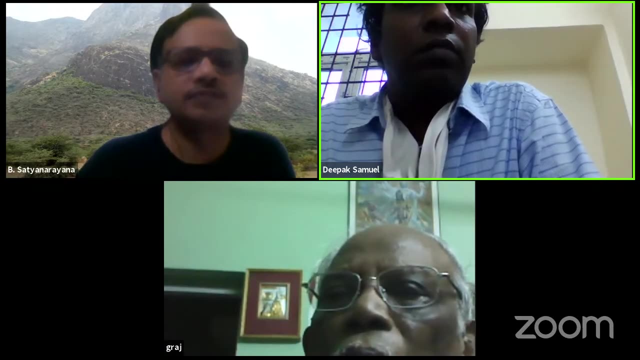 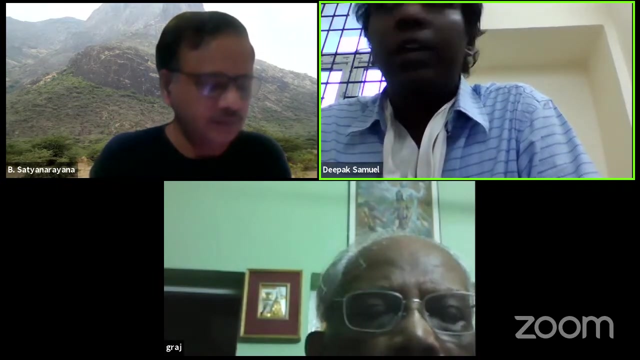 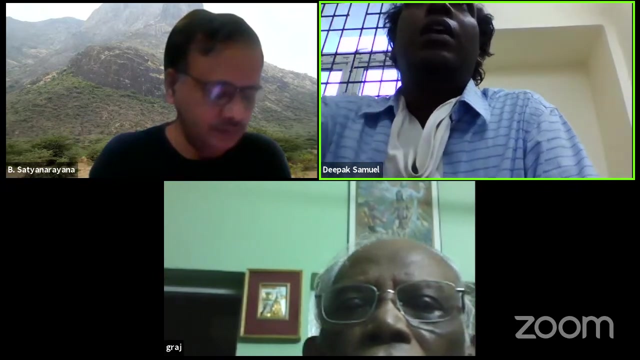 This lecture series we began in, I think, April, 27th of April, and many people have given interesting talks on different aspects, on not only Neutrino physics, but also topics like dark matter and other subjects, and I would like to encourage you to visit the website that we have developed for this, one, which is being currently shown on this screen. 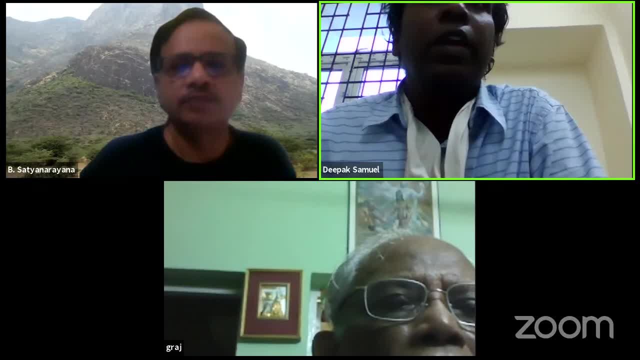 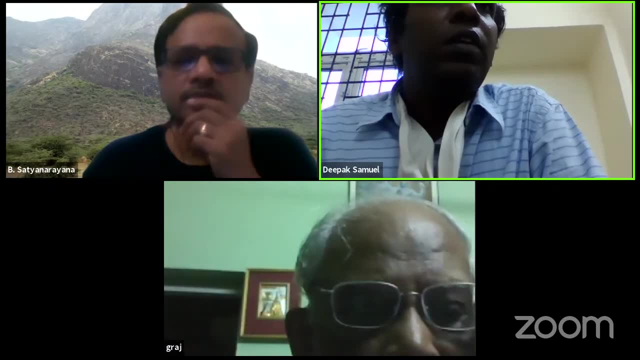 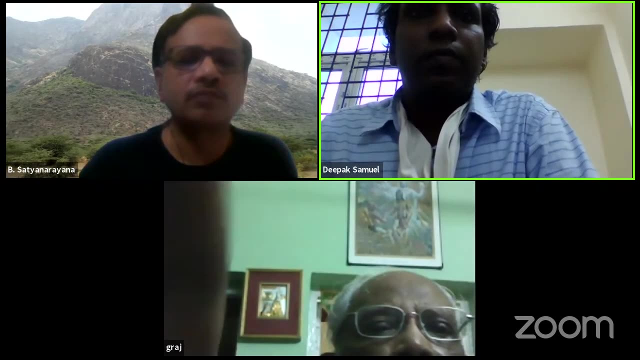 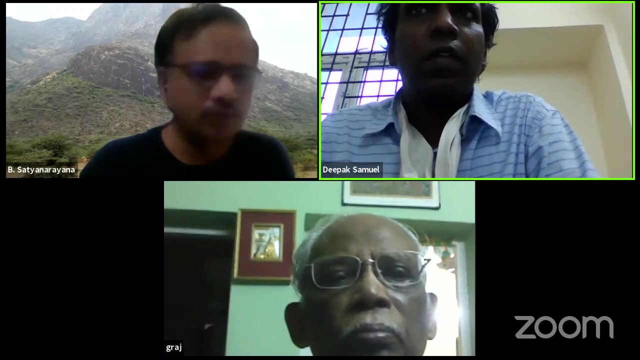 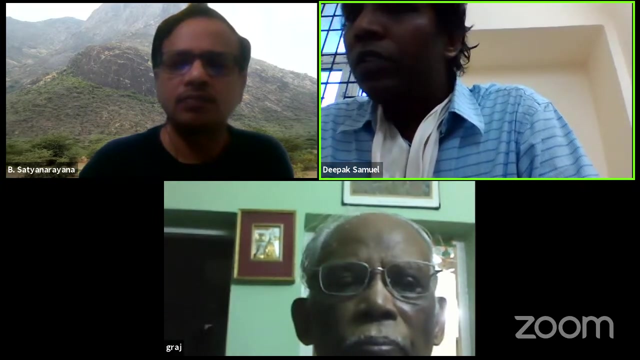 I think Dr Satya is not on this screen. All right, Yeah, Just a minute, please. Yeah, so we will share that screen soon. And yeah, So we also have a Facebook handle and Twitter handle and we encourage you to visit that. 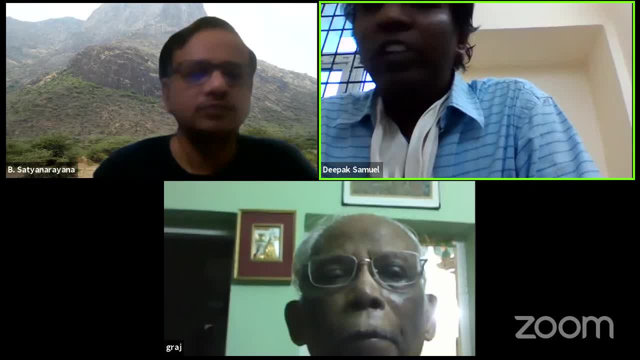 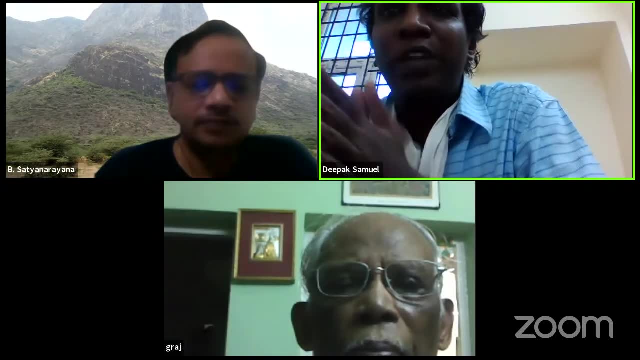 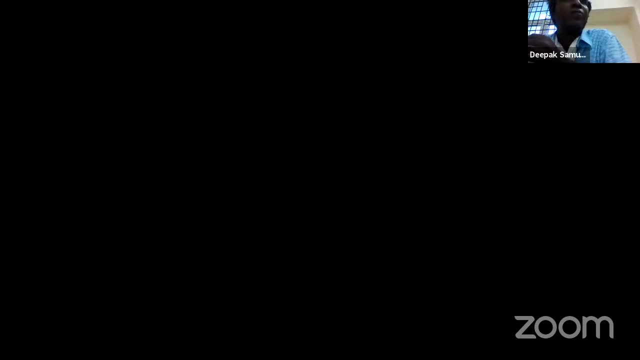 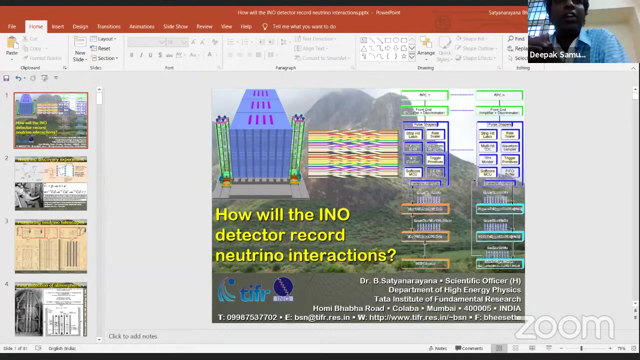 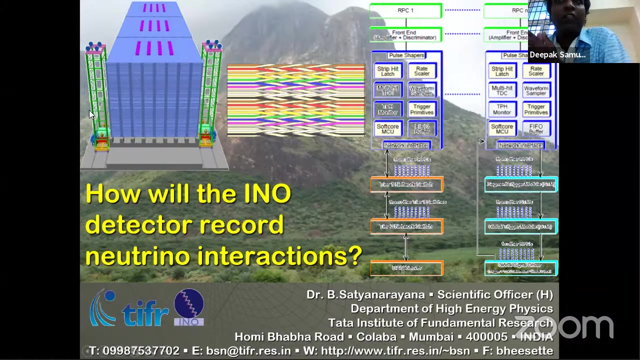 So we also have a Facebook handle and Twitter handle and we encourage you to visit that Department of High Energy Physics, TIFR since 1983 and is currently a scientific officer. He is also a visiting professor at the Applied Science Department of the American College. 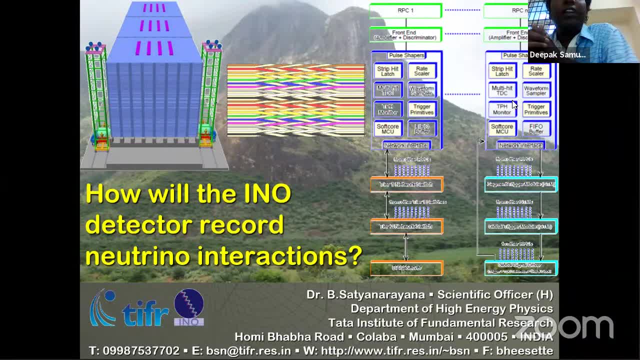 of Madurai. His areas of interest include detectors and instrumentation for high energy and nuclear physics experiments. He worked on many major experiments, including a series of underground experiments at Kolar Goldfields, D0 experiment at Fermilab, Chicago and CMS. 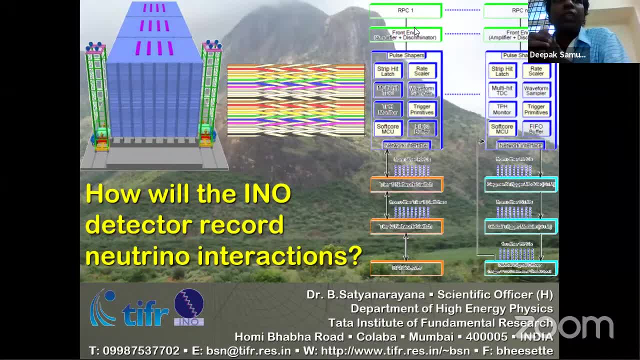 experiment at LHC at CERN Geneva. Currently he is fully engaged in building a mega science experiment called ICAL at the proposed India-based neutron observatory INO near Madurai. And, of course he has vast experience in detectors called as resistive plate chambers. He is 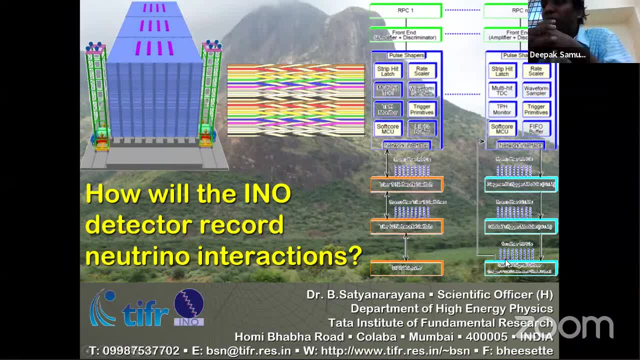 an expert in this field. He started by designing this one-feet by one-feet resistive plate chambers, and then upgraded to one-meter by one-meter and now, I think, two-meter by two-meter and multi-gap RPCs. And, as you must be aware, INO is a mega science project And I must emphasize here that it. 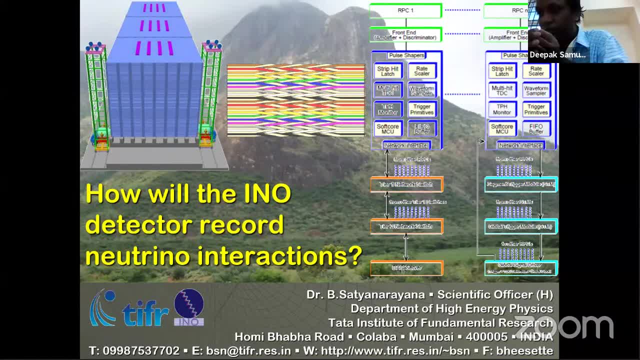 is not just only a physics project, it is also an engineering project. So these resistive plate chambers, in which Dr Satyanarayana has a lot of expertise, Thank you. These are sensitive detectors that will detect the signal left by the neutrinos. So, without 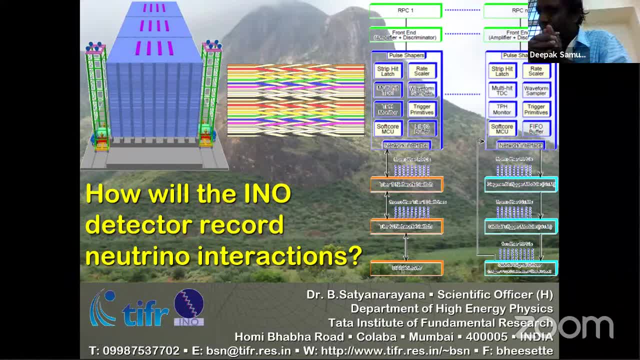 the resistive plate chambers. there is no ICAL, So I invite Dr Satyanarayana to share his excitement of developing these resistive plate chambers. Over to Dr Satyanarayana. Good evening everybody. Can you hear me? Can you hear me? 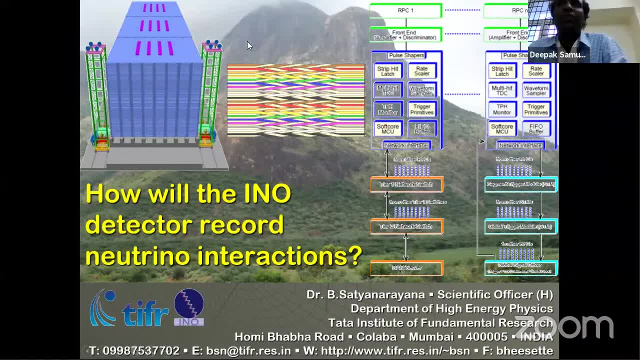 Yes, Okay. Also, can you see the screen? Yes, Okay. So thank you, Deepak, for a nice introduction, And also thanks a lot to Rajaji and also Aacharya, who are on the call. I think I also see a few other friends from INO, As Deepak. 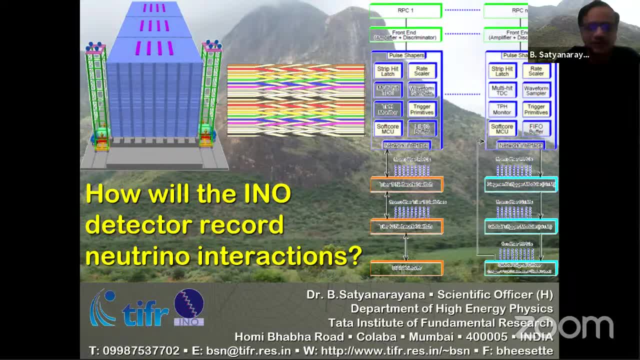 introduced. Of course, we have been having these talks now for a while and most of them have been, of course, given by a real expert in the field of neutrinos and dark matter and whatnot, and of course we also had a few talks on the experimental techniques as well. 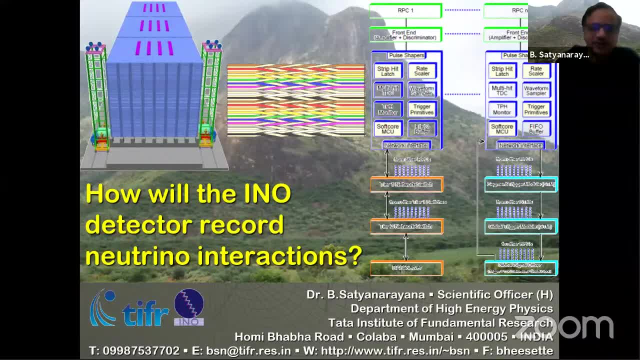 but they have been largely on the theoretical aspects of neutrinos. In fact. incidentally, today it should have been given by one of our past INO students. Somehow I was not able to get him on call, so, as it always happens that I have to pitch in, to give this in. 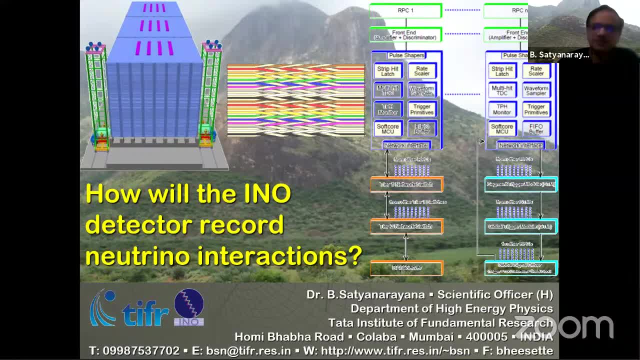 the last minute. I hope I'll be able to kind of satisfy your requirements in terms of knowing about what these resistive plate chambers are and how they are used in iCal built by INO experiment and also other experiments. The title of my talk, as you see, on 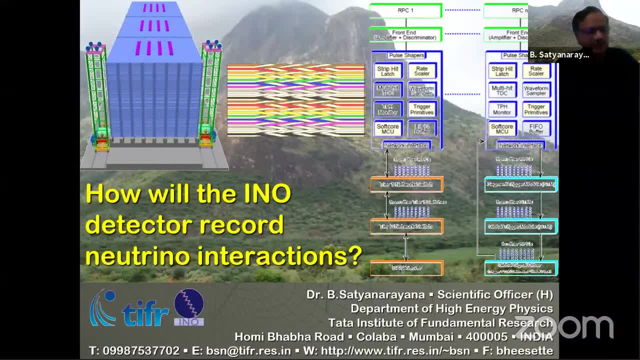 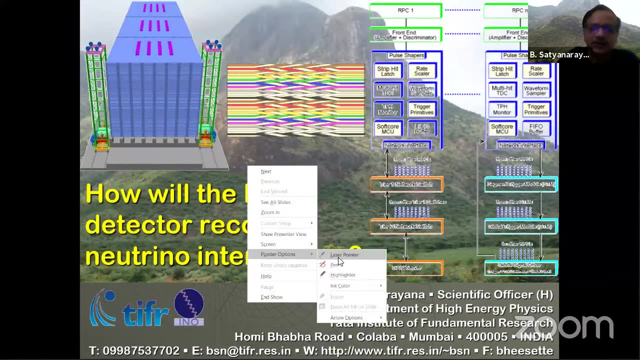 the screen is: How Will the INO Detector Record Neutrino Interactions? that the title is motivated because you have been hearing about neutrino oscillation, neutrino interactions and various other phenomena. but when you really build INO, the big detector, and how actually, when? 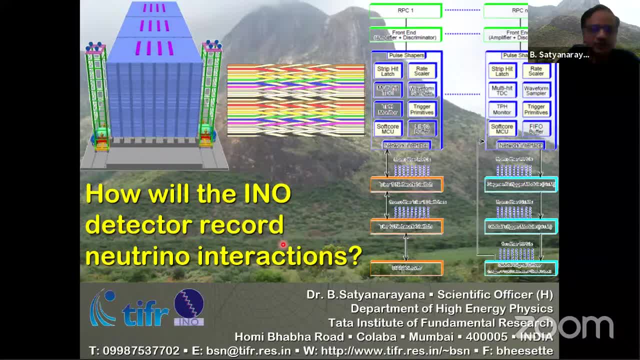 whenever the neutrino interactions do happen in your detector. of course, they are reasonably rare and they're not in big numbers, so how will you actually end up recording them and how do you know that your detector is, you know, live and working to record the data? and also, how do you know that the detector is recording it accurately, in the sense? 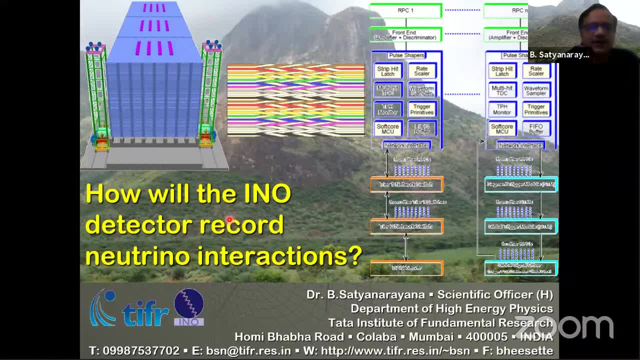 that you know it's not a spurious event and so on. okay, so that is the kind of motivation for this talk, what you see on the left- of course you will see this picture many times later, but this is the so-called iron calorimeter detector of you know proposed INO project. and on the right, of course, 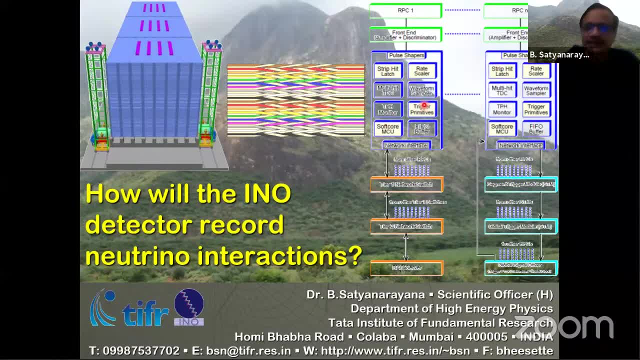 I gave symbolically some blocks of what it looks like some kind of electronics, and of course this we all know is a kind of cable. some of us call it flat cable because it is in flat and there are multiple conductors. so the point is, how do, when? 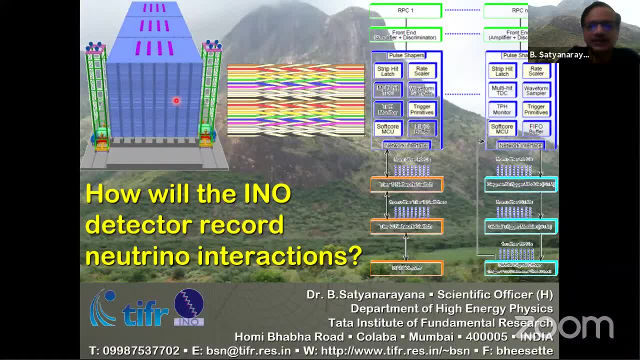 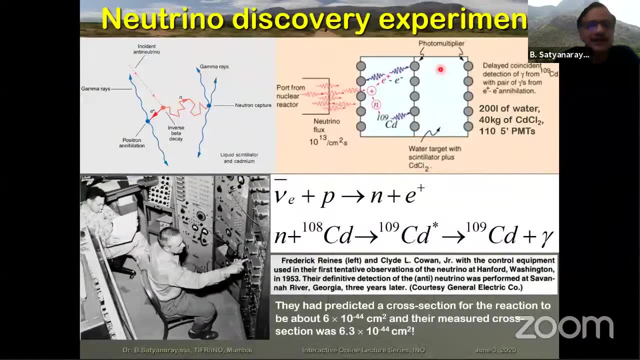 you as and when neutrino interactions or any interesting phenomena happens? how do you actually record them? so that is the theme of today's talk, but obviously we must start when you talk about something recording. of course we should go back all the way to 1956. 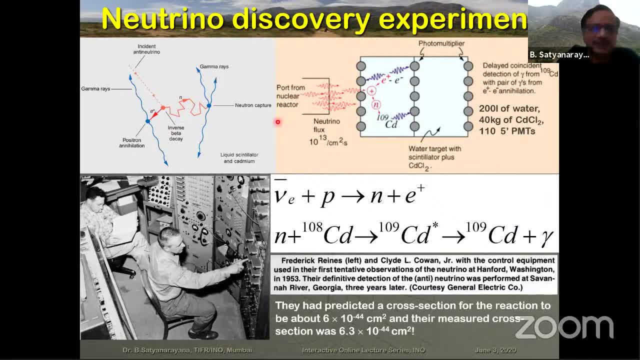 and a little bit look at, maybe just to get the context, how you know, Reines and Cohen, the, the guys who actually discovered neutrino, their very first discovery experiment in 1956, did the that using. you know, today, looking back, it looked like a very, very simple, rudimentary experiment, but 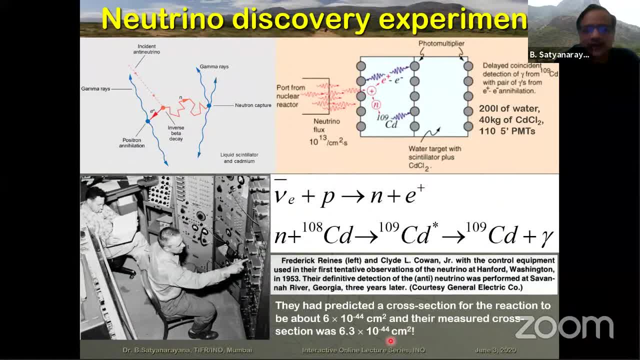 nevertheless, if you look at the kind of numbers they obtained with their measurements are phenomenal. look at this at the bottom. so of course, they used anti-neutrinos which are coming from a reactor. so this is incident at anti-neutrinos which are coming through through this port. okay. 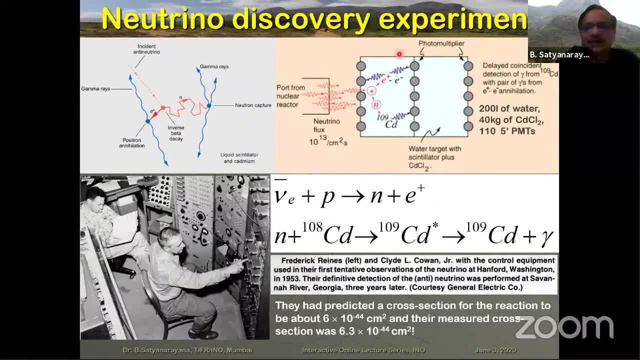 and this is your nuclear reactor. and what they have is a detector like this which is actually made of about 200 liters of water, about 40 kilograms of cadmium chloride and- and, looking at this, the whole thing, these circular objects are, of course, photomultiplier tubes, which are supposed to be about five inch in. 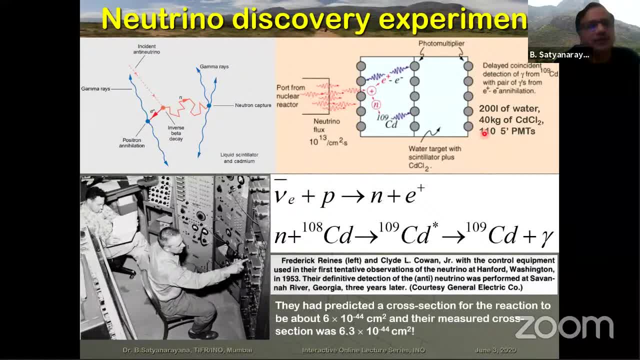 diameter, about 100 of them. 110 of them are used. so when you see an anti-neutrino coming in, and then you know, getting into the volume which is actually a scintillator volume here, you, you, you'll get a lot of information about the nuclear reactor and then you'll get a lot of 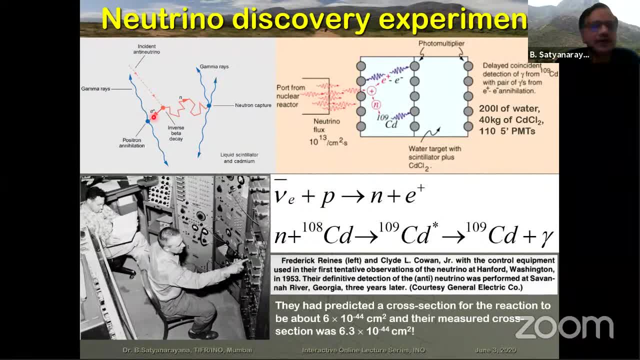 you know, inverse beta decay. you get a positron here and which is actually pass a little bit beyond in this, in this volume detector- volume before it interacts with an electron- and producing the annihilate with each other and producing two gammas back to back. so this is the first event you 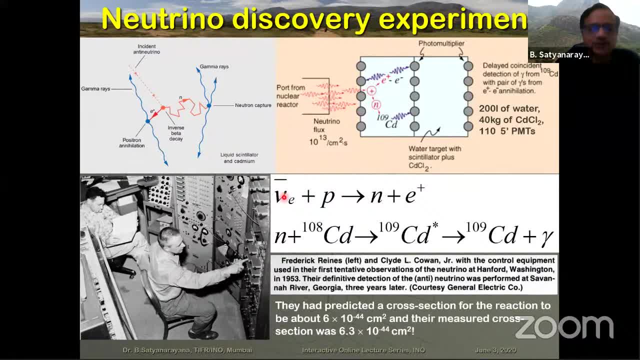 can say prompt event. so this is what is given here: anti-neutrino, coming with proton, producing of course a neutron, and then a positron. now this positron with electron producing two gammas. and you need to detect these two gammas first in order to kind of say: yeah, this is my starting point, this is the prompt and after. 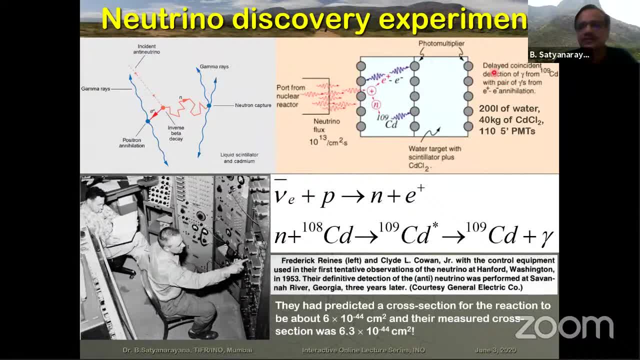 some time. the, you know the delayed coincidence of the, the neutron with cadmium, is going to kind of produce, let us say, photons, but those photons is depending on the fact that there is a delay, which, which is actually shown here by a zigzag moment here now, these gammas are photons that are produced after. 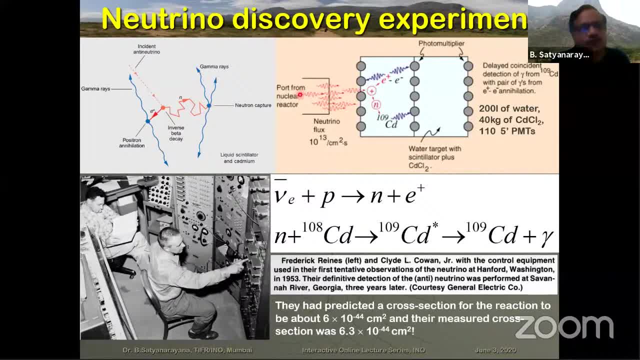 delay of roughly three microseconds. again in coincidence with the fact that you have two gammas here has to be recorded uh correctly in sequence, then you'll know that these two, these gamma came, let us say, roughly three microseconds after these two gammas which were prompt. now these uh detecting the first two gammas and then, in coincidence with the 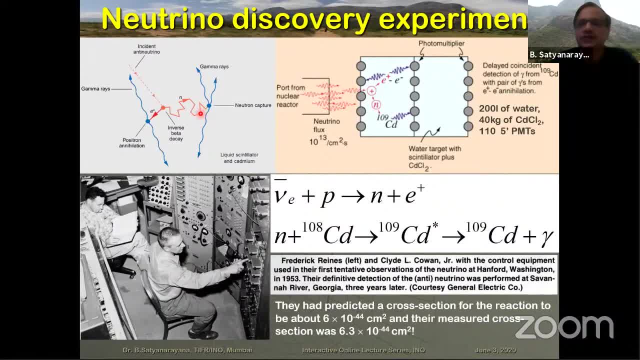 the delayed neutron capture, which is actually giving you uh, the, uh, the, the gammas that are delayed, combined together with duty neutron capture. so combined together is what is going to give you a very unambiguous fact: that is actually, uh, an interaction coming from inverse beta decay. 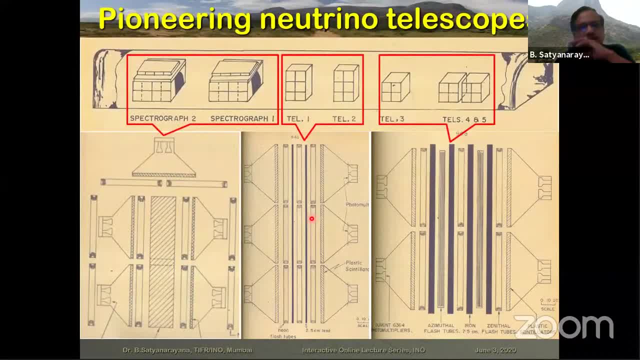 okay, so this was way back in 1956, uh, but uh, maybe 10 years later, nine years later, in 1965, some of my senior colleagues from the department actually built a large number of spectrographs. what are shown here? there are many of them. uh, it's almost about 2.3 kilometers below. 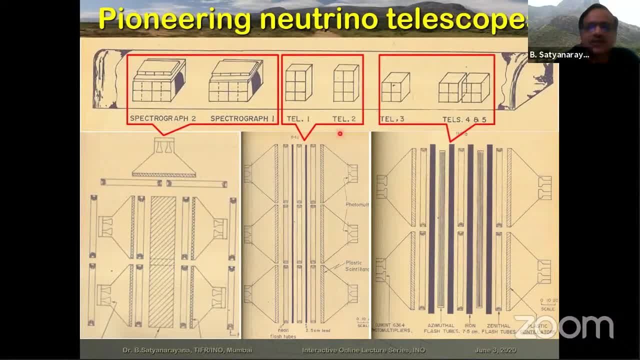 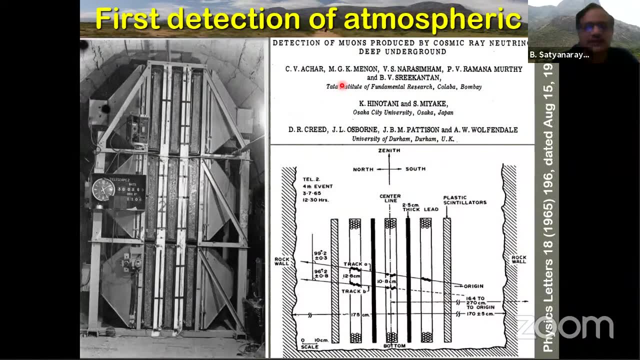 the earth. and here this particular detector that is actually showing is so called telescope 2, and let us go to the next slide to kind of say a little more detail about what it is. uh, a schematic of that is actually shown here. okay, so it's all. vertical looking detector. 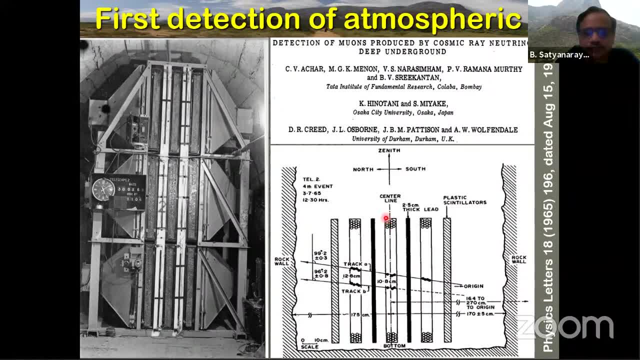 okay, you can kind of see: uh, so there is a. there are, let us say, three vertical walls which are made of neon flash tubes. neon flash tubes, so the flash tubes are actually long, like old tube lights, very thin, maybe about a centimeter or less, but you can see they are sticking perpendicular to 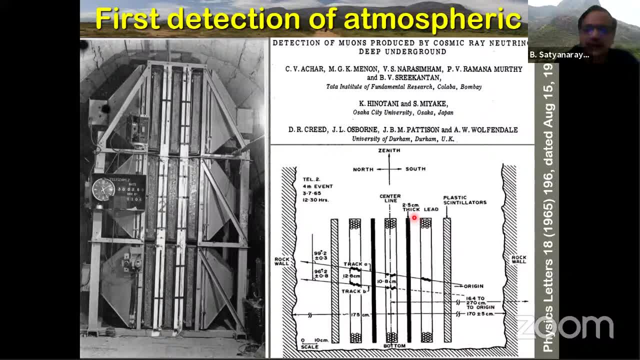 your screens and the black ones. here is led, which is about one inch thick leg, and on either side here which is slantedly hashed. they are these scintillators. so if you want to uh connect them up here, there are scintillators. here, there are center line, as i told you there. 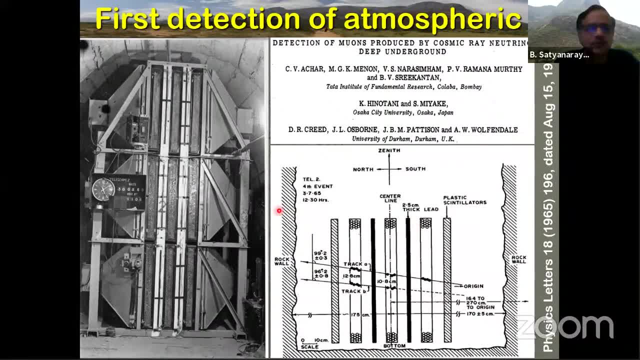 are three layers of uh, the neon flash tubes and also the leg that is uh coming in between now here, of course, they recorded the neutrino interaction that's taking place, uh, let us say, neutrino coming from rock and entering at an angle which is very, very large angle. you can kind 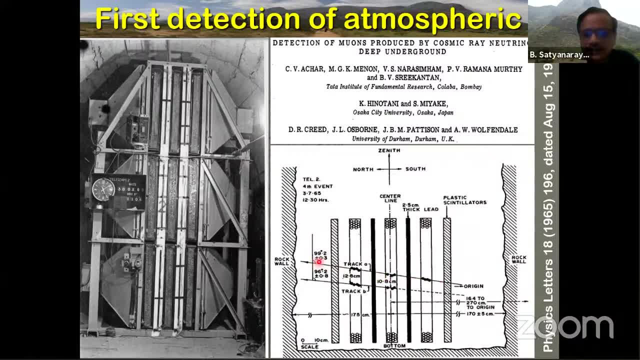 of see here and then leaving a track on this here and also a track, another track, which is actually caused by, let's say, muon decay from uh, from the w, so you have the uh, the muon that is produced here, and also this is a decayed muon, okay, which is also a line which is drawn here, and these 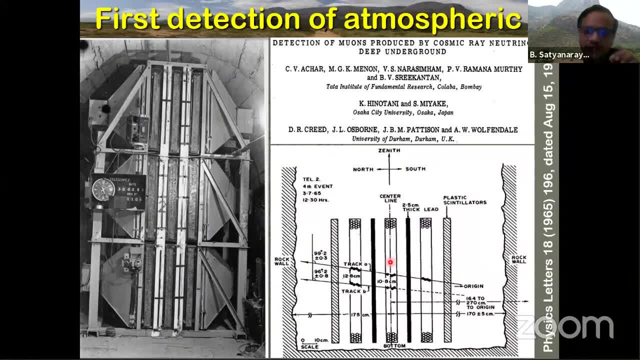 these dots that are going through the, the neon flash tubes. they're actually they're, you know, they flash, uh, they give light when any charge particle kind of passes through. so if you connect them, those you know, uh, those those in line, you actually see a very nice straight. 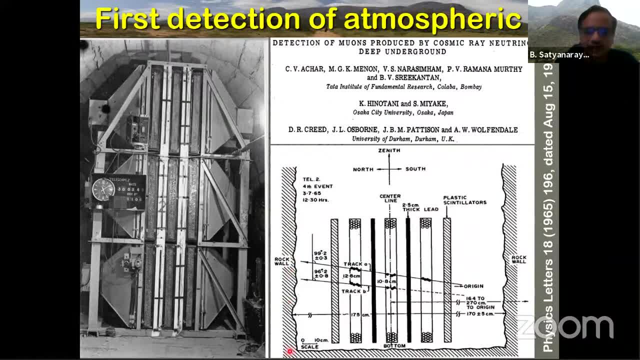 here and this is all you know. i mean, what is hash here is all um, rock and uh. the way you know to record the data when this event has actually happened, you actually hang up or hang a wall clock onto the detector and take a photograph. because this is uh, the detector signals are. 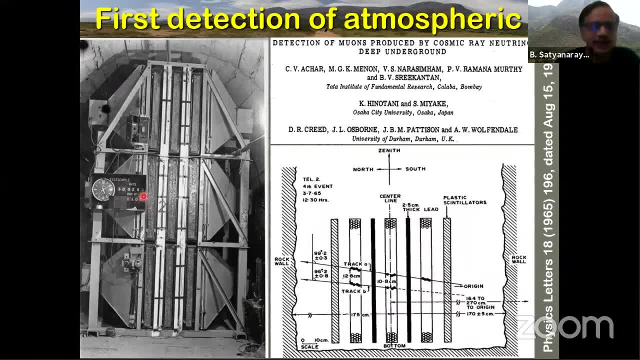 actually a flash of light. so along with that you also see what is the date, what is time. you can see 30th may 1965, and you know also the, also the time, uh, that is that is given. uh, so in 1965, august 15th, in fact, uh, the first detection of uh muons, which are produced by 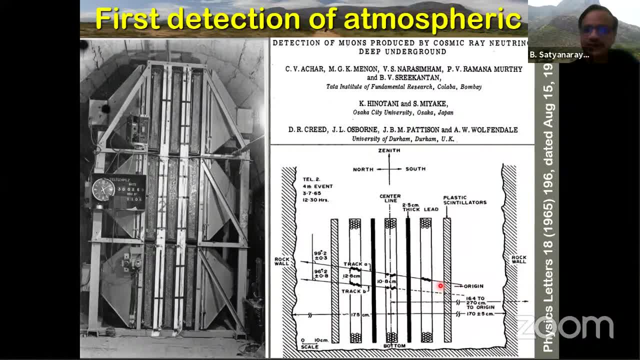 cosmic ray and neutrinos deep underground that was detected, and so this is so in some sense. of course, we are the definitely pioneers in neutrino physics. atmospheric first atmospheric neutrino was actually discovered, uh, in polar gold fields by tata institute and, uh, the group from basata city. 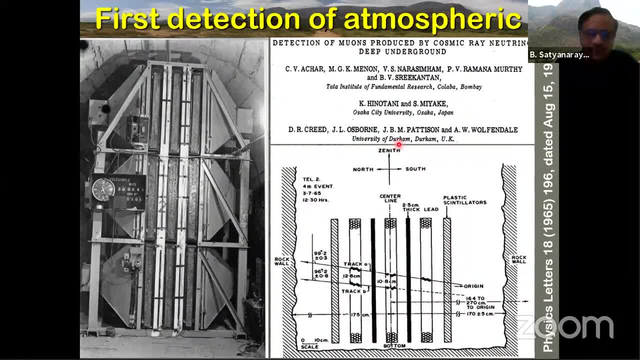 and their home. okay, now why i brought up and showed you these two interesting experiments, to kind of tell you that, uh, to do great physics, to do physics which is of potential, of noble price, you don't really, really require a great high tech or whatever. but what is actually important is the idea of how you design an. 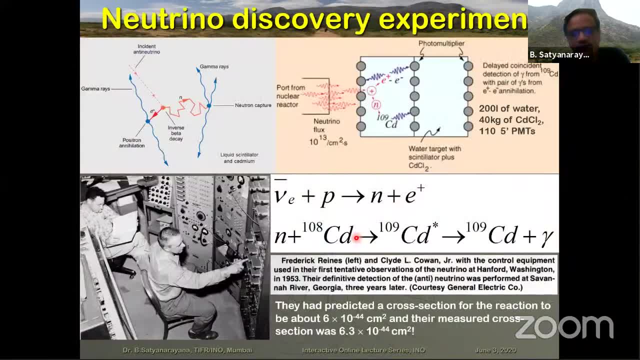 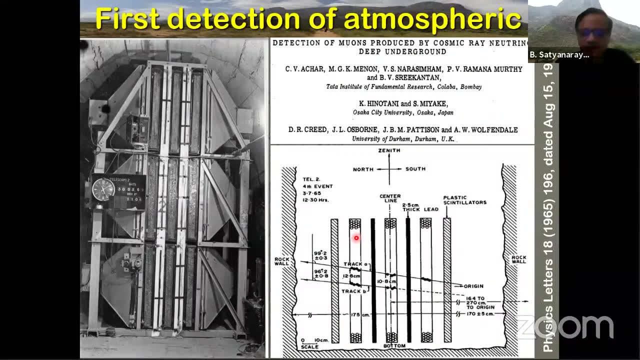 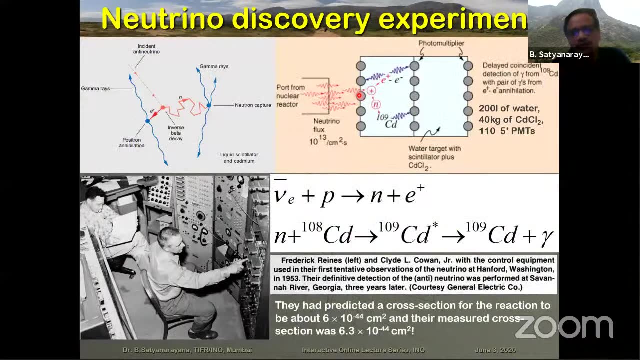 experiment, both these experiments, both- uh, you know- rhinos experiment, as well as kgf experiments, uh, the detection, the data acquisition, the electronics, etc. if you look at you will be surprised, because this one uses an oscilloscope to capture the signals produced by the prompt uh photons and then the delayed uh. 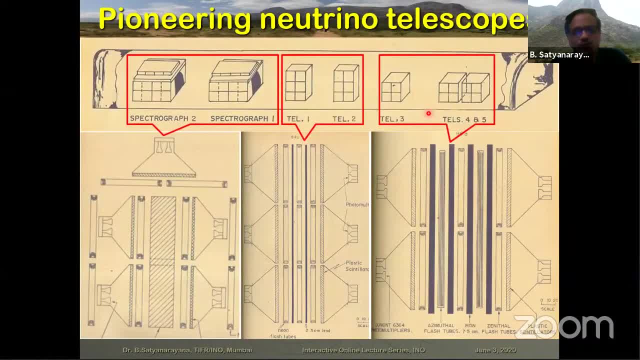 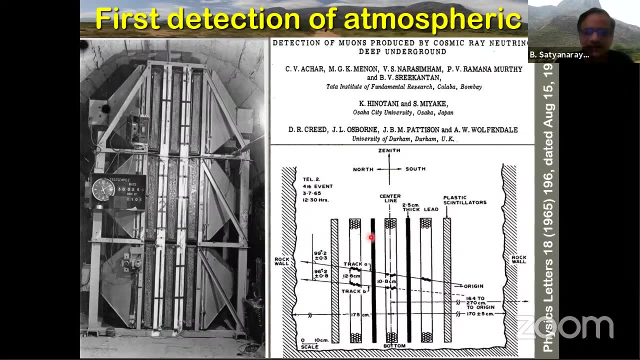 you know, the neutron capture, whereas this one actually uses ordinary camera- of course it's a mechanized camera- to to kind of capture the, the flashes of light that is coming from the- uh, the neon flash tube. so this is what i wanted to tell you. it's all depends on how cleverly 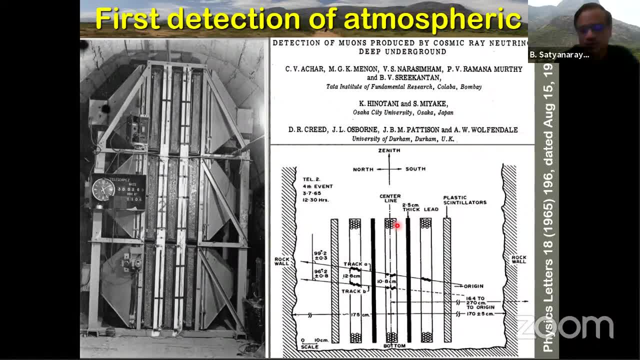 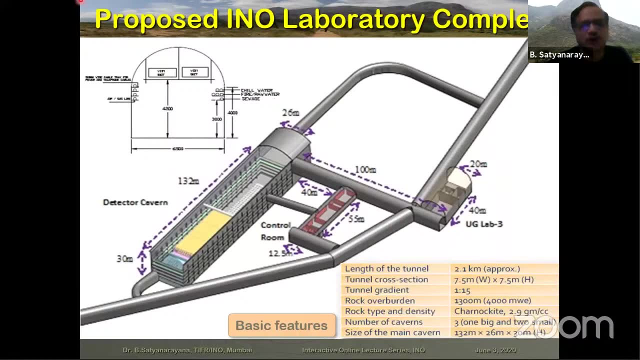 experiments. experimentalists put up an experiment. that is what is more important than really really using. you know, very, very high speed clocks large memories and whatever. so okay, so that is the idea. but let us now come straight to you know, decades later we are. we have proposed an ino laboratory. today's talk is, of course, on. 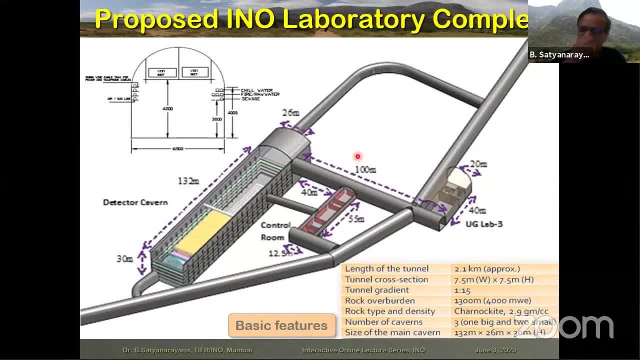 the ino project. uh, this is near uh. this is a. this is a laboratory complex we were planning to build. uh, you know uh construct between a place called uh bodhi okay, and the. it is about 100 kilometers west of madurai, between uh, between kerala and tamil nadu border. what we want to do is: 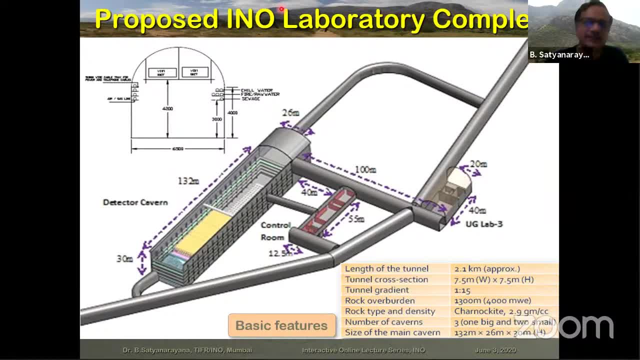 uh, if you can actually see on the, on the top there is a, there is a backdrop that is given a hill called west west border hills and we want to kind of dig a tunnel through that roughly about about two kilometers long tunnel. so this is the, this is the end of the tunnel, and then you build a. 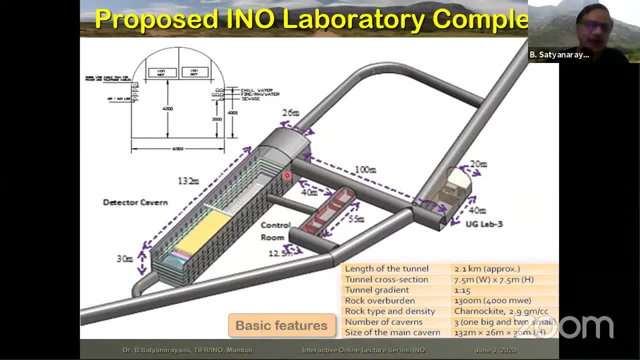 large cavern here. the cavern sizes are very, very large, about 130 meters long and maybe about 30 meters by about 26 meters cross section in which we want to house, if possible, two large detectors: one- what you see here in yellow color, is the one that we are going to describe soon- and there is also place for keeping another, constructing another. 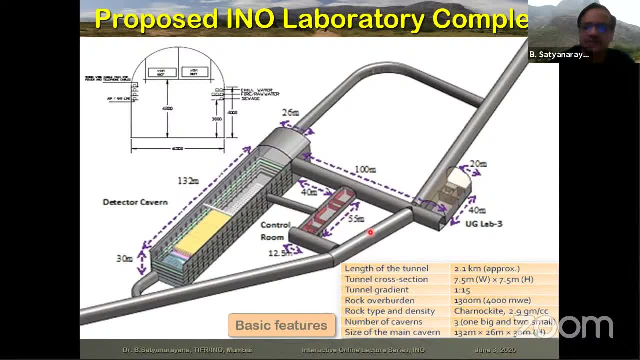 detector here. apart from that, there are also other caverns meant for other underground facilities, one here. it is expected to have a new, uh new to no less double meter decay experiment which, uh, sometime back professor vandana nana talked about, and here we would like also to keep a place. 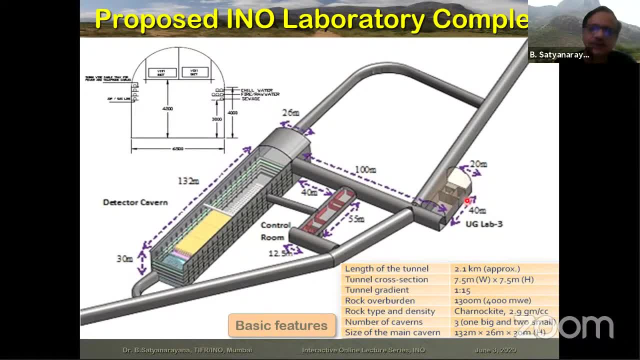 for the dark matter experiment. dark matter experiment, uh, you know, dark matter physics in fact was talked earlier the other day by boston. uh, so it's a tunnel, so i mean it's a large cavern cross section, so there will be two tracks. so you know, one truck going, one truck coming, that is the. 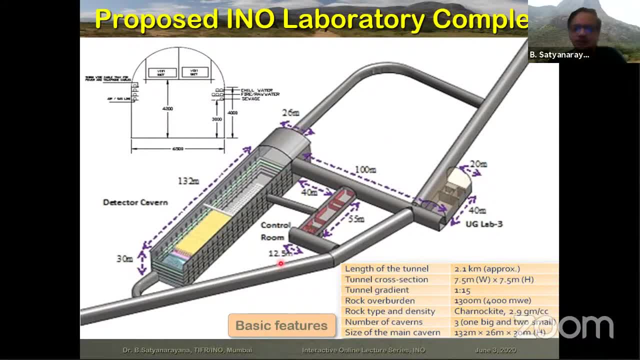 kind of size of this tunnel that can bring you here, and so this is a. this is going to be uh underground complex, not only for neutrino experiments, but also all futuristic experiments. uh, could be ndbd, could be dark matter, could be some material science, maybe geology, maybe some. 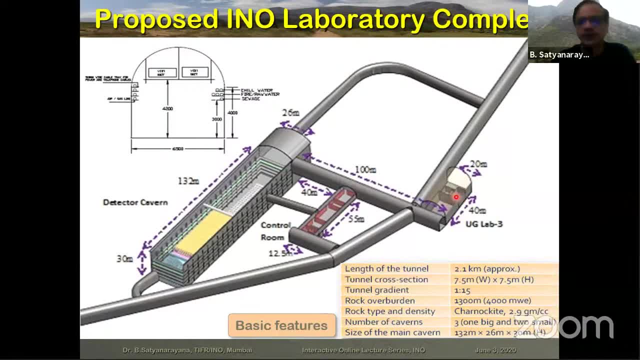 biology experiment. so this is a national facility where we wanted to bring, we want to build such a unique facility- uh, you know, at par with some of the best underground labs in the world. now, coming to the so-called iron colorimeter, which i briefly mentioned, where it is going to occupy this place. 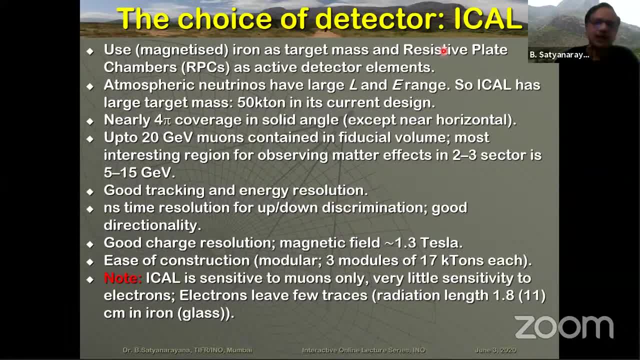 here. so this is actually, uh, why we chose this particular, uh, how we chose this particular detector. we wanted to, of course, use magnetized iron as the target mass for the neutrinos and use resistive plate chambers, where we describe in detail later as the active detector elements. the detector elements are: 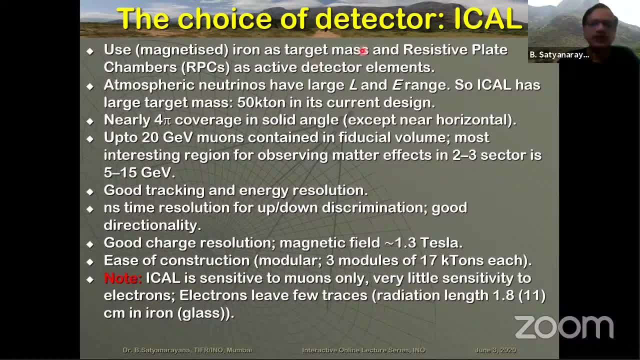 the ones which are going to detect the charge particles. when neutrino interaction take place inside the magnetized iron, which is target mass, of course we use at the source of neutrinos, we use atmospheric neutrinos and then we use the magnetized iron, which is target mass, of course we. 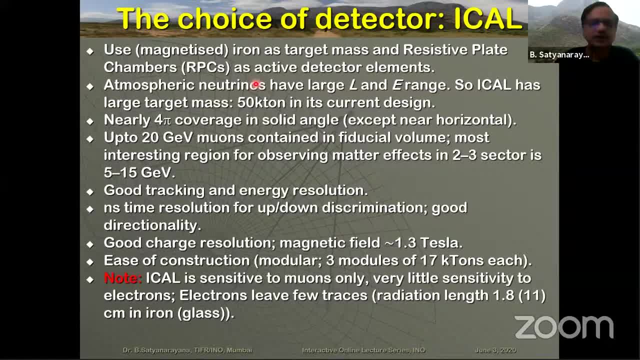 use at the source of neutrinos which are free to use. uh, they're not, you know, they're all the time there. they're available for us 24 hours, seven. and uh, since new atmospheric neutrinos have a large length, large l, and also the e range, which you must have heard many times about the when you talk. 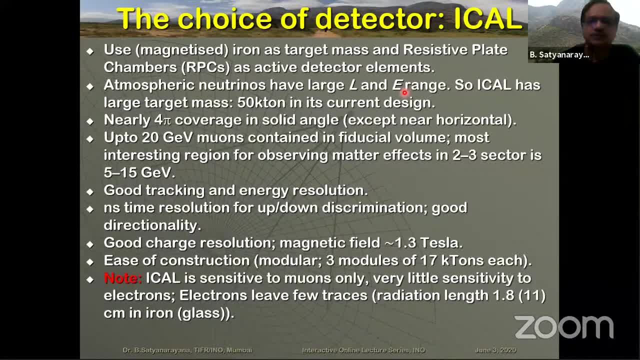 about neutrino oscillation parameters. you always have this um expression as l by e many speakers talked about. so the i cal, as will use very, very large target mass as well. so the, the mass that i'm showing there is of the order of about 50 000 tons in the current design and there is also place. 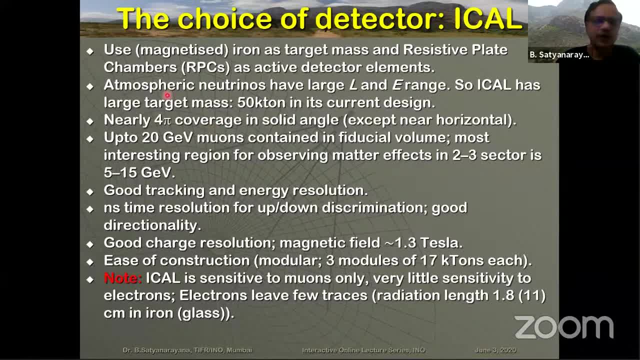 for another 50 000 ton detector if required. we want to cover neutrinos coming from all directions for five coverage angle. so we have- except in real of course, horizontal, because the way we build this detector here horizontally will be difficult to get the coverage now up to about 20 gb muons. 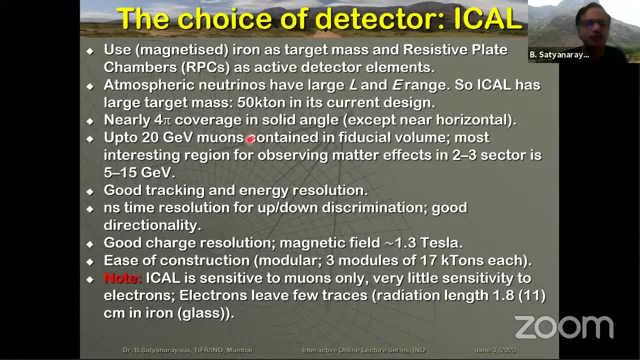 contained inside the detector, what you call fiducial volume and most interesting region out of the area, which is about, you know, about 1, 5 to 15 gb in the kind of sector that we want to probe. obviously, we want to have very, very good tracking, as well as energy resolutions. remember that we. 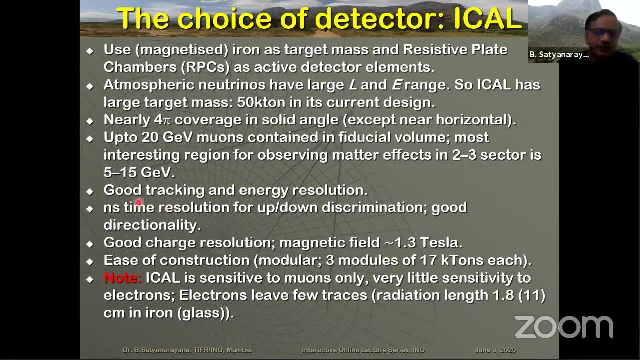 want to measure energy. also, we want to measure the length, so we require the tracking. we see these details a little later, so we want to get, uh, the timing resolution of, for you know, if you want to distinguish neutrinos coming from down or up, to discriminate and hence you want to get a good 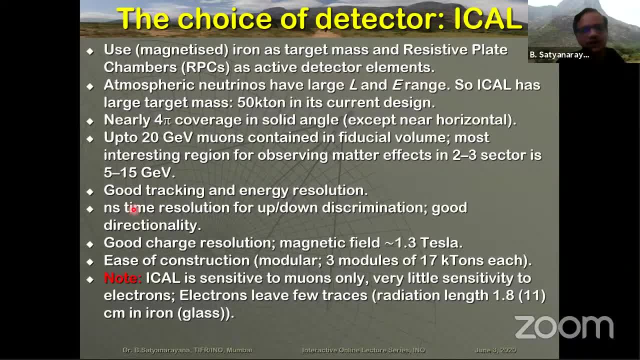 detectionality, you should be able to kind of track the charged particles traveling through your detector at a resolution of 1 nano. So this is like having a stopwatch Instead of having milliseconds resolution that you have in Olympics, maybe tens of milliseconds you. 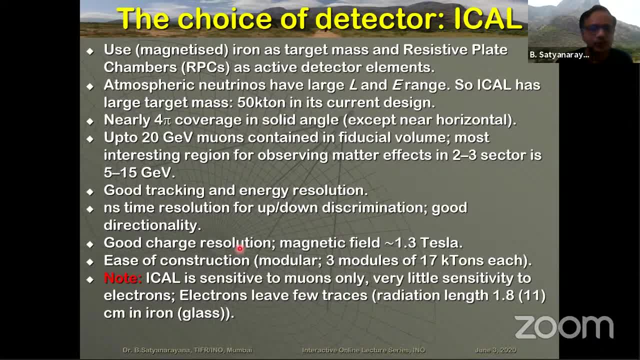 would like to have nanosecond time resolution. Of course you need to. this is magnetized detector So you will be able to get a good charge resolution, whether it's the charged particle produced or positive charge. So we have the entire detector is magnetized to. 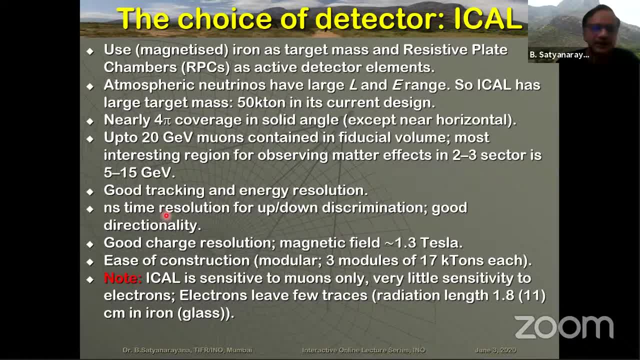 about 1.5, 1.3 Tesla. Of course, any detector that you want to use should be easily constructable. It should be modular. So, for example, we want to have three modules of each 17 kiloton. That is how we want to build 50 kiloton detector. So in principle, when the first detector is 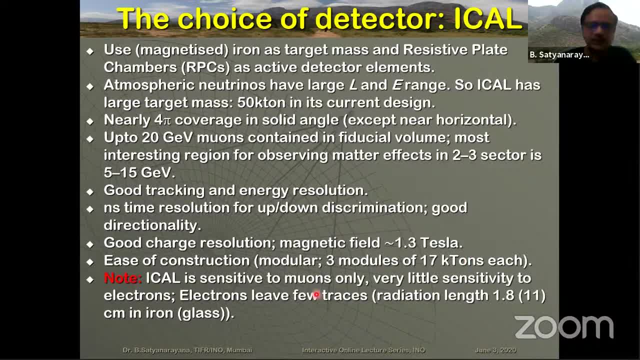 finished and operational, we can start then, you know, building the other ones and so on. And remember that ICAL, the way it is constructed, is mostly sensitive to muons and they're not sensitive at all to electrons, because electrons leave very few tracks in this detector, because we use very, very thick iron plates, right, 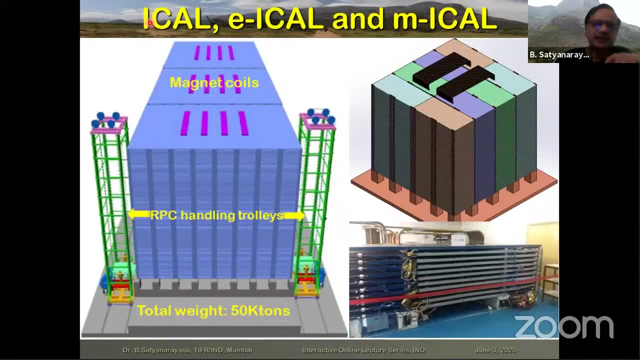 So just to give a very quick what these, all these jargon that we keep talking about, the big detector, the, you know, the dream that we want to build have is iron calorimeter. So that is how it looks this structure looks like. You'll see, of course, more details. 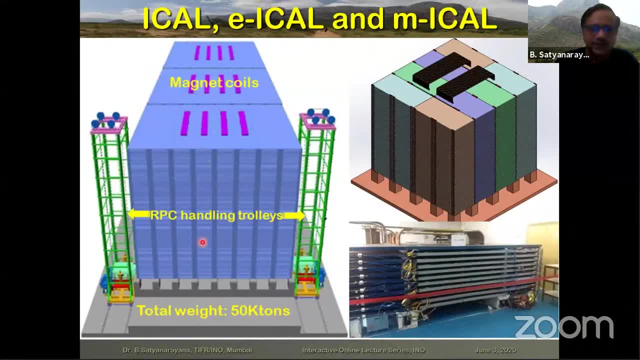 about this, but and the so-called engineering, ICAL. So, before we build the big detector, we want to build a prototype which will, which will enable us and give confidence that we can actually build this. By the way, this is what those three modules that I now 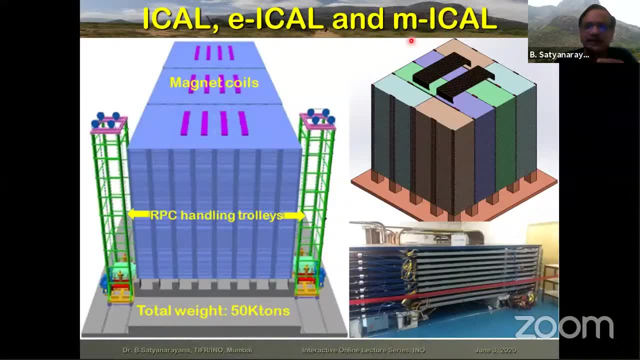 described just now And even before, that we want to build a very tiny, very, very tiny, so-called mini ICAL detector, which you actually see these two are, of course, is in the graphics, but this is real object that you see here And it is actually operational in Madurai. 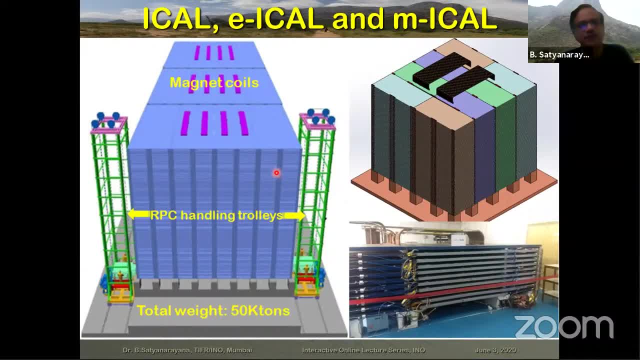 you know lab called inter-institutional center for high energy. So you keep hearing about these words: ICAL. ICAL is the is the final big detector that we want to build Engineering. ICAL is what is here, is the small one. You will see the specs very soon- And mini ICAL is what I said. 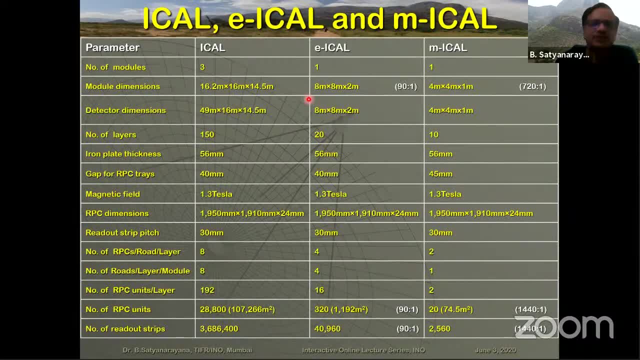 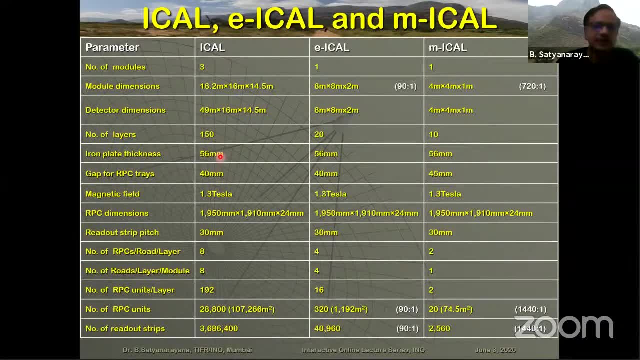 150, 150, 150, 150 layers of iron, which is about 6 million 6 centimeters thick. There's a gap of about 40 millimeters between the iron plates where you are going to insert the active detector elements. This is the magnetic field And Deepak mentioned about. 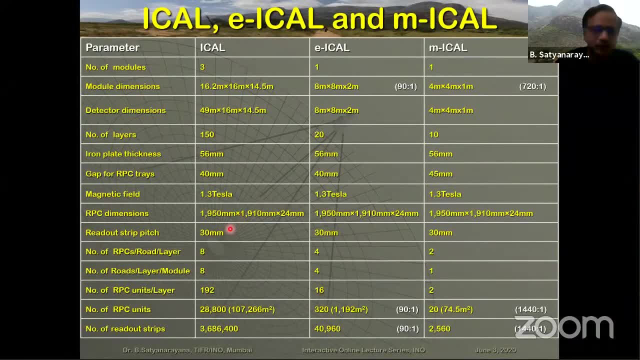 the resistive plate chambers roughly, nominally, of the order of 2 meter by 2 meter size, And you'll be able to kind of get tracks of these particles, Let us say at every three centimeter. Okay, You will see that actual resolution for the position will be much, much better. 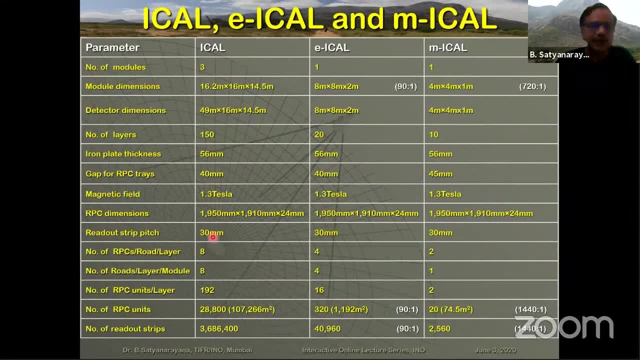 better than this, because this is one track. if you send me, I will be able to give you a position within three centimeters. okay, and of course there are other details here. but what is also important is when you, when you say that RPCs are your main active elements, the question comes: how many of 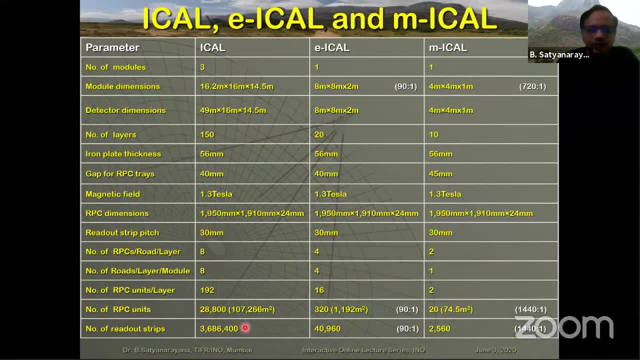 them. you know what is the total area that you are going to cover, because there are 150 layers of, let us say each one of them is 40. you know 50 meters by 16 meters. so if I have to cover them 150 into 50, into, let us say, into 16, you get 100,000 meters square okay of area. these are: 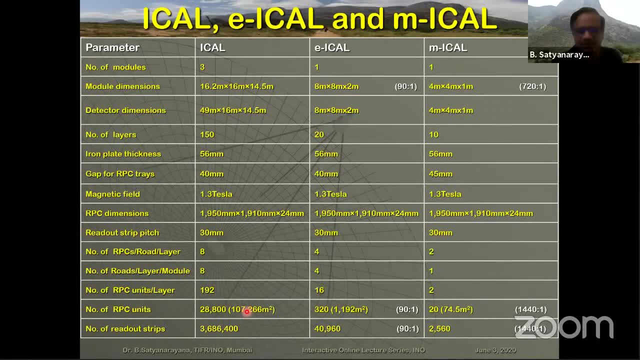 almost you know, 15 soccer fields instance- probably you will see that soon- and the electronics that are required to read this data is almost about 4 million detectors. this is you can really see how exciting it is to build, as Deepak mentioned, this experiment from a completely from an engineering perspective. okay, eCAL is even not 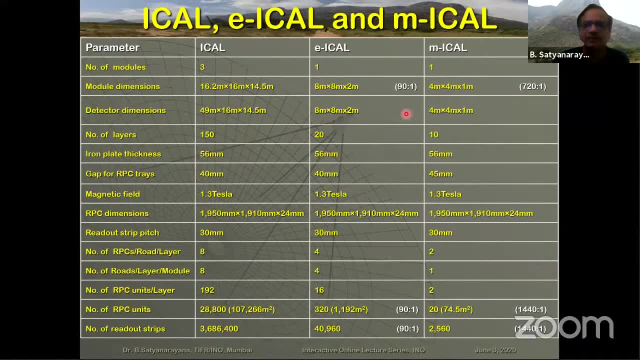 small. maybe, depending on which parameter you're talking about, it's maybe a factor of 100 smaller, but you will still need about 300 RPC detectors and about 40, 50 000 electronic channels. but you will see, all the elements that you are using are exactly same as ICAL. that is the meaning of. 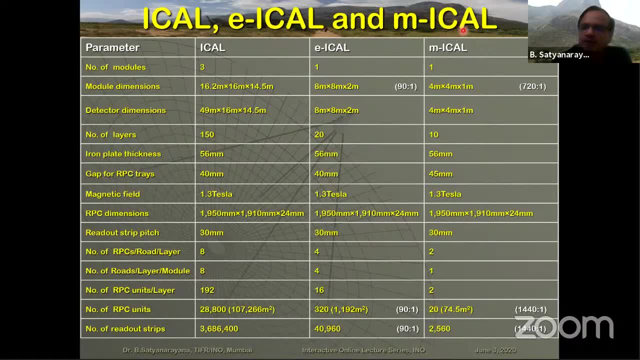 engineering like that, right, for that matter, even mini ICAL, even though it is extremely, extremely small compared to this big detector. but many components that you use here are same as engineering ICAL and same as final detector and you will use only just 20 or RPCs and maybe you will instrument not more than you know about. 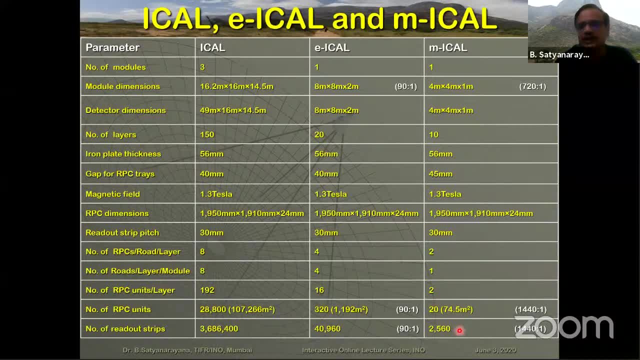 3000 channels. but you will be surprised to see, even such a detector can give you a fantastic physics, can give you half a dozen PhDs. so it is not something when I say small, small compared to this, but this experiment itself is, you know, reasonably involved, right okay? 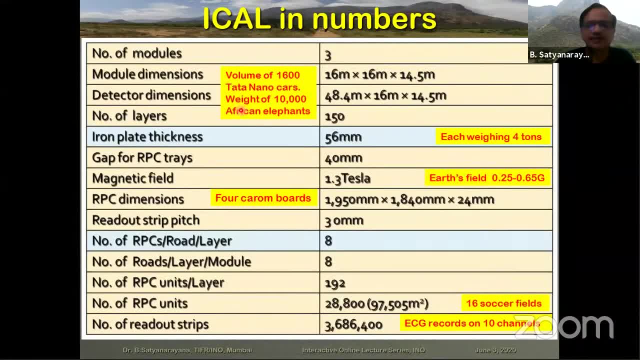 so this is an outreach kind of a slide that I usually make just to get a feeling: meters and kgs and tons and so on. what does it really mean? so if you want to understand in terms of how an ICAL looks like and you want to compare with data nanos or African elephants, this is how it looks. 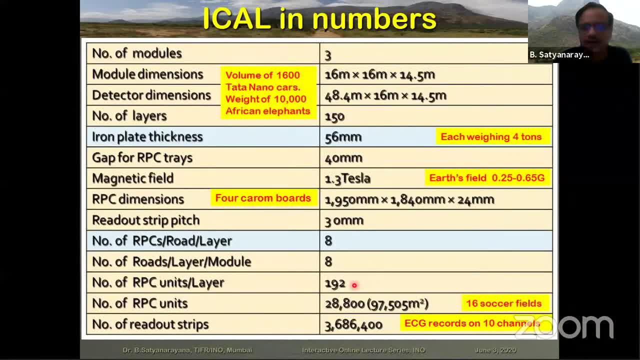 like right. and in case you still wonder how big this hundred thousand meter square that you are going to cover the RPC detectors, so I mentioned to you it is equivalent to 16 football fields that you are going to cover right and you, if you wonder what four million detector channels are, 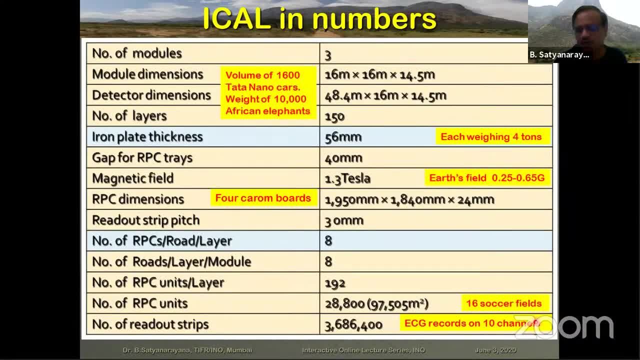 typically an ECG machine has about 10 channels on which the signals receive. you know, received and recorded. so now you can kind of imagine what is one is talking about. but if I tell you, compared to ECG signals, of course, these are about a million times more than. 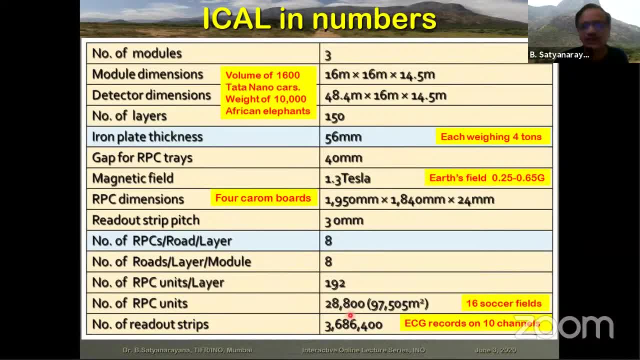 ECG number of signals, but also a million times faster compared to what ECG signals are supposed to be. so that is the kind of figures you should think in your mind when something is a little bit out of context. if somebody is talking about engineering, right? okay, so as I 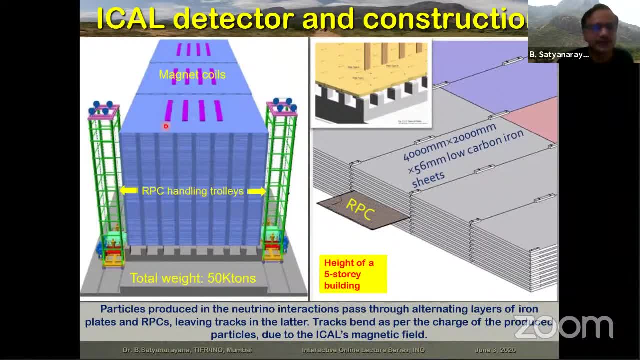 promised, I'll keep showing this detector again and again, but now maybe with a little more details. this detector is consisting of three modules, each one of them 150 layers. you can actually see, in case you wonder how big this is: this is the height of a five-story building. 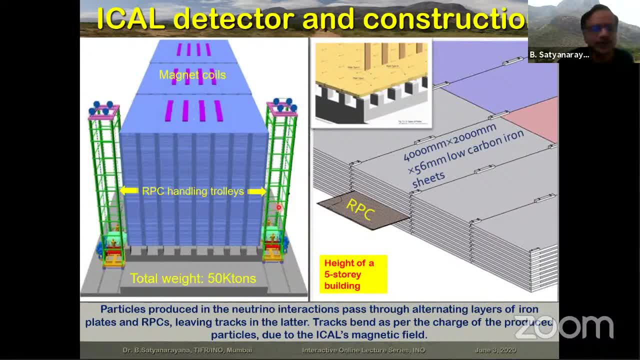 okay, and so you build one module at a time, and these green looking objects that you see on either side are, of course, trolleys by which you can maintain and install this detector. these are the two. There is a guy here standing in this trolley. you can see the size of this person and then 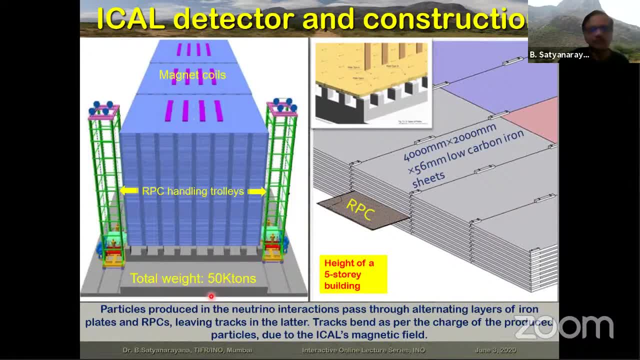 get a feel for it. And, of course, as I mentioned to you, this is about 50,000 tons of detector and these purple colored stuff here on the top are actually coils which go around the entire detector through and that is where you apply, you pass current and magnetize this entire detector. 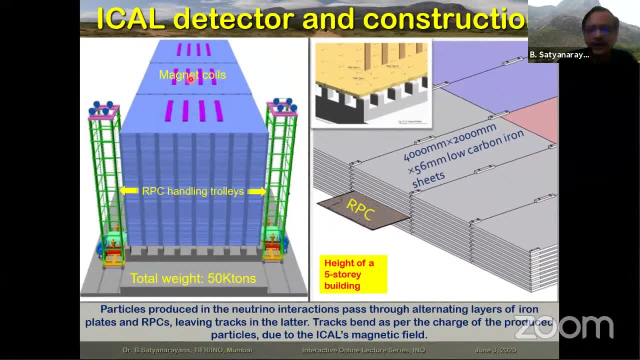 to magnetic field of about one and a half Tesla. So, as I said, the way you make it is you use iron plates which are about each weighing about four tons, and you know, four meter by two meter in area and about six centimeters in thickness, and tile them up one by one and you can actually see they are locked, interlocked. 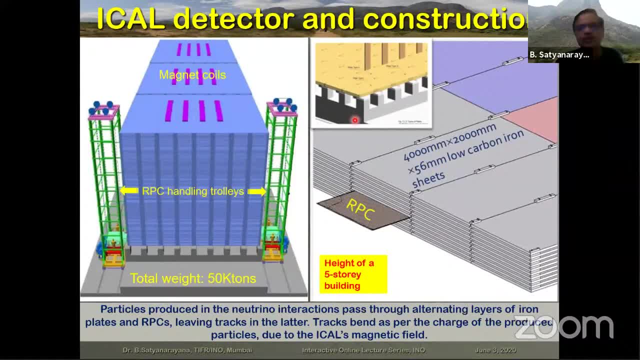 nicely each other. Such layers are, you know, initially put on top of a pedestal and then you stack them, but ensure that between each of these there is a gap of 40 centimeters into which, later on, you start pulling, Using the RPC detectors here. 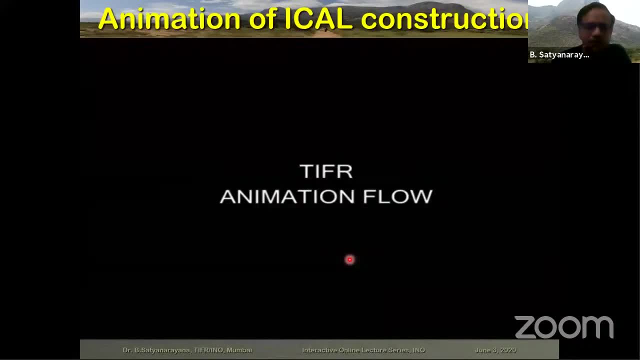 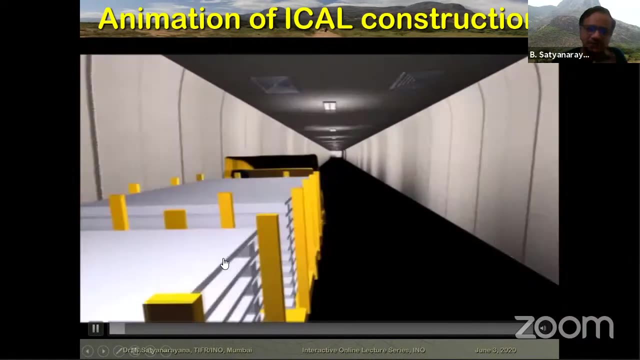 Okay, let me see if I can kind of show you. Okay, I can't find, I don't know why this. maybe I should. yeah, So just an animation to give you a feeling. So this is the 2.1 kilometer long tunnel which is actually through which truck carrying let. 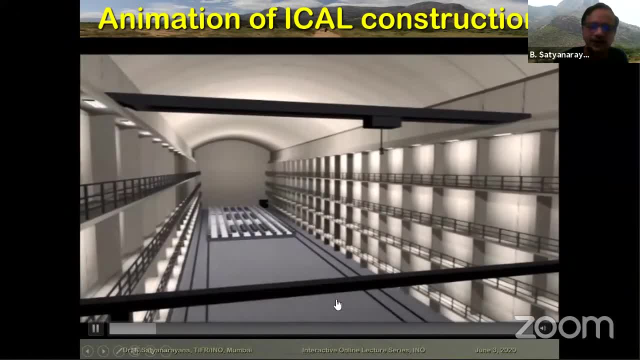 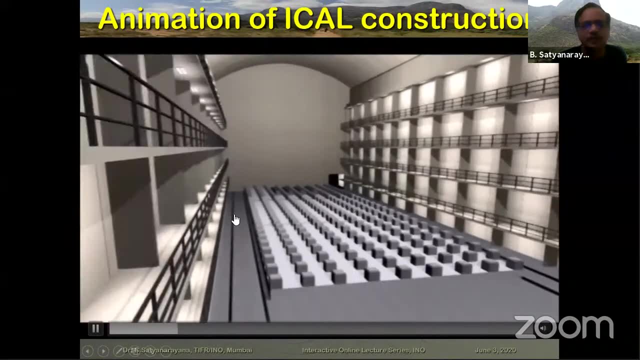 us say, iron plates are going and it is actually now parked at the bay where it is supposed to be waiting. and now you can already see that you have a concrete pedestals on which you want to build the first module and the second module and the third module putting. 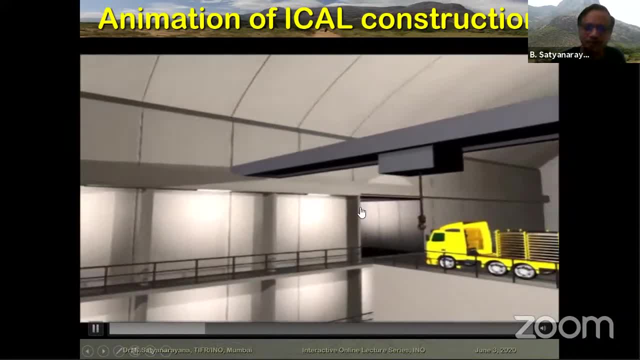 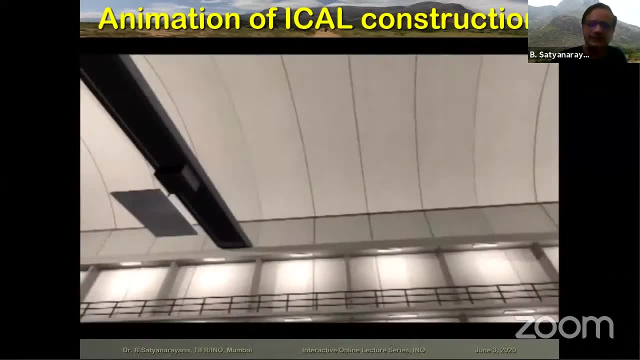 together and here you can see the iron plates are being picked up by crane and they are going to be placed one on top of other- and it is always built layer by layer, as I said, and then keeping spaces between each one of them to ensure that later on you can insert. 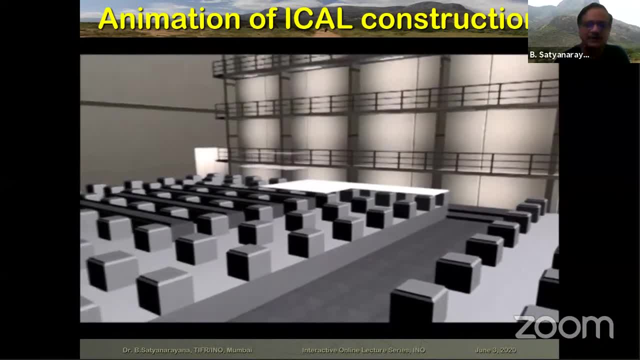 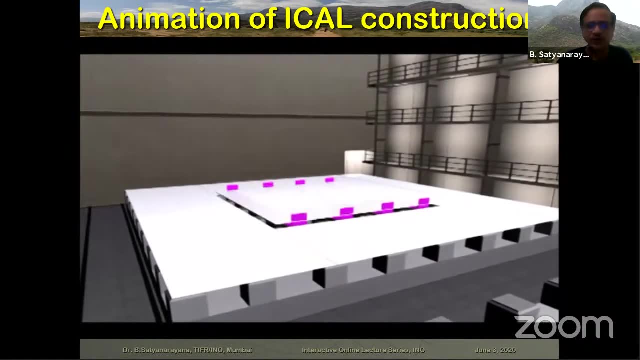 the active detector. Okay, Of course. So you can see every tile and every layer is put in few seconds, but it takes three or four years to actually build even one module. Now you can see the purple color stuff. the magnet coils have already gone in, and so these 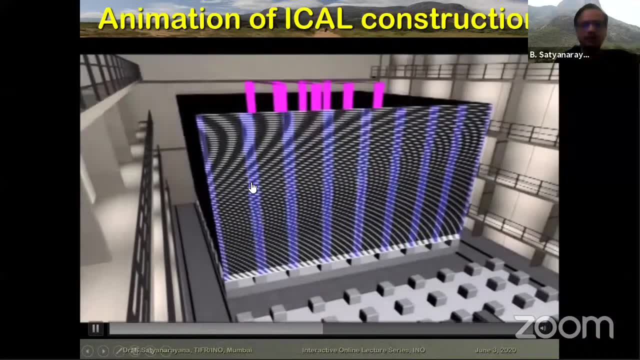 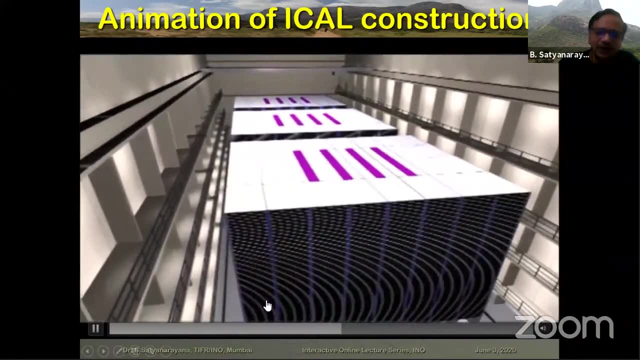 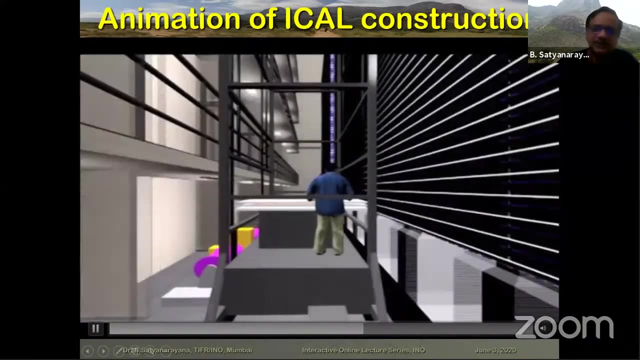 iron plates are special because you can, you know, kind of push through them the copper coils and you can see very quickly. the module two and three has come out. Now these guys are actually taking in a trolley the fully fabricated particle detectors for resistive plate chambers. 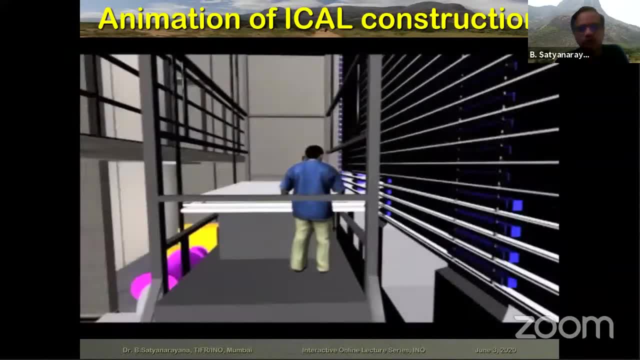 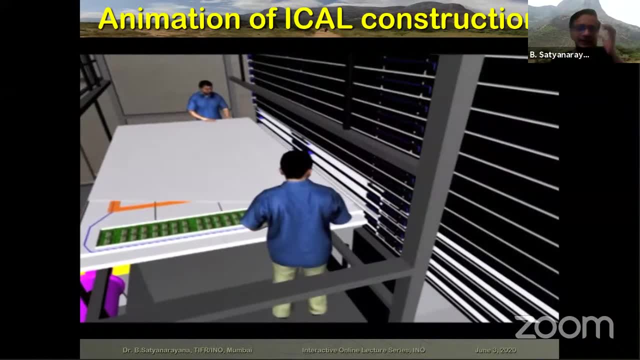 Okay, And they are actually pushing, you know, those into those gaps like a pigeon holes, one RPC at a time and then they'll go to the next one, and next one, and so on, Okay. So, as I said, the whole animation of course lasts only 10-15 seconds, but it's a long process. 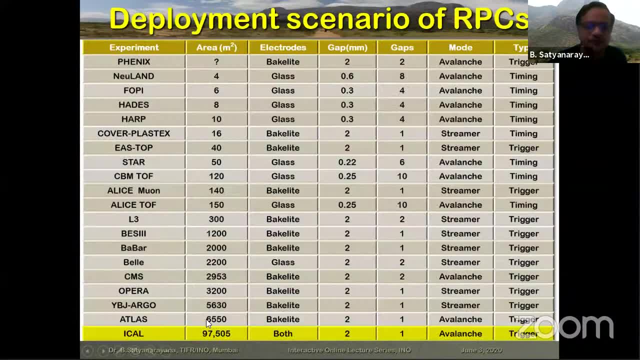 when you want to build such detectors. So this is what I kind of wanted to give a feeling like: when you talk about large RPC, large area RPCs, you are going to use in a big number, how big this big is. So, if you actually see, I prepared this sometime ago. 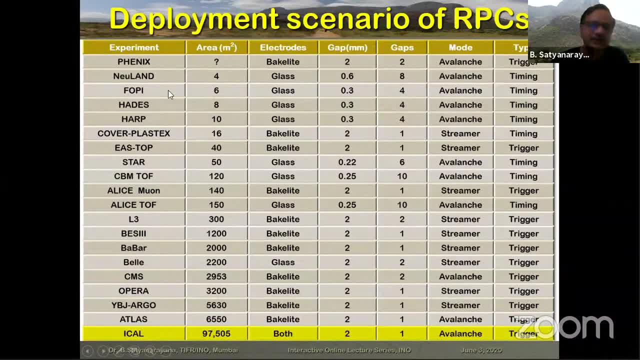 It's a slightly old, old slide but nevertheless it shows the purpose. if you look at all these various high energy physics experiments, cosmic ray experiments, and what is the area of those RPCs that were used, and you can really see it here. you know, compared to even the biggest, 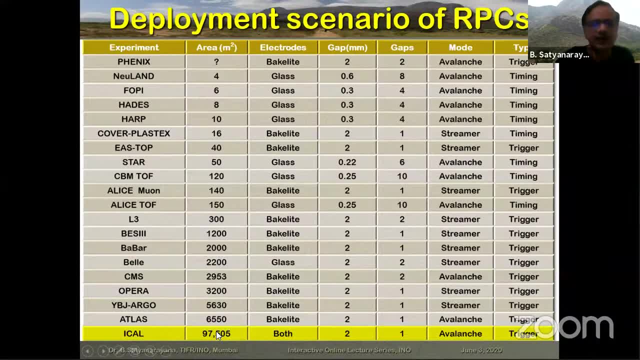 deployment of RPCs in the LHC. it's actually a factor of 10 larger than that, and of course there are many differences depending on what is the electrode material. most people use glass or bacilli. What is the gap between The? you know the, the glasses, and how many gaps, and you know modes and so on, so forth. 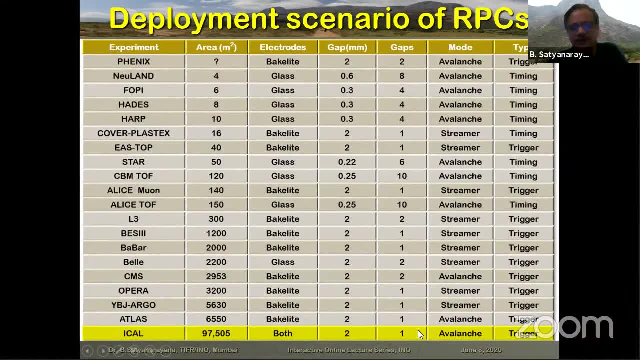 We'll talk about it, but please remember. so this is the kind of challenge that you have, and so the R&D that has started quite some time back, almost 20 years ago, obviously, there was no RPC in the country and we really had to start from scratch. 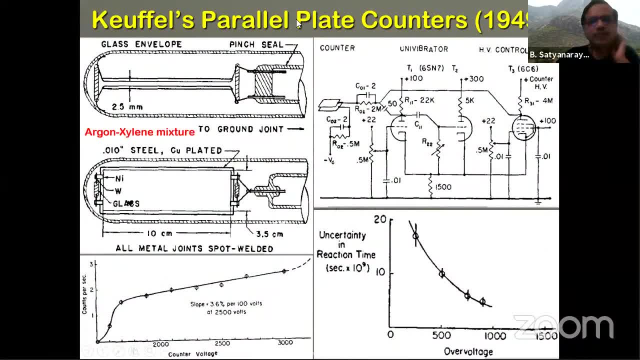 Okay, What is RPC? It comes under a class of what you call parallel plate counters, which are actually started, really you can say invented by Okay, By Cofell in 1949.. These class of counters are called PPCs, parallel plate counters. and imagine, at that time he. 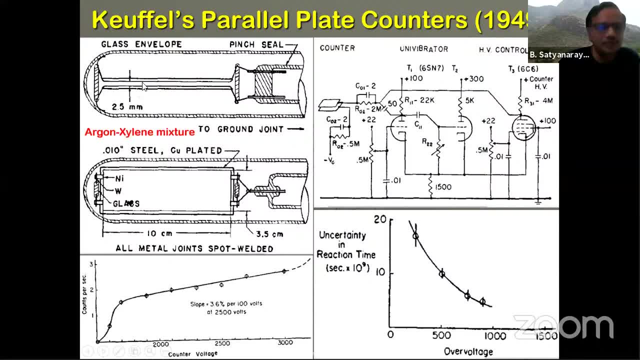 was actually talking about maintaining, you know, machining of 2.5 millimeters gaps, and of course this is a very, very classic experiment. but what I really want to show is not all this complication, but look at even the- you know what they call- that time uncertainty. 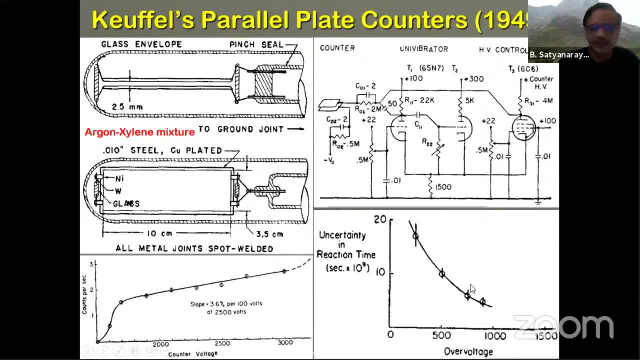 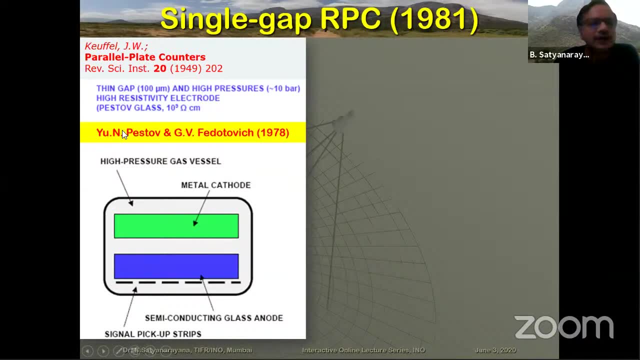 in reaction time. something like a timing resolution that you are talking here is actually is already coming as a function of the voltage hitting. you know kind of nanosecond kind of resolutions at that time. So what? okay, these are Cofell counters, but little later Pesto actually picked up this. 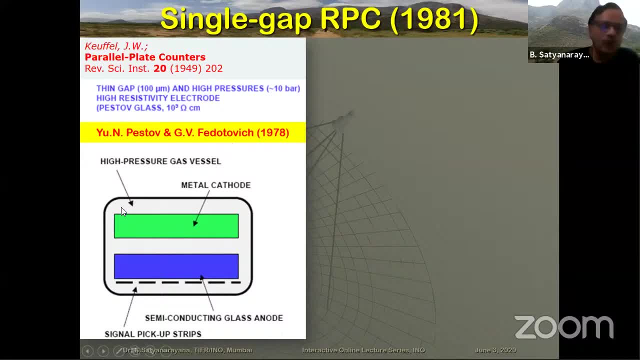 idea Pesto and you know, Fedovit. what they built is a chamber, something like this, which is also a parallel plate counter, but remember, this is made into a chamber- and which is which is, you know, at very, very high pressure, about 10 bar gas pressure. 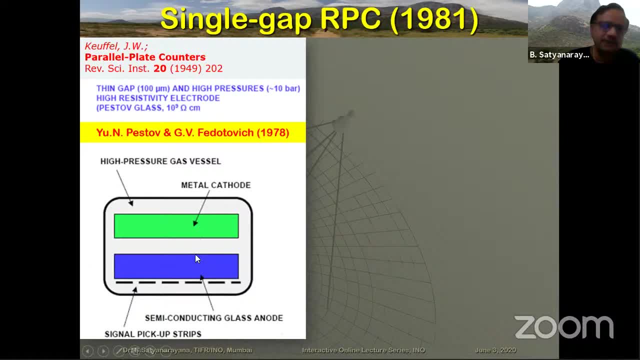 Okay, And they maintain the kind of gap to be very small, only about 0.1 millimeters, and applied, of course, potential across these two plates and these are your signal pickup strips. So it works beautifully and gave resolutions of the level of, you know, 100 picoseconds. but 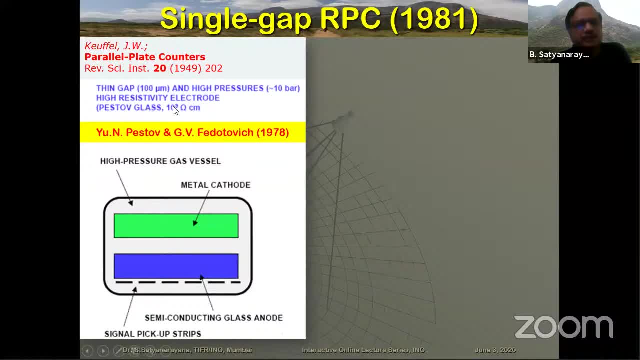 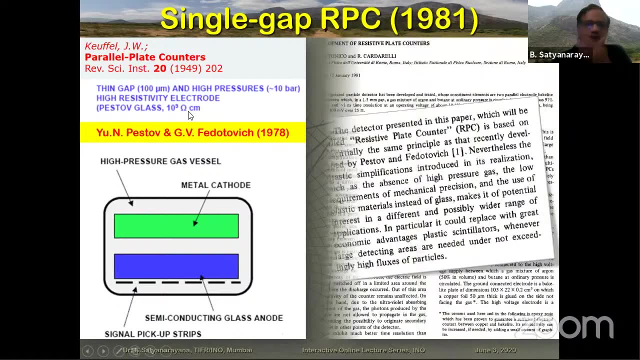 the problem with this is obviously how well you can maintain this mechanical accuracy and how to maintain that such a high pressure and everything is a big problem. So what this People here who actually called you know kind of father of RPC device now is Santonico. 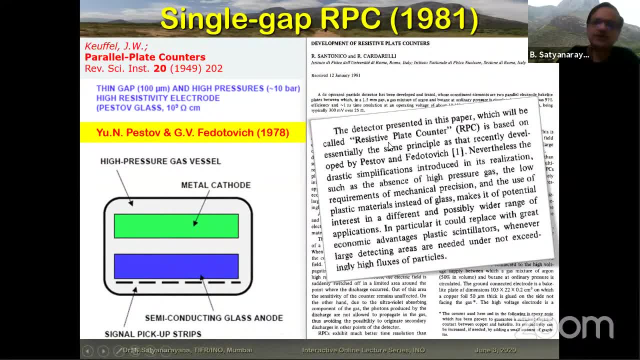 and his colleague did in 91 is actually- you can hear from their words- the detector presented in this paper. this is a- actually the. you know the classic paper is same as Pesto counters, except that they made it a big. you know simplifications in terms of using the cheaper materials and 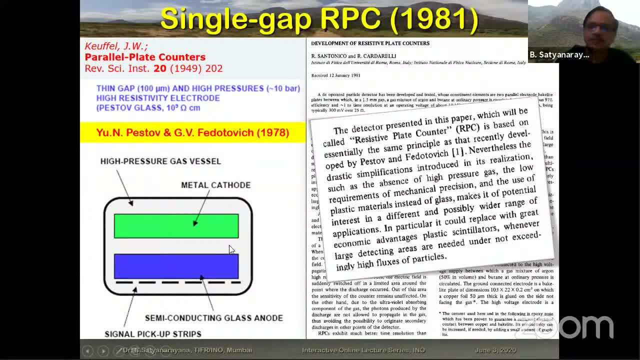 you know, instead of operating at 10 bar- Okay, They try to operate it at- let us atmospheric pressure close to atmospheric pressure, and you know, then it become a cheaper device, it become very popular. but otherwise, you know, it is very similar to this detector that is actually built by Pesto, and it is. it comes 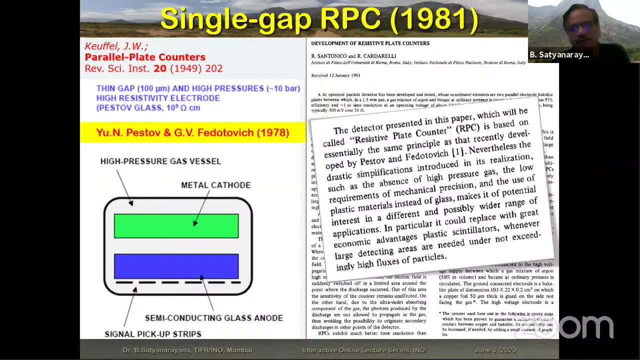 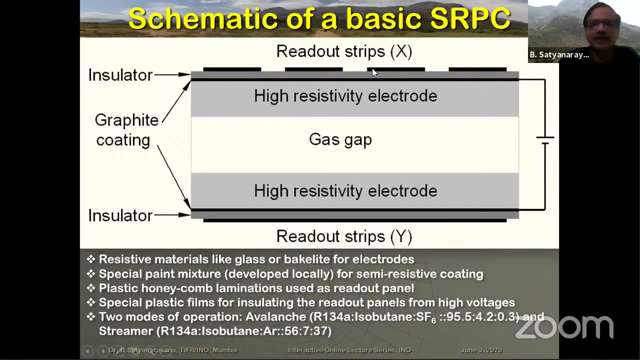 under what you call parallel plate avalanche counters. So just give you a very quick schematic of the basic single gap. as for single gap, RPC is, you take two electrodes, very high resistances. High resistive electrodes could be glass, could be becalite as you like and keep maintain. 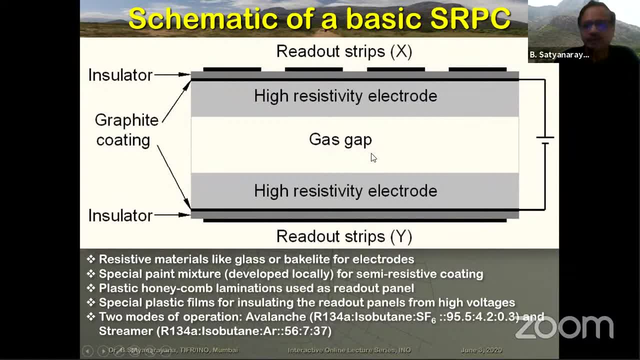 a gap of, let us say, if it is three millimeters and gap maybe two millimeters, you will see how it is made. and then, on the outer surface of the glass, you actually apply some kind of a graphite coating on which you apply a potential and which is what produces a uniform. 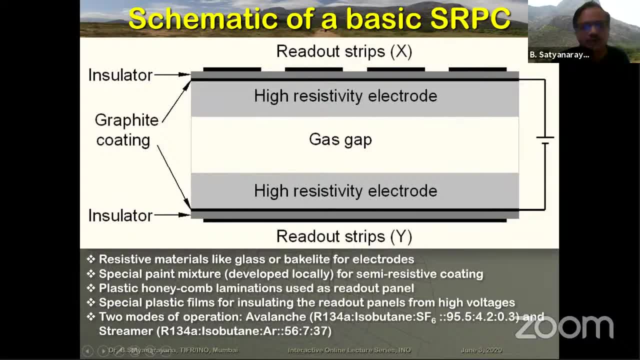 field, between the electrodes and you flow a special mixture of gas. there are two gas mixtures that I noted down here. Either you use: R134A is a freon, isobutane and SF6. this is in this proportion and there is an also another mode, which is called argon, isobutane and argon. R134A, isobutane and argon. 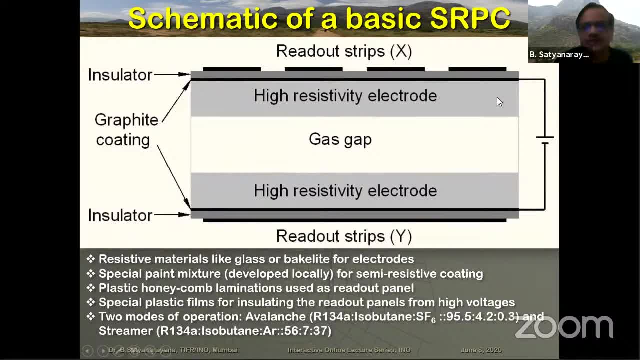 Okay, Now, outside this high voltage plane you actually put an insulator and then put your so called pickup strips or readout strips. but please remember straight away that the so called strips which are given as X, readout strips, which are given in Y, they are orthogonal. 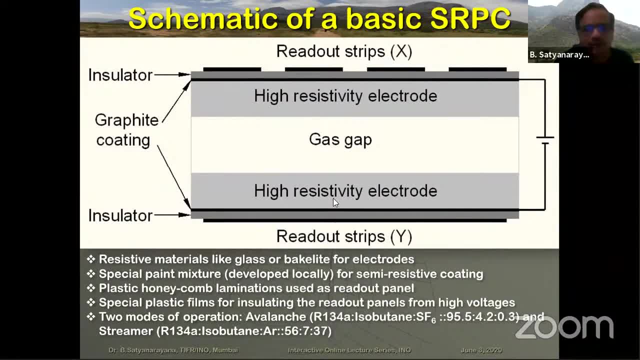 to each other, which means if there is a charge particle passing through and, you know, producing a, let us say, signal, we will see how it is. I am able to kind of pick up a signal both on X direction and Y direction or, you know, like a cross wire. 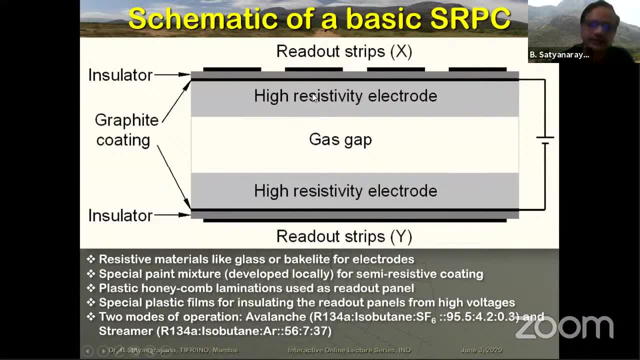 So with one active medium detector I am able to kind of give you both X, Y position of the charge particle. So it is very nice compared to, let us say, solution where you have a charge particle. It is a solution where you have an X plane detector, you have a Y plane detector and 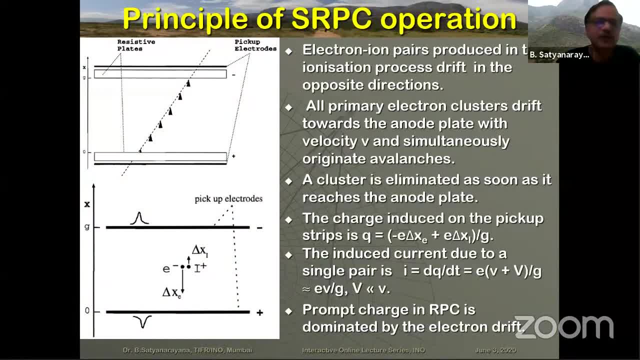 so on. You do not have to do that. So just to give you a very simple principle. so if you see a charge particle passing through, of course this is the gas mixture that I talked to you about, and so electron ion pairs are produced in the ionization process and they start drifting. 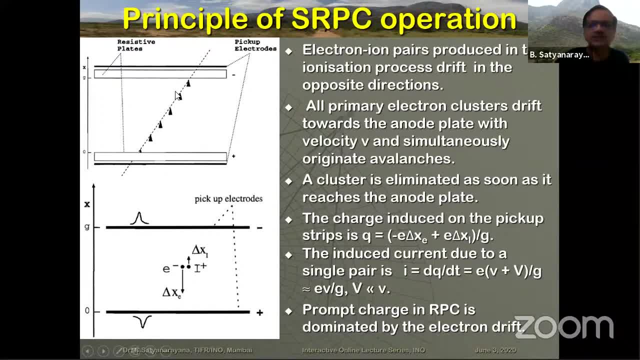 Okay, So the electrons, of course, come towards anode, and then the ions traveling in the opposite direction. Now, So the primary electron clusters, as I said, they start drifting with, let us say, a velocity v, simultaneously, and as they go along, of course, they do, furthermore, have reached, let us say, 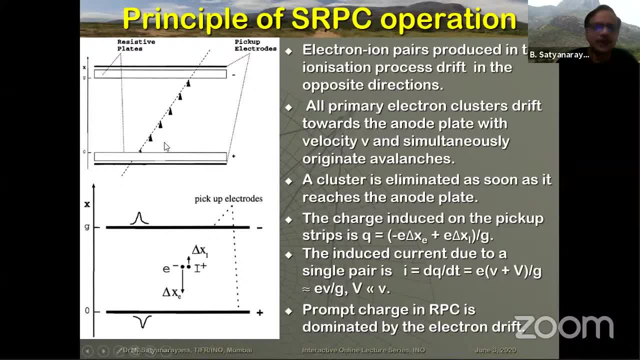 anode and it kind of is eliminated. Now, the charge due to this which is induced on the pickup panels which are, As we saw, maintained on the outside, it may be given as, let us say, as given by the electrons and as the given by the, let us say, ions, right, and they will be traveling, let us say one. 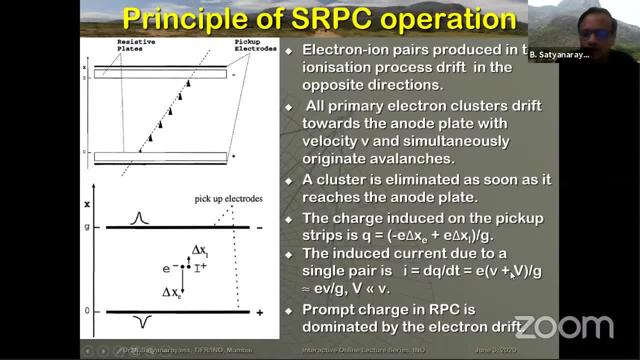 at a drift speed of v and the other one small v, and the other one is, let us say, capital V, But ions, of course they travel much smaller. so you might say that the current which is induced on the panels- here is excellent- Is almost entirely due to electrons. so therefore you can say: this is the electron charge, this 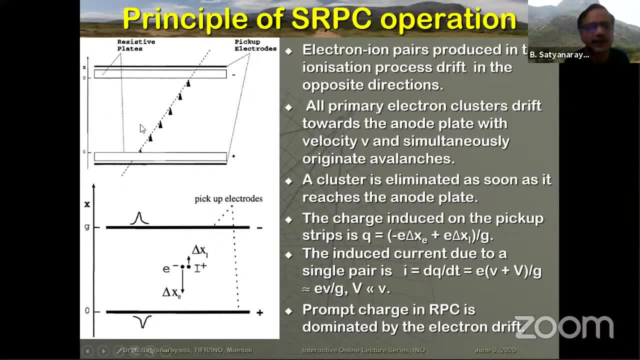 is the drift speed and the distance that you have, the gap you have between the two electrodes, which is, you know, what we call either two millimeter or three millimeters, as they propagate. Okay, So the charge that is induced, the signal that you are actually getting on the pickup panels. 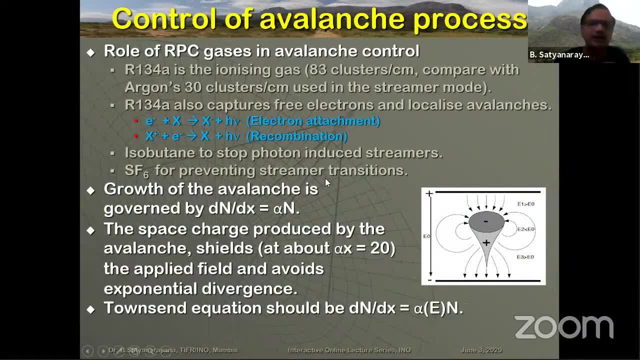 is mostly contributed by electrons here. Okay, A little bit about the dynamics of how you actually control what this avalanche that happens. you actually use, as I said, a three mixture gas. you use R134A is the mainly for ionizing gas and you use same R134A is also is an electron affinity gas which can also. 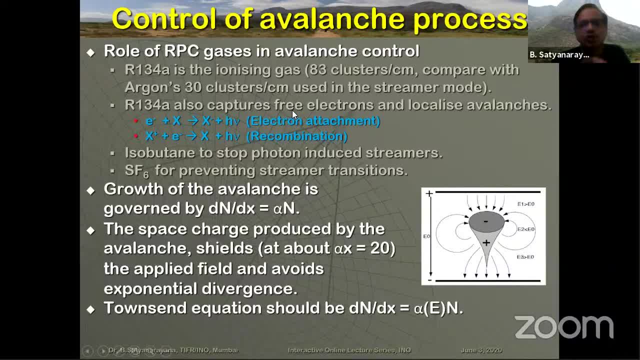 capture the free electrons which are produced and you want to localize the electrons rather than you know spreading the ionization to the entire, let us say, chamber, which is never a good idea, Because then you miss on the position resolution capability. Now there will be these two reactions also keep happening. I mean there could be electron 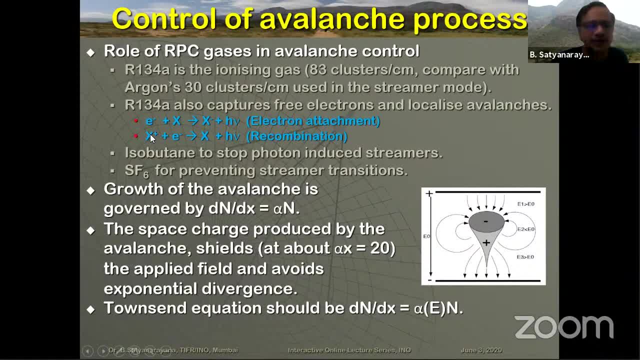 attachment which is actually given here. it could also be recombination of the ions and electrons which are produced especially before they start taking off their journey. In both those cases, you will of course produce, you know, photons, and those photons can actually induce streamer if you don't contain them properly. 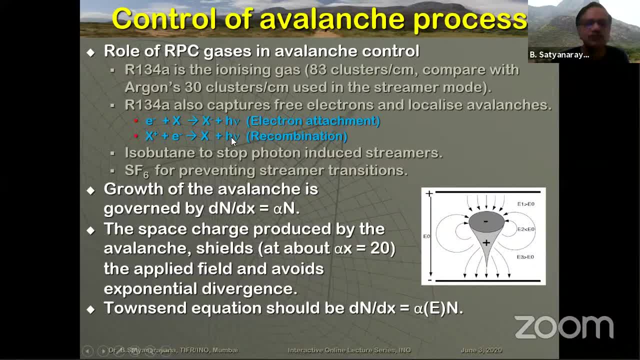 So isobutan is actually used To kind of kill these photons, which are especially at high energy photons, so that they don't again produce further stream, further ionizations laterally in the gap. and SF6 is actually used also to contain the gain of the gain of the detector, so that you know the streamers are. 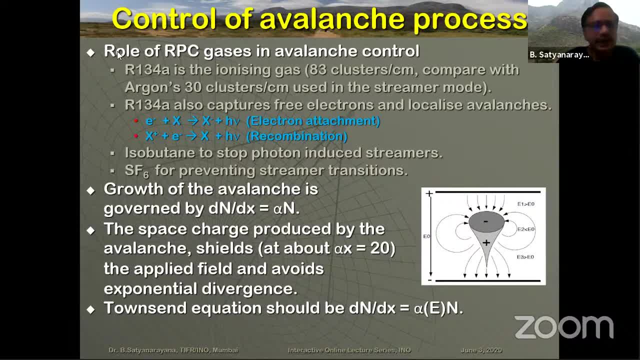 maintained, the streamers are avoided. So the gases you, these three mixtures of gases, you use in some proportion, which obviously you have to do studies to optimize it Such that That you get good gain. at the same time you also avoid streamers, and you know and things. 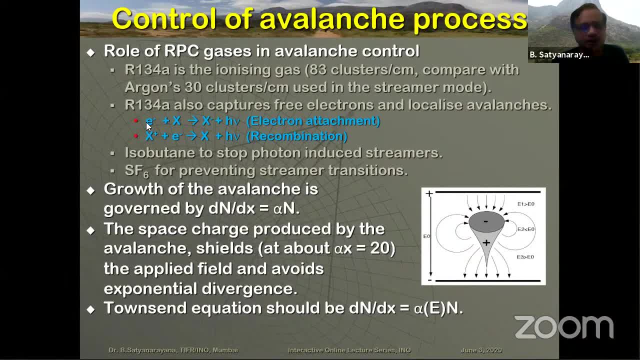 like that where, because it can spoil the longevity of the detector as well as spoil the position resolution. So you have to really play with these two parameters, which are, of course they are governed by so called Townsend coefficient and attachment coefficients. Townsend coefficients are, of course, the- now the distance before it travels and hits to the other gas molecule, and the 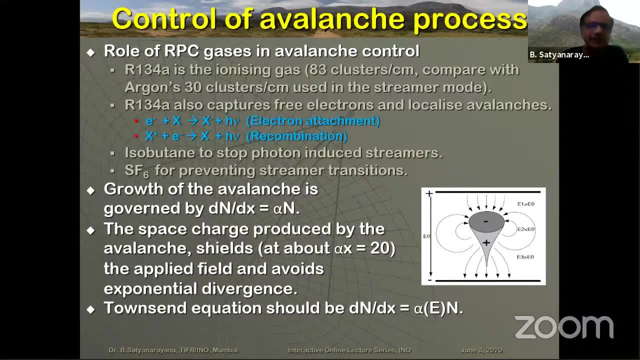 attachment coefficients are. you know what are the number of attachments that happen for the unit distance? So obviously, the effective Townsend coefficient is difference between these two. Now, when you say that how I am actually going in terms of the avalanche is actually decided by the rate of number of number of electrons that are produced, which is of course proportional, 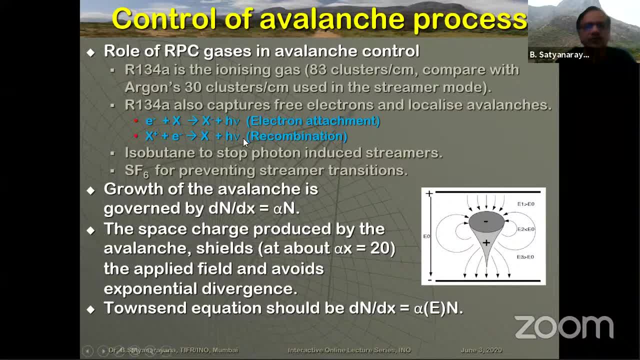 to the, this alpha, and also then is the number of primary ionizations that take place. Now you want to make sure that this phase charge, which is the phase charge which is produced because you are producing the big cloud of electrons, they themselves are moving, which is actually influencing the so called in the uniform field that you applied by applying 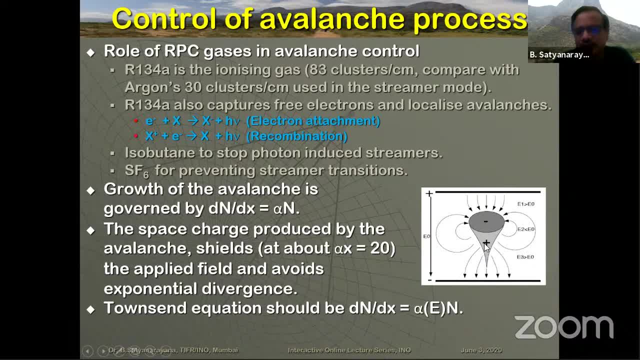 voltage across these electrodes. but at the same time, depending on whether you are talking about close to the electrodes here or close to the way the electron cloud is transferring, the fields are quite different in this area. in this area, where it is larger than the uniform field, and at the center, of course, it is slightly smaller, 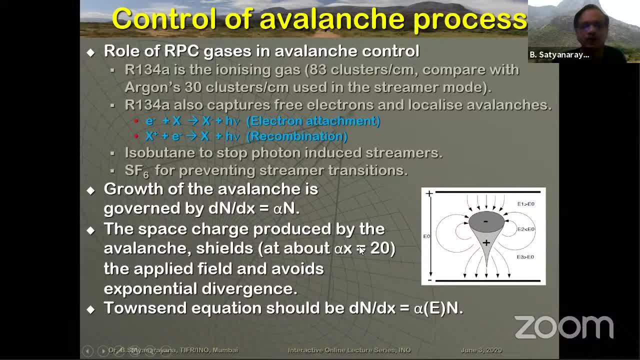 But you want to maintain that you don't want to reach the limit and you want to maintain the avalanche growth in such a way that they don't become into discharge. So in a way, the Townsend equation- though we say it's alpha n but alpha itself is depends- 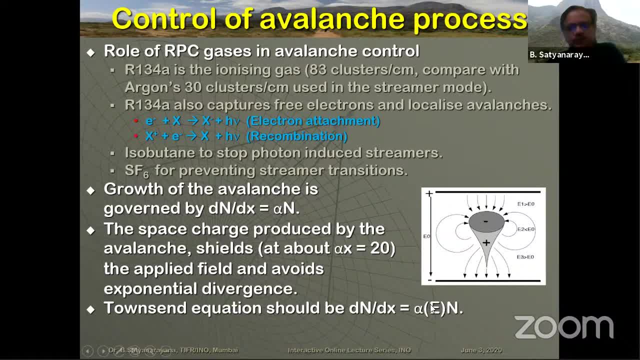 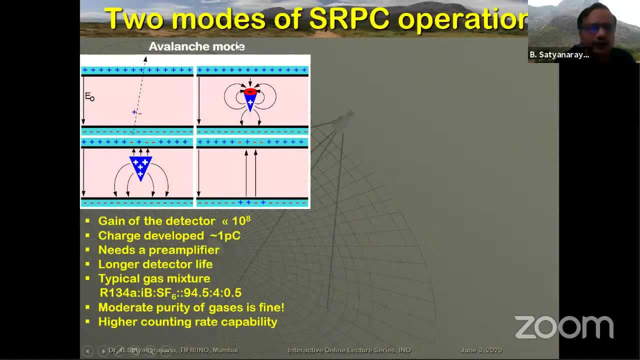 on the field. So therefore you may have to say as alpha e, n. Now, the same RPC that you built, the way we have described, can be operated in the so called avalanche mode, which is a proportional, semi proportional mode, which means that I Operate with the gas mixture in the high voltage in such a way that, when the ionization taking, 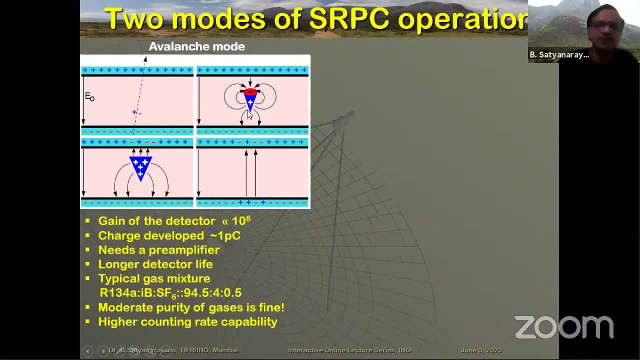 place now you saw that picture that I described before, and then the, the avalanche starts kind of moving and when the electrons move to the, to the anode, of course you can see that you already, you can already see that you started neutralizing very, very tiny place here and 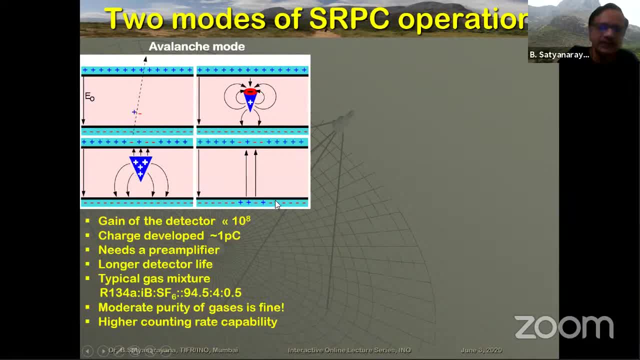 the, the ions of course reach much later, and then when they reach the anode, the cathode, here you of course get The. You can see that some of this local small area get neutralized. now when, when that happens, you will see the field which was at whatever you applied, uniform field, and if this field 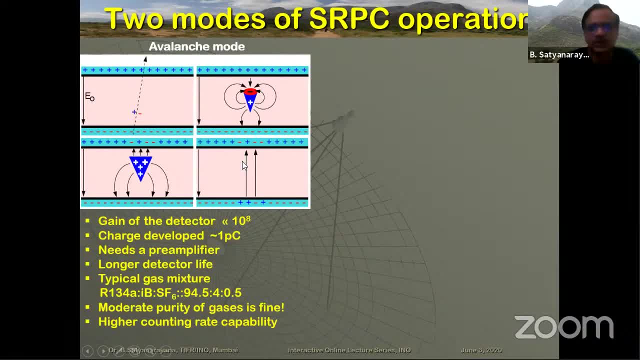 has dropped down suddenly, then you will find that the avalanche actually stops Now, as as the as the flux inside is actually now varying- electrostatic flux- because one is of course uniform field, the other one is the field that is produced, a change of field that is produced. 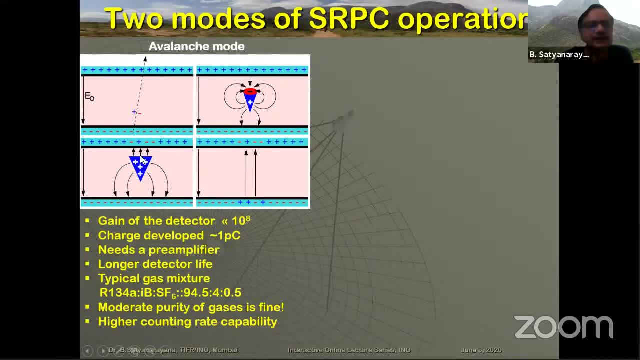 By the change of the movement of electrons here, and that change of flux in the electrostatic flux is what is actually inducing signals outside the electrodes, using Ramos theory. Now, in the avalanche mode, the signals that are induced on the, on the, on the pickup panels here, are relatively smaller, of the order of about one picoh volume, and this we say. 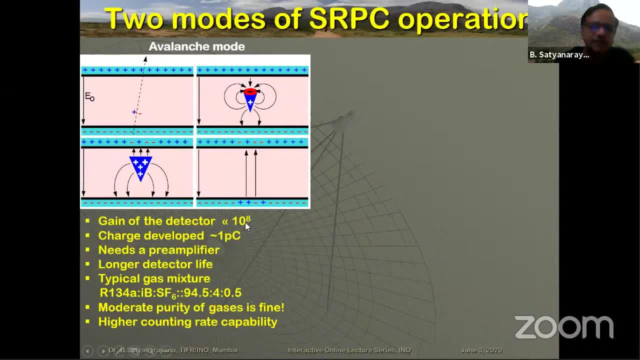 the gain is. that means, compared to the number of primary electrons, what is the total total avalanche that happened? It is of the order of about, I know, one-tenth of a billion. of course, these are good in the way that the charge is less because it increases the detector lifetime, but the signals are. 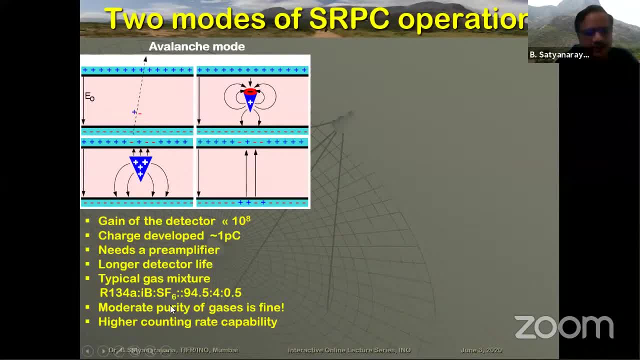 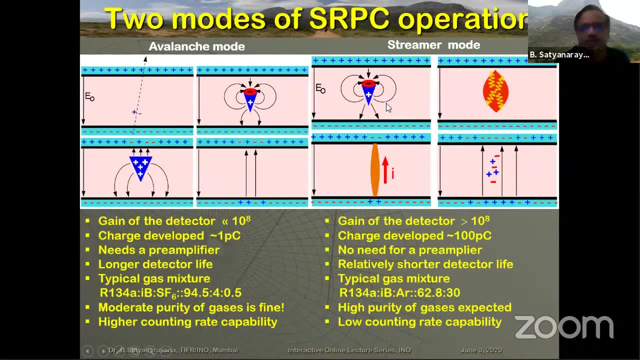 small so you may have to use amplifiers outside and this is the typical mixture and so on. Some people who do not like operate it at such a low gain. you can actually change the gas mixture and hydrogen and so on and you can actually start seeing a much bigger multiplication. 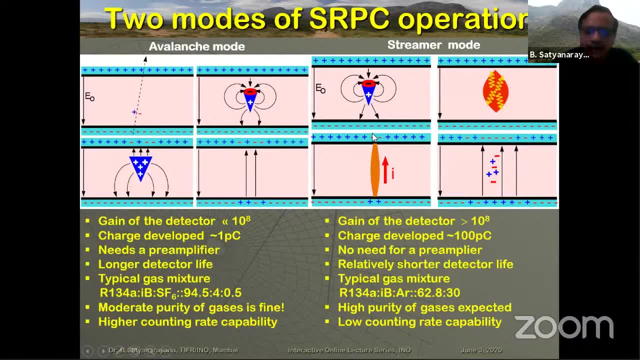 much bigger Avalanche. Avalanche is taking place and and so much so you actually see a big. you know it's almost like a, like a conducting electrodes here and producing a huge current between them. the signal that you see on induced on the electrodes will be almost about hundred times more than 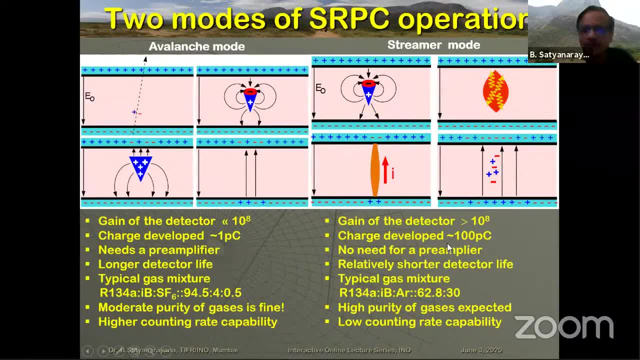 what you will actually see. So you will see much bigger pulses, maybe about 100 picoh coulomb instead of one picoh coulomb, and therefore you don't need any preamplified. but the price that you pay is that, if I have 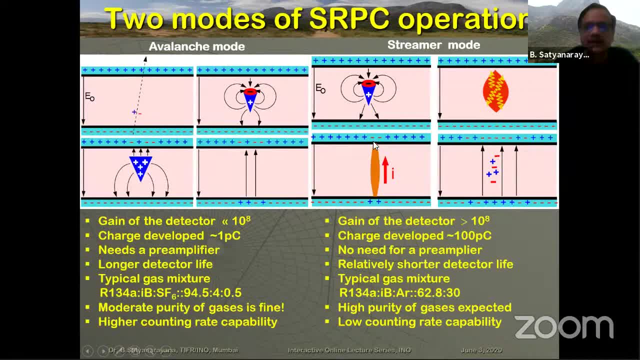 a very, very high charge The regime inside the gas chambers, it is possible that I actually start damaging the inner surfaces of the electrodes and then that is not good for a for a long, you know, detector life. and it is also sometimes problem for me to get what you call, let us say, the counting rate. 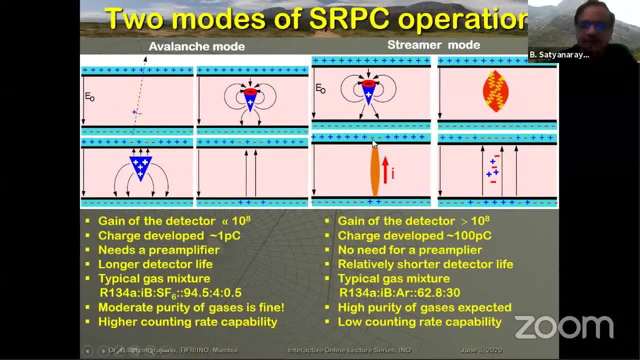 capability, because a much larger area gets dead here, because whatever you found here, the discharge, This has to be charged only by the power Supply, which is which you applied to produce field right. so that of course takes time. and then the larger the the current that I have replenished, the larger the time it takes. so 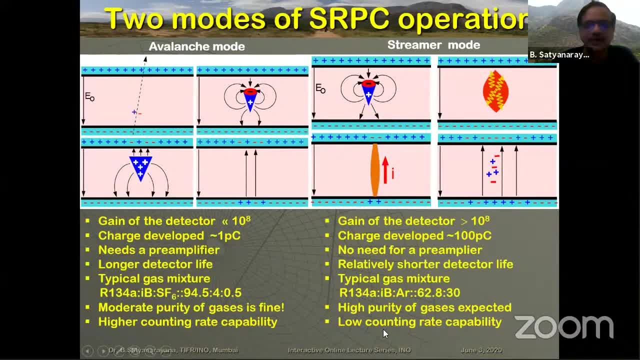 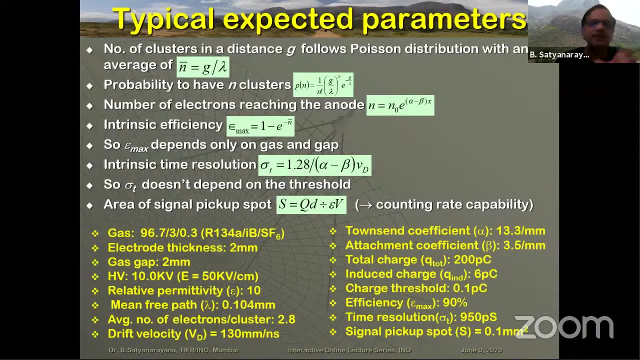 therefore I will also get a low counting rate capability, which means if you want to use such a detector in accelerator based experiments, then that will be a big design one. So just give you a kind of figures: what, what, what are the kind of typical figures you will. 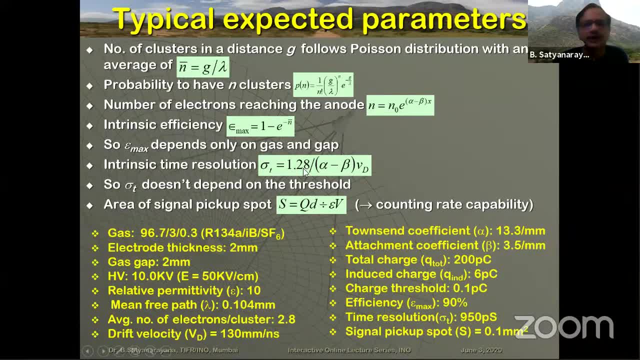 kind of get from such a detector. Okay, So here I have, starting with N, zero number of electrons, I will actually get, as I said, exponential alpha beta. this is Townsend effective, Townsend coefficient, and this is where I say: these are the number of, let us say, electrons that are reaching at the anode and the efficiency. 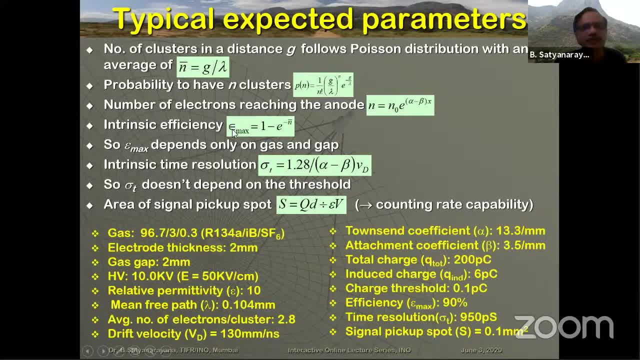 intrinsic efficiency is given here, which means the Emax is only depending on the gap G as well as, okay, the gas, the mixture that I use, because that is what decides this expression. So, and similarly, the intrinsic time resolution that I get from here is, again mostly depending. 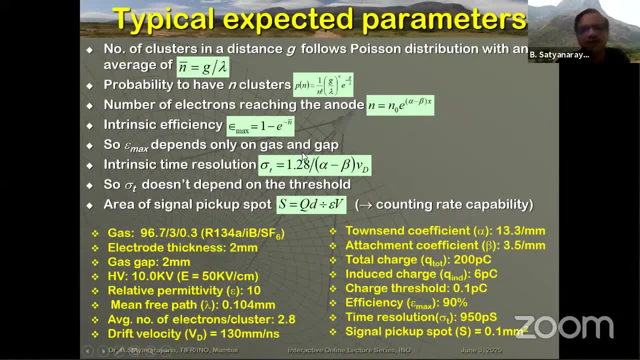 on the drift velocity as well as the Townsend coefficient. it does not depend so much on the threshold on which you know, I am kind of operating my D-Aque system. If you remember, I was kind of telling you that if you operate the detector in the streamer, 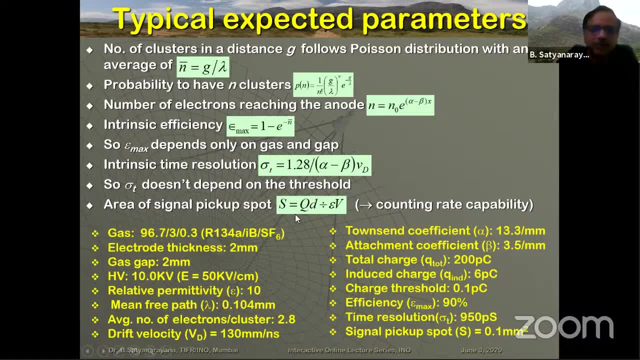 mode I have a much larger, you know, signal pick up spot, okay, which is, again, you can see, it is proportional to the, the Q, the total charge individually- Okay, Charge induced, and also, of course, the distance and so on. So which means that if I want to operate them in the avalanche mode, I get a much better. 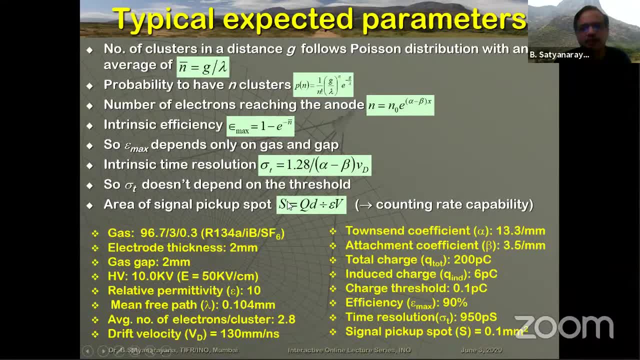 counting rate capability. but if I use in streamer I have a bigger streamers spot signal pick up spots which is of the order of about 0.1 millimeter square, which means my counting rate capability. that means I cannot really use it in a high rate environment. 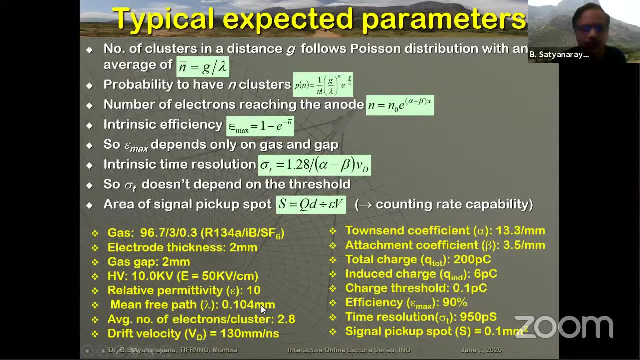 Okay, but typically you get for such kind of RPC detectors, with whatever parameters I have listed here, You get of the order of about a few picocoulomb charge. you get more than 90 percent efficiency, close to 1 nanosecond resolution. So these are good qualities of an RPC okay, and what we described so far is so called. 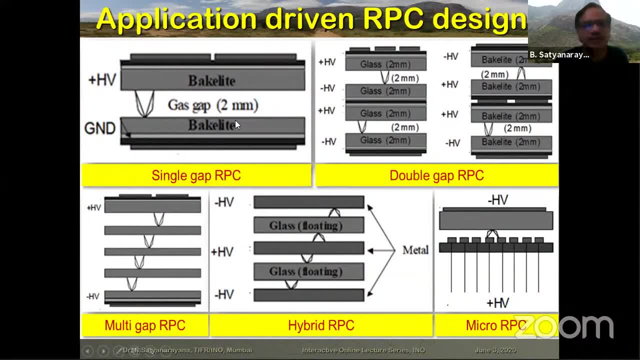 single gap, RPC. but because there is only one gap and these two are electrodes but you can stack two of them and you make so called double gap, you can improve the resolution. You could also put a common pickup between the two individual electrodes, So you can stack two of them and you make so called double gap, you can improve the resolution. 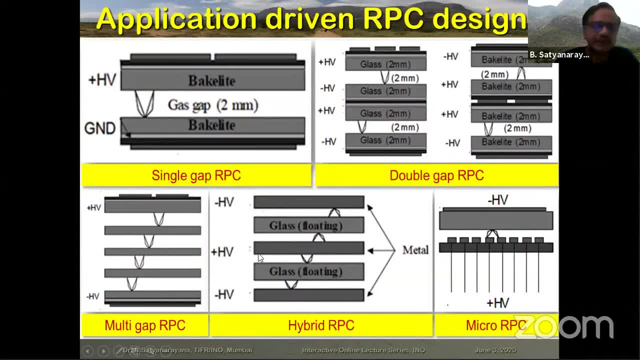 You could also put a common pickup between the two individual electrodes. Butagine, there is a single gap. okay, a variation of the same. you might remember Dr Mdabet thodi sometimes back about the so called multi-gap RPC's. so divide this gap into multiple. 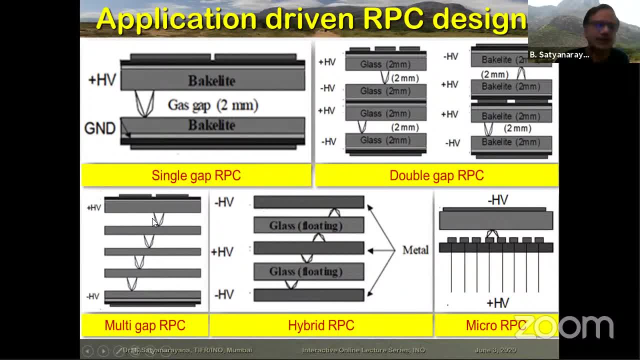 gaps and it, you know, improve on the timing, resolution and use for medical and other applications. you could also make that. you know the so called hybrid. instead of using the glass RPC's, you could also glass electrodes. you could also use other, you know metals, each one and then. you catch the gap RPC, So you can also short circuit RPCs if you are spectrometer or, I should say, anybody else. so, depending within making extrêmement in the case, if what you are doing in the say in the case like what is happening, talk about. I don't want to waste the, though it's actually. 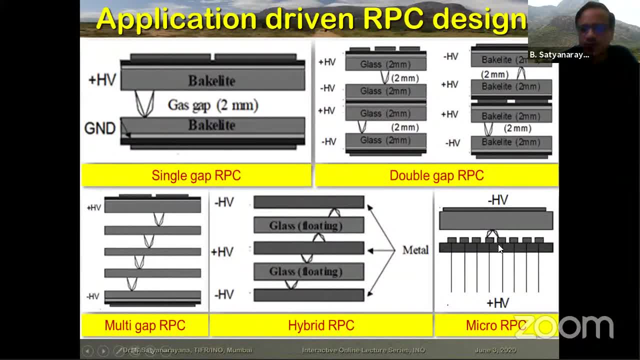 bet there is a you know a number. you can catch off the sensor. you can completely much of it怪 the so called he had. actually you could not such a series of iclaw is. and there is also so-called micro RPC, in which one of the electrodes you kind of, you know, make 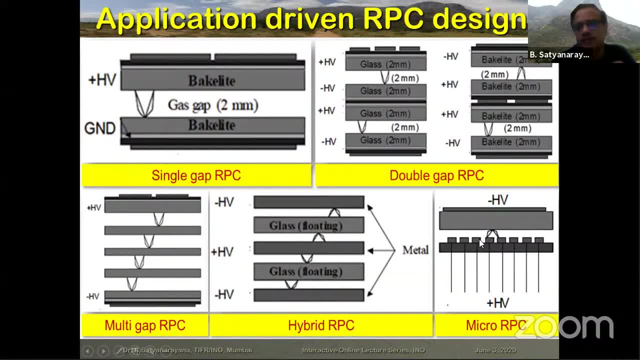 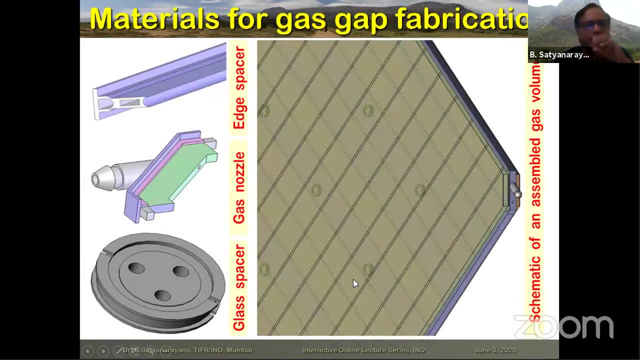 segmented electrode and then you can get you know much better resolution. maybe you can use for x-ray detectors and so on. this is called micro RPCs. These are some geometries. How do I make an RPC? Of course, for making RPCs you require many materials. Since I told you, you use two. 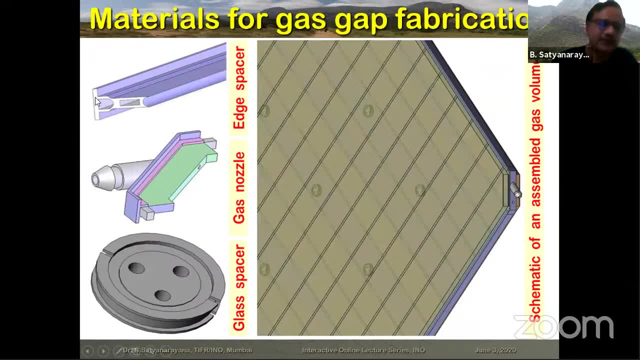 glass, glasses which are held parallel to each other. you need such kind of a spacer- like a photo frame if you like, you know which- on which you put one glass here, another glass at the bottom here, and this decides what is the thickness or the gap between them. You need to flow the gas. 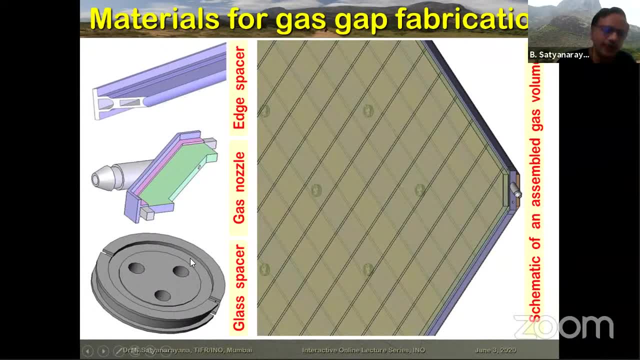 in and out. So these are what you call gas nozzles. You want to maintain the gap very uniformly, because when you apply voltage, the field is, of course, is depending on what is the gap that you are maintaining between the electrodes and if these, if the gap is not uniform, of course, you 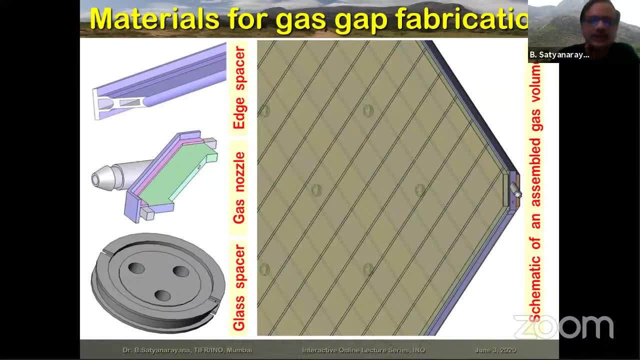 will get different fields at different positions and that means it's not uniform. The gain is not uniform across, right? So when you actually make this the cartoon of the actual RPC, you can see that these are the spacers that you put cover all four sides. These are the gas nozzles and these 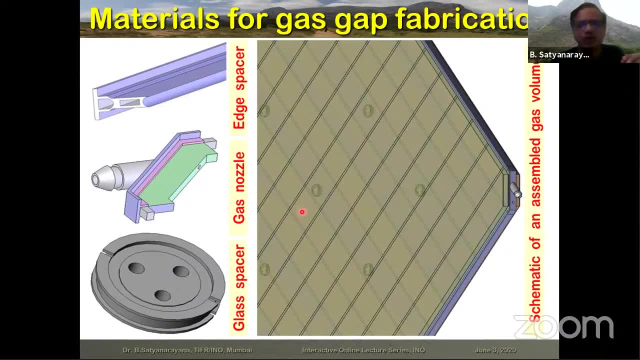 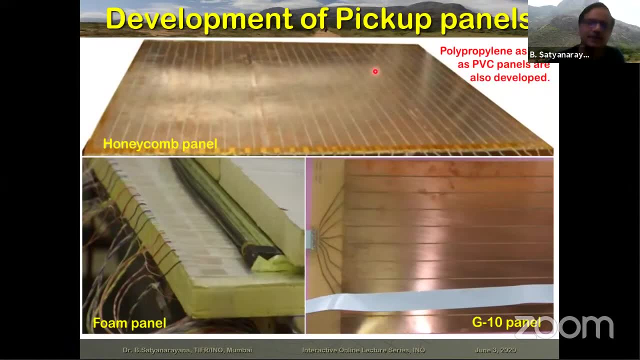 are the buttons which are inside between the two glasses, right, I'm only just showing you and to kind of say, that is how delimiting the space between them. Now, I mentioned sometime back that the detectors which are placed outside the so-called gap are the pickup panels which are 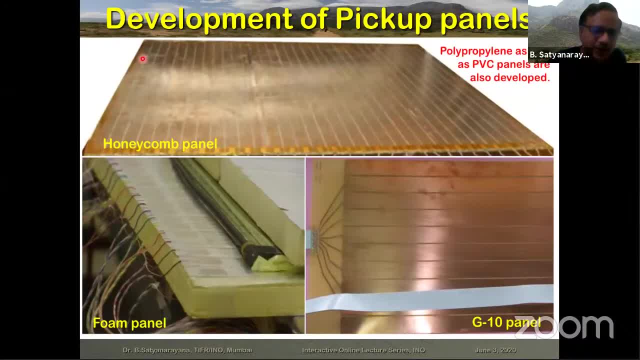 actually allowing you to get the signals on. you can actually see. each one of them is roughly about three centimeter long. So, as I mentioned, one such panel you put, let us say, on the top in this orientation. at the bottom of the gap you put one orthogonal to this, So so that you can you. 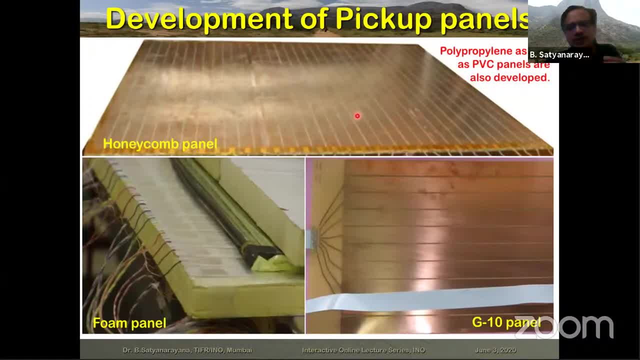 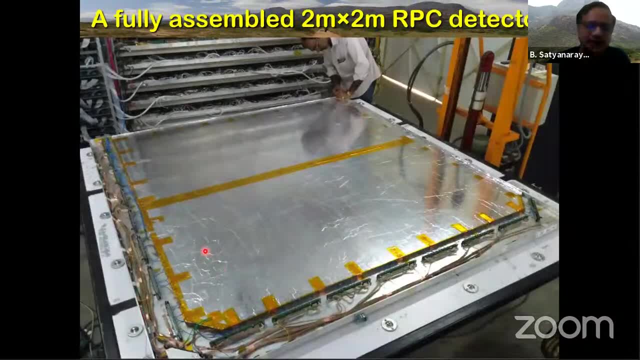 get a pixel of three centimeter by three centimeter. when a charge particle pass through, you will be able to kind of get the signal, such kind of resolution, right. Okay, Now, when you build like the way I shown, you take glasses. 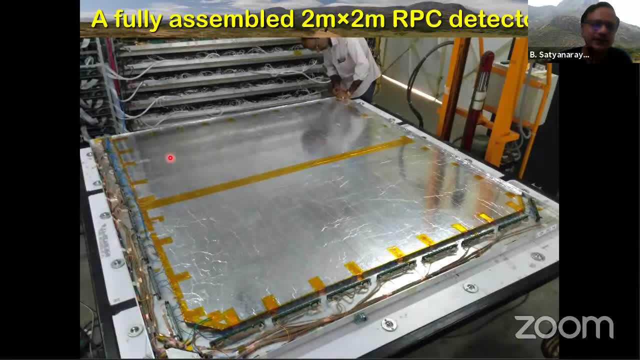 you put them together, you put the spacers around and you put the pickup panel on the top and, everything put together, you put the electronics that is required to pick up signals from both front. You can call this as X plane and you can say: this is the Y plane And so this is a. 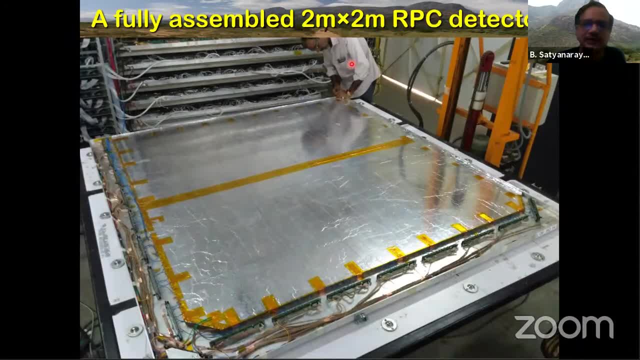 completely assembled so-called two meter by two meter RPC, And my colleague in Madurai is giving finishing touches before he is going to kind of push this into a stack here. Okay So, but it of course takes a lot of steps and a lot of care everywhere. Now, when you put on such an RPC. 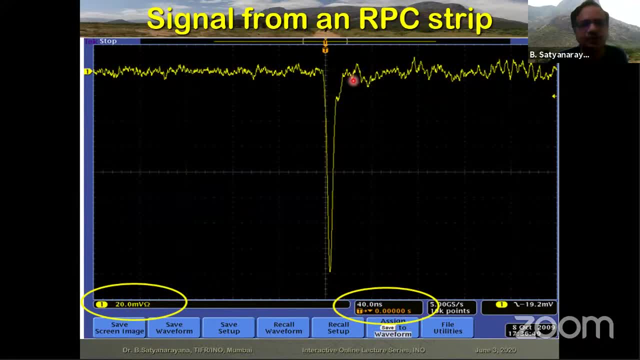 you will see a beautiful pulses like this. These are actually already amplified pulses, but you see, this is the kind of voltage that you are talking about. This is already amplified to close to about 60 or 70. And the scale is about 20 millivolts. So you have roughly about six. 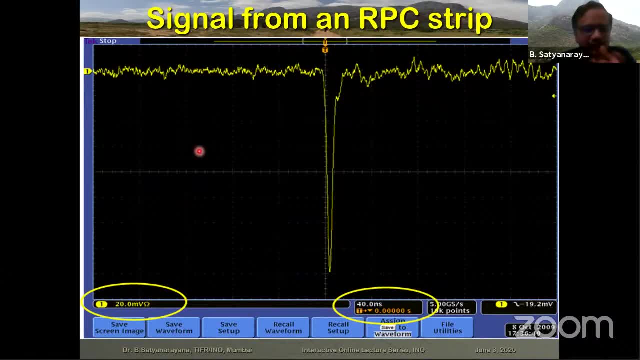 divisions about 100, 120 millivolts, And this is the kind of voltage that you are talking about. So you have roughly about 60 or 70 millivolts, but divided by 100 roughly, So it's about one. 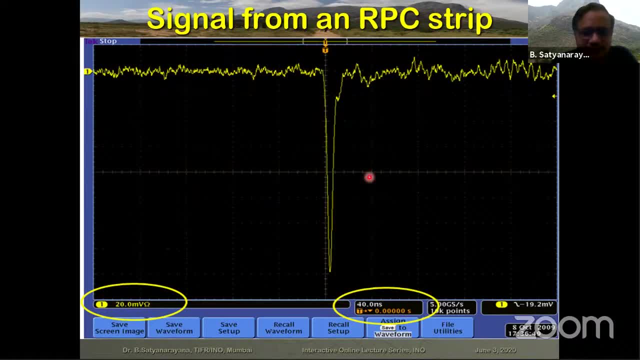 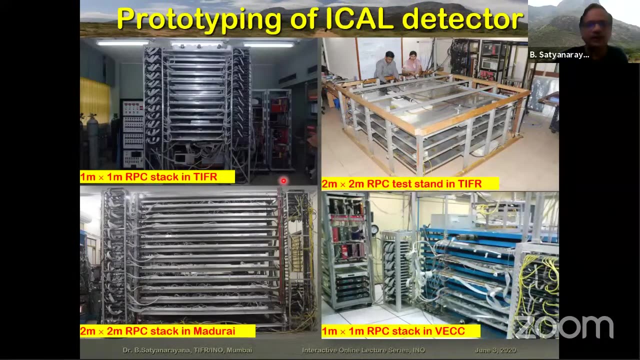 millivolt signal is what you're going to see. You should also see what is the time axis. Time axis is 40 nanoseconds, So each division is 40 nanoseconds. You can see how narrow this pulse is. Okay. So how do you know that you actually mastered the design and working you know? 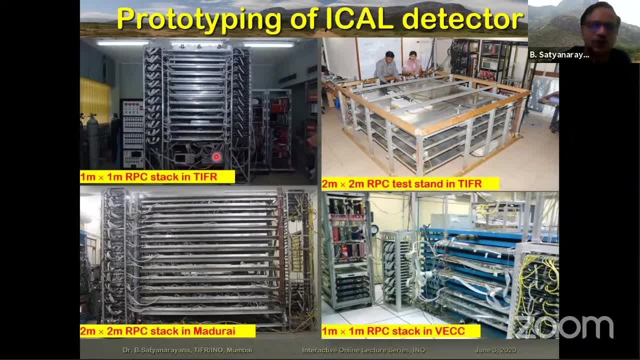 manufacturing of these RPCs. Then you go ahead and build what you call prototype stacks. here I'm showing you four of these, and this is one of the first stacks that was built in TIFR. This is still working. There are about 10, 12 landings here, and we made 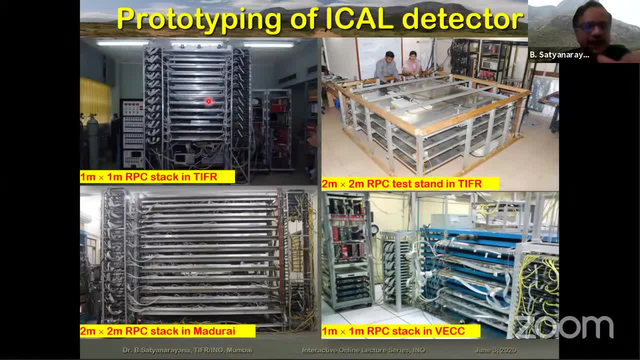 one meter by one meter area RPCs. They're actually stacked Here. you can see there are 12 slots. here There's electronics, here There's a gas system, electronics and so on, And of course you can happily track charge particles, which are all available to you, which are cosmic rameons. 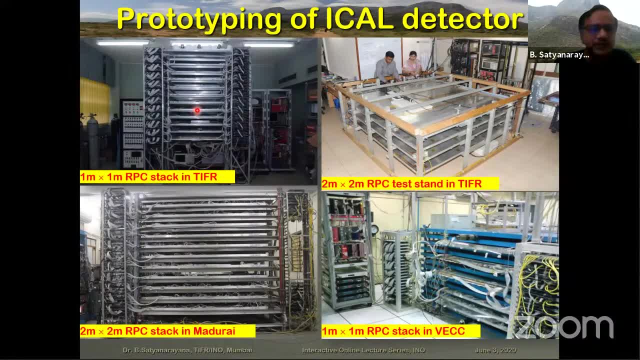 which you just go through straight through your detector And as they pass through each one of the landings, you're able to see the RPCs. So you can see the RPCs. You can see the RPCs. If it is efficient 100%, you're supposed to get a point there. You'll see that. Okay, This is. 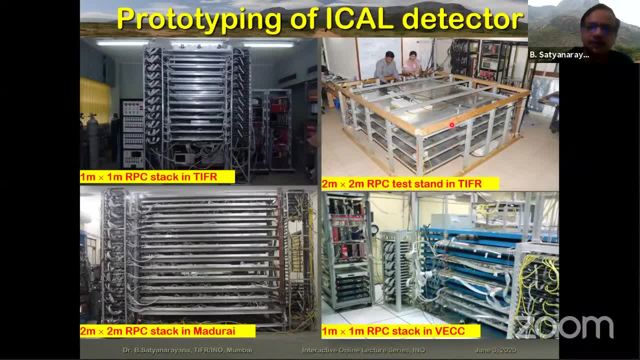 you can see, is the two meter by two meter much longer one which is also built in TIFR. Another one: one meter by one meter, RPC. This was at VCC sometime back Again. two meter by two meter in Madurai. What did it give you? Several years of running of all these prototypes gave. 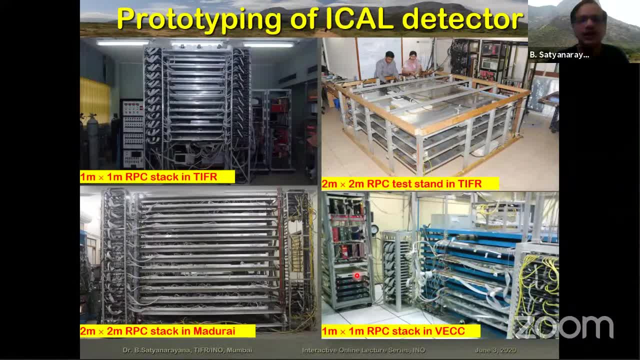 you confidence that you can actually not only understood how to design an RPC, but also their long-term stability. This is the most important. This is the number. ICAL experiment has to run for decades, Okay. So only when you know your confidence, such a detector works very efficiently as well as for long-term. then you will be able. 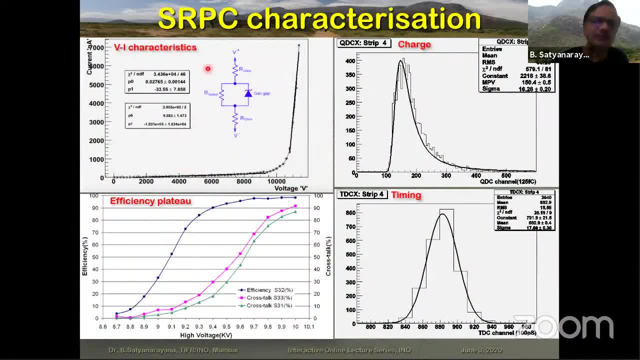 to install it for a neutrino detector. Of course you also have to. when you build a detector as a student or a faculty, you are supposed to also look at whether each one of these parameters that you build it's working. For example, there are what is called IV characteristics, just like a. 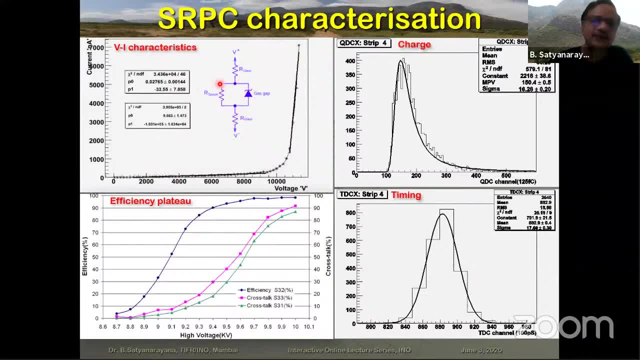 diode. For example, if you convert an RPC detector the way it's shown, there's a glass here, There's a bottom glass here, There is a gap here. And if I apply voltage here, and what? how should it behave? Okay, So until this, this particular Zener turns on. I want to see. 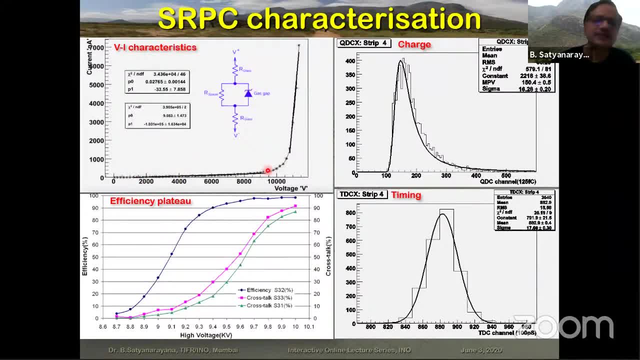 like a VI characteristic, like a ohmic resistance, the way it is actually showing for the spacer. And once the detector starts working, I want to see this as the current getting shooting up. So I want to, as soon as you build a detector, if you apply voltage and look for current. 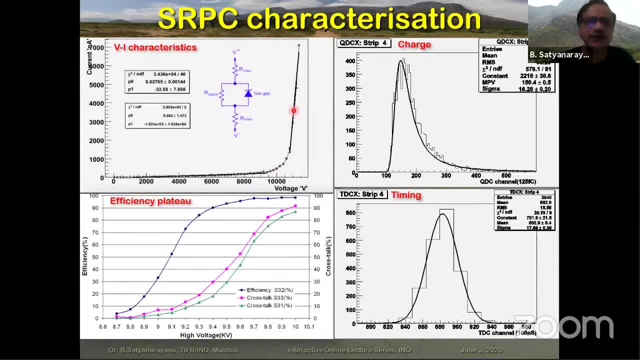 not like this. you are sure that you built a good detector. That's what every student in ICAL does. that After that you look for whether you are able to get enough charge out of the detector, which means the gain of the detector is quite fine. This is what is called. 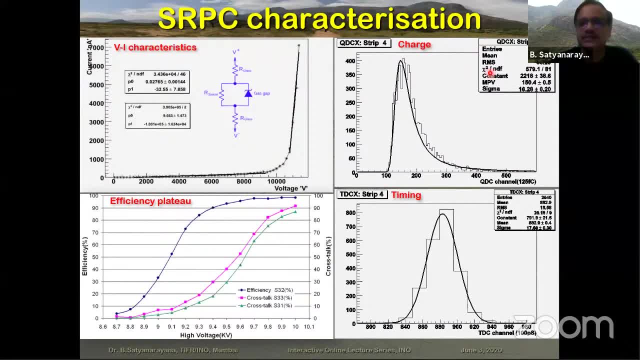 charge distribution for cosmic ray muons And you can actually see that you this is about one fourth of a picoculum and you've got about 200 count. So roughly about about 50, 60 picoculum is what you've got as a charge. What is also important when you build an RPC: 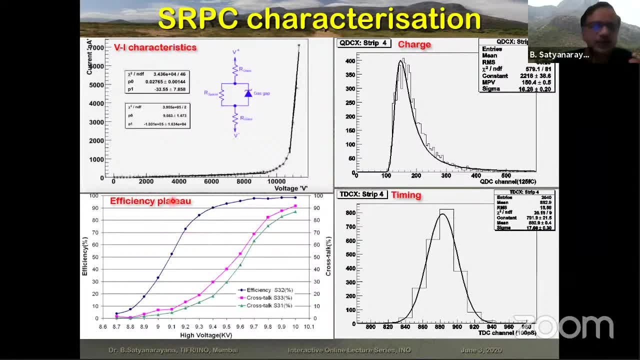 you want to see what is the operating voltage, at what voltage I should operate it. The way you do it is you actually operate this RPC as a function of high voltage that you applied, the field that you applied and start looking for cosmic ray muon efficiencies, right. So how many cosmic muons out? 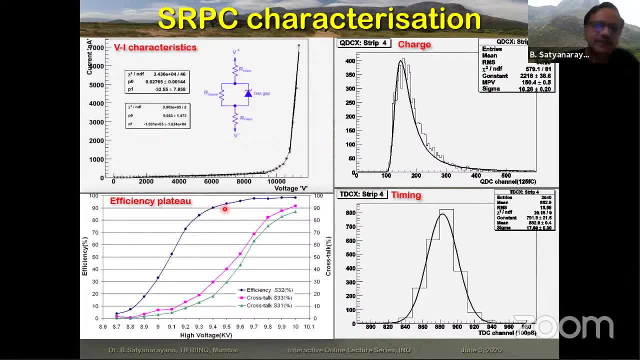 of what you actually gave through a cosmic telescope that the RPC gave you a signal. Now you can obviously see if you operate this at a low field region, obviously you're not very efficient. but once you reach a place where it becomes a kind of rather a water, 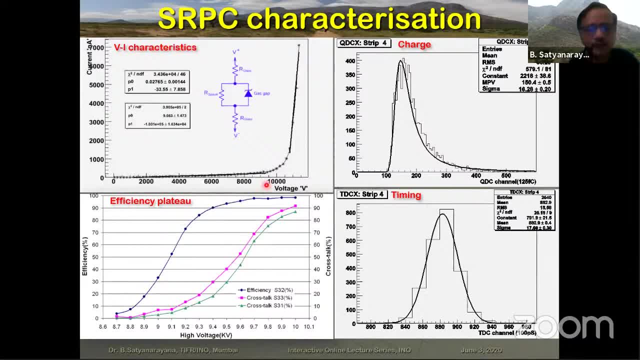 particle efficiency plateau and this is the place where you would like to kind of operate this detector when you push it inside the ICAL detector. And, as we said, the most important parameter for using RPC is also the timing. We should be able to kind of discriminate whether up-going or 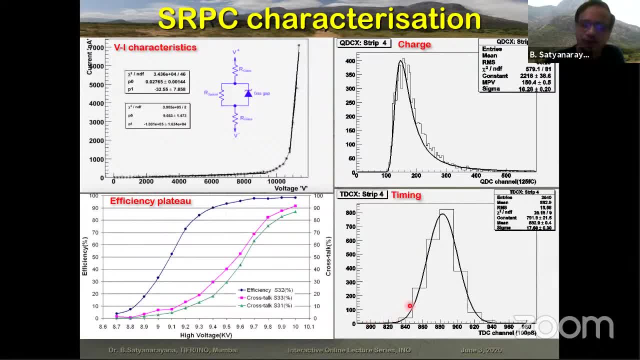 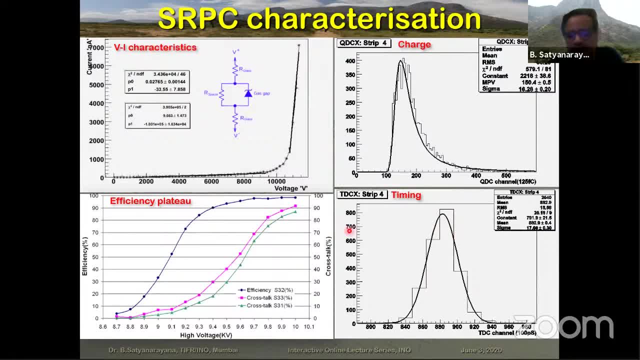 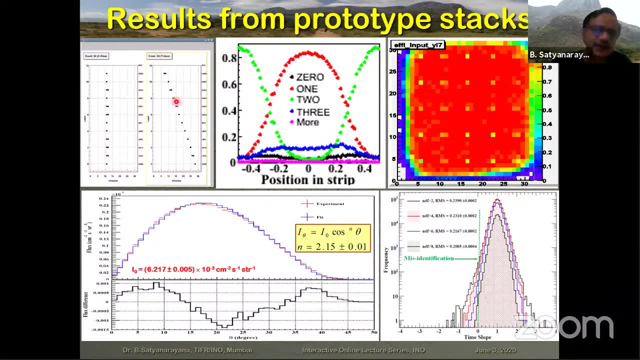 least of the order of one or two nanoseconds, right, Okay, So all these parameters, I need to do it. You need to go even more. You can actually see that such a detector that I've shown you the tracks are you can really see for a straight going cosmic muon and it's working beautifully. 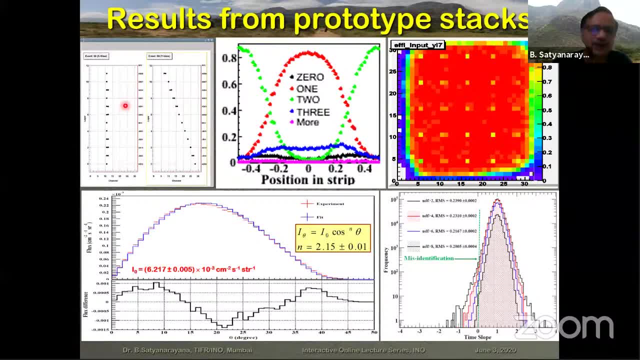 and it is actually giving you confidence that it is indeed working as a particle detector And depending on where this cosmic muon is passing through between you know, with reference to those strips that I told you, pickup strips of three centimeters I should be, if it is going, obviously, to the middle of, suppose the track is going in the 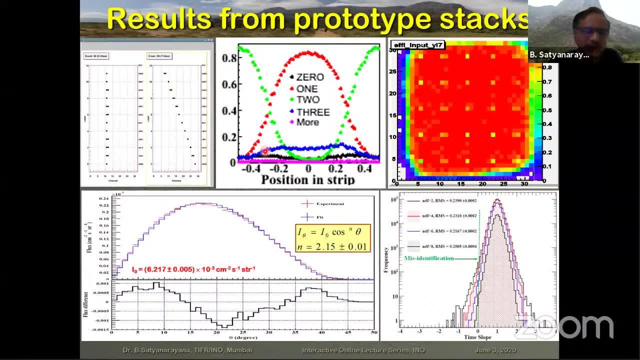 middle of a strip, I want to see that as only that strip firing, But if it goes slightly to the edge of the strips, the adjoining strip also might fire, and so on and so forth. I want to see such kind of distribution, what we sometimes call multiplicity distribution, whether it is one or 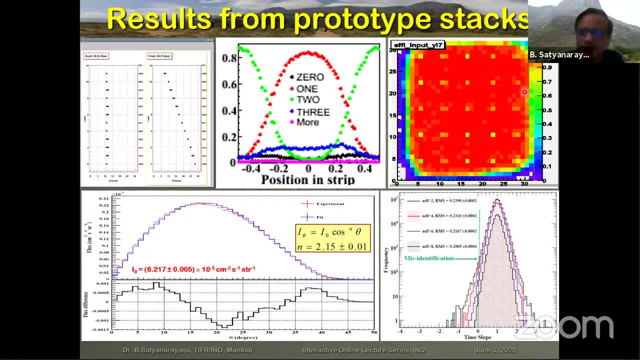 two or three and so on And, as I mentioned to you, this is the top view of an RPC which is mapped down due to cosmic muon, and you can really see the place that you have here which is showing. I mean, the red is, this is the scale, efficient and, of course, blue is least efficient. You can 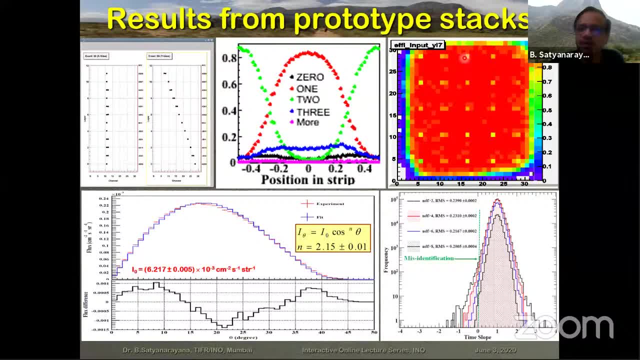 really see. these yellow dots are actually those spaces where you kept buttons for placing between them, for keeping the uniform distance. Otherwise you can see it is giving you overall when you take millions of cosmic ray particles through each of the RPCs and when you can track them. 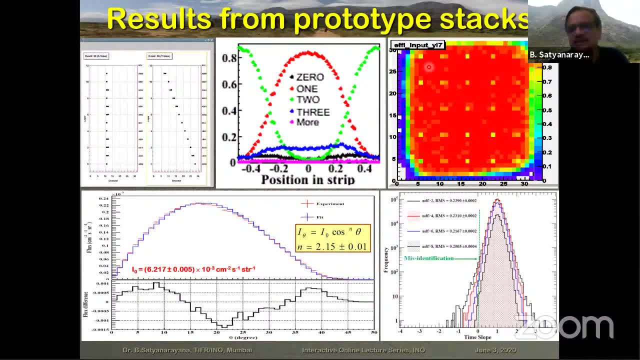 and put where it is coming from in the RPC And you say: this is the efficiency, uniform efficiency, uniformly efficient, for the entire one meter to the one meter. I can also go ahead and you know, try to kind of see what is the cosmic reflux even. 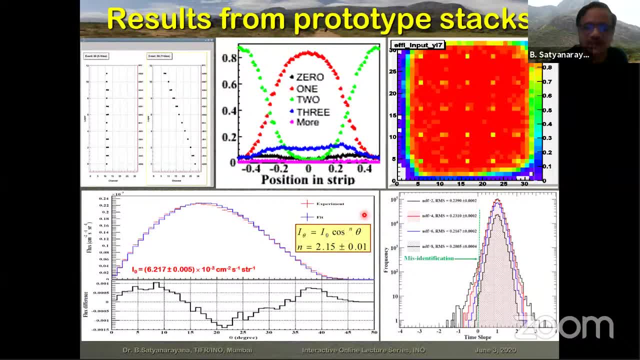 using such kind of tiny modules And you can see these numbers come quite close to what is actually given by standard. you know big detectors that were built and obtained Since the main idea is to get the- you know discrimination up or down going discrimination. 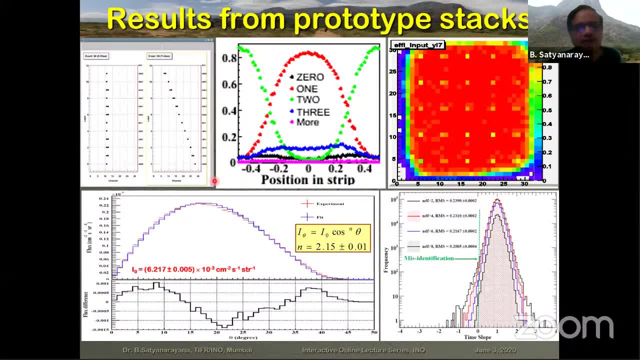 you can also see on the surface. of course, you'll always see cosmic remittance going from only top to bottom And you can actually see all this actually coming only on the right side and very little on the, you know, so-called misidentification. 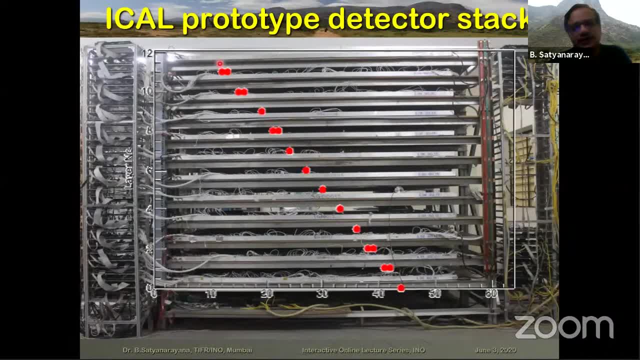 Okay. So this is what I'm kind of trying to show. If you have such a detector, each of the stack, each of these landing, you're going to see one point which is actually telling you the trajectory of the cosmic knot. 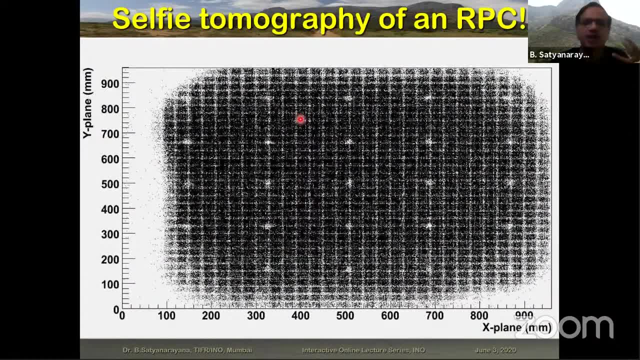 Now, if I, as I said, if I take each RPC for a long time And, you know, if I project such a particle trajectory, I can actually see something like what is called a tomography And you can clearly see these white spots. here are the ones with our dead regions, which 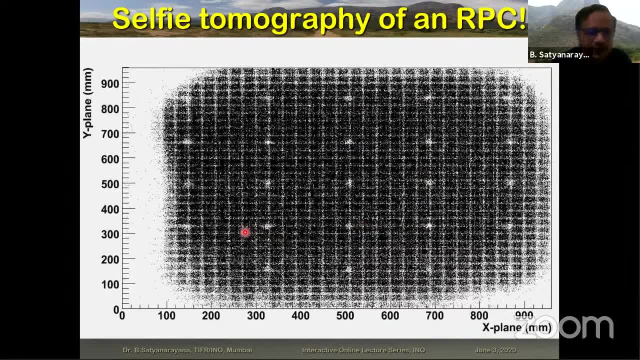 are caused by the spacers that we use. Otherwise you can see each of the strip, which is three centimeter is, and there is a gap of two millimeters in between. It's very nicely, kind of visible. Okay, Even such a tiny small detector, you can actually track cosmic muons, which are multiple. 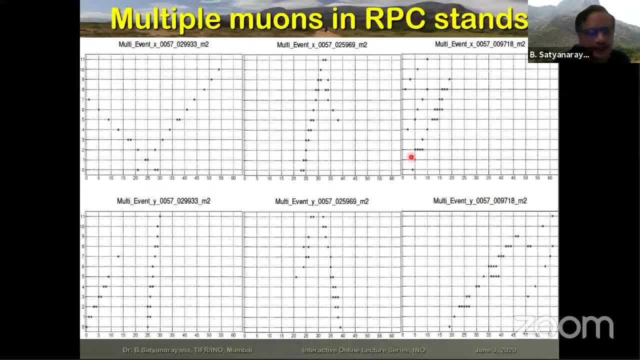 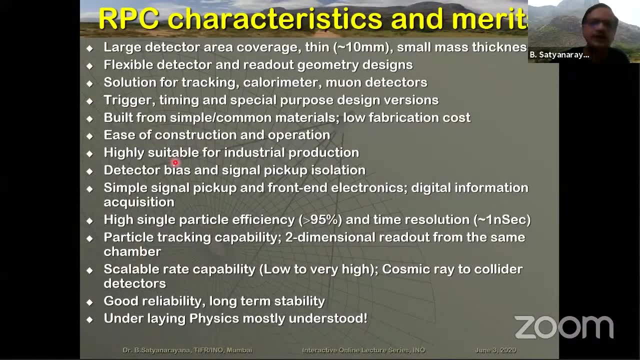 muons within within about two meter by two meter detector And you can see they're beautifully tracked. It's not just single muon tracks, but even double RPCs are very good in terms of- for you know, using it for detectors like ICAL, because, 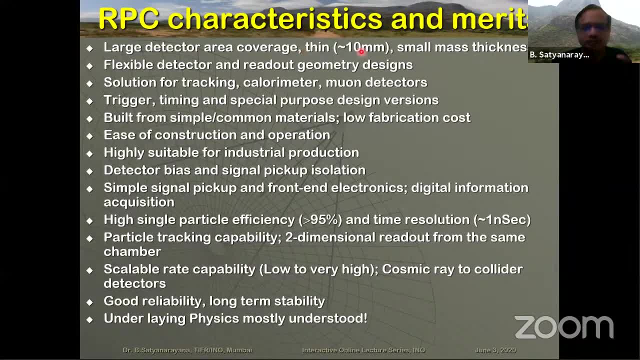 you need for very, very large area and very thin, because they are only about 10 millimeter thin And, of course, with material et cetera, it will go to about 25 or 26 millimeters And they're very flexible detector. 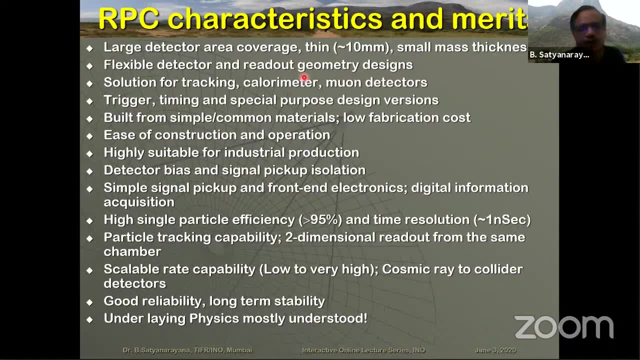 I can design the geometry the way I like. I can do X- Y, I can change the pitch of the pickup panels, and so on. I can use the same RPC for tracking calorimetry as well as muon detectors. I get excellent timing, as I told you. 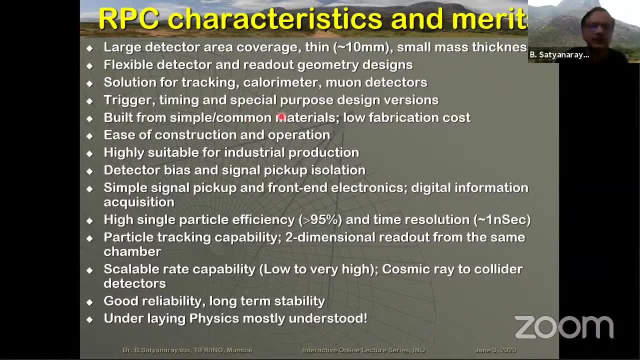 And they're all used from you know, simple, common materials. Remember, high energy physics detectors are very large in number, very high in in account, So you can't really build with the very expensive materials. It's very easy to build, as you saw, and very, very suitable. 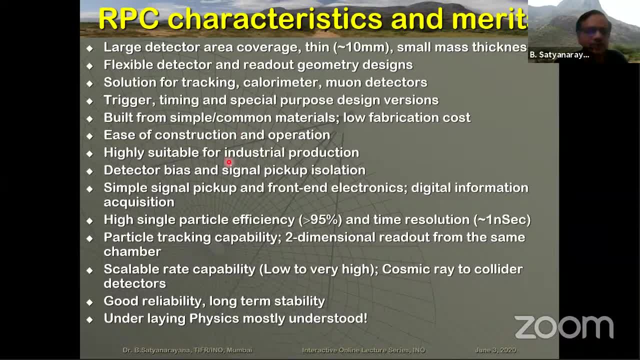 Ultimately, you don't build 30,000 RPCs in your lab, You have to build in our industry. And there are many other nice characteristics. I don't want to go for want of time, But RPCs are really nice. you know suitable detectors for such a detector. 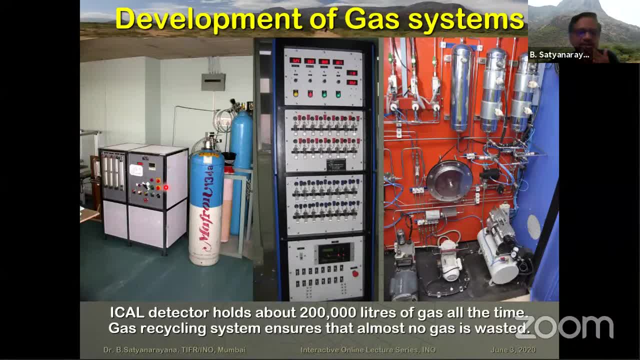 Of course, since RPCs are based on gas, gas is the detector media, So you also have to build So-called gas systems. gas systems are the units where it takes those mixtures of gas in cylinder and mix them in the proportion that you want and flow through the RPCs. 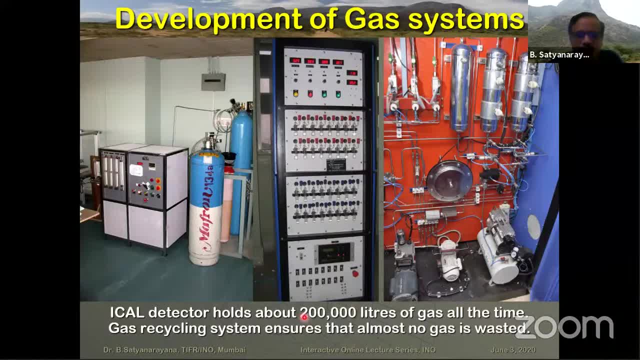 OK, but remember, if you build the big ICAL, it will require about 200,000 liters of gas And you can't really throw the gas into the atmosphere. And also, I mean even of course, it's not allowed. 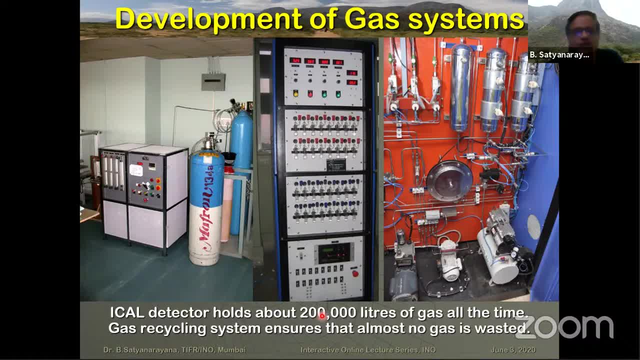 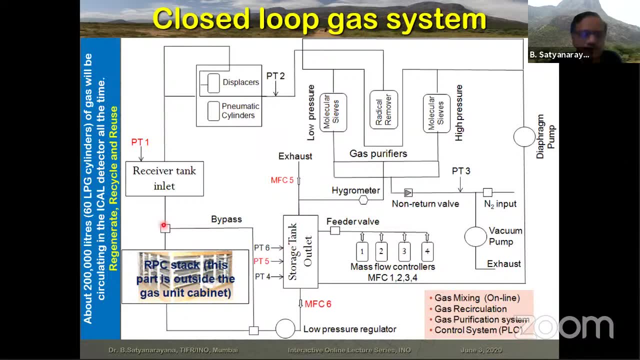 But even if you sell out, it is a waste of money, Right? So what you do is, when the gas is mixed together, when it is Flown through your detector, here what is shown? but after all, it is only used as a detection medium. 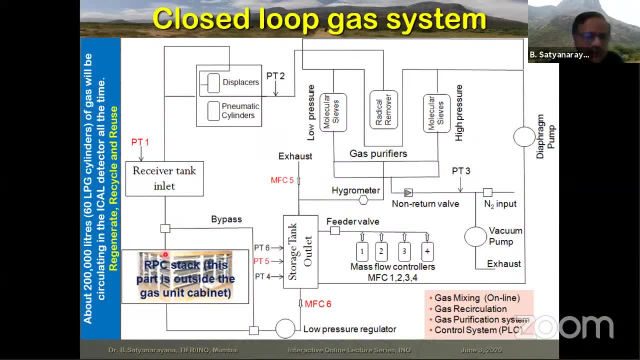 It is not something consumed in that sense. So take the gas out and take it out and, you know, maybe clean it a little bit, because it's due to a lot of leaks and going through the pipe etc. There may be some little contaminants, moisture, oxygen, water. purify it using molecular sheaves and other materials and push the gas back. 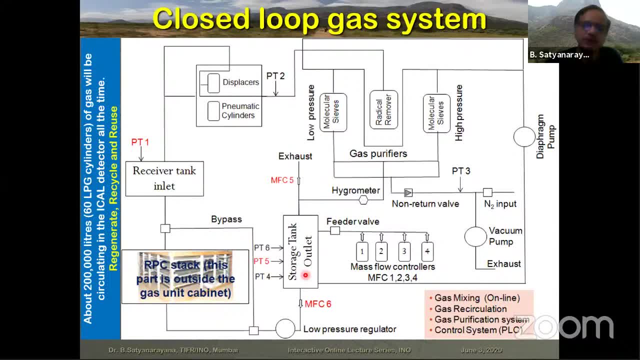 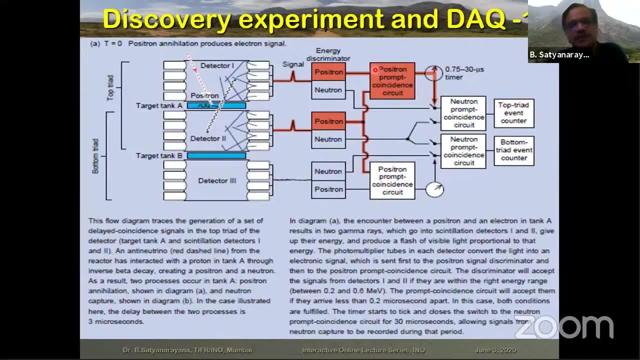 So you'll be using only a few small percent of new gas every time. Right, And this is what we call closed loop gas system, And that is what is kind of developed. OK, now I'll skip some of these plots. I mean slides because of water prime. 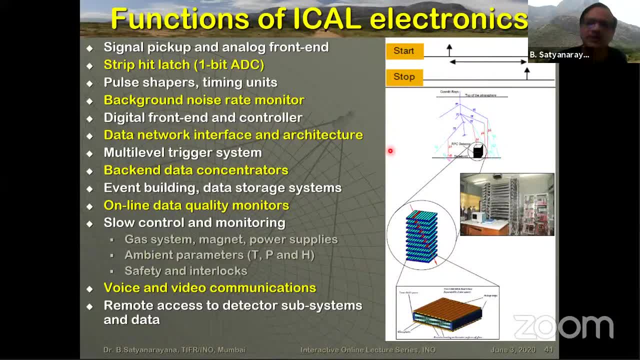 Now I want to go to and just tell you a few things about in terms of electronics. What is it required, Remember, when you have a stack like this? what you are actually asking is essentially want to see what is the path of these charged particles that are passing through. 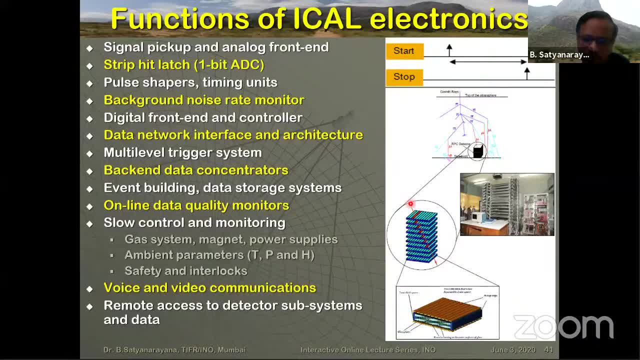 So suppose this is your ICAL detector. If I see either muons passing through or a neutrino coming in and then interacting and producing, let us say, muon charged particles, you want to track them. To track means as it is traveling. you want to see what are the coordinates of X coordinate, Y coordinate and Z coordinate. 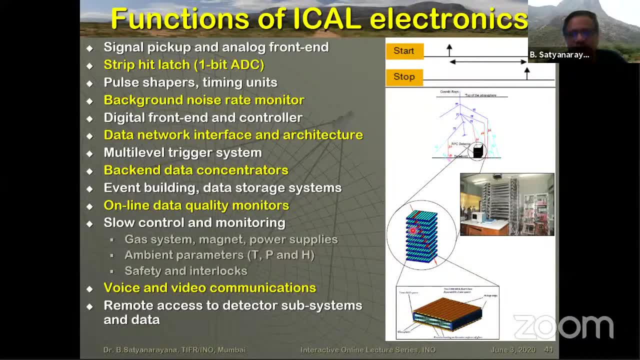 Of course, Z coordinate is given by the so-called layer. You remember we talked about 150 layers, right? But X and Y are given by the so-called pickup panels which are orthogonal to each other We talked about OK. so the information that I want is, at every level, which is one Z coordinates. I want to give you one X and Y, and another X and Y, another X and Y, and so on. 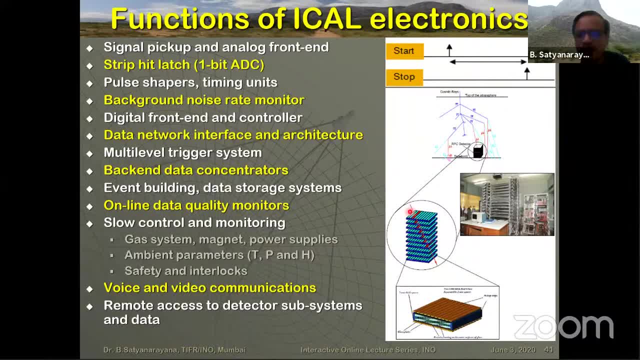 So that you will be able to kind of do a fit of this, depending on what you want to do, whether it is, you know, with magnetic field, without, and so on, so forth. So this is one piece of information. The other piece of information, as I said, as the particle is, let us say, passing through, you should be able to get a timestamp, which means, with reference to 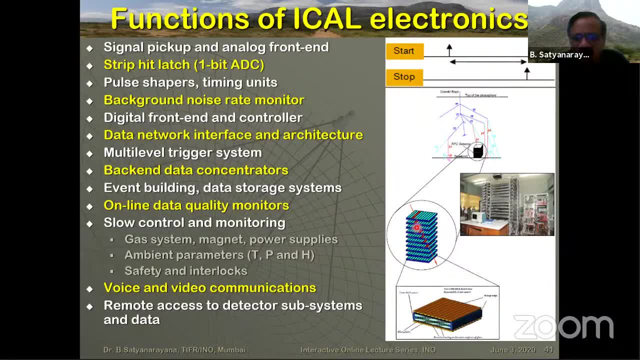 The passing of the particle, At what time the particle entered here, what time it entered here, what time it entered here, what time it entered here, then if it is in this increasing order of time, then I know this particle is going from top to bottom. 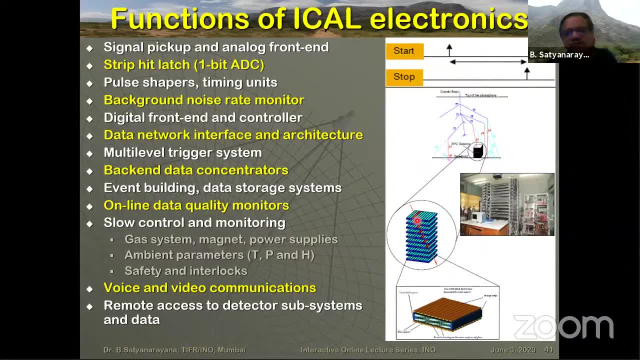 And if it is the other way, it will go from bottom to top. So I'll be able to kind of give you a, you know, directionality capability. So, which means there are two informations. One is, as I said, so-called latch. 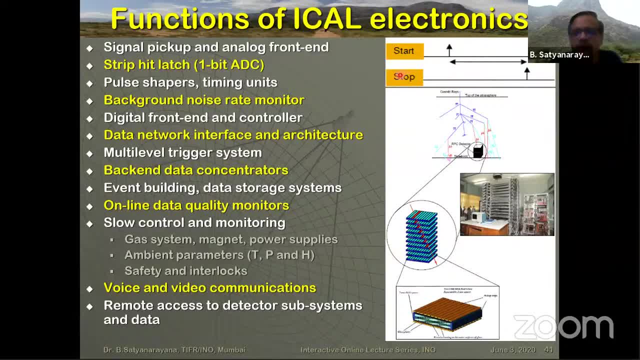 That means giving you X, Y coordinate. The other thing is compared to, You know, let us say, passage of the particle, how, what is the time that it took to hit this layer? you know, next layer, and next layer, and next layer and so on. 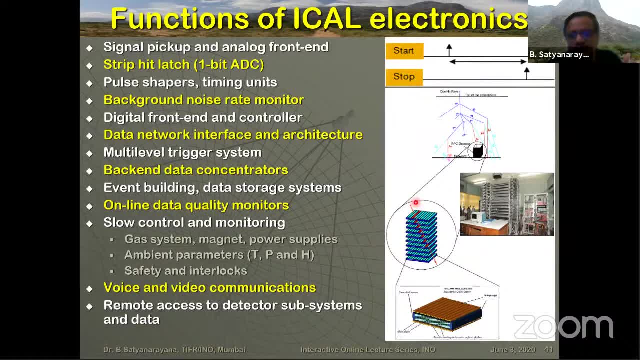 And if I see a cosmic beyond particle, you know if it is going all the way down and if it's going through all 150 layers, you will have 150 such informations. Okay, So that is the main information that you want to get it. 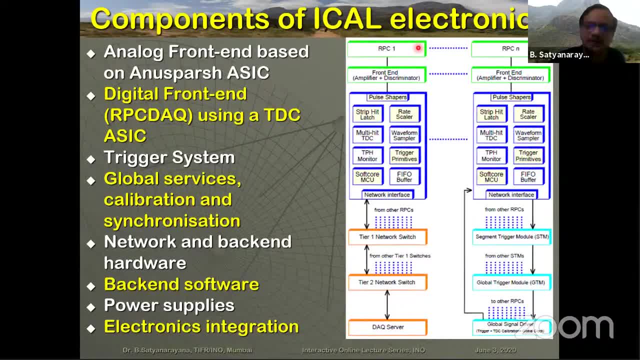 So of course we get down and say that this is my PCI. the signals being may not be very big, I would like to Kind of, Kind of have an amplifier here, and then I want to signal process the. the signals that are coming out of this RPC need to be kind of you. remember we said you need X- Y coordinates. 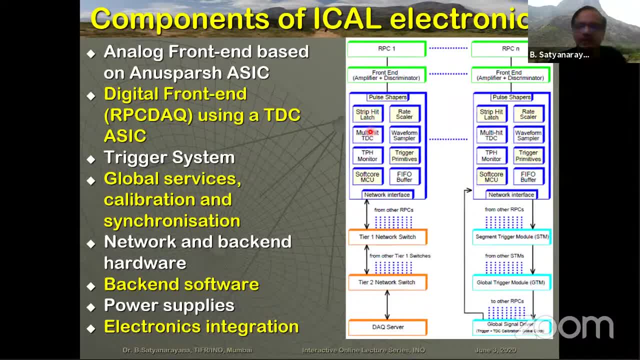 You need to kind of measure the time difference between the particle passing through and hitting the detector and so many other you know monitoring parameters. So you kind of block and you know break down the electronics requirement into into this, but remember you also have to generate what is called a trigger. 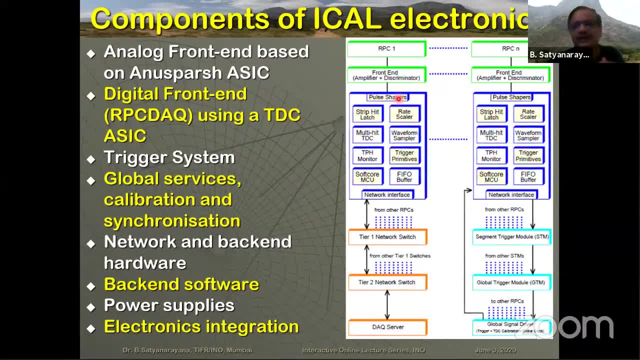 Trigger Is a system which is telling you when to record data. Otherwise, you know, there there may be a lot of other spurious events. You don't want to trigger them and this is the most important system. So you need to also build an electronic system which is going to decide, based on the track of the particle or the topology of the the hits, whether this is an interesting event or not. interesting, right. 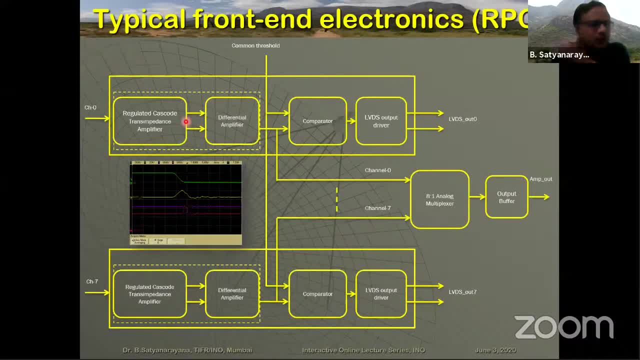 This is the electronic, So the first thing first. so there'll be students who will sit down and say that, okay, this is the requirements that I need, This is the amplification I need, This is what is required for my detector. 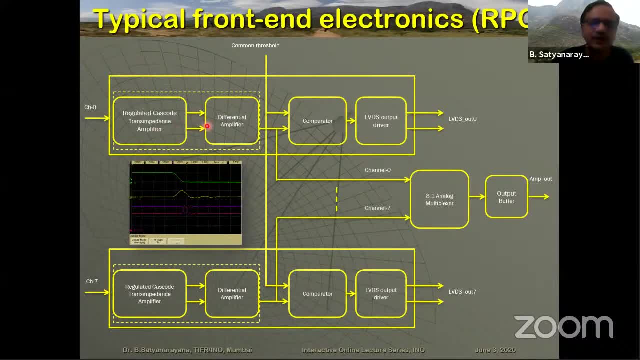 And then they make a block level diagram and say I need an amplifier here, I need a comparator, because I want to convert an analog signal into digital signal and so on and so forth, the multiplexer and so on. So this is the basic drawing that is required. 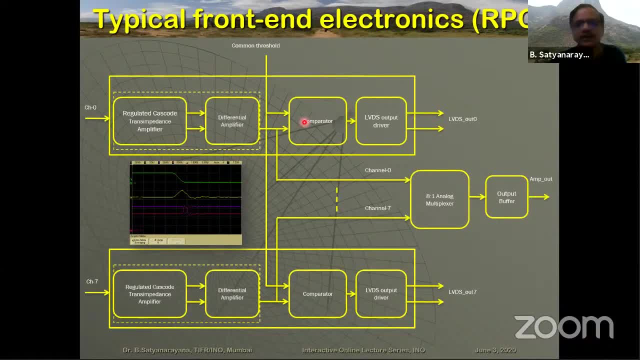 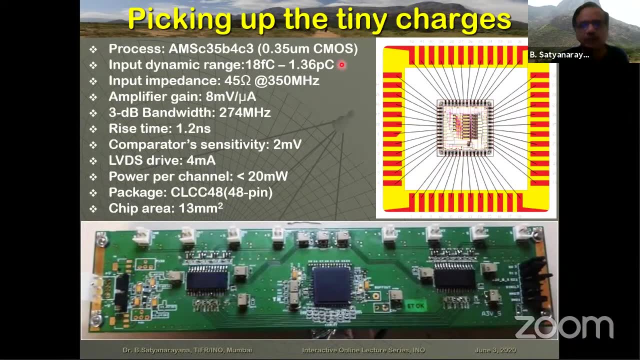 Very simple textbook is drawing. but what is important is, unfortunately you can't go to local market and buy an amplifier for you, So you have to design because the signals are very small, They're very fast. Such kind of very, very high bandwidth ICs or optiamps or something are not available in the market. 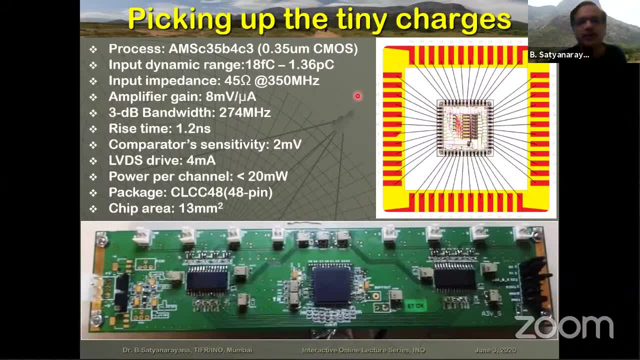 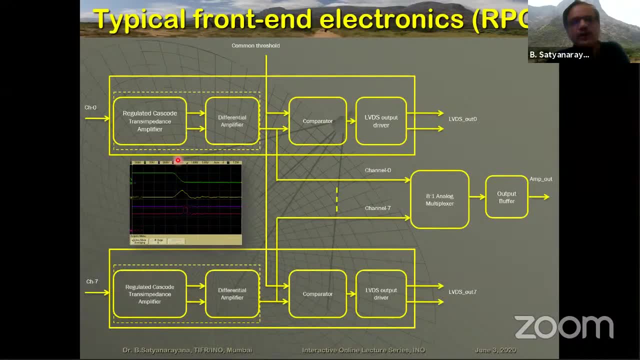 So some of our students go and sit and design what they call application specific integrated IC, starting from very basic electronic circuitry. they actually go and design this chip by themselves, Okay, And then we go to a foundry. Unfortunately, we don't have good foundries in the country. 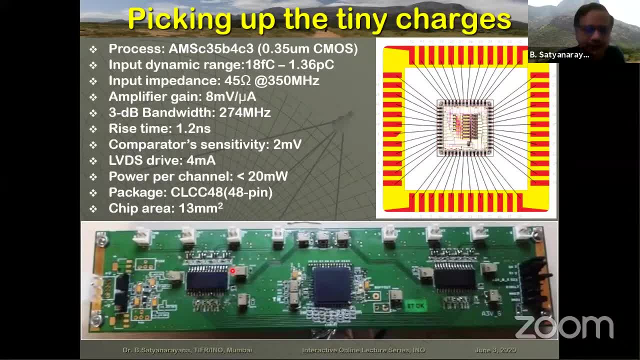 We go out somewhere, and maybe European foundries or somewhere, and get these chips fabricated. So these chips that you see here, Here, here, these are not bought in local market, but actually built, designed by the collaboration and, of course, manufactured in a IC foundry. 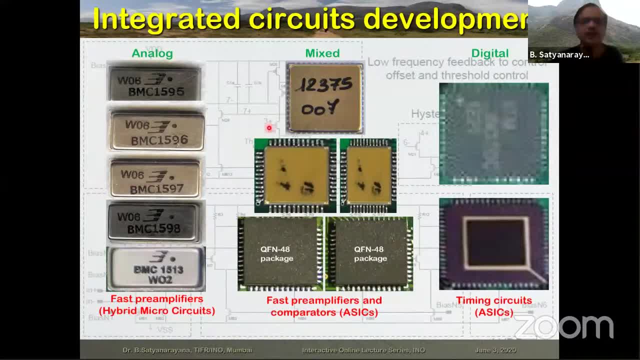 Now you can really see there are a large number of such chips which are produced by INO within the collaboration itself. Okay, Initially we started with some what you call hybrid chips. Now they're called ASIC chips, both for analog, for amplifiers, etc. 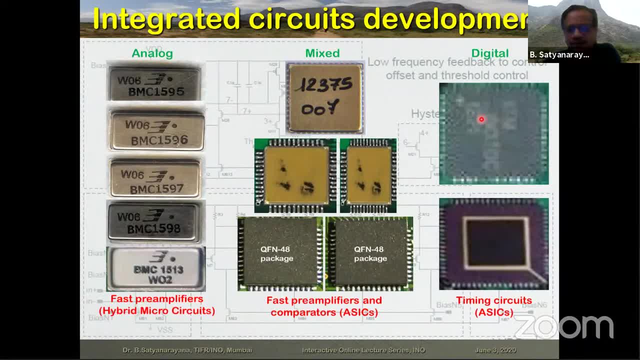 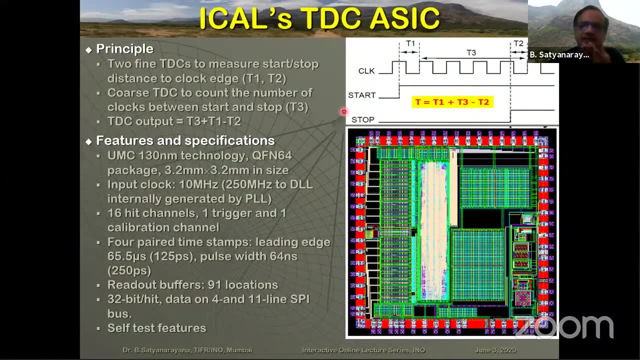 And you remember I was telling you the ones that measure the very tiny difference at so-called time-to-displacement. This is again designed and developed in inside the INO collaboration. If you want to measure a particle passing through with reference to where it hit each one of those landings, if this is a start signal which is produced by so-called trigger system, what I'm actually asking you to measure? difference between these two. 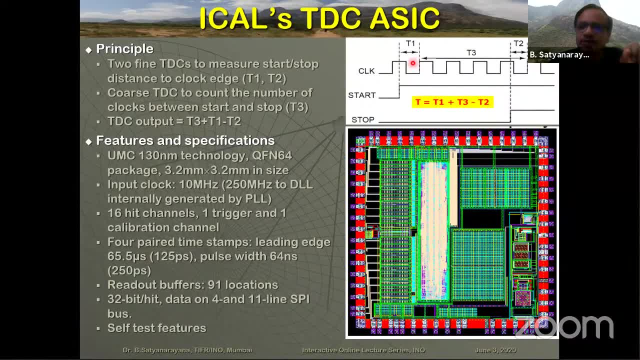 Right. So if I provide a clock to you, I'm actually asking you to measure how many full clocks it is, And then obviously you can measure the time. So basically the start can come anywhere and the stop can come anywhere. So I should be able to measure this T1 here. 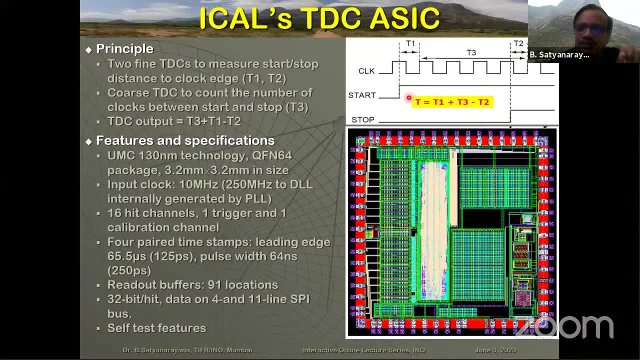 I should be able to measure this T2 here and say the time difference between them is T1, which is total, this pulse here and T3 and then minus T2.. Right, Because you don't want to count that extra one. It looks very classical and very simple. 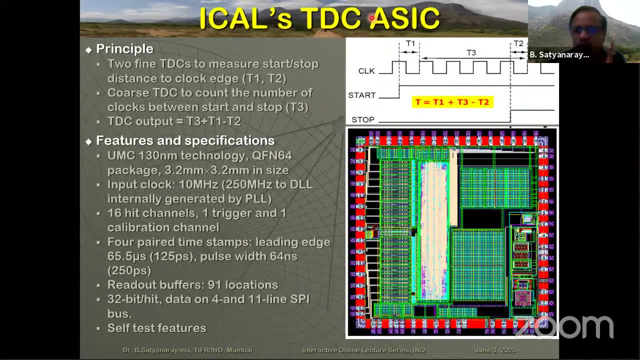 There are many configurations and many ways people can build so-called digital application-specific integrated circuits. One that you see is here, But just remember That what you are actually asking is to distinguish something like 125 picoseconds resolution. So you are measuring this difference at a level of one-fourth of, let us say, a nanosecond, which is very important because that is what gives you a capability to be able to kind of give you a directionality of this signal. 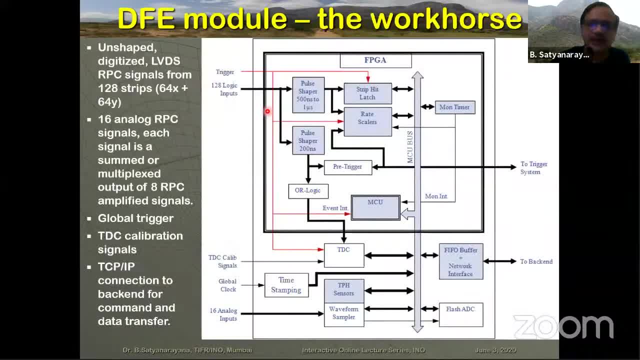 So this is again produced in the collaboration. Now there is another thing before I go quickly out of this. electronics is we also use, Heavily use, what you call field programmable gate arrays. They are like circuits which come to you when you buy it. 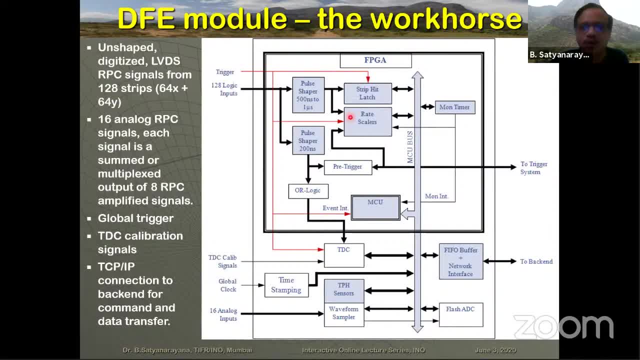 There is no circuit inside. You can decide what circuit you want to put that inside, And then you know: download, just like the way you download a program from somewhere, And that field programmable gate array becomes a digital circuit all by itself. 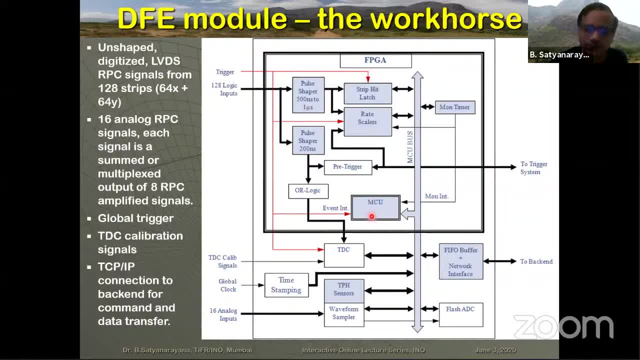 And then you can start using. You can put a lot of complexity inside. You can even put microprocessors inside, microcontrollers inside and so on and so forth. Okay, So such kind of a big, big, you know modern field programmable gate arrays onto which, where we put all the digital logic inside the digital converter here. 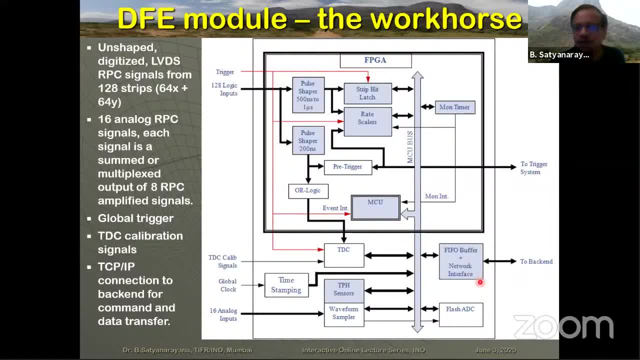 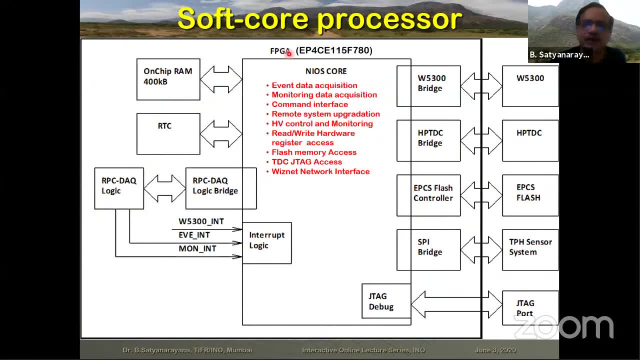 And then the data that is digitized is actually coming through you know a network which I will show you in the next slide. Okay, And everything inside that field, programmable gate array, can be programmed So somebody can actually write to do what data acquisition software that they want to do. 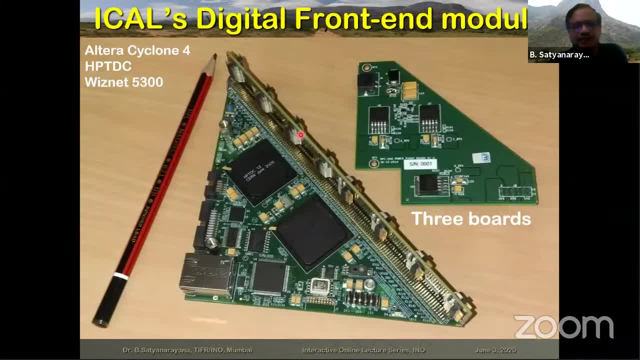 And when you build The entire system it looks like this: It is a very funny looking triangle, like board, because you will see soon why we need to take very small space for the electronics: because you want to get good area for the detector active volume, right. 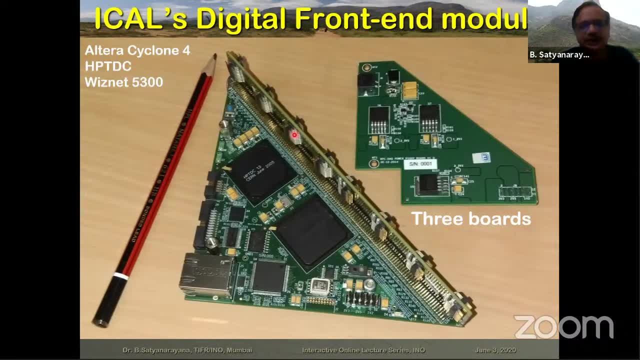 So you see this vertical wall in which the entire signals from one RPC are getting into. You know this is the time to digital converter, where you measure the tiny time differences, And this is the field programmable gate array into which you put All the electronics that you require that digitized data will come through this chip and come through this connector. 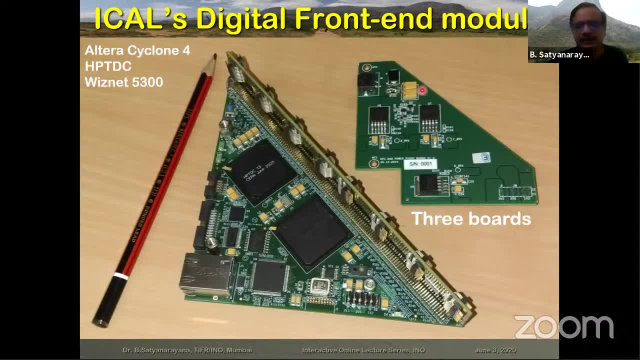 This connector, you will be familiar. it is the same as your internet connector And this board is supplying power which will go on the top of this. Just compare this with your pencil size. It will tell you. this is just about 10 centimeter by 10 centimeter. that to a triangle right. 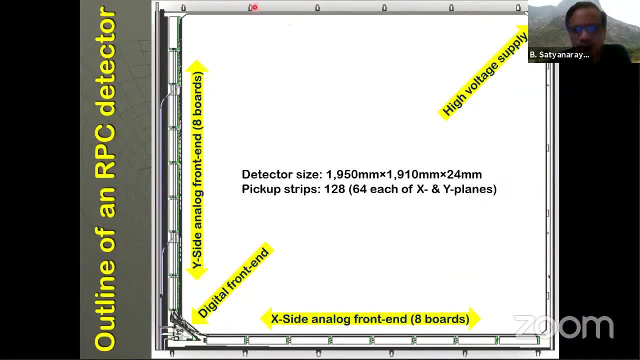 Why such a small thing? Now you compare. This is your RPC, which is 2 meter by 2 meter. In that area you're only occupying this little space for the triangle- Okay, Okay, Okay. And this little space for power supply, which produces field, which produces, yeah, which you want to produce, uniform field, you apply a voltage here. 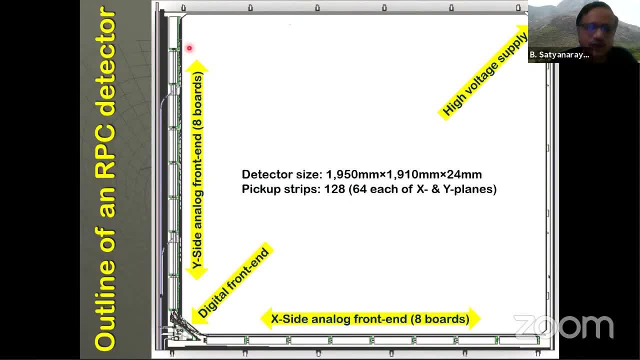 Rest of the area is all you want to keep it for the active detector volume. So this white area, everything is active. This is the top view of an RPC. Of course you can see the amplifiers that we talked about, for the Y side, marked here, and for the X side, these rectangles are here. 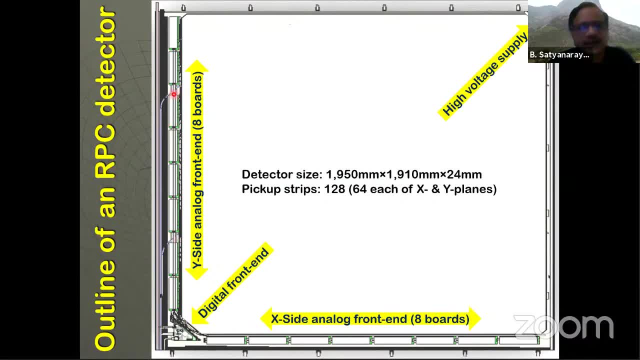 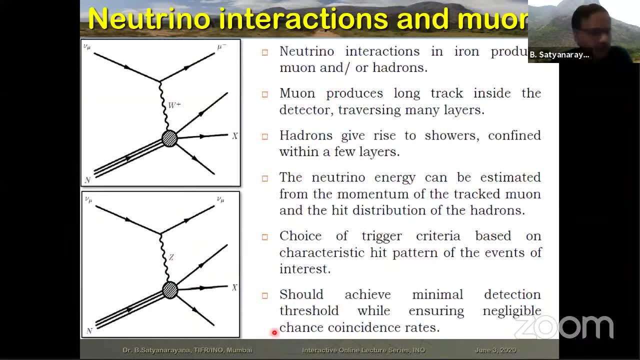 So that are the only area which is so-called dead area. The rest of everything inside a big RPC is maximized. that, Okay, I want to quickly go to an important system I hope I have. Can I take about 10 minutes? 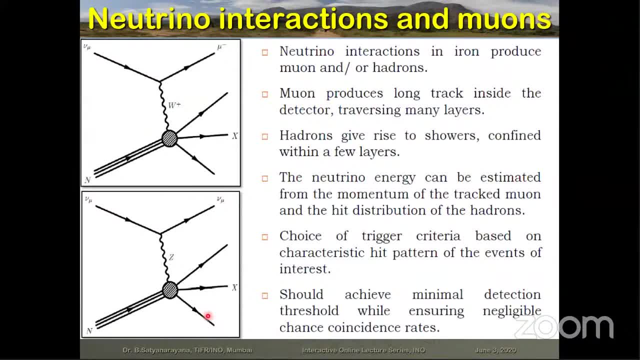 Deepak, All right, Yes, Yes, Okay, So of course you want to. you want to detect neutrino interactions that are taking place, right, So they depending on whether you know they are charged current events or the neutral current events. 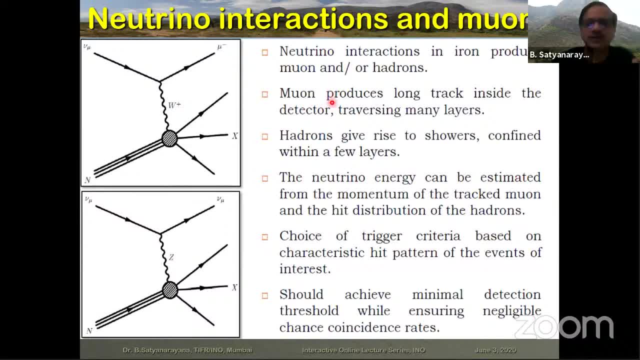 you typically produce, For example. so let us have beyonds, which are produced long tracks inside the detectors and they go through many, many layers of RPCs. So therefore, it is probably one way of detecting them. The other thing is those when, when, when you want to look for Hedrons, they don't go through long tracks because you are using very thick material. 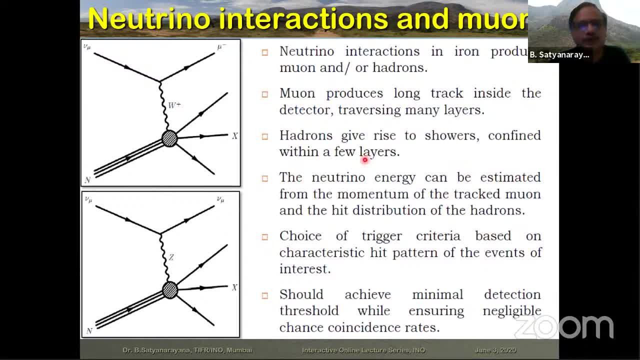 So they might actually shower out and confine to only a few layers. So when I want to say that I am actually looking at both for charged particles- we all like particles as well As Hedrons- I should have a strategy where I should be able to track them or I should be able to recognize them inside my detector volume, right? 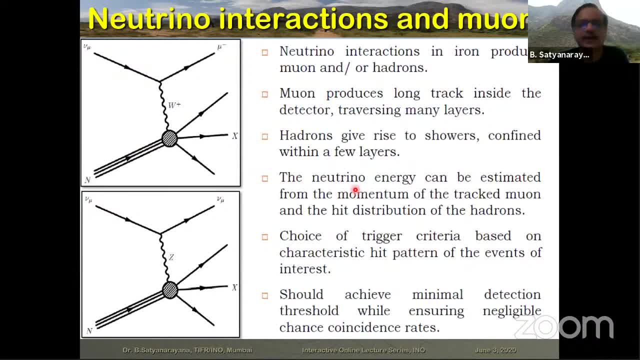 For the, when you want to estimate the neutrino energy, okay, for this, beyond of course, it is easy to do it because you have magnetized detector and then you have X, Y coordinates for each one of them, You reconstruct and get the tracks. okay, from the track, from the magnetic field radius of curvature, you can get what is the energy, whereas for the for the Hedrons, you actually have to see how the Hedrons are going to interact with each other. 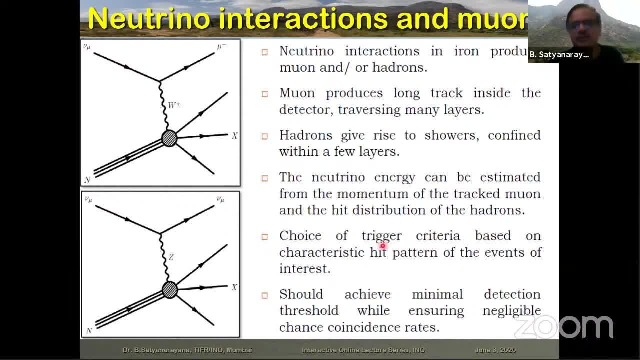 Okay, Okay, How many such pixels got fired, and from there you may be able to kind of get what is the Hedron energy. So it is indirectly kind of obtained. So the choice of so-called trigger criteria, based on whether I'm talking about the charge current events or your neutral current events or muon-like events, 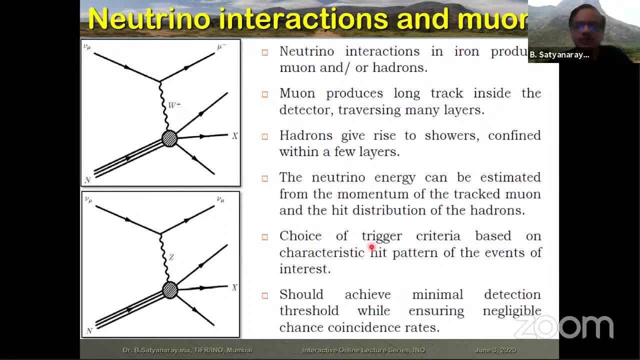 that is what is dependent: only on the hits that you saw. What are the hit pattern. You don't use any other detector, any other information. Obviously I want to have a very minimum detection threshold so that I don't miss. At the same time, if my threshold is too small, then I get a lot of chance coincident. 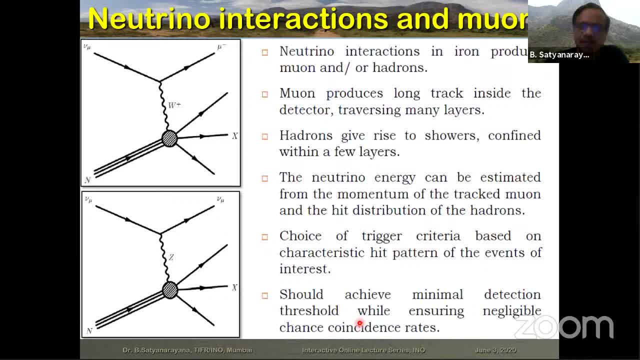 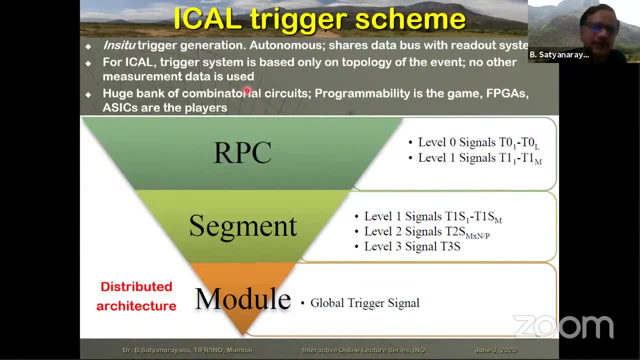 Chance coincidences where, just because there are random signals coming from the detector, by combination of that, I should not produce the wrong signals. So how you produce trigger, Some signals are produced right in the RPC detector itself, so that they are called trigger primitives, so-called level zero. 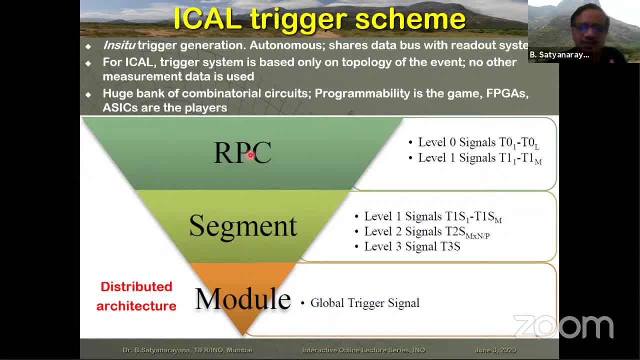 Some basic decisions about. you know whether or not this is useful or not is produced right. Okay, So you have the RPC one detector element and the segment is a part of ICAL detector. So the next level. so these signals go to the segment level where higher decisions are taken. 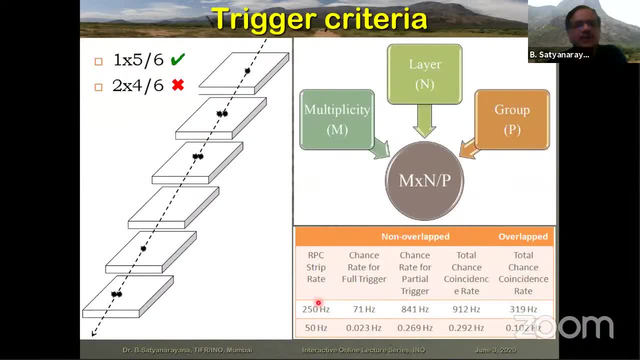 And finally, the global trigger produces at a module level. Okay. So, for example, if I say this is my track, it is passing through six layers, And if I say tell me that out of six layers, at least five layers must have at least one hit, 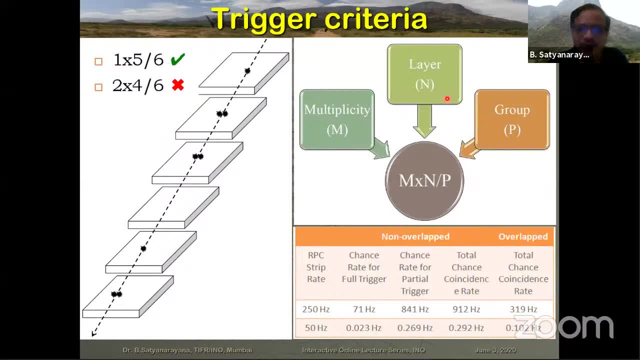 Okay, So that is out of six layers. At least five layers must have at least one hit. Okay, That is m cross n by p. If you can see that, I'll be able to pick up all of those muons which are passing through, because they typically hit one. 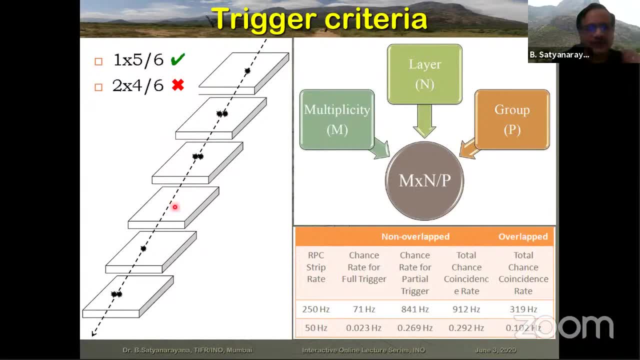 But I'm also taking care. once in a while one of the detector might be inefficient. So I'm not asking six out of six, but let us say five out of six. But let us say somebody is looking at little hadronic kind of interactions. 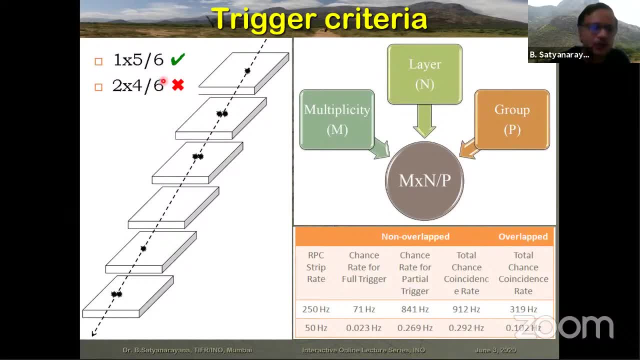 So I'm asking no now I want to, for example, in this: if I say you look for a six out of four out of six, but let us say, see two hits, the the doesn't generate trigger because you have only one, two and three of them have two hits. 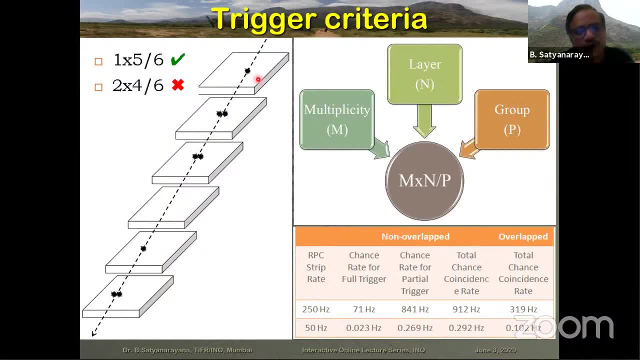 Okay, In some cases, if it is only confining to only fewer layers, then I have to generate another condition. Maybe, say five out of that, maybe two, maybe two of them. Maybe I'll be then able to get more shower like triggers, and here more muon like triggers. 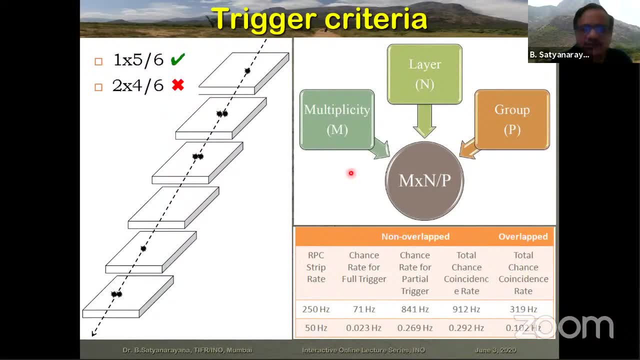 I have to really decide and put all those conditions in these various combinations, but I don't have time here. but I also said it's also important when you choose what is your trigger criteria. you also don't want to generate all spurious so-called chance, coincident trigger. 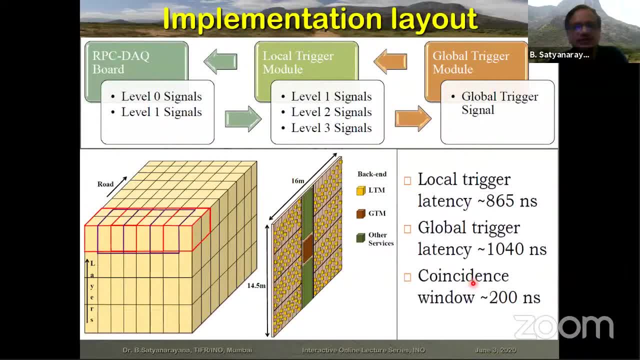 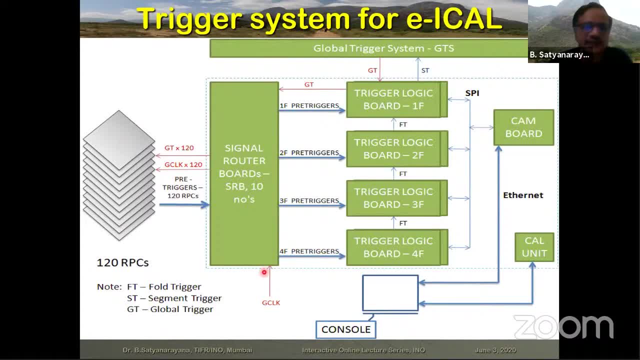 So, therefore, you have to be very, very careful about those things. Okay, So when we put together- so this is your, let us say, a segment of your RPCs- you bring all those detector here and, depending on whether it is a one hit, two simultaneous hit, three simultaneous hit, four simultaneous hits, four. I mean four strips, three strips. 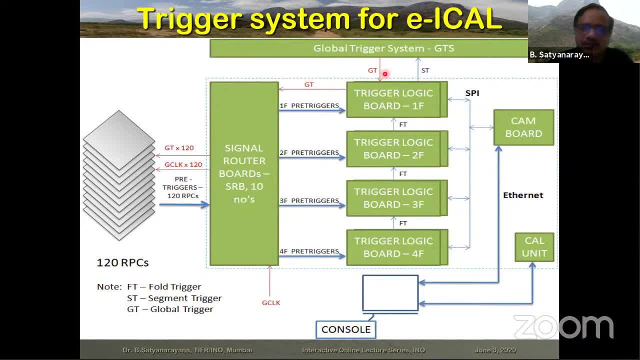 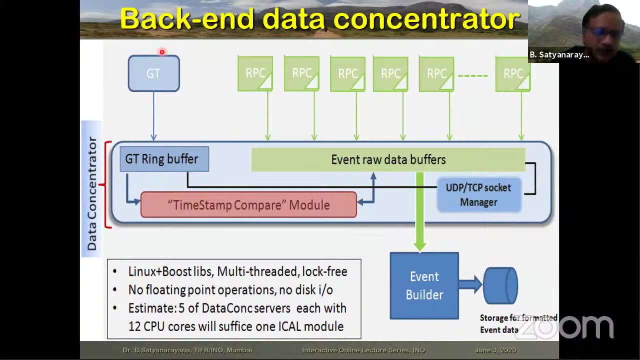 Two strips and each one of them, you allocate that trigger decision by a separate board here and all of them put together. Finally, they decide what is your, the final trigger system, the global trigger system. Once the trigger is produced, what I should do, I should. once the global trigger is produced, the backend system should receive the trigger and then say, oh, at this moment of time I have actually received a trigger. 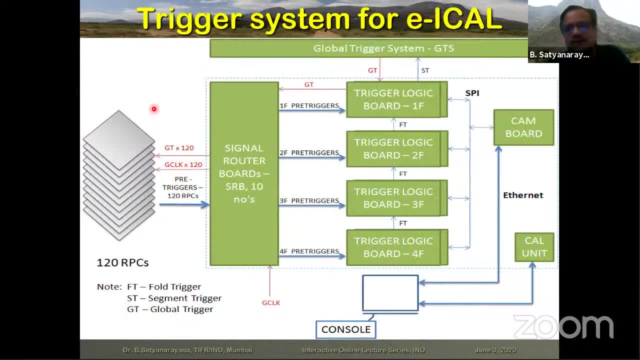 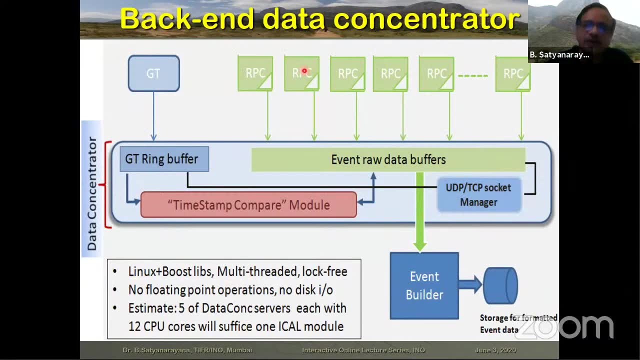 Immediately, that trigger is also going to All the all the RPC units, because that trigger goes back to them and each RPC. you remember the triangular board that is actually picking up collecting all the data- time data, pixel data, everything- and immediately started transmitting data, just like PCs transmitting data, sending data to the server. 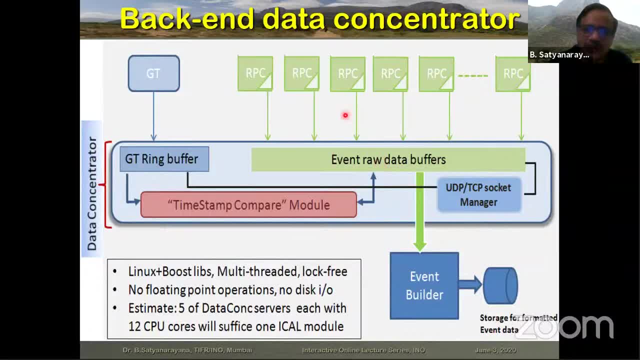 All this data comes to the pipe. here They're called event data buffers. They can come at any order because they come through the internet And this, this particular piece of hardware, is going to Look at the time of the recording, the time of the trigger here, compare that. 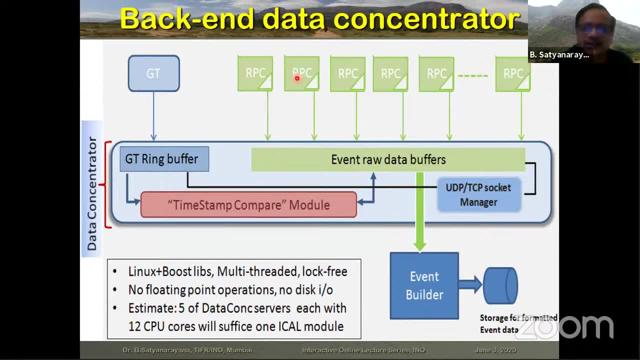 And if it is satisfied, saying that, huh, this RPC, this data, this data, they all belong to a particular trigger and then make what you call event. You build an event. Event is for that particular trigger, which are the RPCs which are, you know, giving you that data back to you. 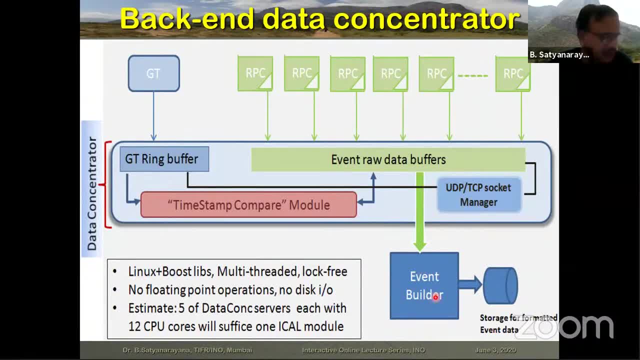 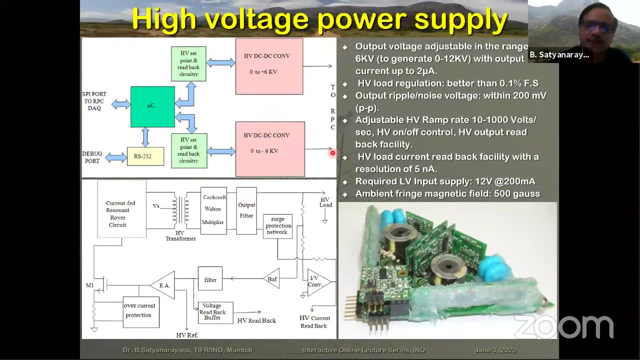 So all the data comes to you and then finally put a make, a build, an event and put it on your storage. Of course you will also Uh-huh, Use the signals and display the uh tracks and so on, on the on the thing. just remember, it's not just the uh sips and you know uh ICs, et cetera, that we will be even go ahead and build even the power supplies, high voltage power supplies- that are required to power the RPCs. 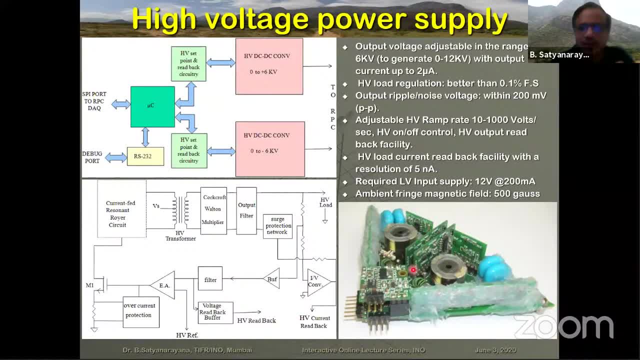 This is as for supply, which is looking a little ugly to you because it is not packaged, but this particular unit, again looking only 10 centimeter by 10 centimeter, taking, let us say, a voltage of about uh, six, 12,, 12 volts. 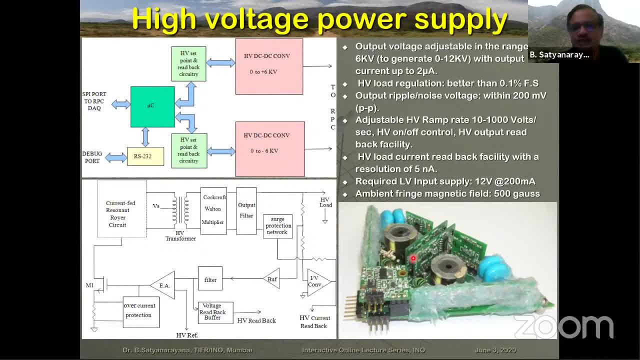 Yeah, It can actually give you plus or minus six kilovolts- Okay, Plus six minus six on both- which you can connect to your RPC on two electrodes and you will be able to produce, uh, let us say, 10 to 12 kilovolts between the two electrodes and produce the fields that you require. 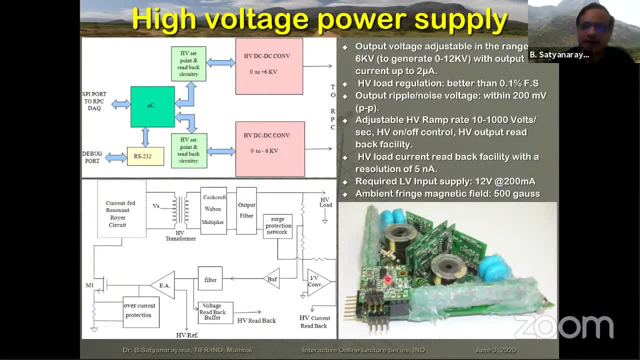 This entire unit will be is also a designed and fabricated, and we need, of course, 30, 40,000 of those things. even power supplies have to be produced for specifications that are required. You don't buy it, So you can see a big collage of all the developments. 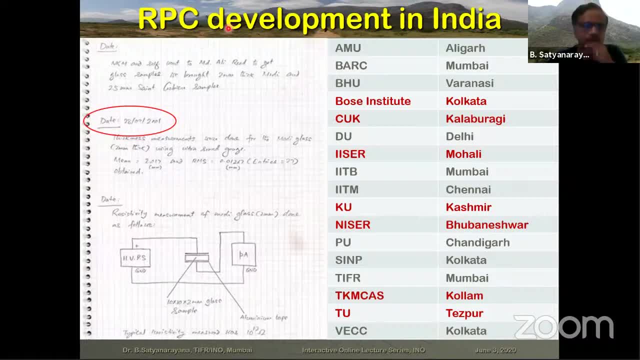 That you see here And uh, as um the book said, the RPC story in India started in 2001,, September 28. here you can actually see a log book which is actually a page of that I shown. 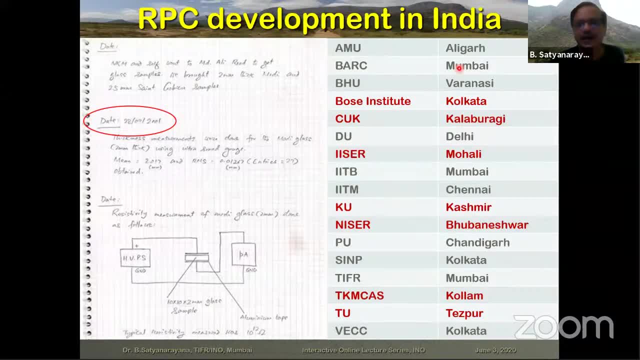 But today you can see there are so many institutions. uh, they have later on built RPCs, RPC labs. They also built for many other experiments. The one that's shown on right are the students and postdocs that went out of INO and built their own RPC labs in their new institutions. 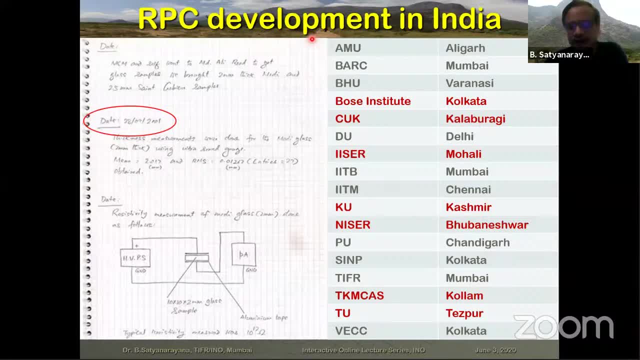 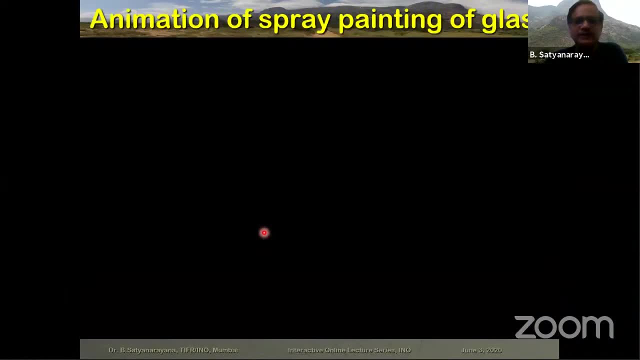 Of course, when you start RPCs like this, which you build and characterize in the lab, you have to also go to industry and fabricate them in the in in large numbers, Right, Uh? so, for example, many methods that I I was telling to you, uh, saying that you know, you paint uh uh, you put a graphite uh uh code on that so that you can apply voltage, and so on, and so forth. 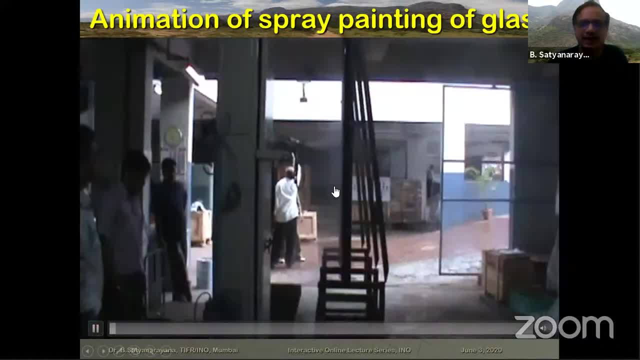 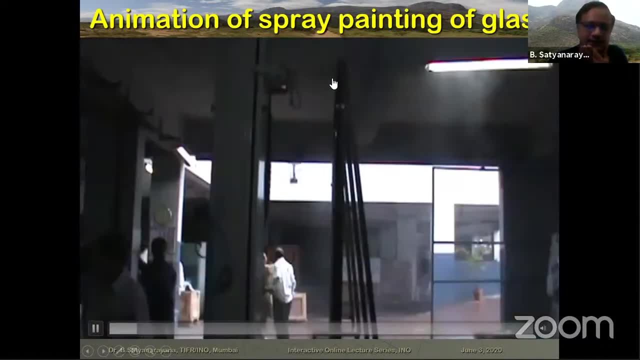 How do you do it? You can't do uh uh, take a brush and start painting. So you have to Actually make such kind of gadgets where it should be able to kind of paint on a glass. This is a two meter by two meter glass. 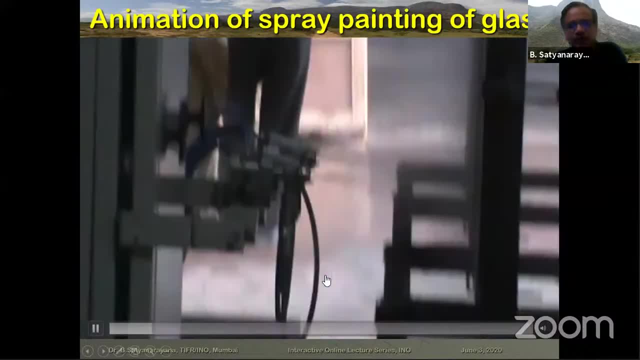 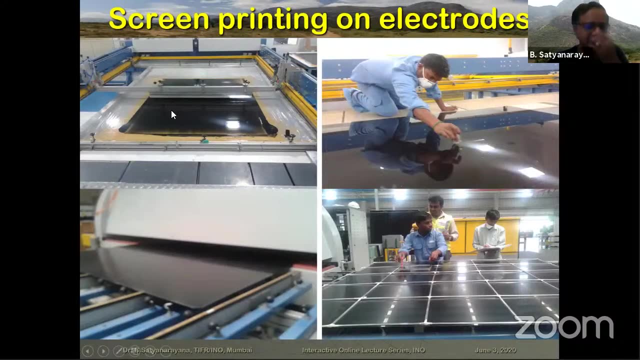 You can see how easily it is able to paint X and Y positions. You can also paint it using what is called a screen printing. You can see, this is two meter by two meter glass on which, in an industry- glass industry- this is actually being printed and, uh, you know- cured. 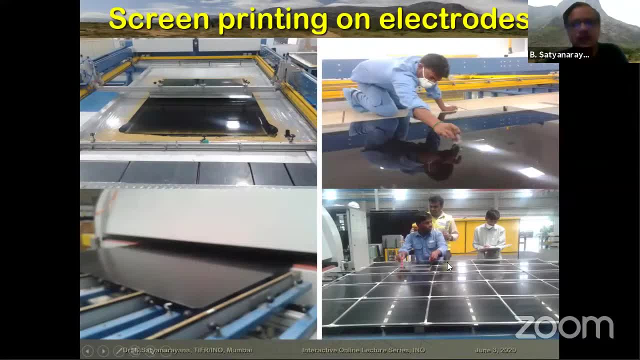 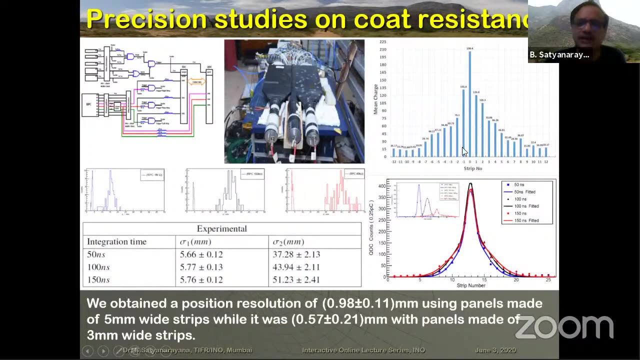 And also the measurements are made on this, And some of the students actually do projects and say, uh, depending on what is the resistivity of the paint that I show? And here, um, uh, what is it here? Uh, what is the kind of you know, pickup or crosstalk that is going to happen from one channel to another channel? 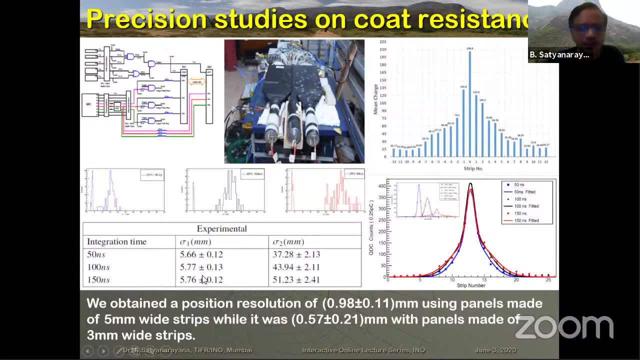 This is very important. You can see a result here which tells you that, uh, depending on how what's, how fine the pickup strips that you will be able to use. For example, I said we are initially- I said- 30 millimeter wide strips, but if you go down to three millimeter wide strips, you can actually get a half a millimeter resolution. 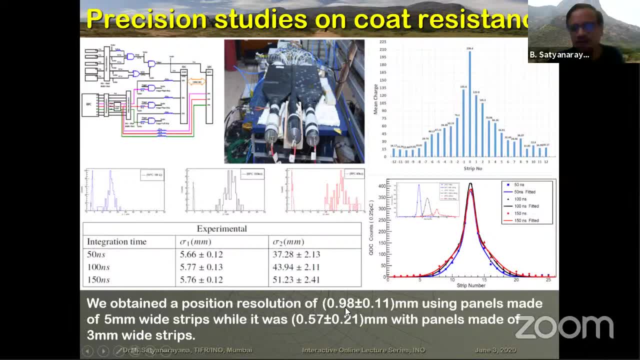 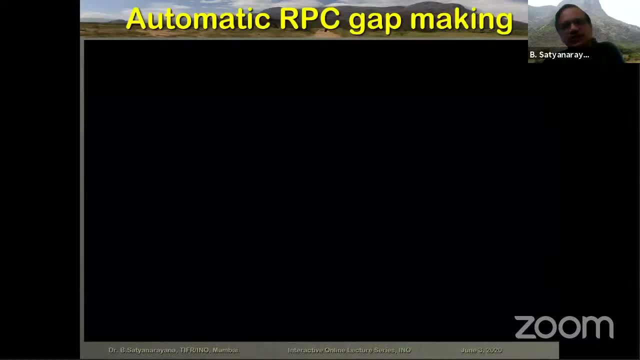 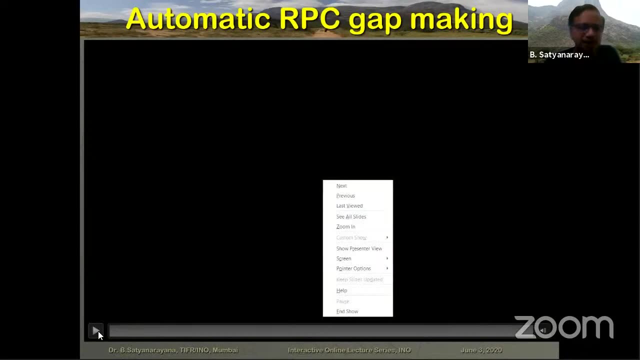 If you use five millimeter pickup strips, You can get one millimeter resolution. So this is what you can actually get subsequently after you get the basic raw data. So these are the kinds of studies the students do after you get the glass. Of course, again, you don't go and make uh things the way you make it in the in the lab, everything manually. build a robot to do that. 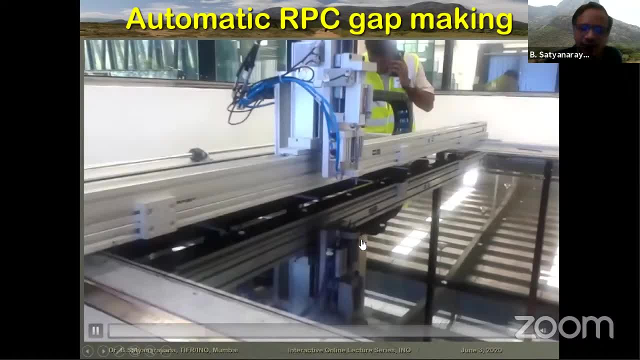 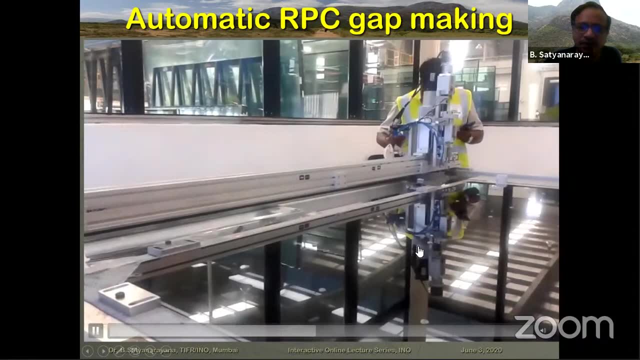 So you can actually see that there is a glass which is sitting at the bottom and these buttons, If you remember I mentioned to you, they're all placed here and glued here and this mission, One button at a time, going and placing them, going and putting glue, and then you know and go and so on and so forth. 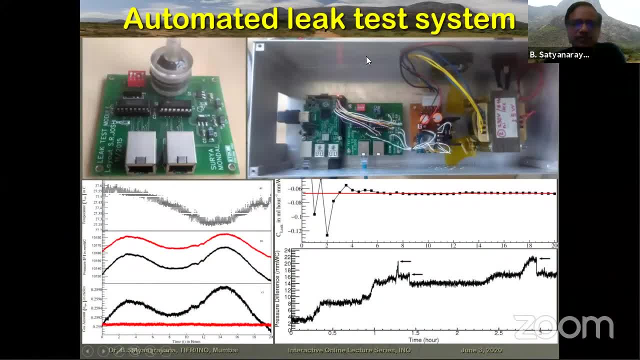 Right, And after you build the entire gap, of course you should also ensure that it is all leak proof, And another student actually built this system using an embedded system. You know, nowadays people use agrinose and raspberry pies and things like that. 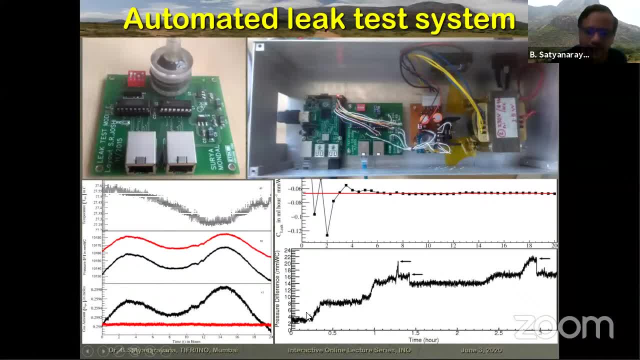 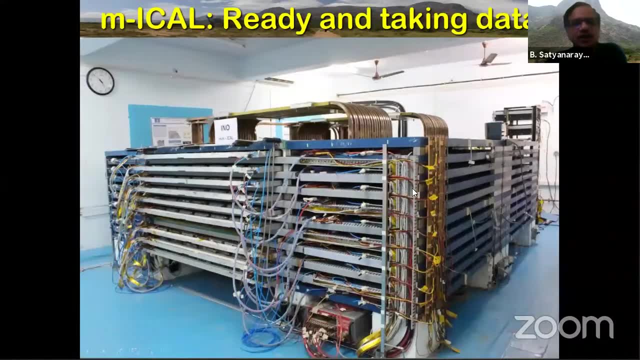 And very beautiful system which can kind of find out very, very minute leaks in that, Yeah, In the full gap of, you know, two meter by two meter, by two millimeters. Okay, After all that hard work, of course, we build this tiny little baby, what I call mini I cal, which is now a reality. 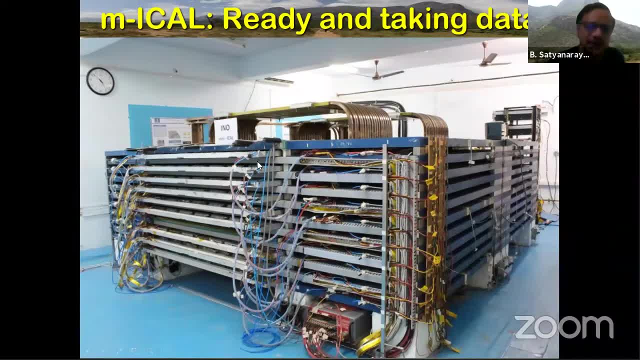 You can really see that these are the iron plates that I showed you. These are the last two meter by two meter, our pieces which are inserted And this is the coils that is actually producing the magnetic field, This magnetic field that I talked to you about. 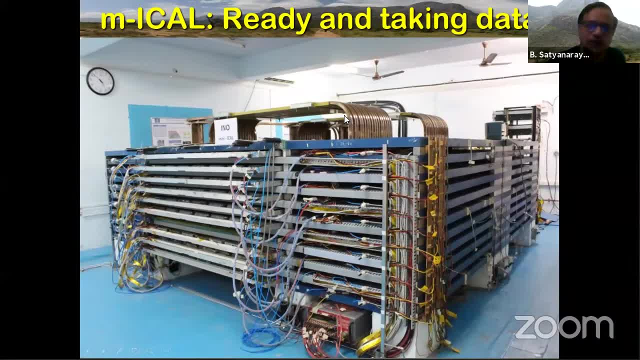 And there is a big ancillary system which is also, which also cools this coil couple of coils. There is a cross section to which you cool low conductivity water, chilled water, so that you know it doesn't decrease the temperature when you flow thousands of amps of current. 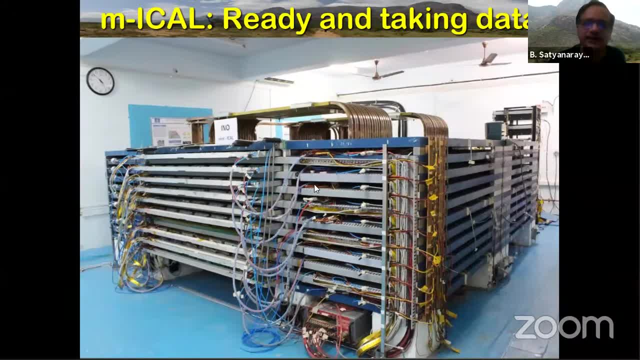 Right, Okay, And so you can see it has every component that is required for a big detector, But except that this is about four meter by four meter and only about 10 layers here. But every component, single component of RPC is actually demonstrated. 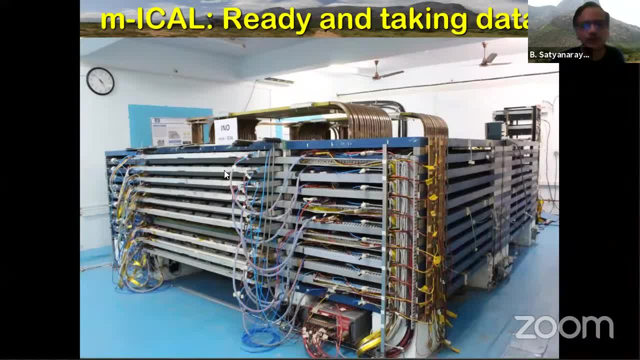 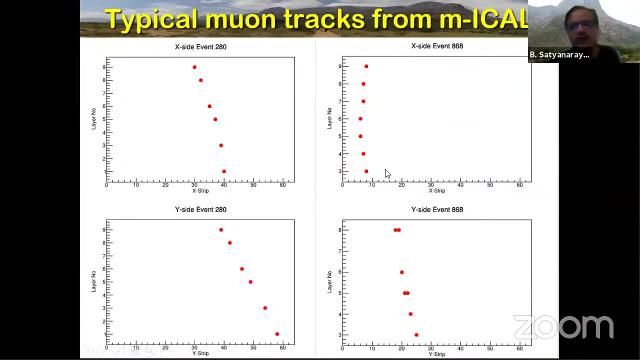 And you will feel very happy When you magnetize such a detector, when you see the cosmic muons- of course this is on surface and the band and students working on it and able to kind of look at the momentum, you know when they can calculate such a bump for this muons- you'll feel very happy that the whole detector is working the way it's working. 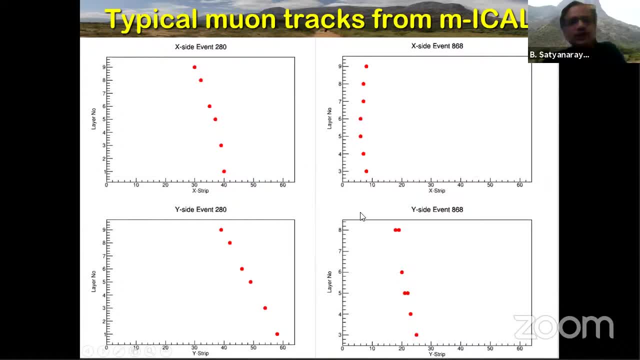 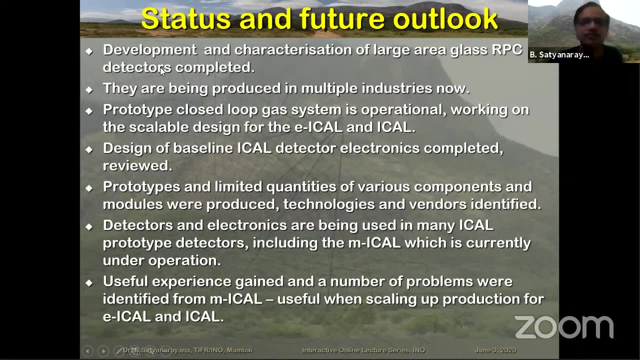 And it is now actually scaling up in industry is what is kind of frequent. So I want to. I'm sorry I took a little more time. I just want to end by saying development and characterization of very large- Yeah, Area class RPC is actually completed. 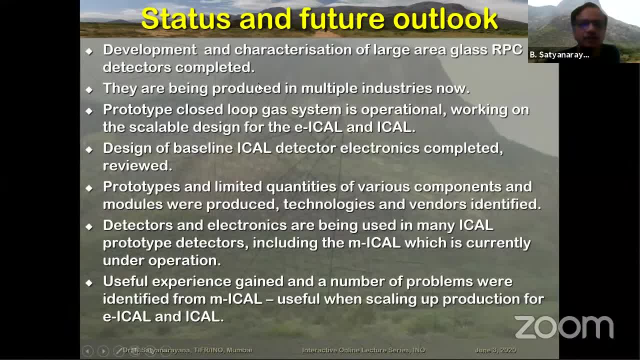 That's a very, very exciting journey. And then, of course, now being produced in multiple industries, especially class RPC class industries. We also build closed loop gas systems And I showed you now for the bigger detectors. of course, you need to scale it up. 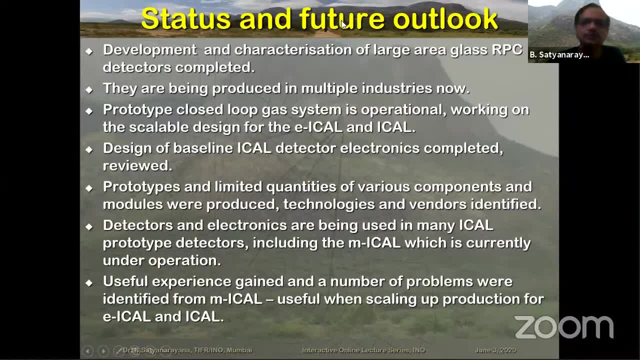 And all the electronics that I very quickly went through are actually designed And now we are waiting for them. Prototypes are all limited quantities purchased And the detectors and electronics which are actually Being used in many, many prototypes. I've shown you four or five prototypes and, including the mini icon which I showed you with the last, that is what is giving you a confidence that the whole system and it is put together. 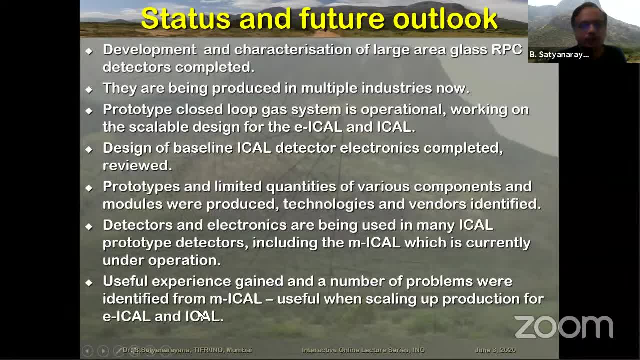 It really works, So useful experience gained and a number of problems which we identified during the mini icon operation itself. That is very useful because when you want to scale 20 to 300, 300 to 30,000, this experience becomes very important. 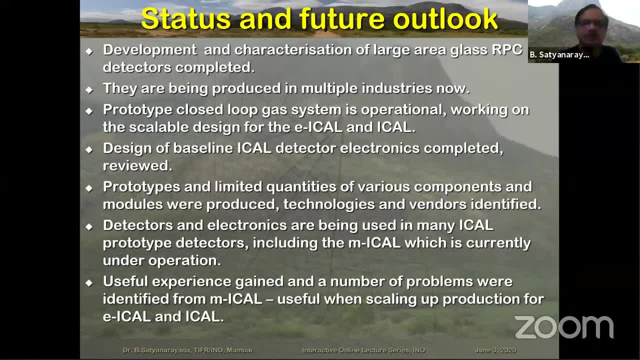 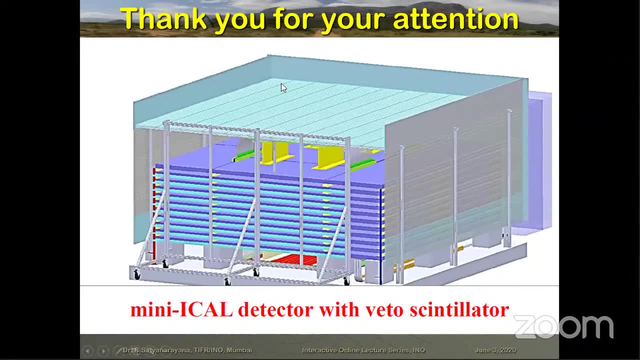 Okay, So I want to thank all of you. Uh, Thank you for your attention. Thank you, Dr Satya, for your nice talk. So now the session is open for questions. So if you have a question, please raise your hand. 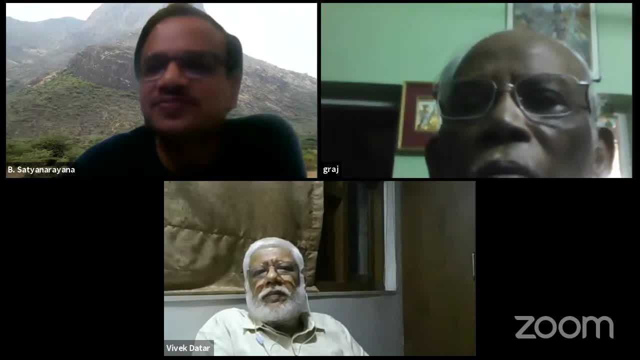 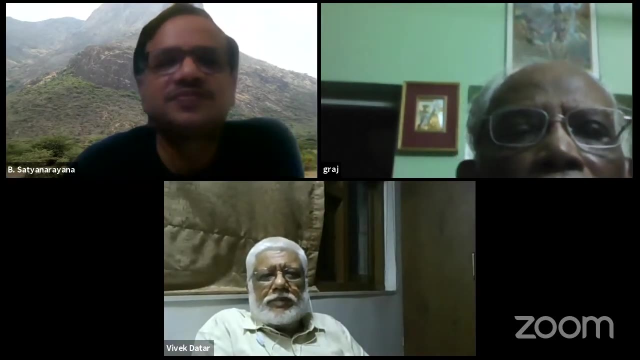 I think Silas has a question. All right, Yeah, Uh, uh, Silas can. uh. yeah, I think he has gone now. Oh, okay, Yeah, Hello, Yeah, He can hear you. Yeah, I have a couple of questions. 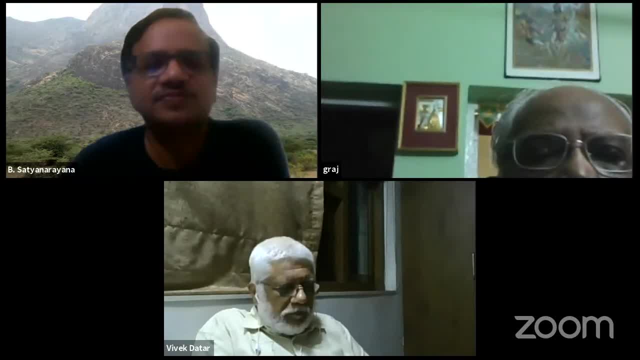 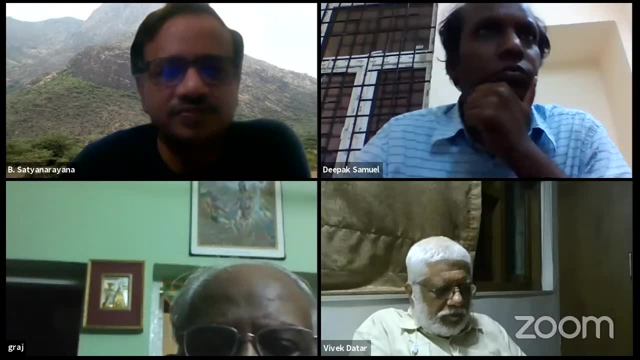 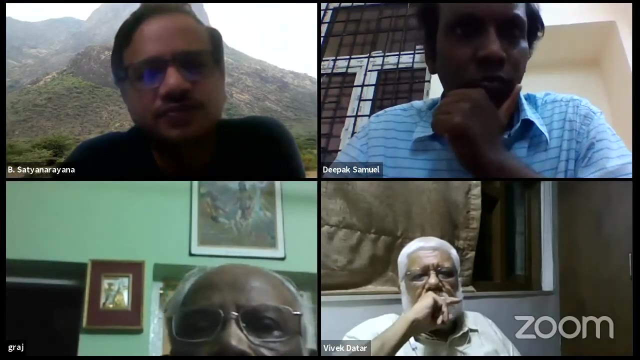 Okay, Uh, in the covenant rains detector they had a delayed coincidence which, uh, which proved to be a better technique to remove other possible background events. Okay, Is there a similar possibility for ICAL, where there could be some other delay? 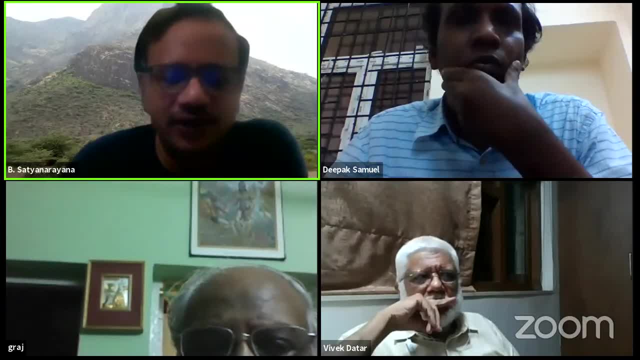 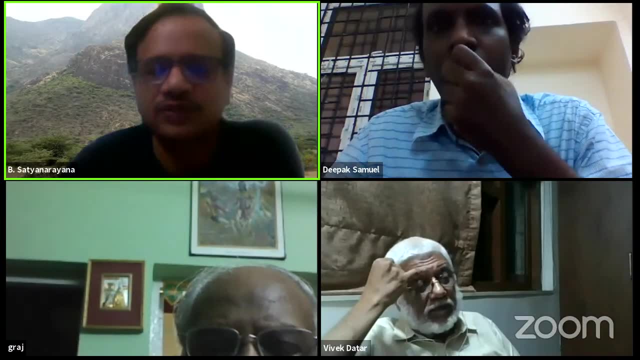 Could you say that there are some other features to it. Well, it all depends on what detector that you designed and what is the process that happens inside the detector, Right? Uh, so I mean, yo, what kind of technique that you want to use? 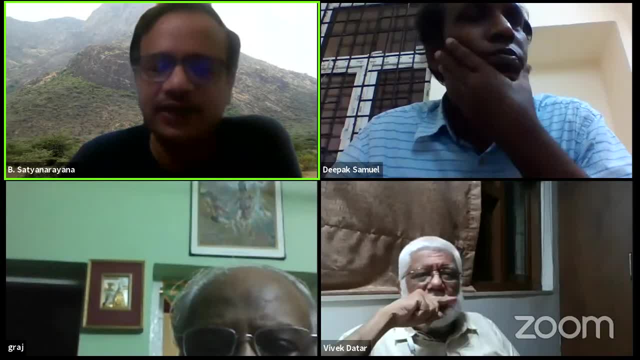 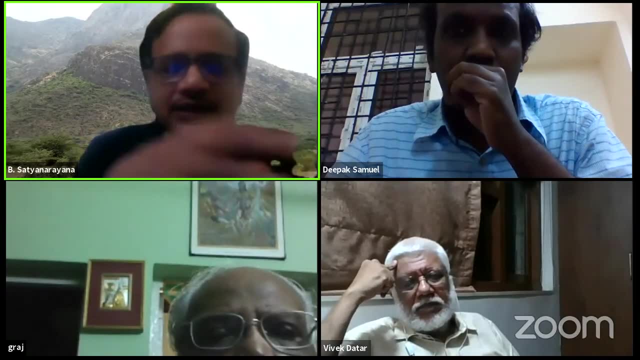 Very much depends on what, what did the detective technique itself. then you can really see, uh, you use, uh, let us say the prompt, um, the, uh, the photons, and then delay the Neutron capture right. 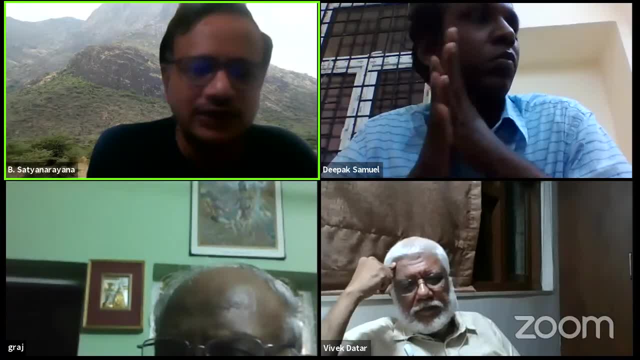 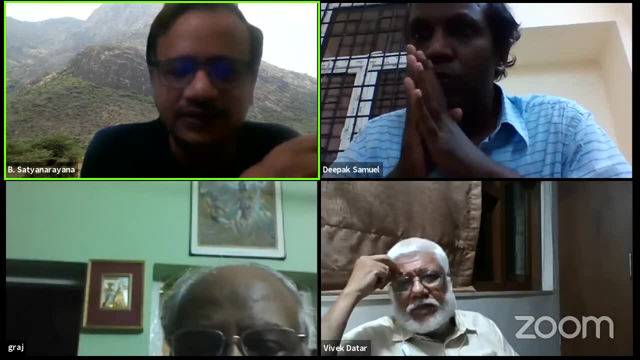 So for them you can't stay that effect if you capture only the two photons that are coming out and you declare them as an event, because it could always happen through many other processes. But when you actually tag them together, you are nailing down saying that this is the process that happens in my 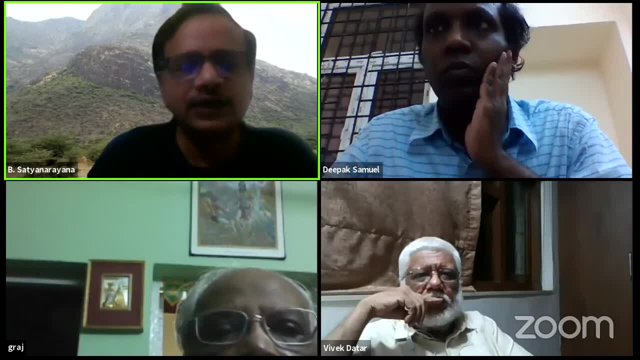 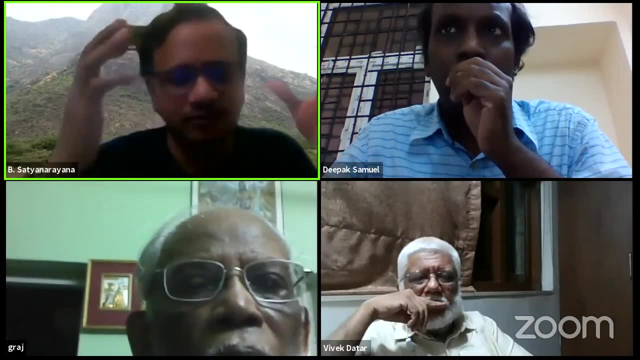 active detector volume, and this is how I detect. In this case, the idea is different. Here you are using a magnetized iron calorimeter. Now, as the you know, either plane cosmic neon, which happens once in a while, maybe pass through, or, let us say, the charged particles. 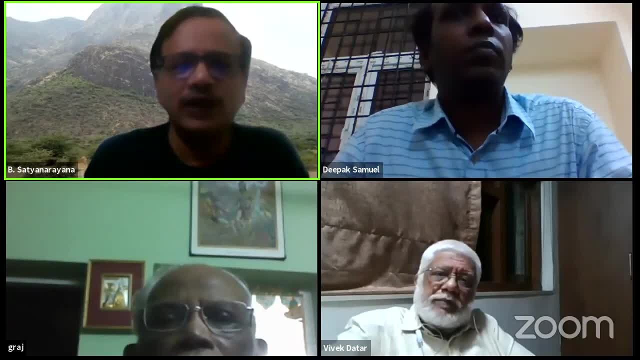 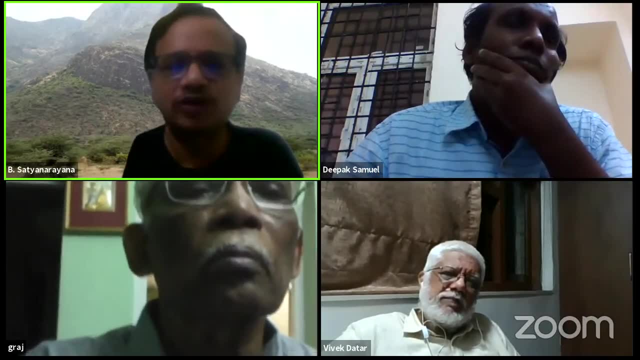 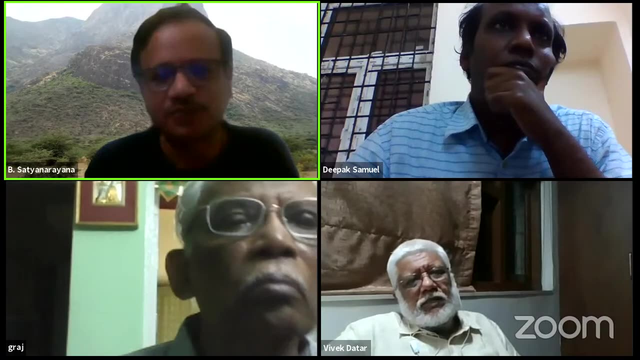 which are produced due to interactions taking place. you only have to measure their kind of. you know, what I said is their coordinates, and you also have to measure the timing, because you want to see, let us say, whether they are going top to bottom or bottom to top. 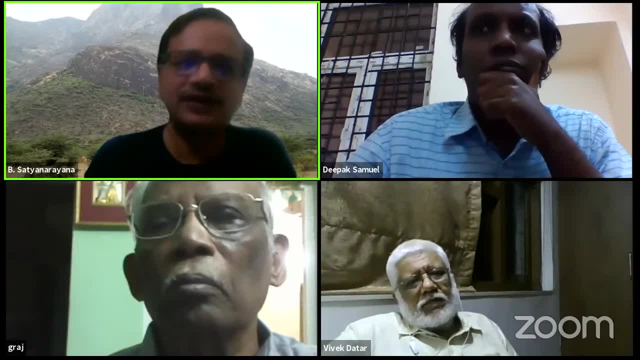 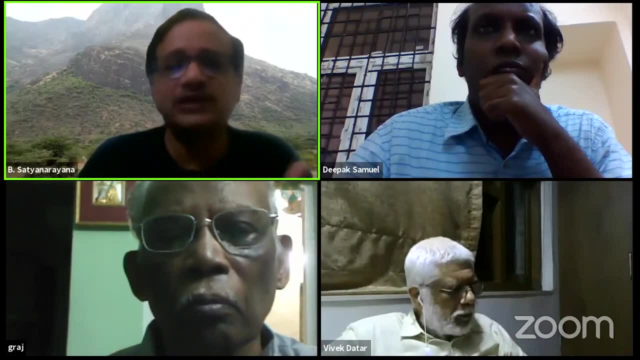 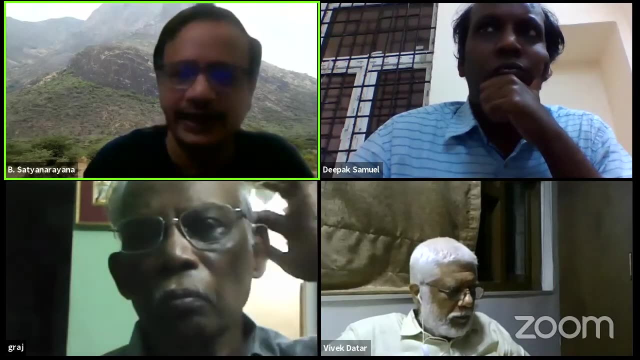 So this is the schema of things here- are different than the schema of things that they had in their detector. It all goes by. you know, for example, the same detector, suppose you say. I also want to look for very, very slowly moving particles, for example in the ICAL. 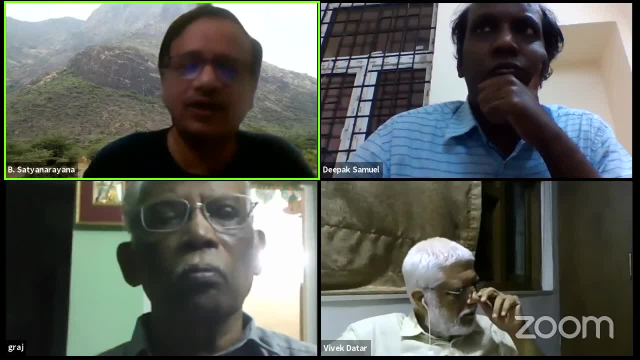 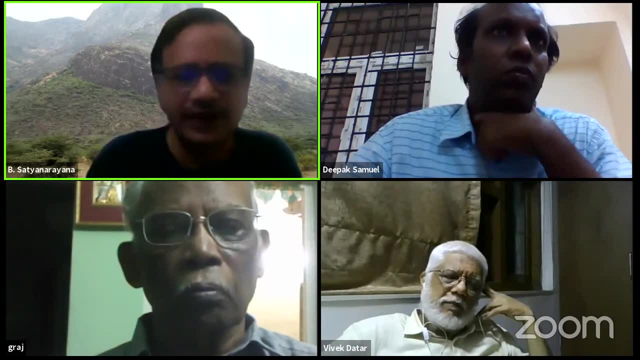 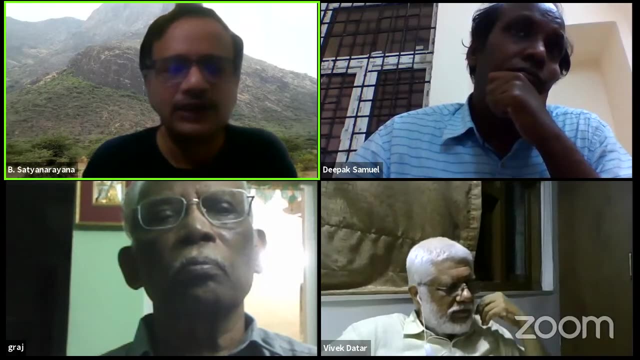 Okay, Then maybe your concept will be different. Here they're all relatively particles, So you can put a window and then look within that window. you know, for a trigger right, Because even such a big detector you can. you can put a one on one. you know, one microseconds. 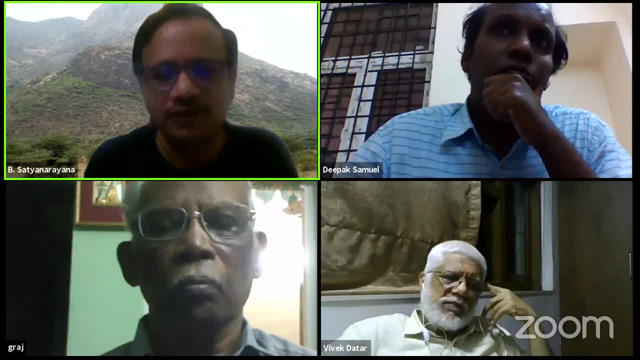 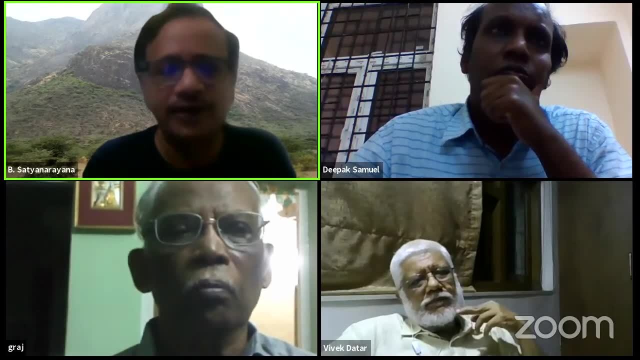 window and things like that, and provided your chance, coincidence rate doesn't become too large. But if you say that I want to look for very slowly passing magnetic monopoles or some such thing, then I can't brute force have large window. right, Then it is possible. 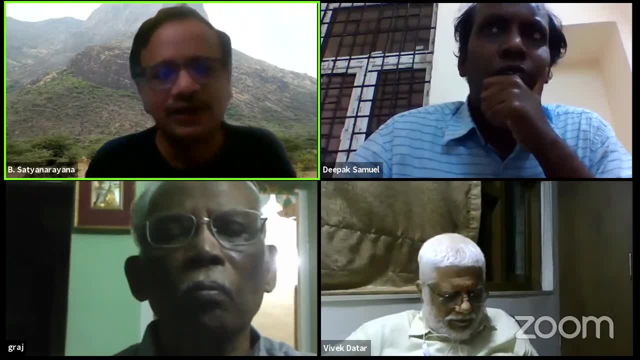 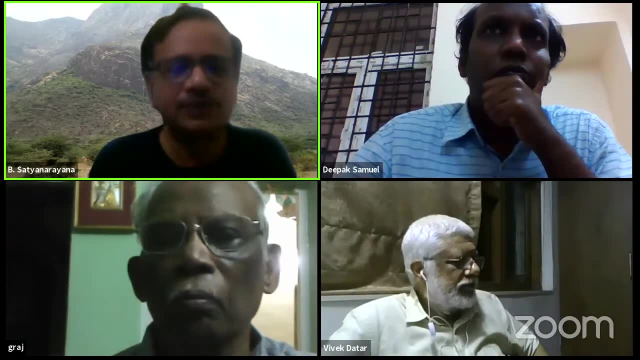 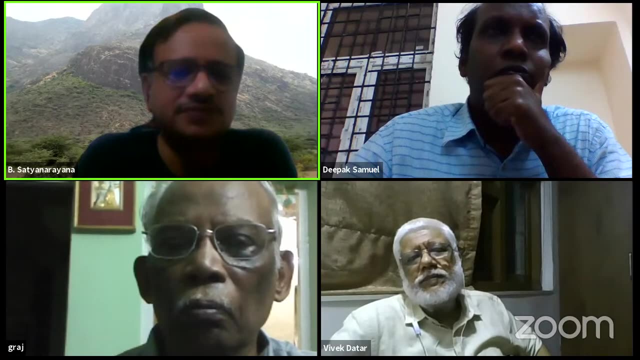 that I may have to look for such a sequence or some other smart way of capturing this, So it all goes by. what is the what is the detector concept and how you want to build the overall sequence, The overall detector and the trigger system and the instrument? 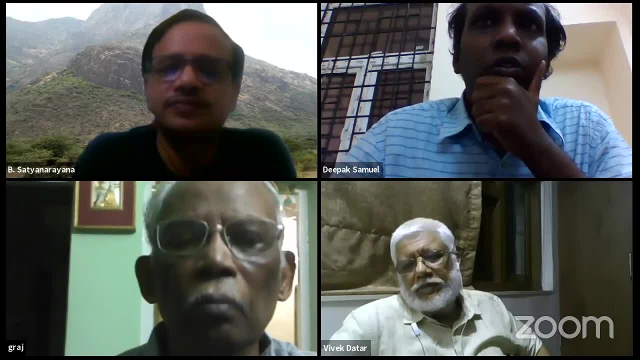 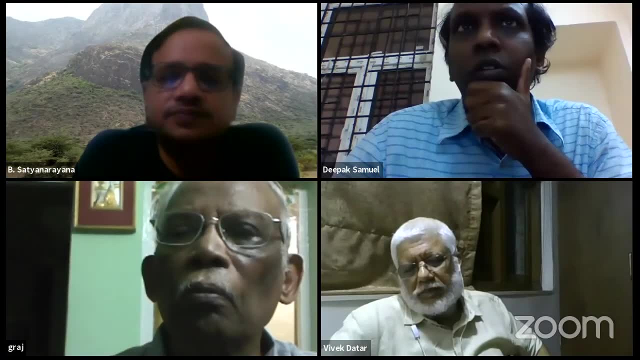 And my other question is: like the individual electric components, like the transistors and all the things which we are using, they have their own individual time delays of the order of maybe picoseconds or nanoseconds. So there are a lot of them in the circuitry. So can 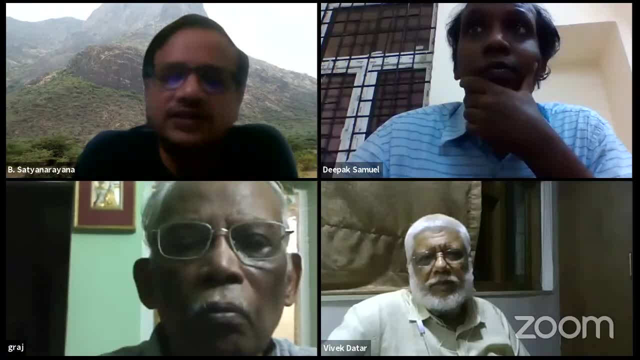 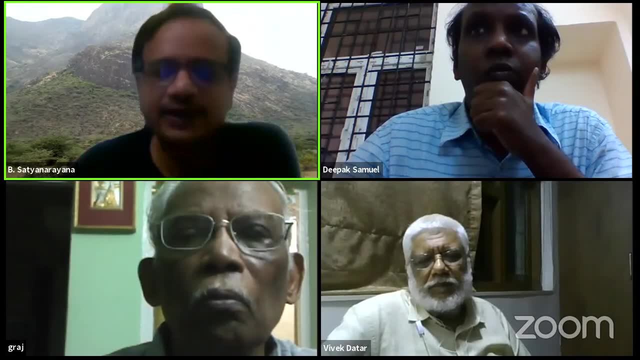 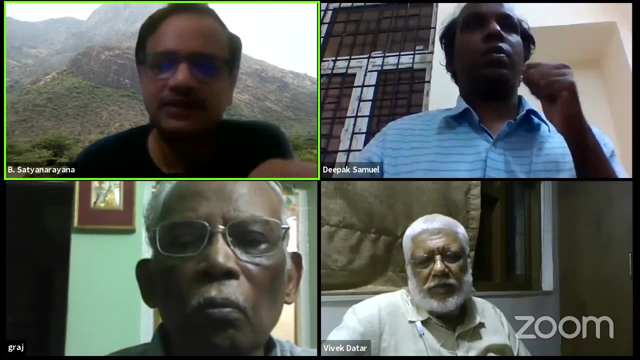 we still get the nanosecond resolution in our detector? That's a very good question actually. As you said, that typically, depending on how you design your ASIC right, There could be a lot of jitter. if you kind of call, For example, for analog system, it is different for digital. 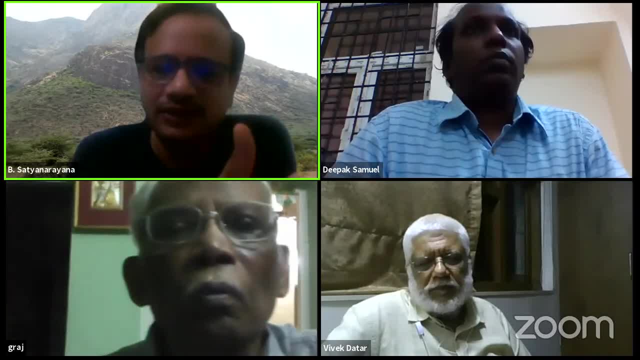 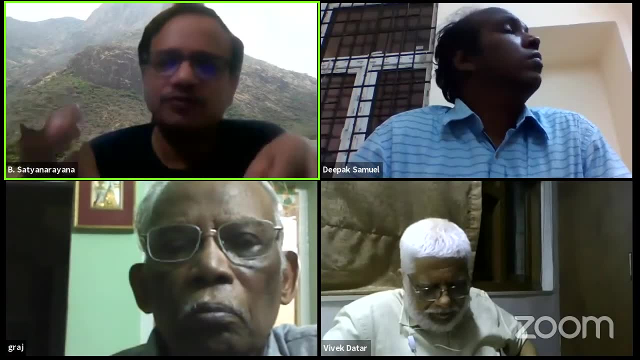 systems. it is different. Let us first look at very quickly about the analog system. Analog system use like, like what you saw. one of them is an amplifier circuit, right, Okay, So, which is, in a way, it's like an op-amp, but op-amp built with, let us say, transistors. 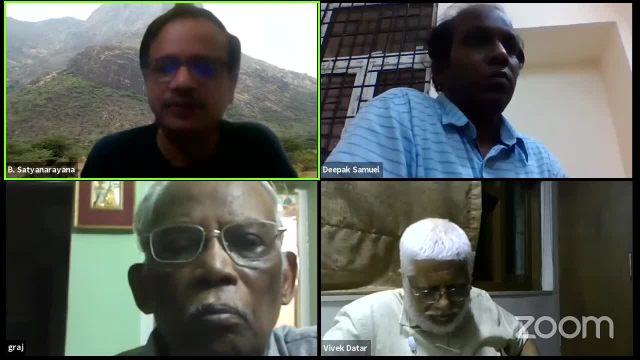 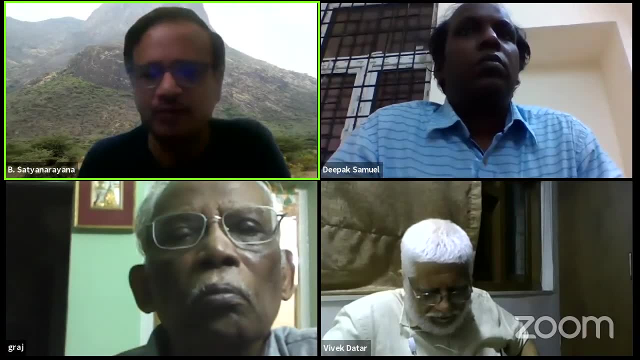 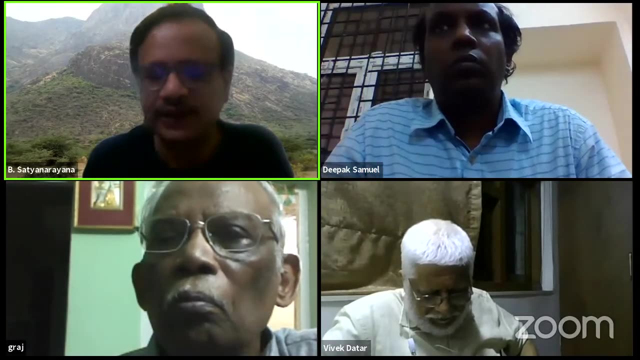 a large number of them. Now, depending on how they, how you connect between one to another, there will be always a jitter between, let us say, one stage of an amplifier to the other stage of amplifier, even within a chip- not on a PCB, or you know, tracks or wires or something like that, Okay, Whereas if you go to the 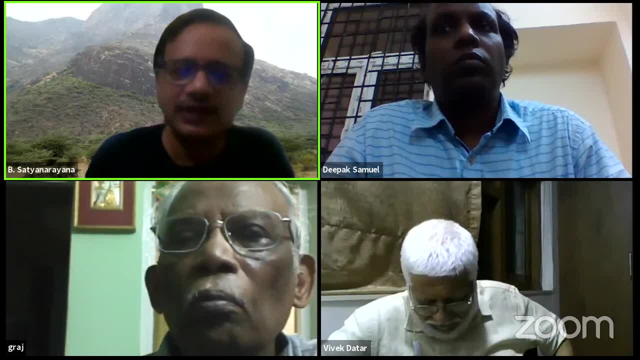 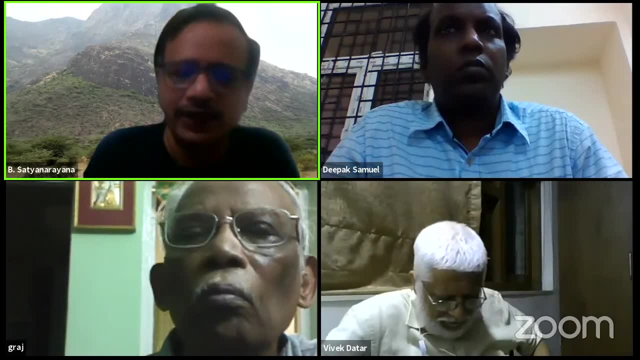 digital system. it is a little more complicated because many times the way you route them there are like gates, ultimately Okay. Now you also have to look at what you call a routing. just like you do on a PCB, you route one track from one to another, you also have to. 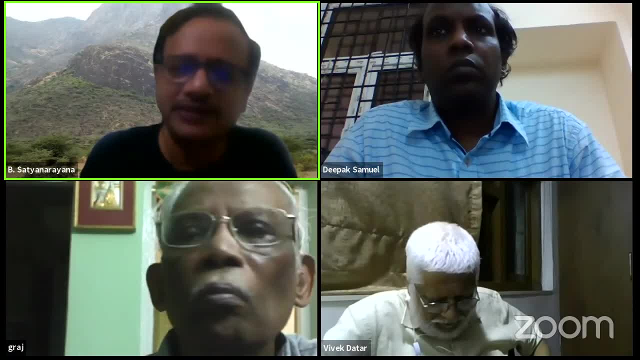 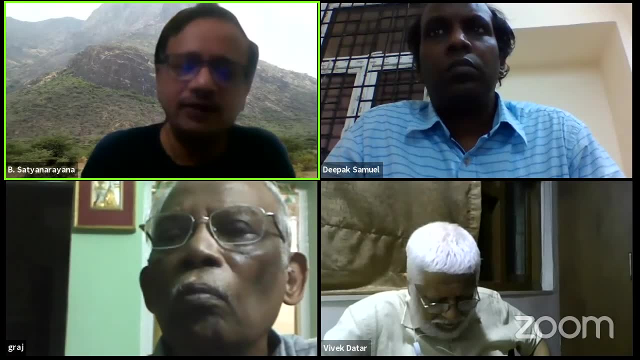 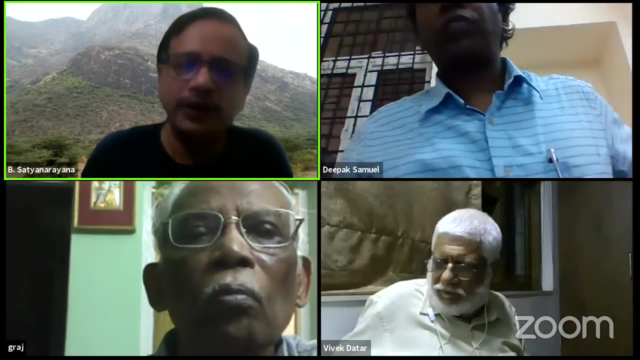 route inside and IC how the signal is passing by. Okay, It is true that you have to match to a large extent and thankfully, many of these VLSI designed tools- okay, sometimes they are called EDA tools- They allow you to able to simulate these systems to such a great. level. In fact, they use many times Monte Carlo simulation To get this high quality to level where these multiple path delays are optimized in such a way that it will give you the best possible input to output delays. So of course, there are parameters that you have to play. 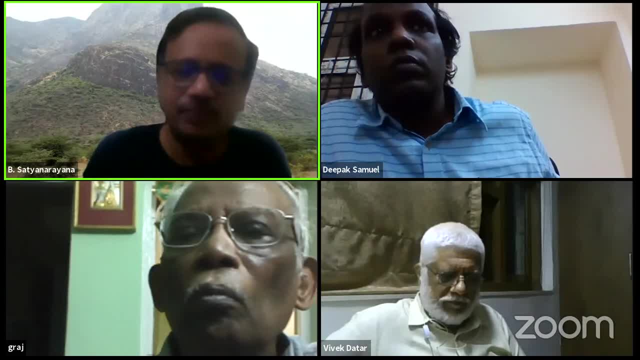 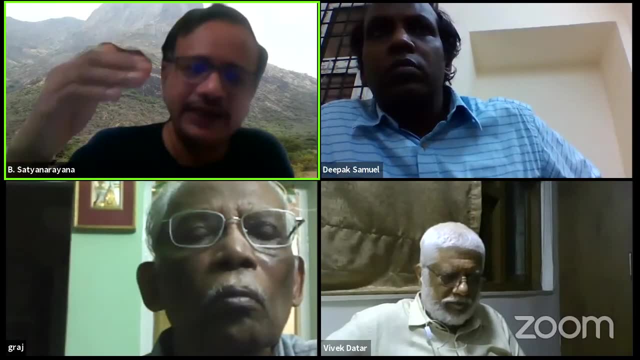 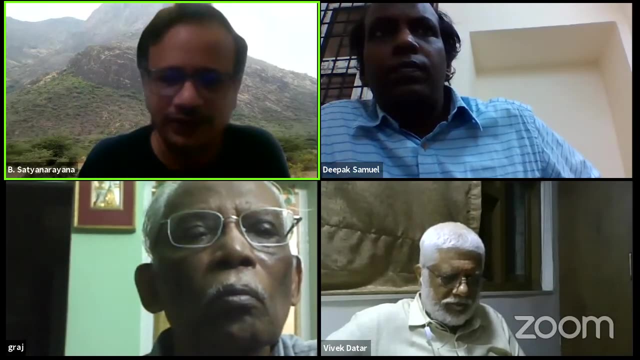 with Chip size versus power, versus number of channels, versus the speed versus. there are many parameters. but you can say that I would like to maximize my jitter, I would like to minimize my power, I would like to minimize whatever, whatever. And then these simulations really work. 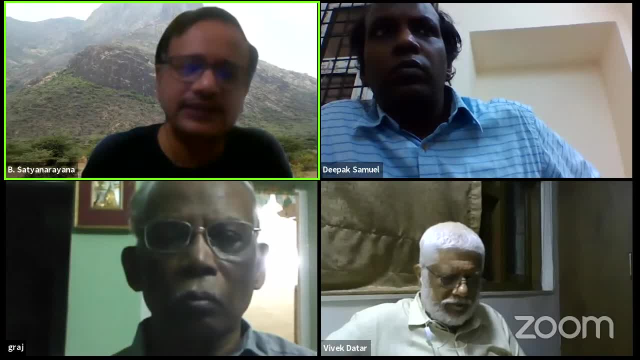 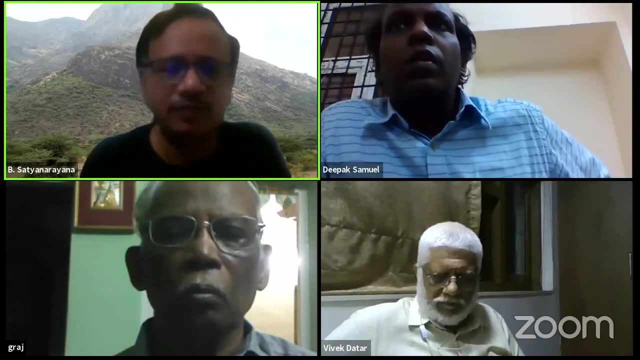 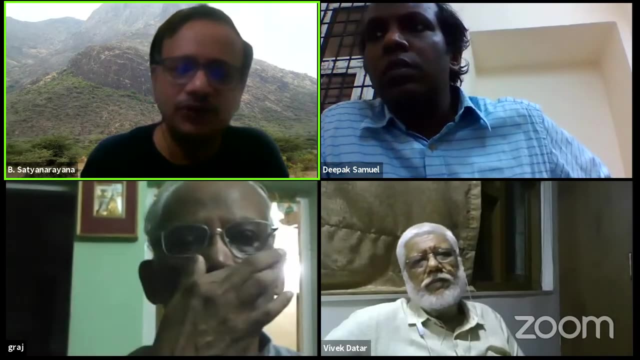 very well to you And the question is really nice in the sense: the RPC detector in this case, plus all the electronic chain that you see from amplifier to all the way there, when you actually do a characterization study in test stands the number that you come to you. one nanosecond to two nanoseconds or whatever. sigma is the one which is actually the sum total of all the jitter that you see. So this is detector plus electronics. Of course, there are also other parameters you should worry about. One of the most deadly thing is so-called time walk. The time walk is the smaller charged. 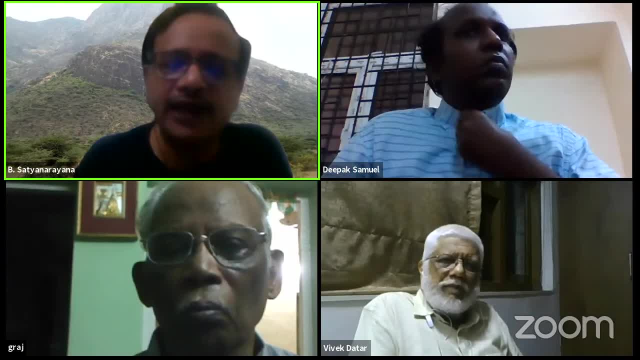 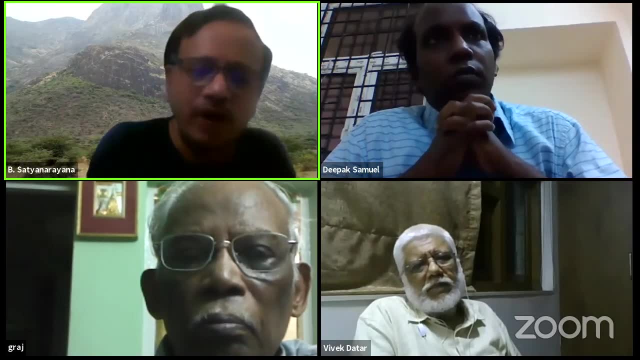 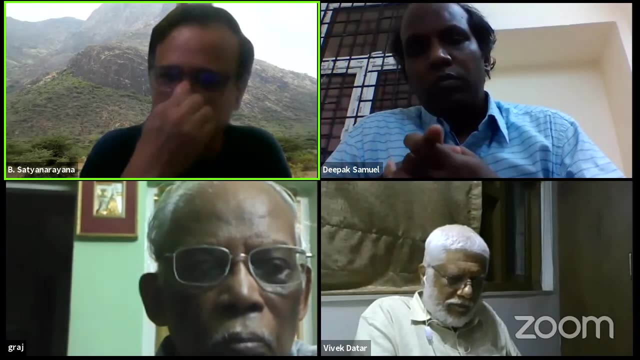 signal, higher charged signal. They do not have the same time profile, So the bigger signals are produced faster compared to the smaller signals, So they become kind of very slow. Now that difference itself can can kill the resolution that you are looking at in the RPC. So therefore you have to be really 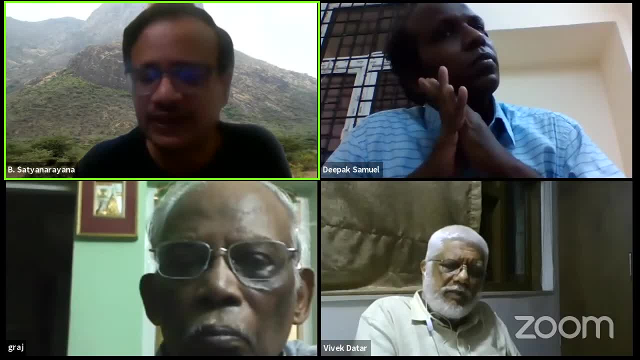 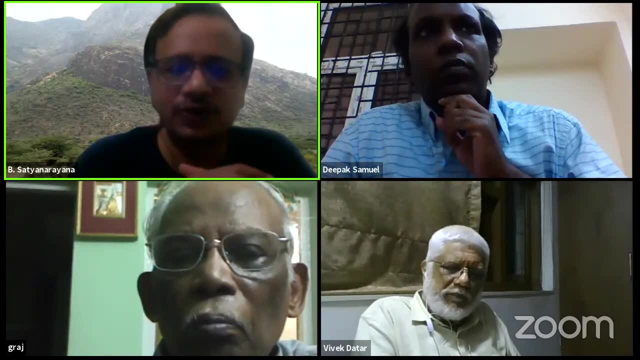 careful to overcome all these differences? Yes, but that is a nice question that you can't just simply or you know, or look. Yes, both detector side and electronic side, people have to come to. Thank you very much. Yeah, So we'll take a question from YouTube. 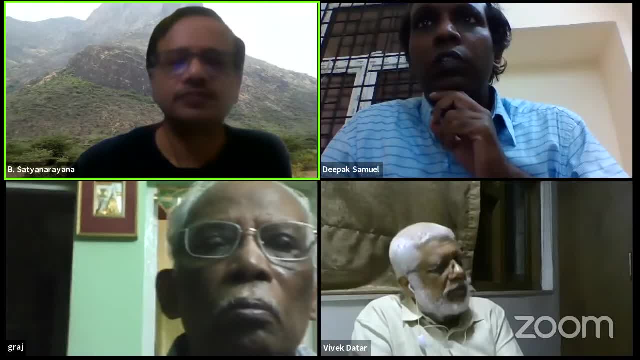 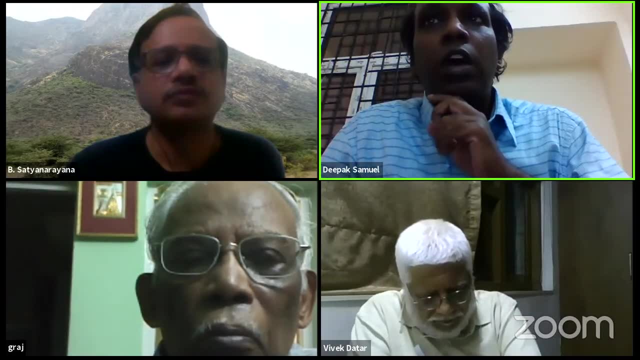 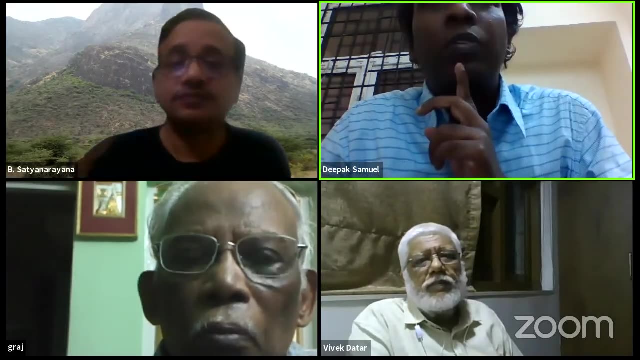 Okay, This question is from Sadashiv Sahu. So why do we need a continuous flow of gas rather than say, static gas pressure in RPC? Does it have any role with size of RPC? Does it what? Have any role with size of RPC? 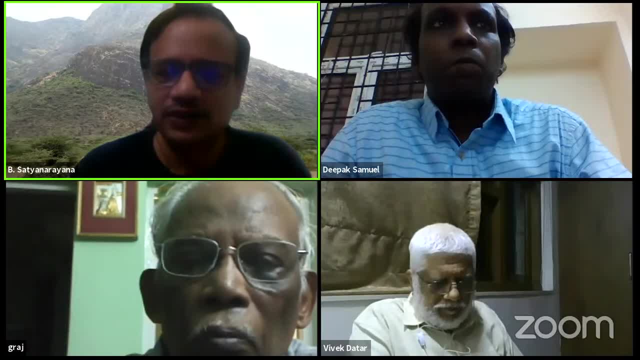 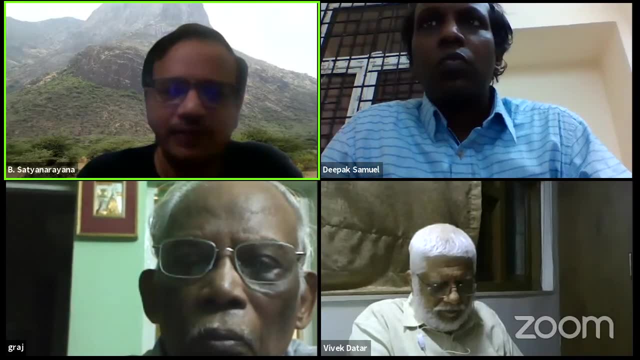 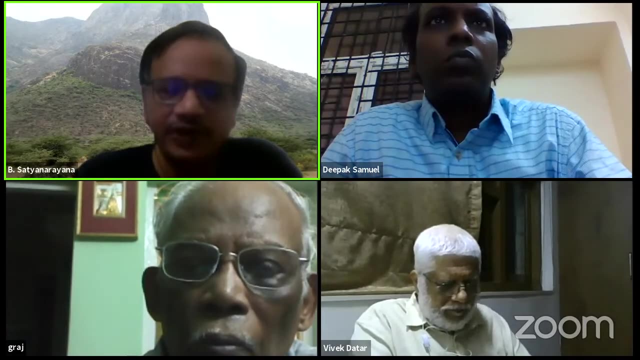 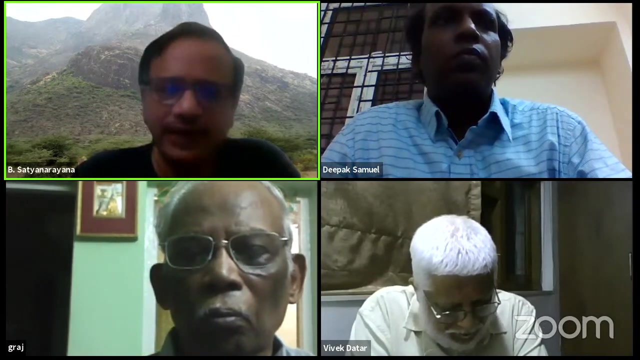 Yeah, So his question is about the so-called, you know, packed detectors, which are, you know, typically, classically, would have seen many proportional counters, cyanization counters, many of them, versus the counters that we have here, which are, which are operated at very high, let us say, electric fields, very small, you know. 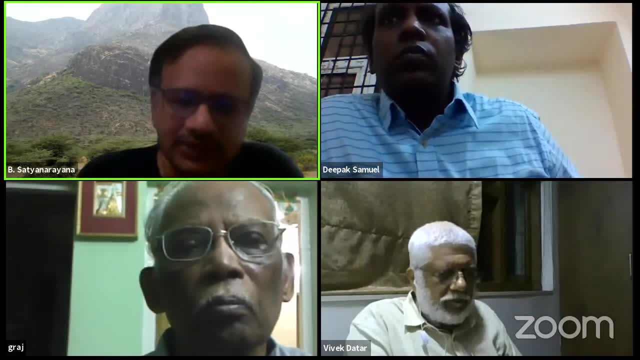 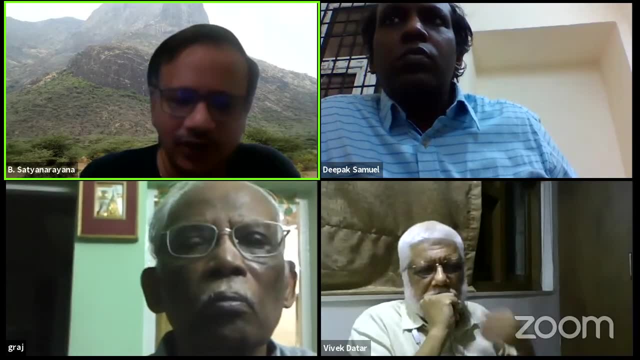 electrode gaps, And the process that you are looking at here is also very fast processes, not like olden days where you had rise times of few hundred nanoseconds. You are looking at rise time of the order of a nanosecond or two. Okay, So you're required to maintain. 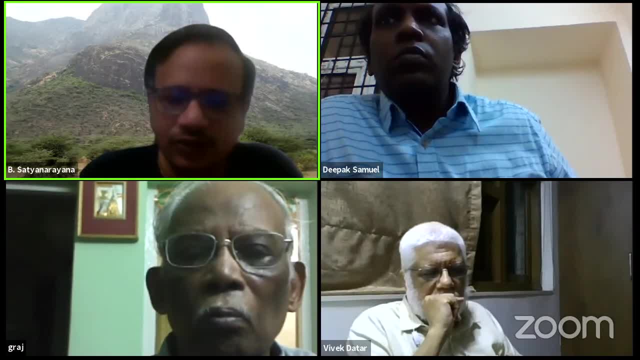 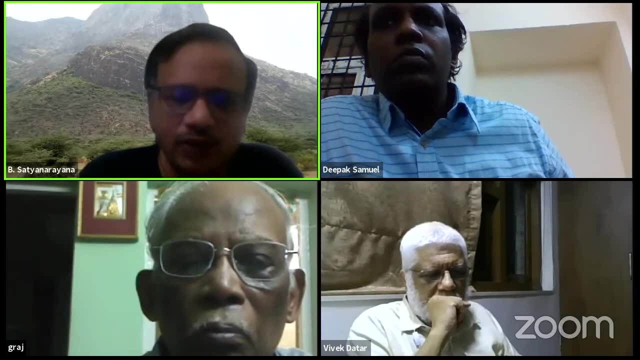 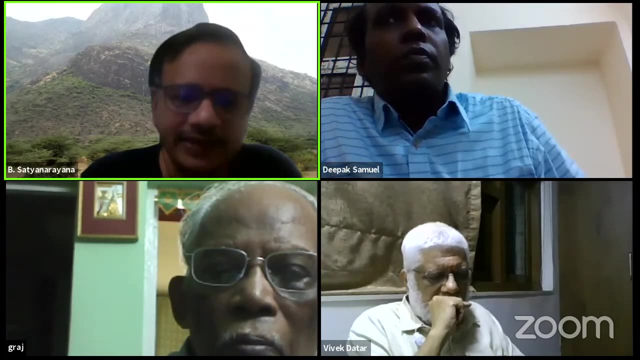 certain purity of gas so that otherwise, you know, the signals can be very kinky The signal if it is contaminated with some gas, some other, you know outside could be also giving you very funny pulses. So, in order to ensure that the gas volume that you are projecting or presenting to 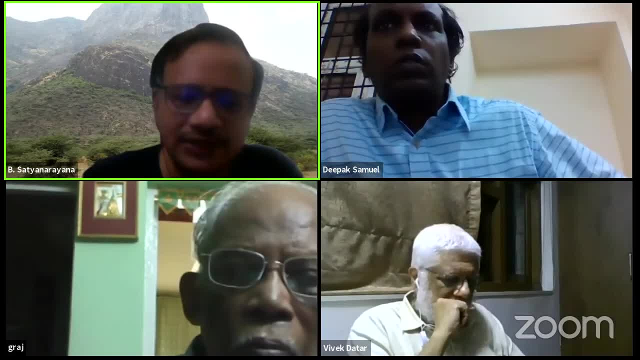 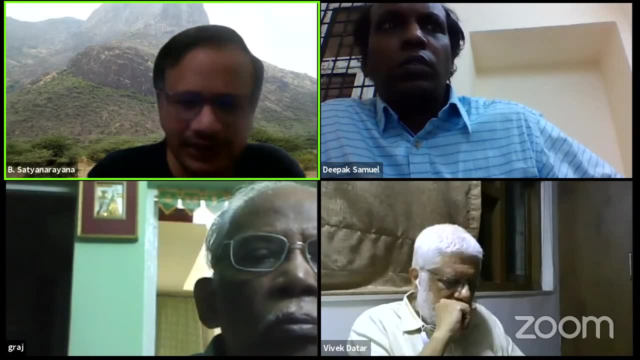 charged particles is uniform and it is always, you know, very clean. so it becomes very important you kind of use them as a flow type. Now, that is just a broad answer, But in this case what becomes important is that when you 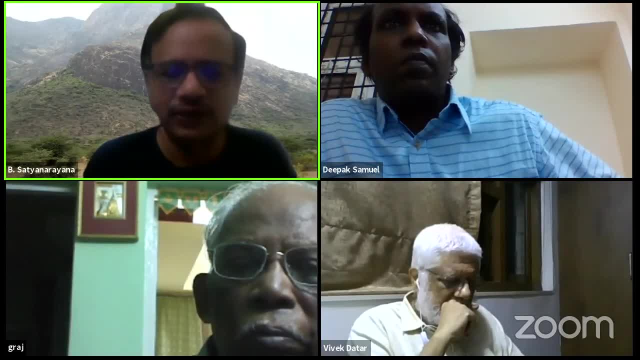 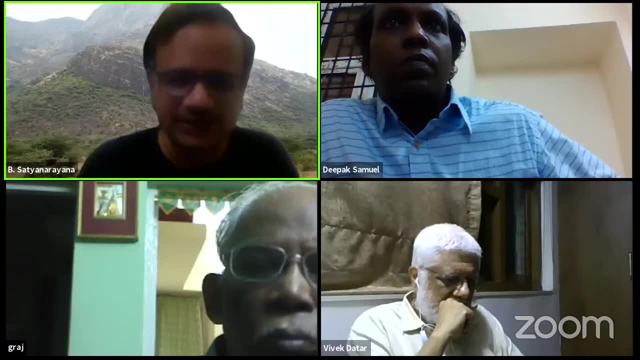 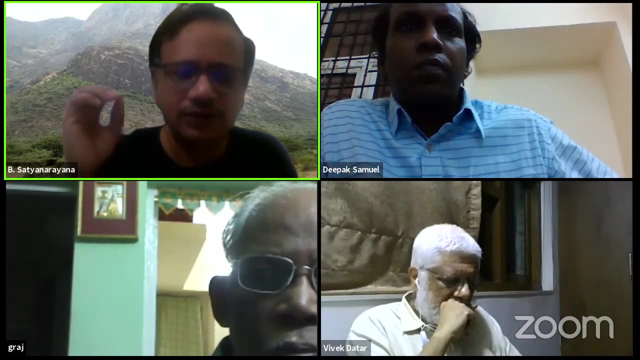 have I told you something like you know, 200,000 liters of gas and literally hundreds of kilometers of actual linear area, linear distances of pressure of gas pipes. if you can look at Now, even if you are, you know, few ppm level kind of even gas tightness, if you can. 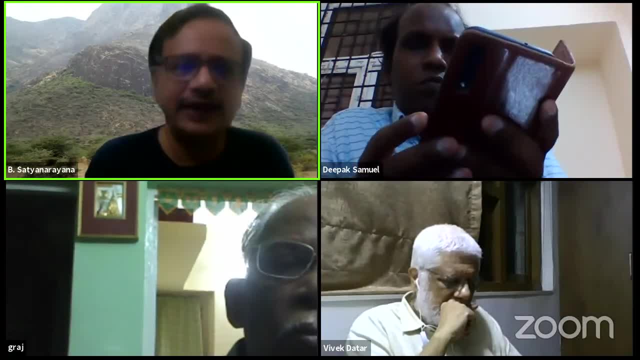 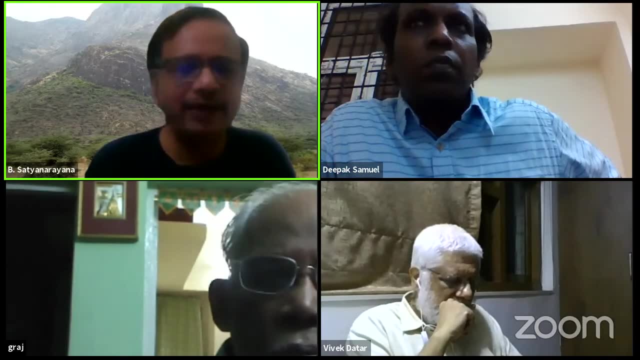 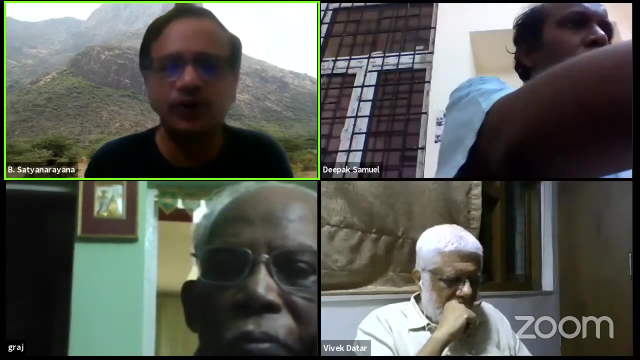 maintain. still, there will be a lot of area where there can be kind of you know the leak possible. Now, the easiest way, I mean you can say I will make zero leak detectors. okay, If you can make zero leak detectors, yes, then there is no need. But it is very, very difficult when you do an 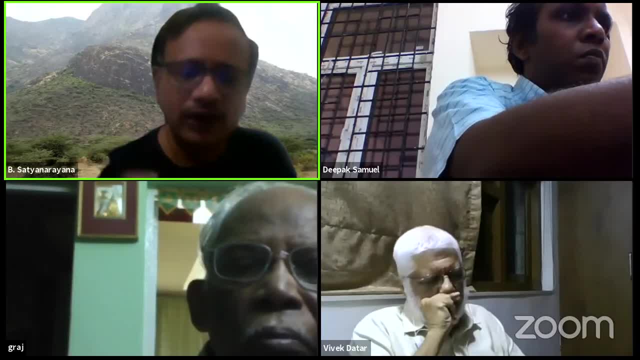 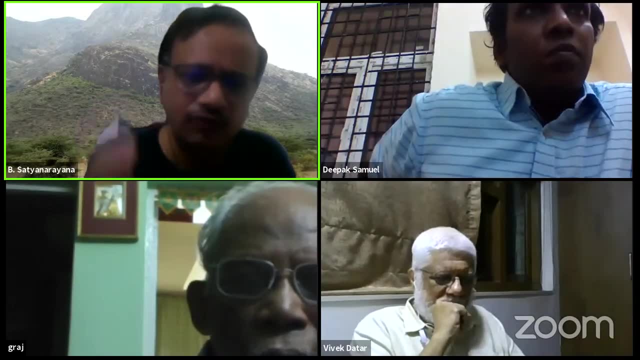 industrial process. So another best way, because you are actually not operating them at a very high pressure. You are operating almost close to the atmospheric pressure. So another simple method is to start flowing with, let us say, a few millimeter water column with a very low flow. 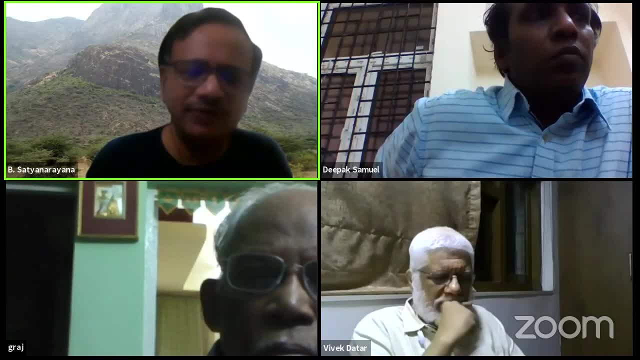 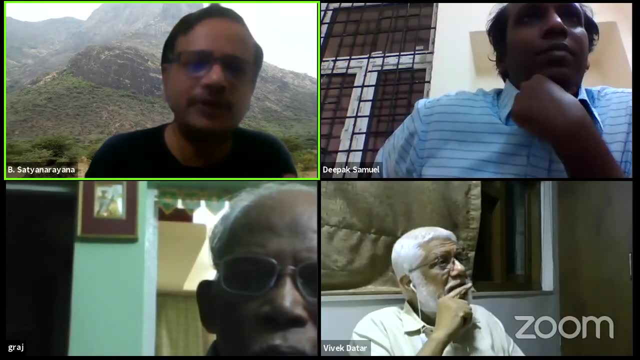 and flush the gas from input to output So that even if there are some small leaks that happened in between, then the gas still is fresh. So therefore, the operation will be better. Now it is important: when you do flow type, you do not want to waste the gas that is coming. 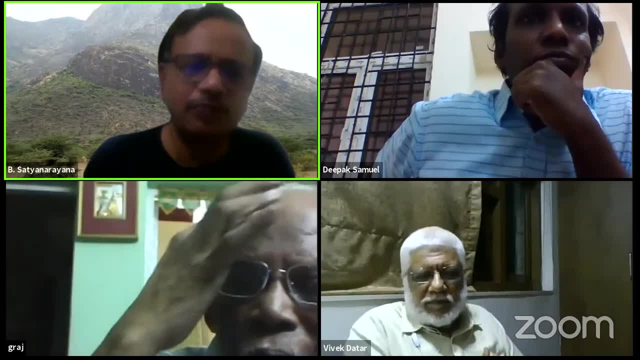 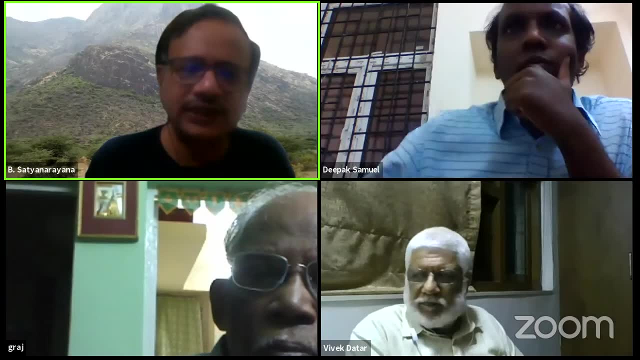 out, as I said. So the best thing is actually take the gas out and actually purify and put that So it becomes important to maintain closed-loop system. So the question that you asked at the end: yes, it becomes more important when you have a larger detector than a small one, I mean. 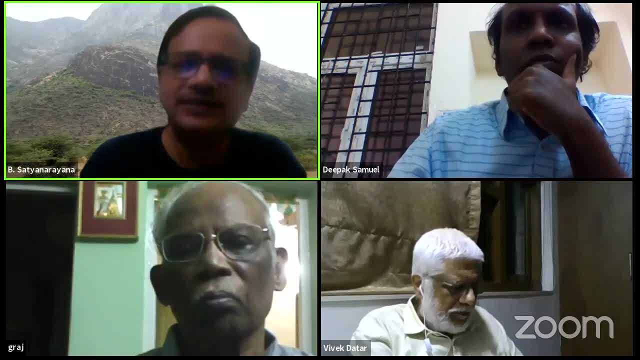 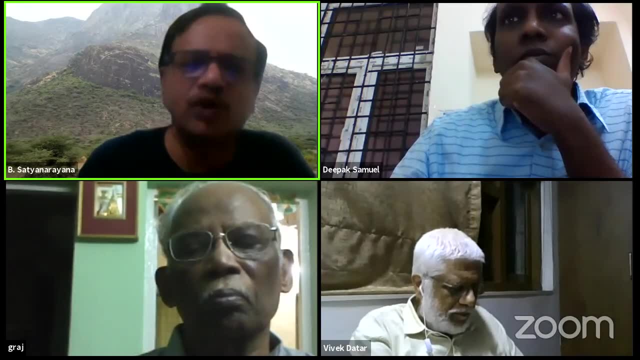 you can make a one centimeter to one centimeter and seal it like mad and you do not have to really do flow type gas. Of course we also did studies about what is the minimum flow of gas that is required per, let us say, unit time. 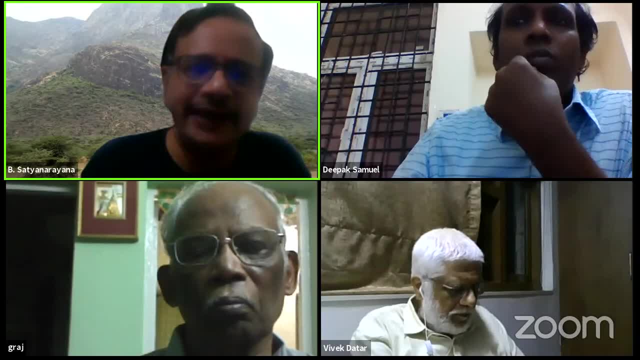 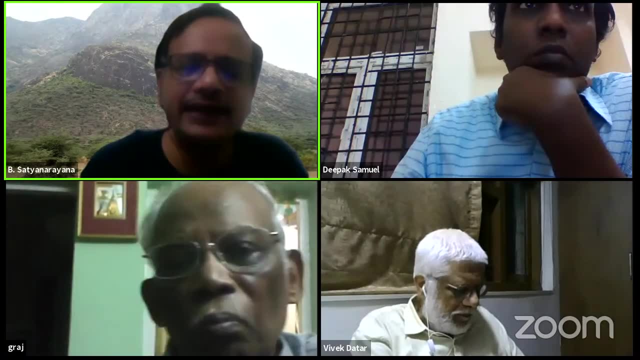 So roughly one volume change per day. That means roughly about eight liters. you know, two meter by two meter by two millimeter is about eight liters of gas. If you do per day it is good enough. We in fact even sealed one. you know some gas RPCs. 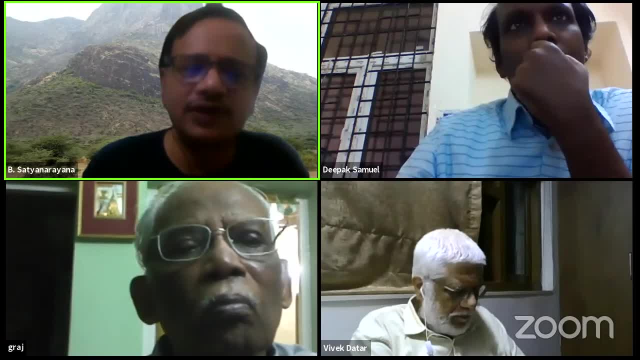 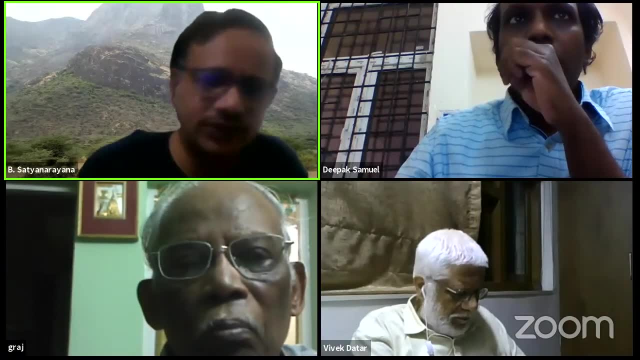 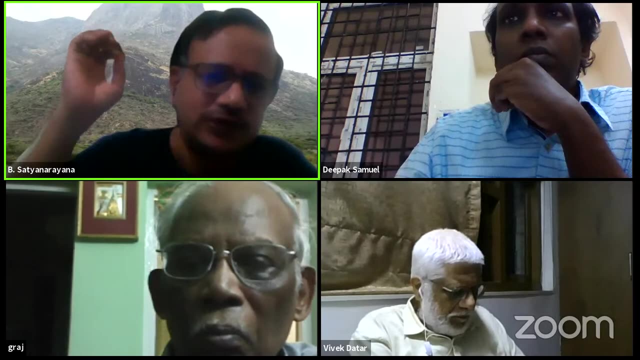 for months together we did not actually find so much of a problem, except that the RPCs had leaks. If there is no leak, then you can actually maintain in the. of course there is a small fraction of radical formation. that happens due to signal formation itself, ionization and avalanche. 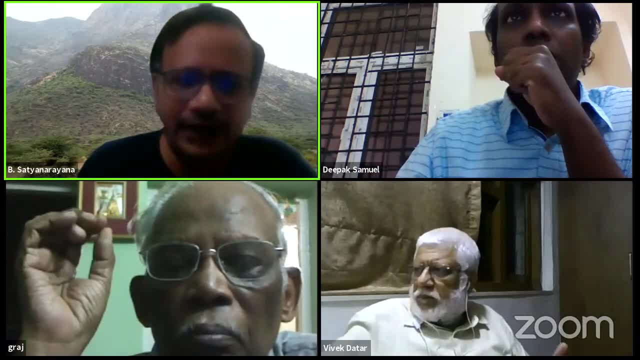 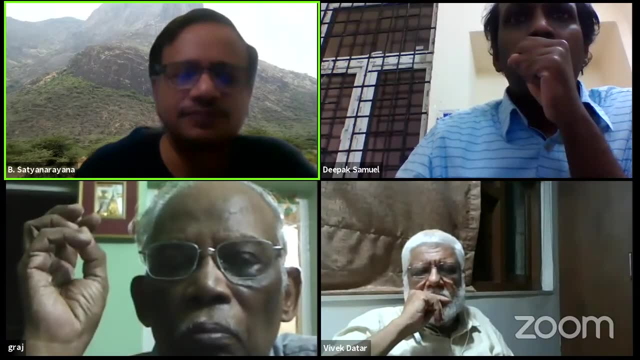 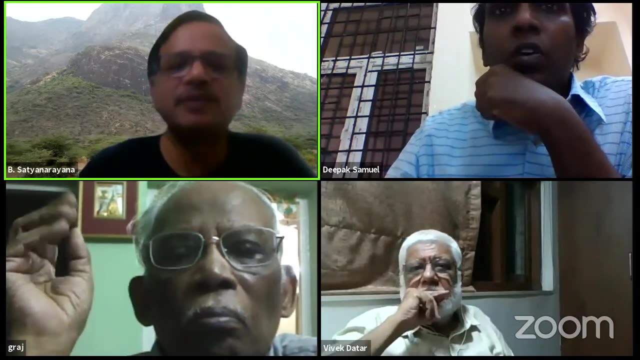 And if you operate them in streamer mode, you have bigger problem of radicals being formed and you need to kind of flush them out. But if you operate in proportional mode, that problem is, you know much less. We can't hear you. Deepak, Deepak, we can't hear you. 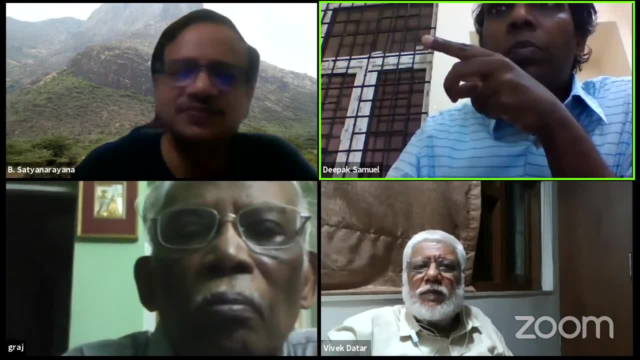 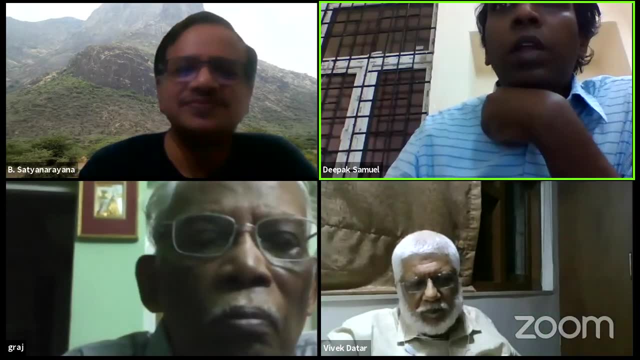 Now, Yes, Now we can hear you. Okay. So one more question from the same person. So he has asked, in the animation of iCal construction, if we need to repair any part typically, do we need to disassemble all the? 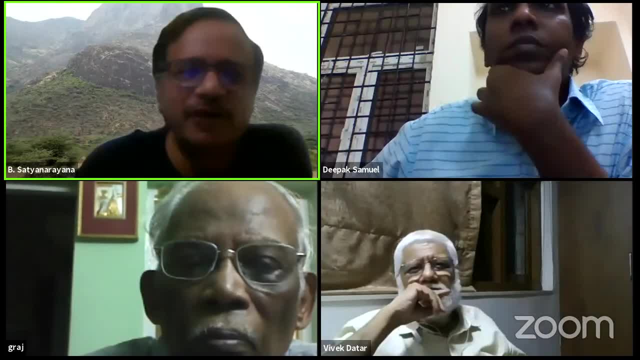 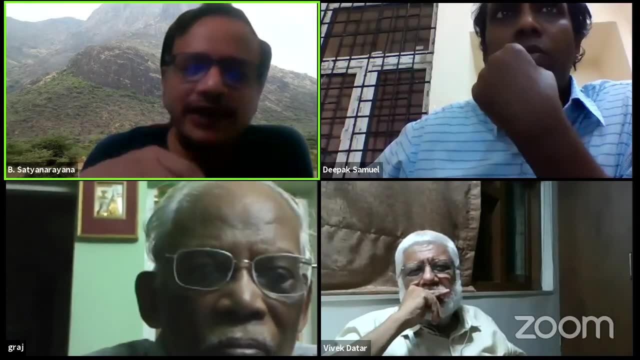 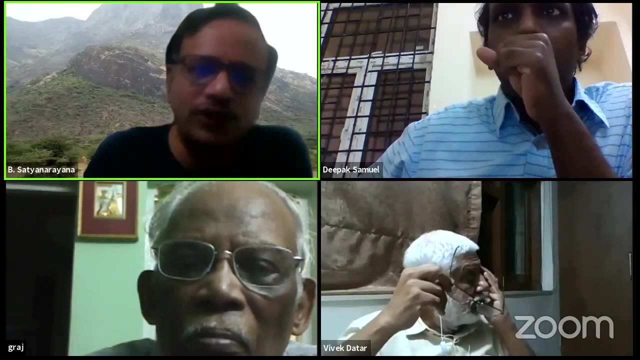 Yeah, So this anyway is Murphy's law. So I didn't go into that detector construction, I just went very quickly. One module is, let us say, eight roads. You know, roads are just in parallel lines Into each road. 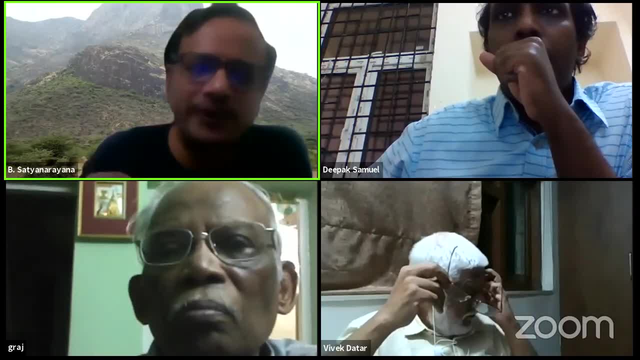 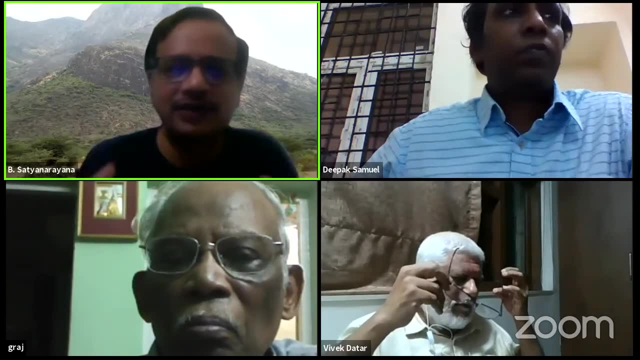 you push. each road is 16 meters, So two meter is one. two meter by two meter is a RPC, So you can push eight RPCs in one. The way we do it is, if you remember that drawing that I gave- 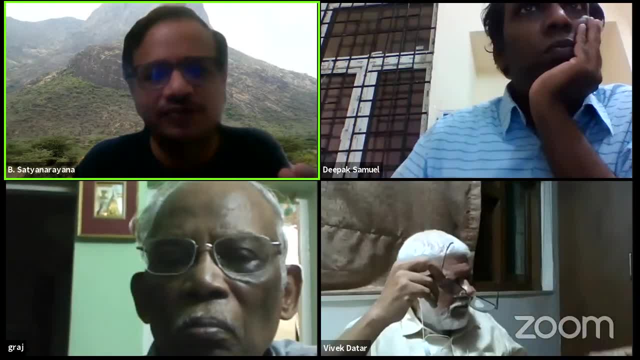 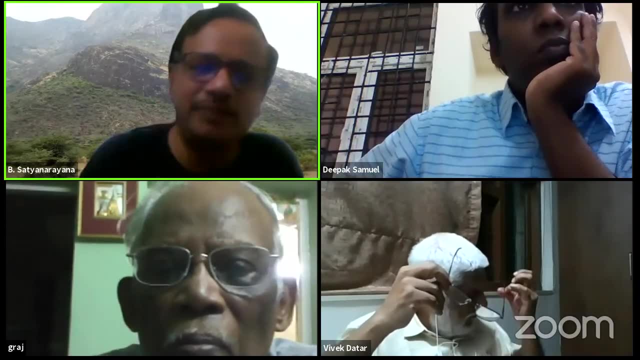 there are trolleys on left side and right side. You push four RPCs on one side, four on the other side. Now why I said Murphy's law is it is possible that third, the deepest one inside, might go bad. So out of 30,000, if you see even one percent of them, 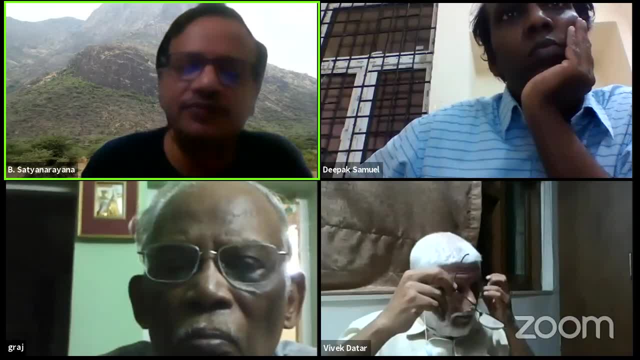 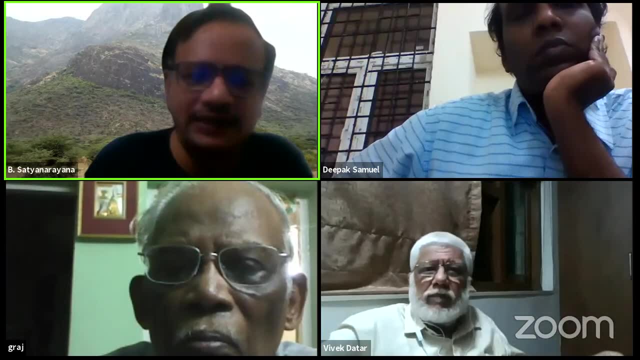 goes bad. it is a big task. Normally what we do is if the RPCs are having some minor problems, we live with them for some time. We don't go and replace that. each small problem, one gap, one channel, two channels, etc. 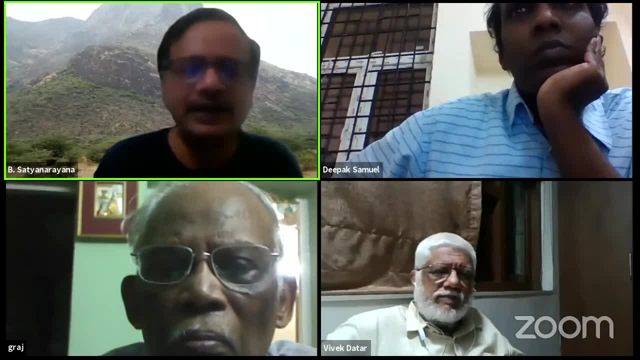 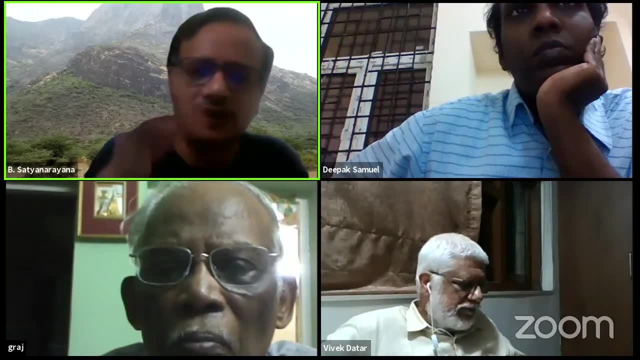 But if an entire RPC goes bad because of, let us say, high voltage is bad or something else, the electronics is bad. obviously we have to take it out. So the way you take it out, if you see those trolleys which are going and you saw in the animation, so you have to pull them out. Three of 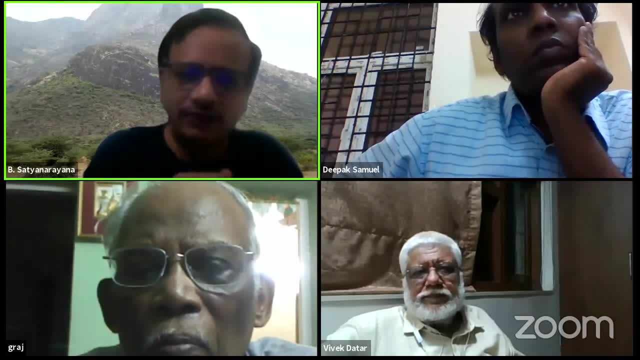 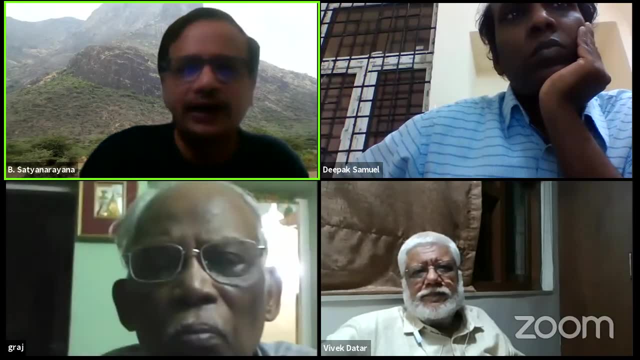 them. you have to pull them out, stack it in the trolley, take a good one, of course, along with that. So push that one and then bring the faulty one down and repair it down. You cannot repair anything 15 meters high, So you have to push that one and then bring the faulty one down and repair it down. You cannot repair anything 15 meters high. 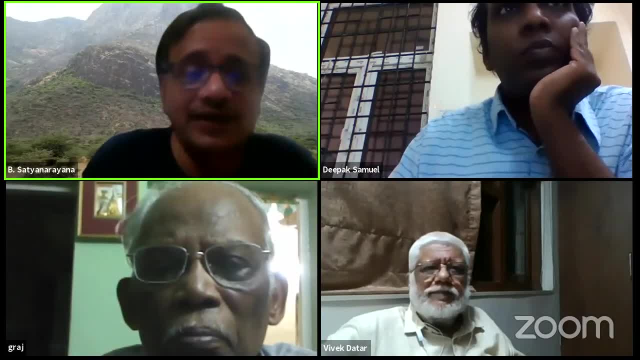 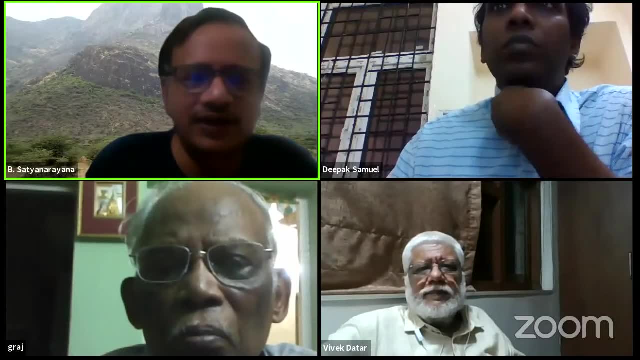 So unfortunately it is. yes, it is a painful thing, by the way, But this is how all energy physicists around the world work. There is no shortcut. If it is only at the tabletop experiment, then you can do repairs easily or you can send to the manufacturer. 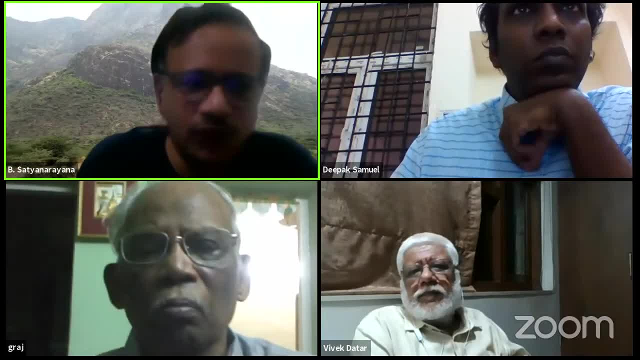 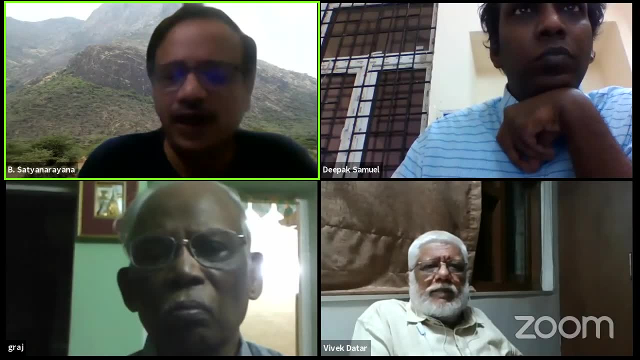 they will repair and give you. But in high energy physics experiments you have to repair yourself. That's why the students and everybody should know what the detector is, what electronics is, how they work, how they don't. Many of our students 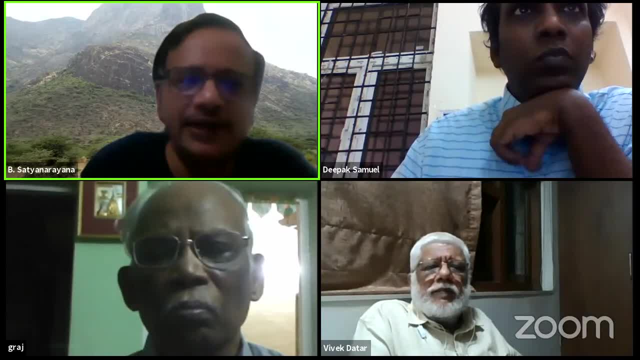 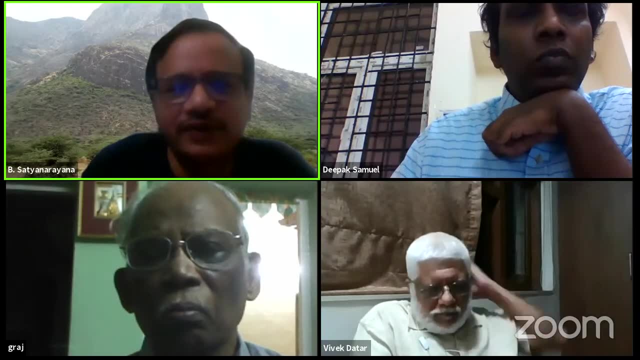 actually, they spend all the time looking at data and to tell you where are all things going bad. Even with that tiny detector, I showed you- we learnt a lot of it- how to operate it in a long term way. One more question from you two, from the same person. The question is: 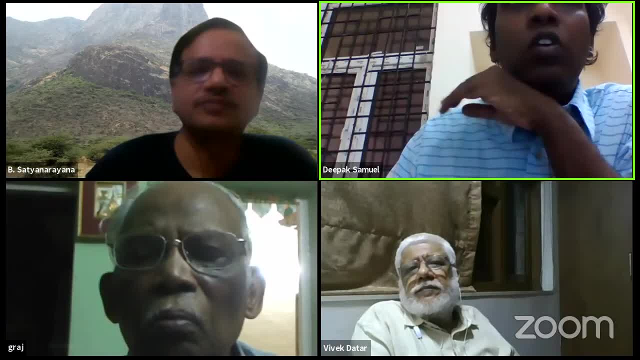 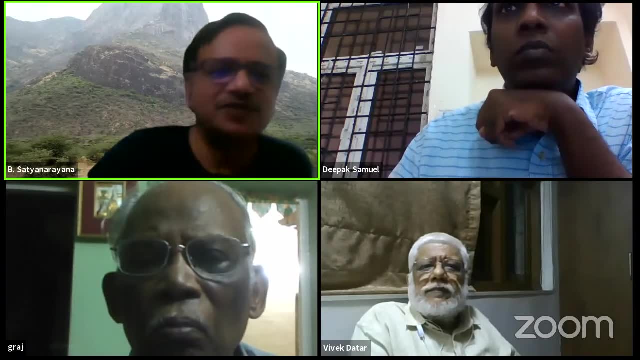 can we replace RPCs with plastic scintillators and silicon photomultipliers? Okay, By the way, I hope these are not all I&O students. So for I&O students, you can wait till the little end. I will tell you that I&O students are not all I&O students, So for I&O students, you can wait till the little end. 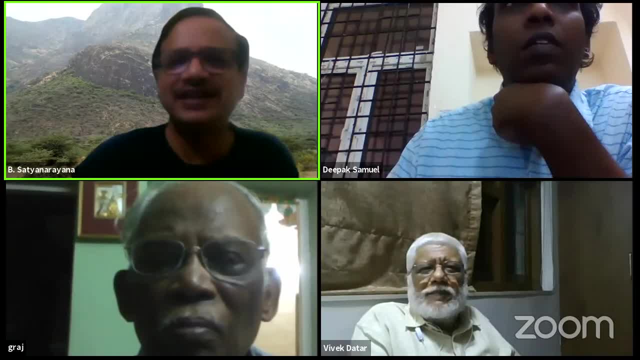 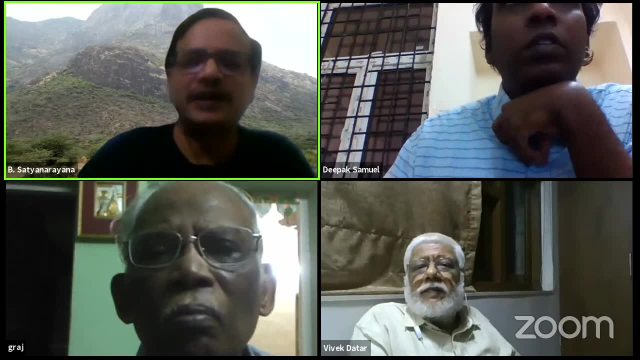 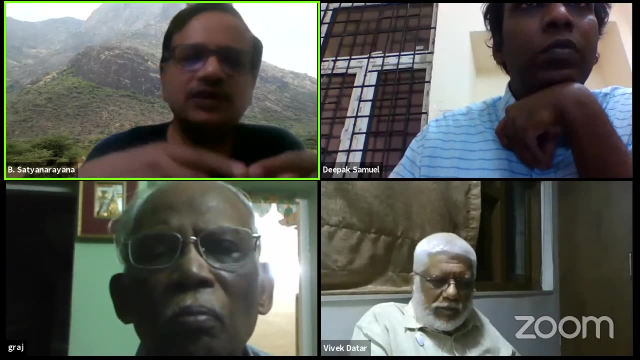 You can take maybe the other students. Okay, Nevertheless, I will go ahead. Who is this? Who asked this question? Okay, It doesn't matter, Sadashiv Sahu, Sadashiv Sahu. Okay, Yes, in principle you are right, Sadashiv. It's a planar detector. 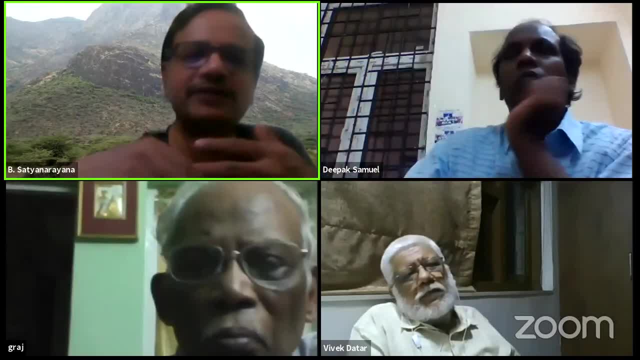 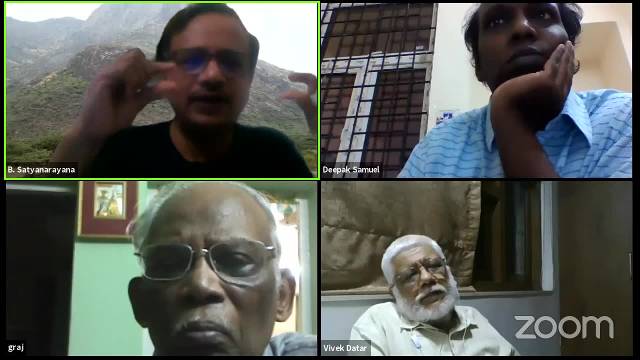 When we went for this baseline design of RPC at that time, all we needed is tile-like detectors so that you can insert them. That is the most important thing And also it's important. I rushed through that, but it's also important if it is thin enough. 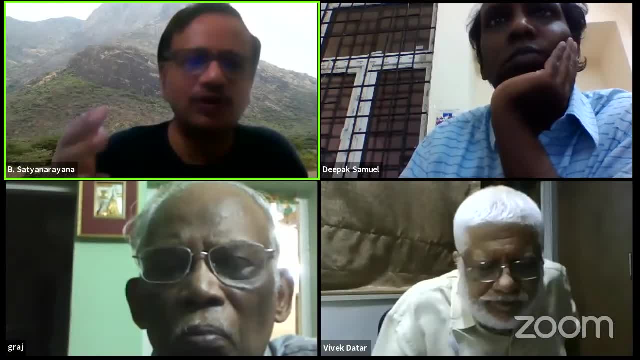 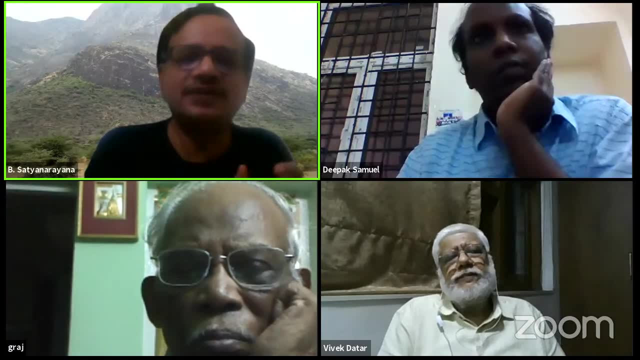 so that then you occupy less space, You can fill it up with more iron. Okay, Now if you want to compare, for example, there are problems with RPCs. One of the biggest problems is, of course, you have to flow gas, So that issue is there, And similarly, you have to generate high voltage. 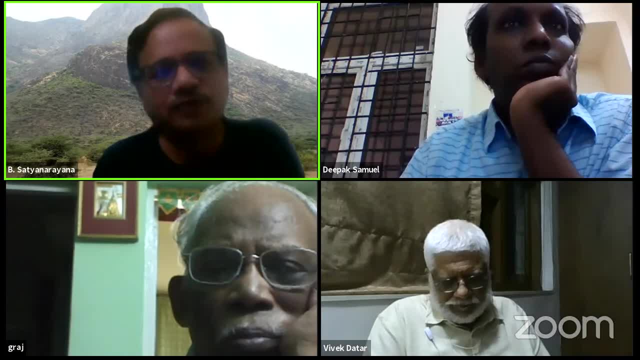 locally and so on and so forth. Now that problem won't be there for scintillators. Scintillators: once you push inside, put a fiber inside, etc. they stay there. They don't require any gas or anything. 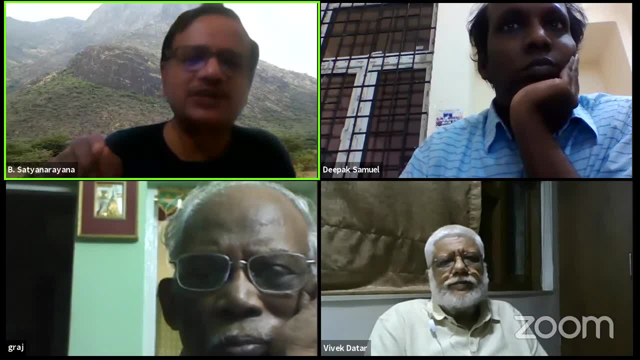 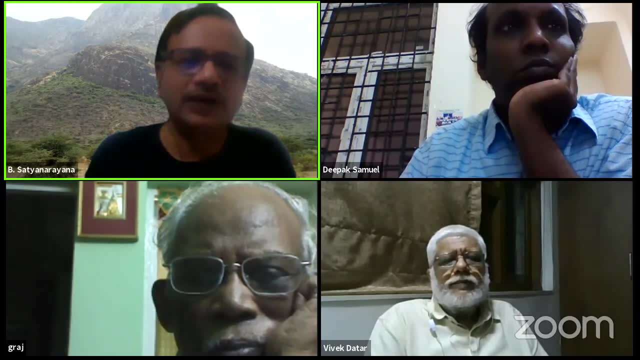 no high voltage and so on and so forth. The silicon photomultipliers were not existing when the iron was thought about it. They of course become reality much later, But even now they're okay. They have become very cheap, But it's not that. if you want something like 4 million, 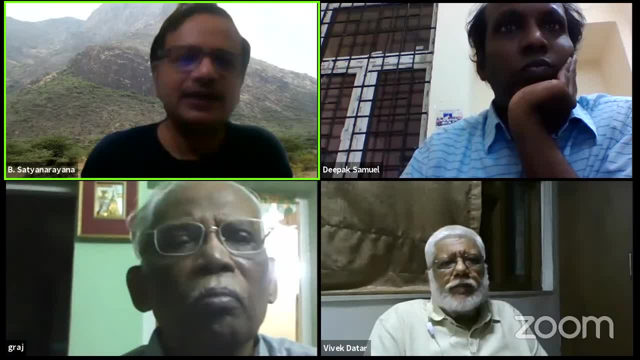 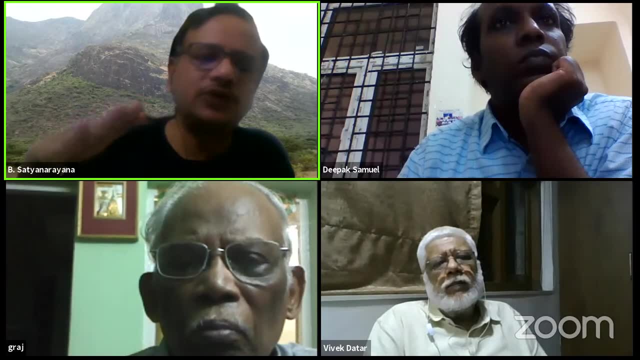 silicon, pms, etc. they're reasonably costly. And also remember that you need to do segmentation. Now, if you look at scintillators, you want to do x and y segmentation for it to get x and y channels right. 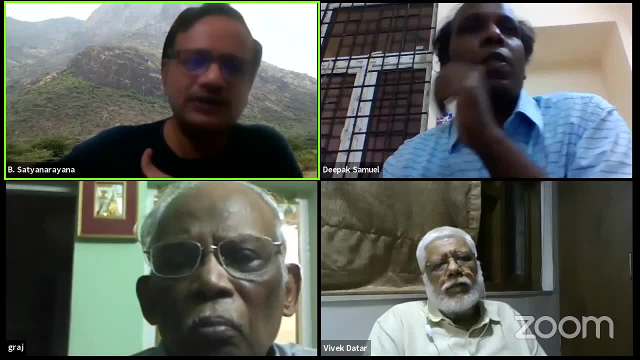 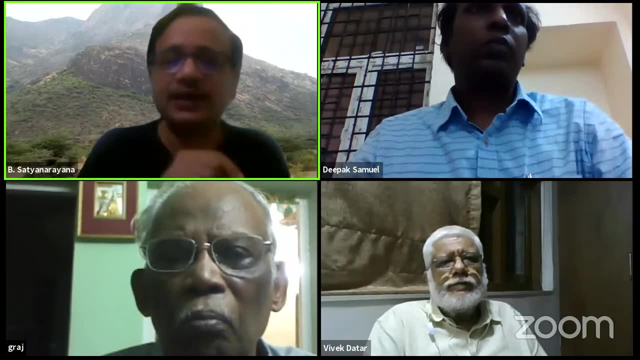 We remember how the RPC is. So you have 64 segment channels on one side, 64 on the x side. So you also have to design the scintillator in such a way that it actually does it has a segmented scintillator. Of course you can use like strips, packed together. You can. 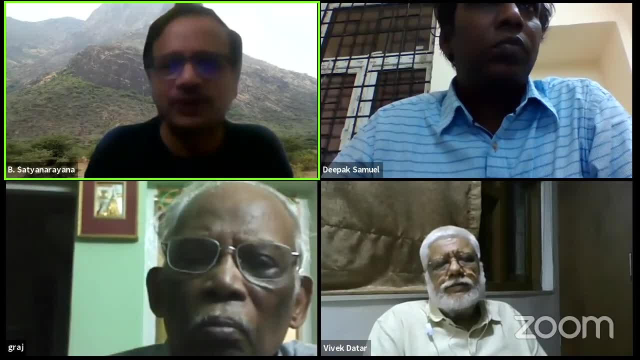 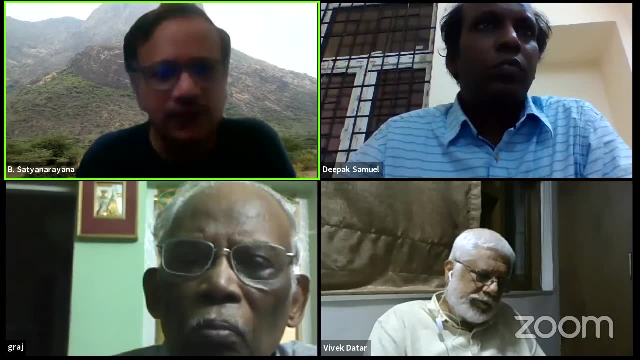 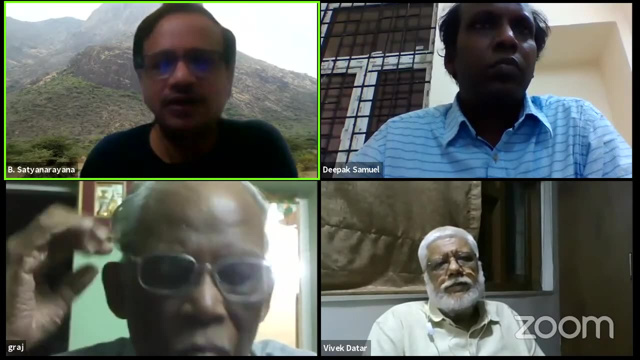 also do vertical isolation and then make them optically separate. There are techniques to do In principle. yes, In principle. you can use scintillation tiles or extruded scintillators, read by wavelength shifting fibers. At the end of this one you use silicon pms. it is possible, But 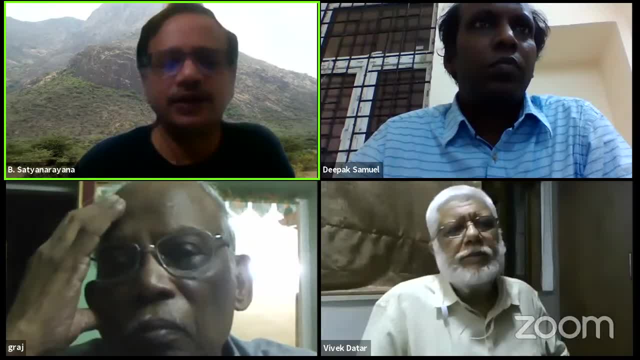 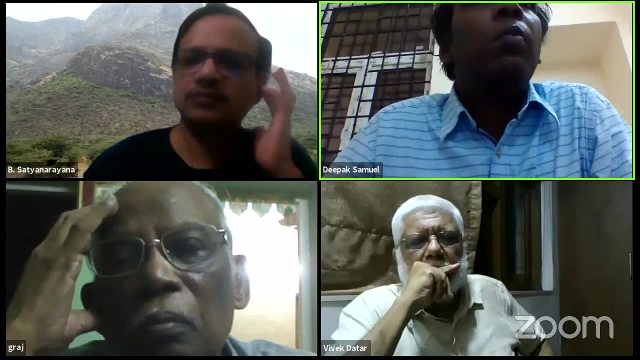 just at an extent, one has to also look at cost and things like that. the benefits. Yeah, that's right, All right. So now we take a question from zoom Bala Subramanian, So I will, Yeah. 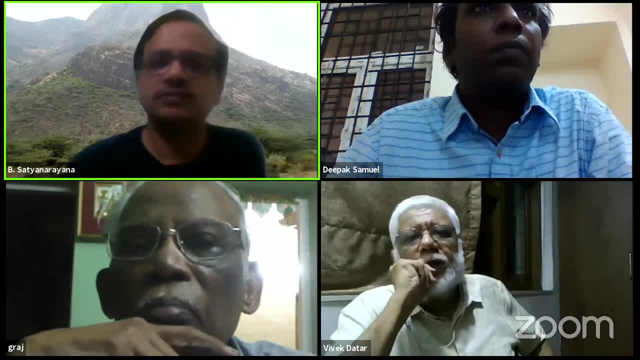 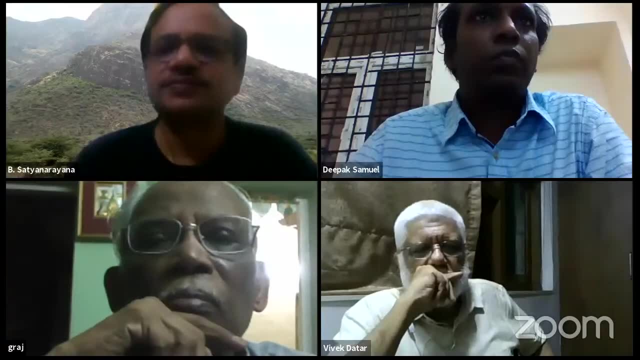 Bala Subramanian, I will answer this one. Yeah, Bala Subramanian, I will answer this one. Yeah, Bala Subramanian, I will answer this one. Hi, good evening everyone. So why is this 1.3 Tesla magnetic field? Is there any characteristic? 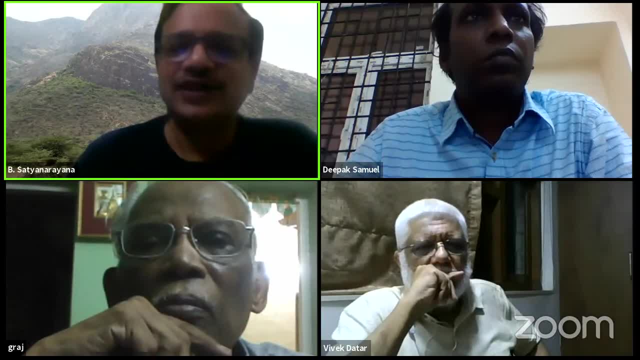 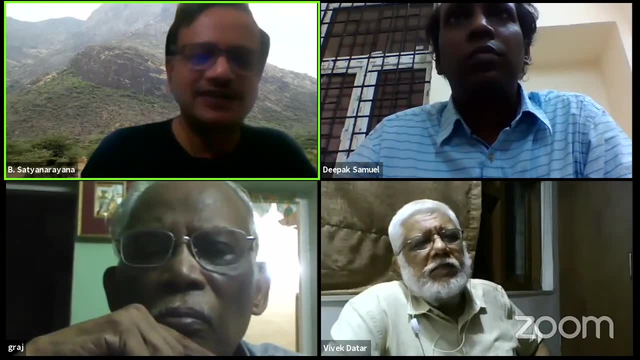 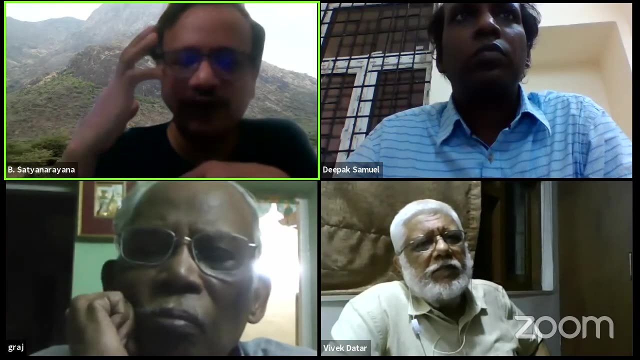 reason behind that. Okay, actually the expert on this is actually in the audience, But maybe I will just start, and maybe Professor Raddathar can add. I mean, what is the magnetic field? that requires? to certain extent, is depends on what is the physics that you are looking at, right? So, ideally, 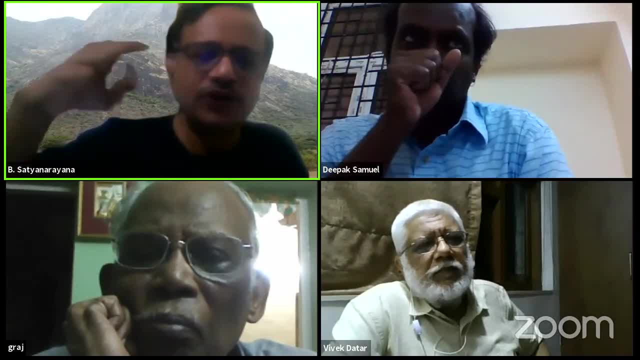 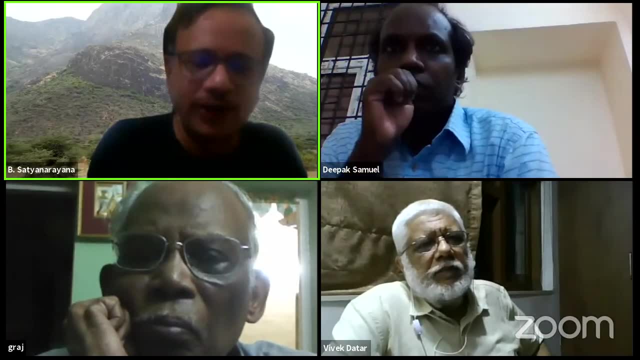 you are going to kind of do. what are you going to do? You are actually going to have iron plates, you are going to magnetize them and you are going to look at the x- y coordinates of the track as they are going Now, depending on the momentum of the particle that you are. 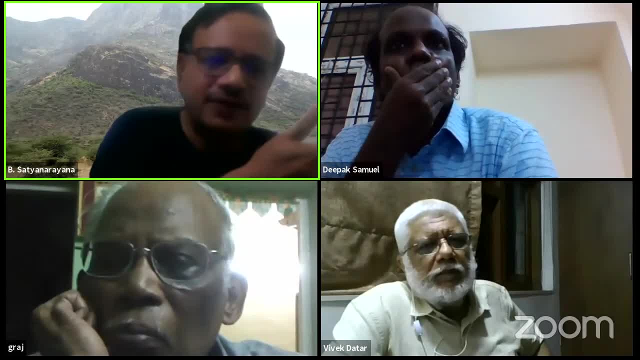 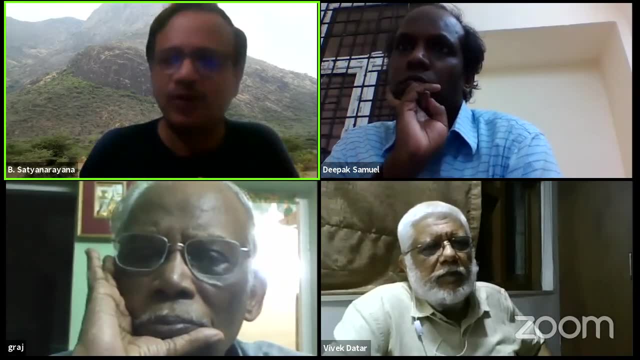 looking at, either you will have a, you know, very curved kind of a track, or maybe you know the radius of curvature. what I mean could be larger, could be smaller, basically based on the moment of the particle: a higher or lower? 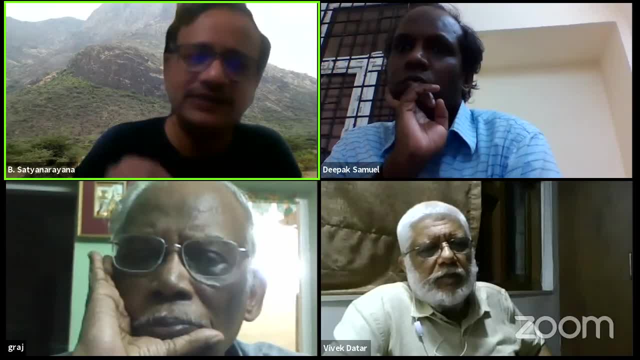 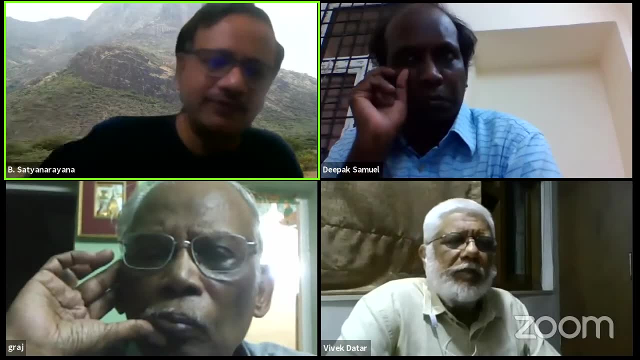 Okay, so now there are some problems you will start facing. It is very nice to track particles which are going, cosmic muons which are going without magnetic field, But when you start having magnetic field, when the when it starts kind of bending, it is possible that your 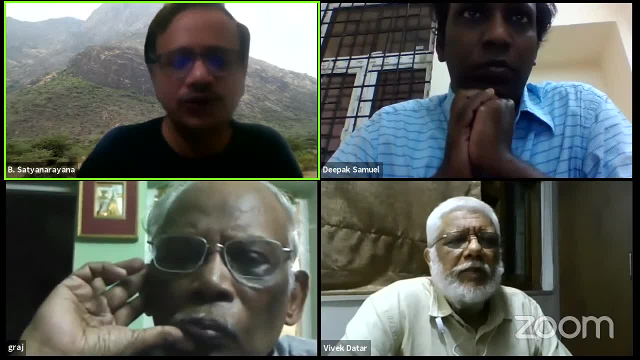 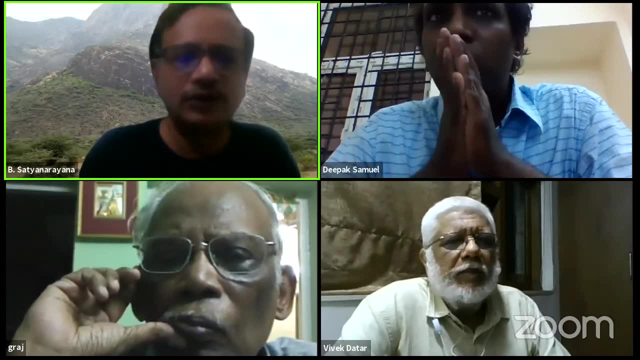 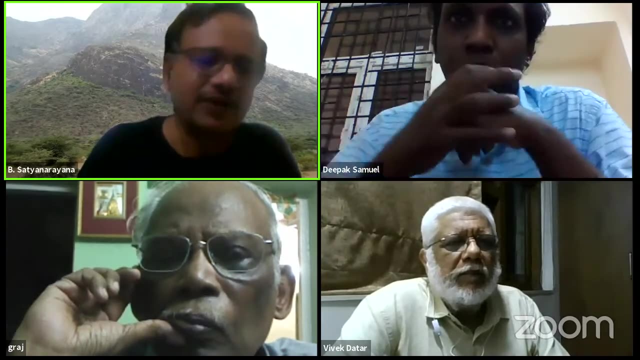 position resolutions are not as good as you, as you wanted to see. Of course you can also use timing information that I talked about also to improve to some extent. You know the the reconstruction efficiency. okay, But if I can have larger magnetic field, 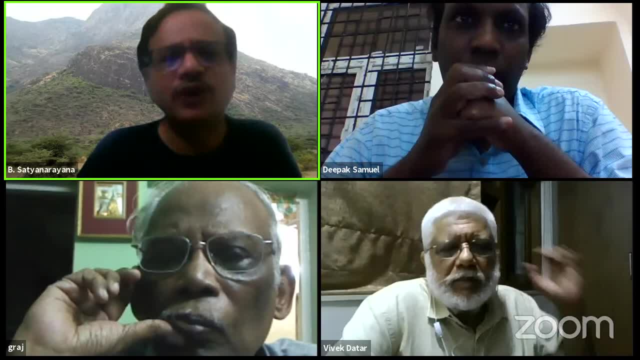 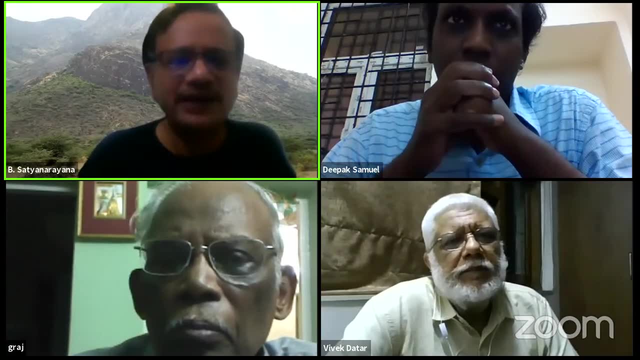 probably I will have another handle on this, or So what? what is the point? I mean I can, so can I have four Tesla magnetic field? I can three Tesla magnetic field now, but it also makes things bulky. it makes operation, because this is a conventional magnet. This 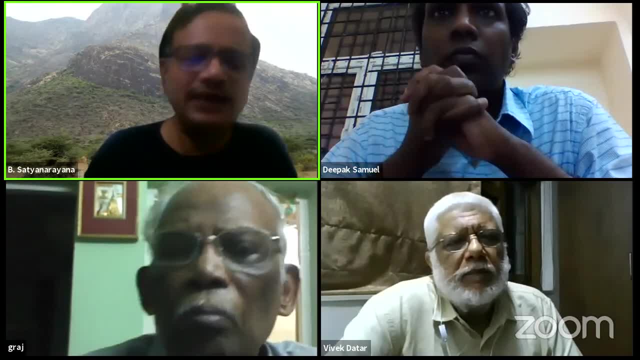 is not a superconducting magnet. So things become very bulky and very difficult to operate if you go to very high. So you would like to kind of have roughly the. the range of the magnetic field should not be much bigger than 5.. 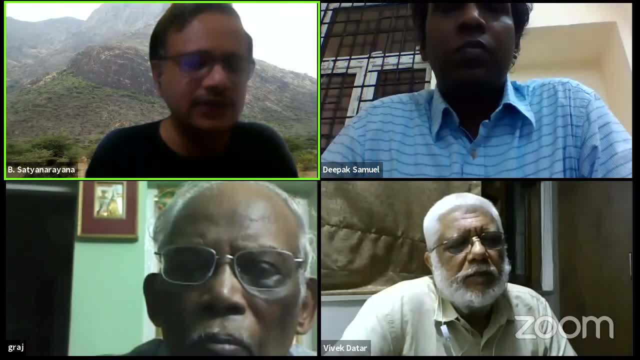 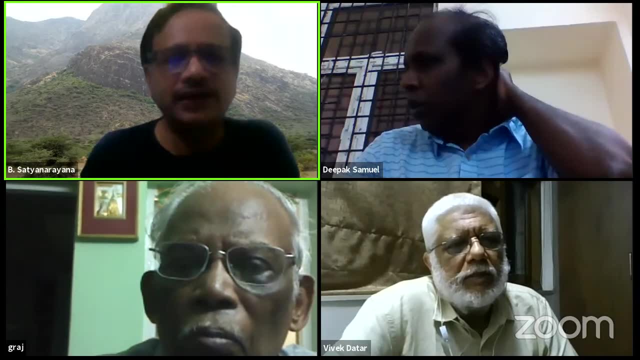 Okay, The rule of- I mean the basic specification that worked about, it is from the physics studies- is about 90% of the detector volume. you would like to have a magnetic field which is, let us say, a Tesla and above. 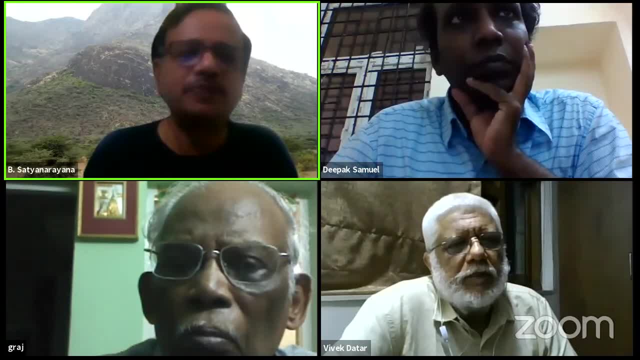 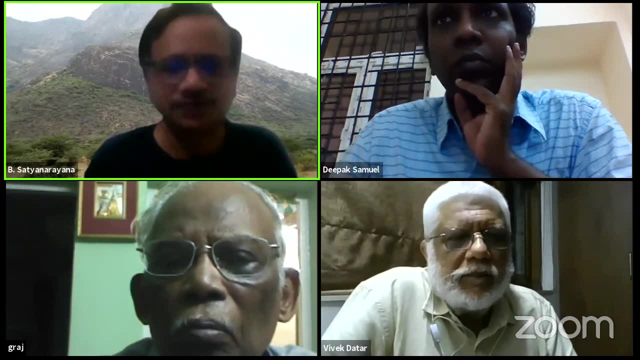 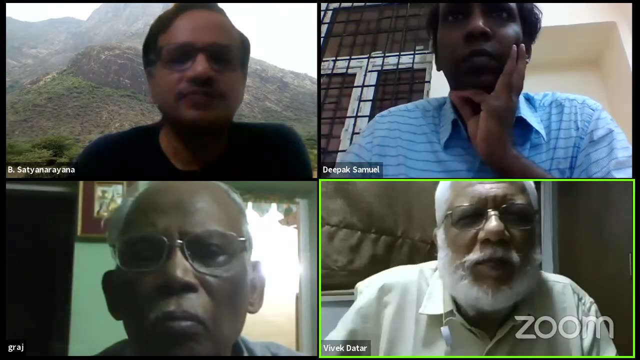 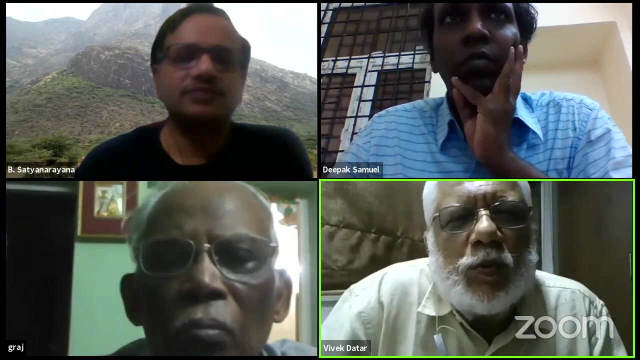 So with that kind of a picture is the whole system is being designed. But, as I said, I would like to take some opinion from Prasiddhata on this. I think, yeah, you have basically answered the question. So ideally we would like to have as high a field as possible so as to measure the momentum. 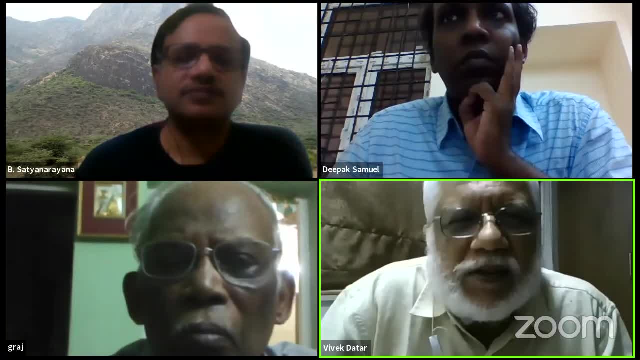 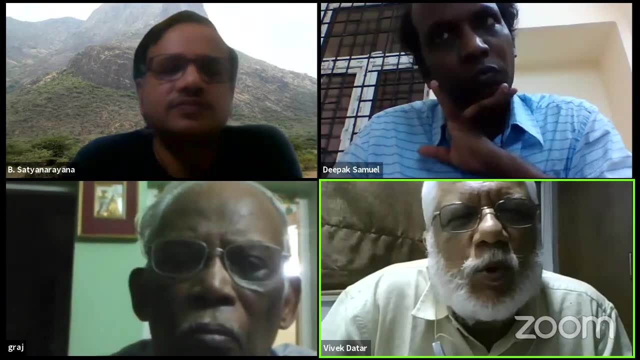 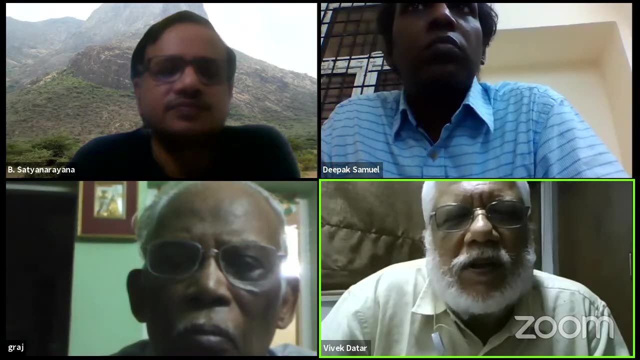 accurately actually momentum by charge, mu plus and mu minus. But on the other hand iron saturates at about two Tesla And of course if you have such big, you know iron plates manufactured in industry, they saturate. I mean they start bending over. So you have a B versus H curve which starts bending over at already, at about 1.4, 1.5 Tesla. Now, if you want to go to 1.6 Tesla, let us say, then you might require 20 or 30% more. current, because this is an electromagnet, So the power requirement will go up by 60%, and so on. If you want another, you know 1.7 Tesla, it becomes even more expensive. So this average, or the over 90% area, as you said, a field of the order of 1.3, 1.4 Tesla, seems to be adequate. In fact the simulation people at the time we were designing this said that even a 1 Tesla field is OK. So 1.4 Tesla seems to be a reasonable number, And we can get that with the low carbon steel that is manufactured in the country rather easily. 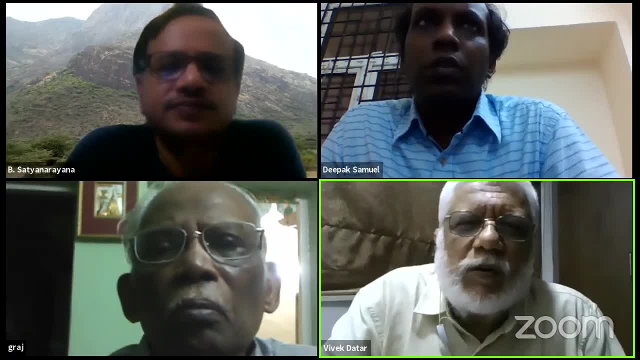 Easily, So that I mean one can go really at you know some BHT level, So that I mean one can go really at some BHT level, So that I mean one can go really at some BHT. 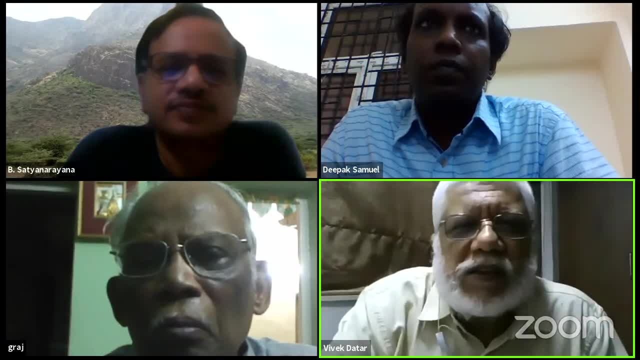 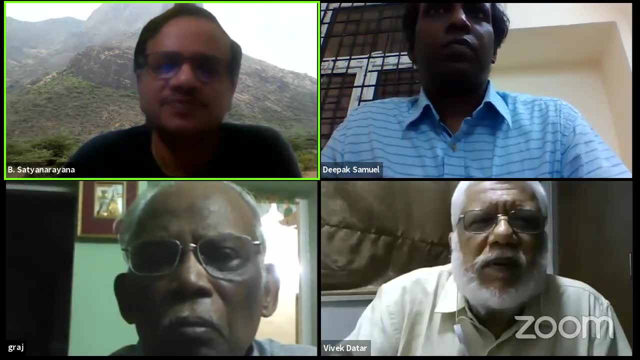 which is extremely sharp and it starts bending over at 1.8 Tesla. But then that iron is extremely expensive- It's about, I think, three or four times as expensive- And also difficult to handle. Yeah, So we have to also look at practical consideration. 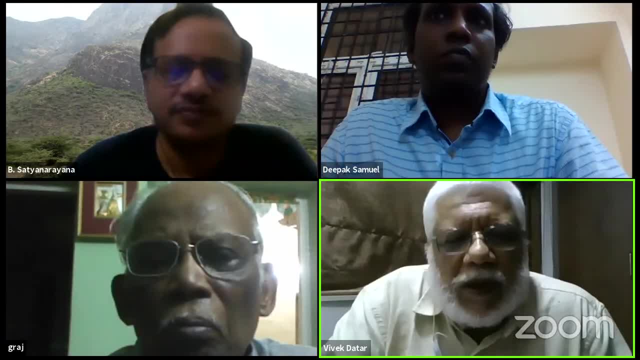 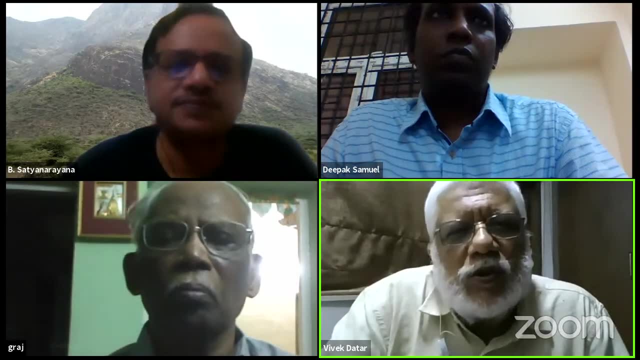 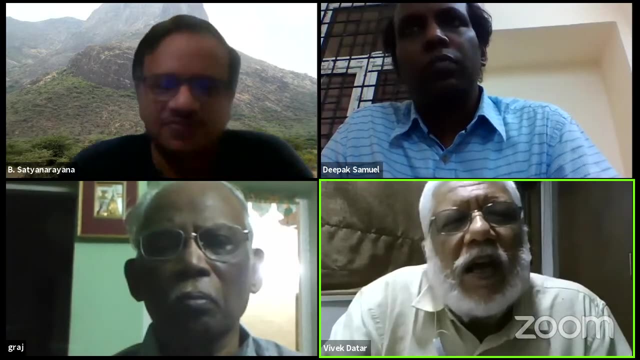 We have to keep cost within reasonable bounds, But at the same time we have to get the detector to perform as we want it to. So this is a. In experimental situations it's always a compromise, And this seems to be a reasonable compromise. I think I might also want to comment on the 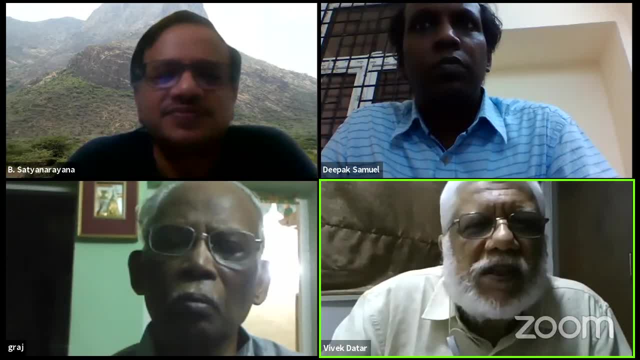 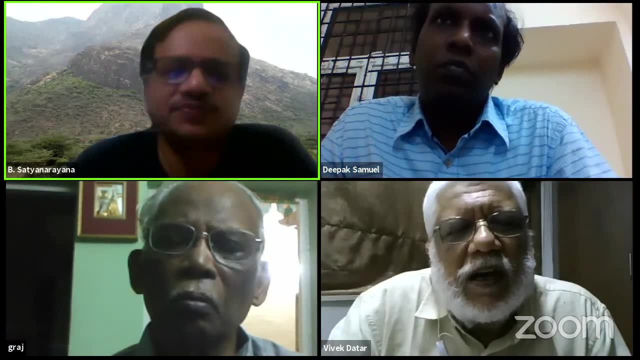 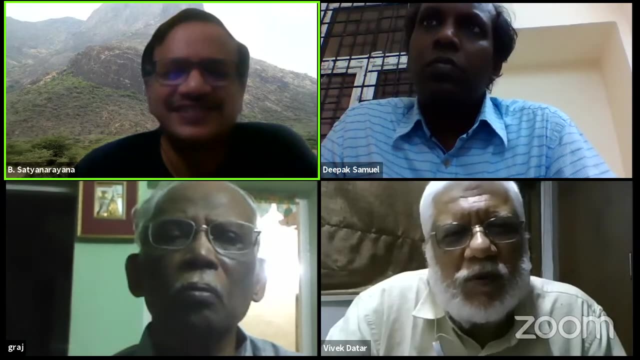 plastic versus RPC. So at the time that we started the plastic detector was about three times as more expensive, And already the RPCs contribute a reasonable fraction of the total cost. So three times more expensive would have been No SIPMs at that time. 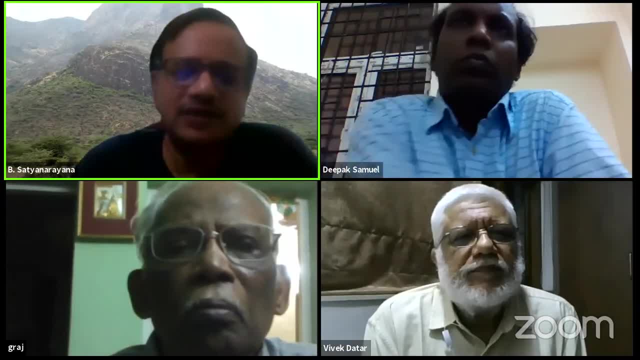 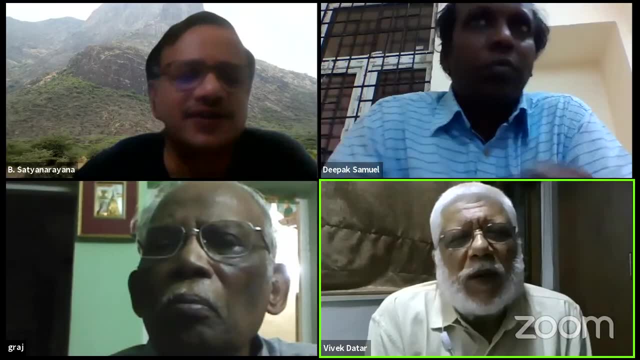 Yeah, So you had problem in terms of you know I mean segmentation and you know read, and each tube was a few hundred dollars. So with the price you have to pay with the glass RPC that it's a little more difficult. 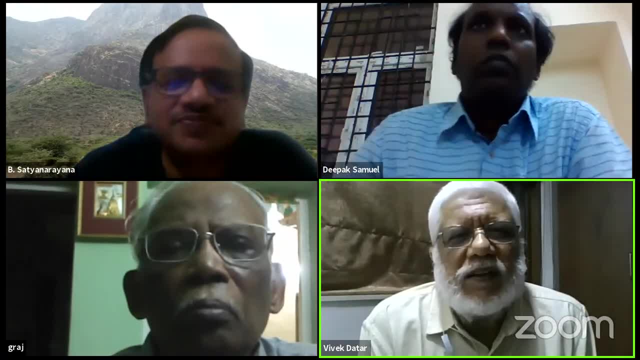 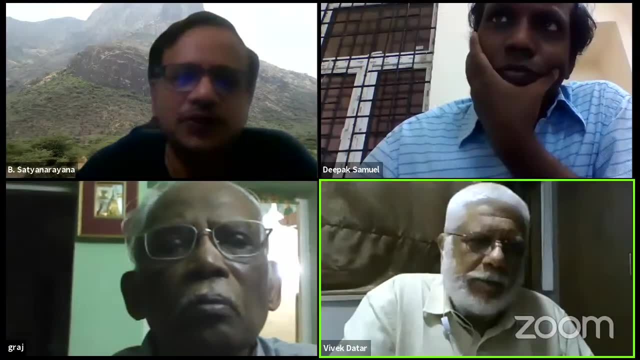 to handle. But if you- I mean, we have learned the techniques on a small scale, we will have to do this on a larger scale. Also, operational cost: operational cost and then the fact that you have to flow the gas, and somebody asked this question about 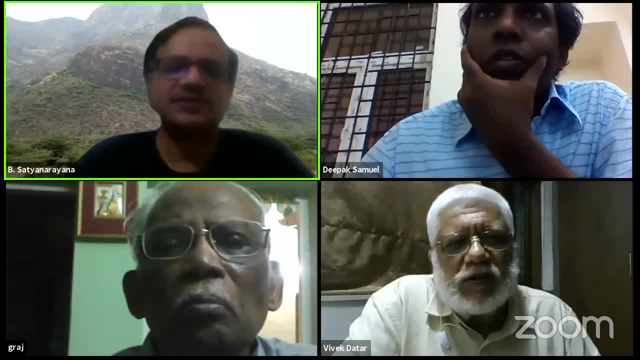 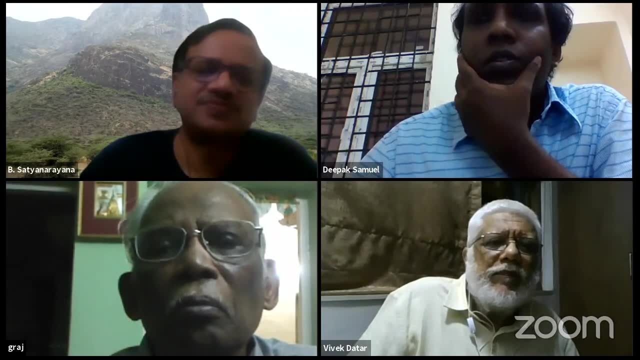 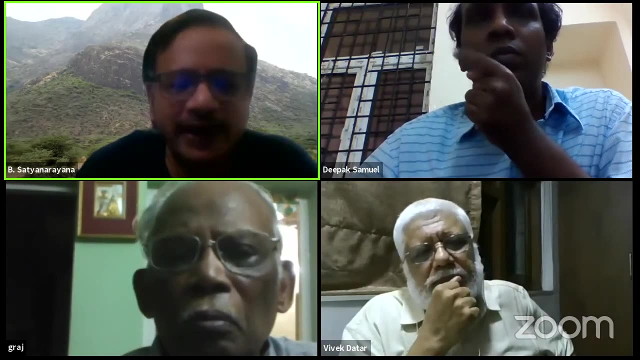 The running cost versus capital cost. Yes, Thank you, sir. Hello, I have one more question. With the data collection, are you going to, I mean, have a grid computer or See? sorry, I because lack of time, I couldn't spend much time on the backend side. No, we. 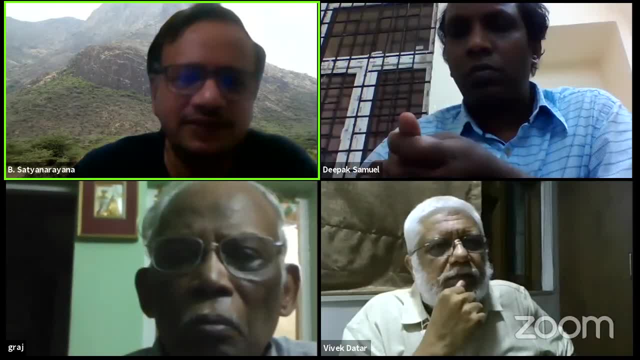 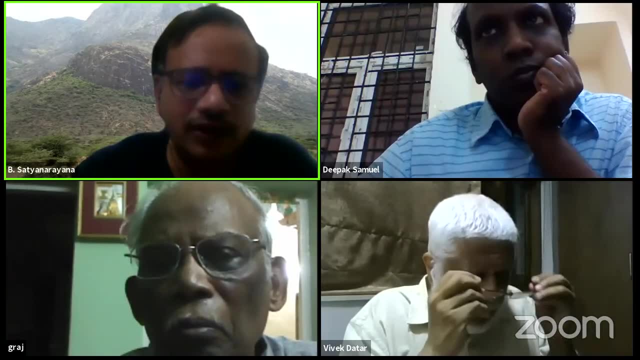 don't have to go to cloud computing. Unlike the petabytes of data that the LHC pours in, the data that comes from here, as you could somewhat imagine, is very small. For example, you are only recording, realistically speaking, the data that comes from here, So the data 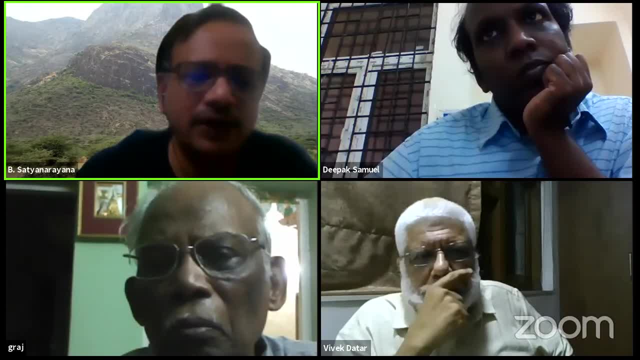 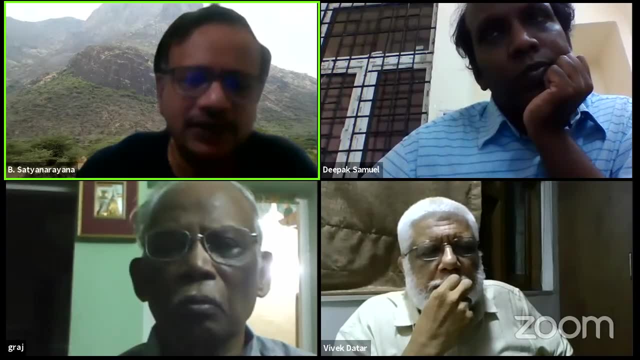 that comes from here, as you could somewhat imagine, is very small. For example, you are only recording, realistically speaking, just one bit per strip, So you have 64 plus 64, so 128 bits, right? Maximum, That is for the position, information And, let us say, take. 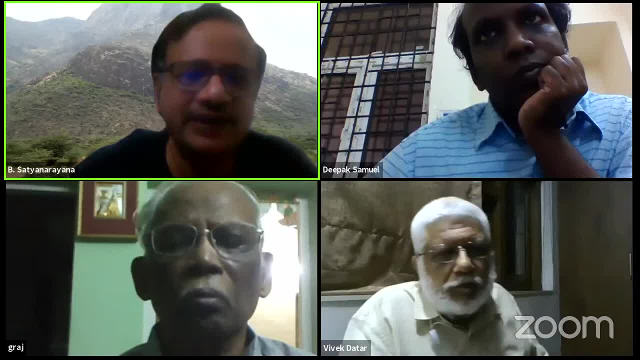 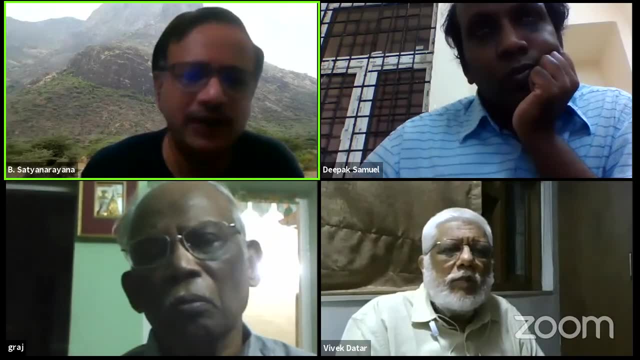 another 24 bits or 32 bits even for the time EDC. But if you look at the so-called occupancy means typically, out of your 3 million channels, how many channels are going to fire by simple cosmic muons or muons produced neutrino interaction? 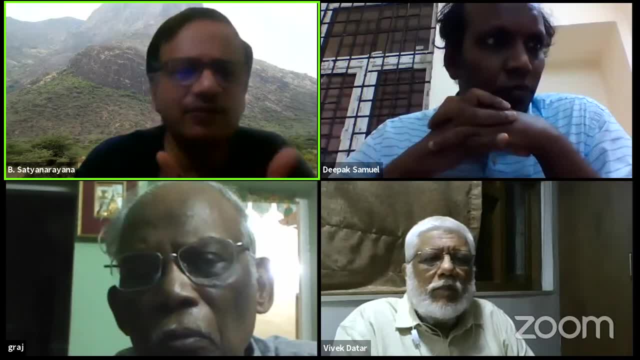 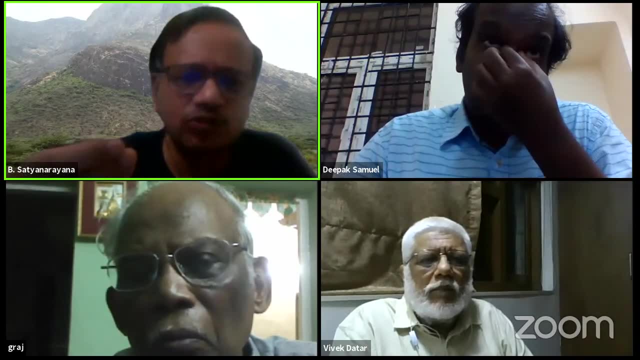 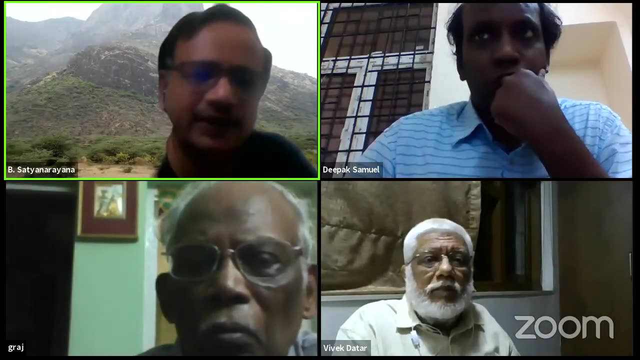 Yes, Or even showers. okay, That will be very, very small. So I can assure you, out of 30,000 RPCs which are manning your detector, a small, maybe a few percent of them are actually going to have data fired. Now, once a RPC is fired, the total package of data is only about 600. 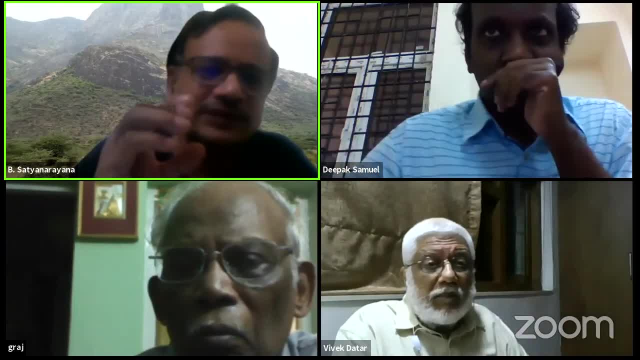 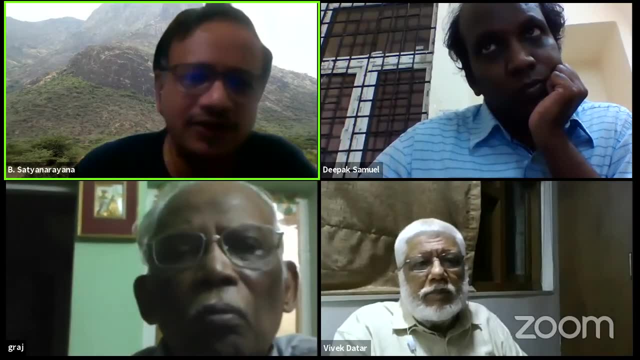 bytes And believe me, out of the 600 bytes, most of them is actually header. You know I mean very little actual data. So the data that comes out, you know can be, you know can be recorded very easily. But again, you look at what is this trigger rate that you 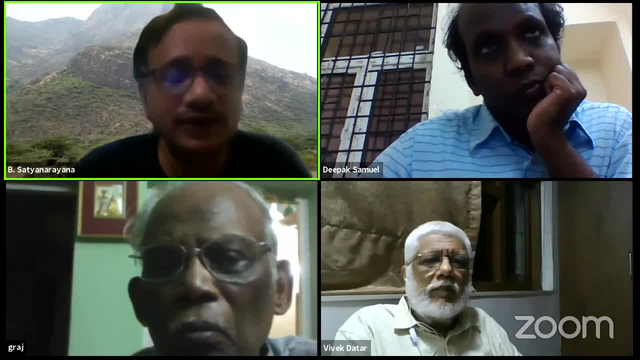 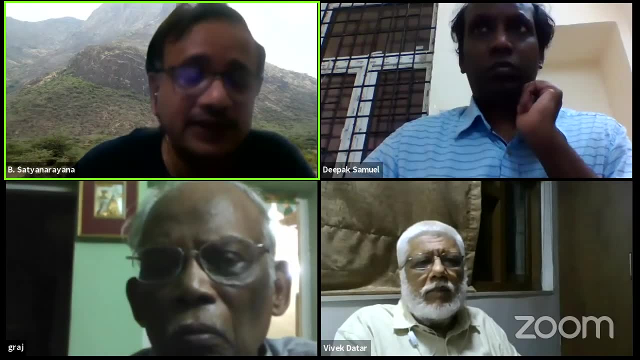 will see underground. If you see on surface, yes, But when you go underground I mean you can. if you calculate, probably it will be, like you know, less than 10 hertz. That is the trigger rate for the big detector. So you, most of the time you are just sitting. 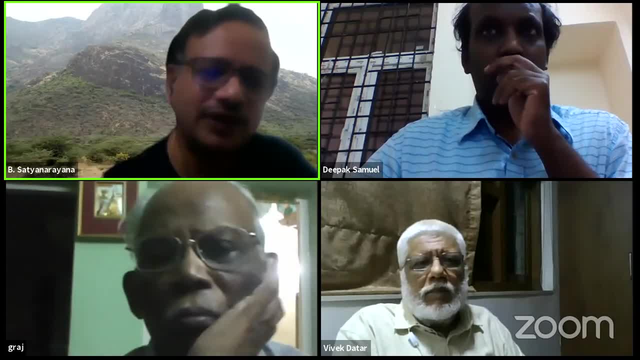 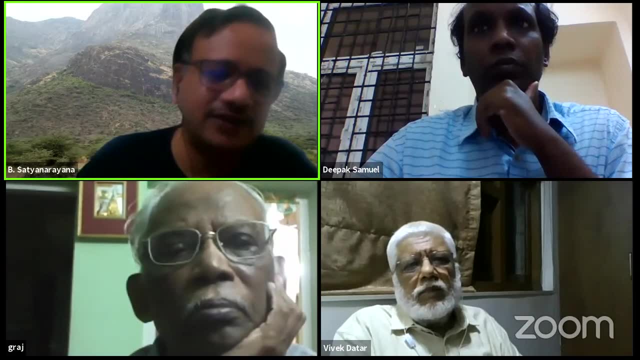 idle and only doing the monitoring of ensuring that all 30,000 RPCs, electronics, everything is working fine And once in a while, when the event comes, you actually trigger and the system will you know? you will be able to. you know. you will be able to you know. 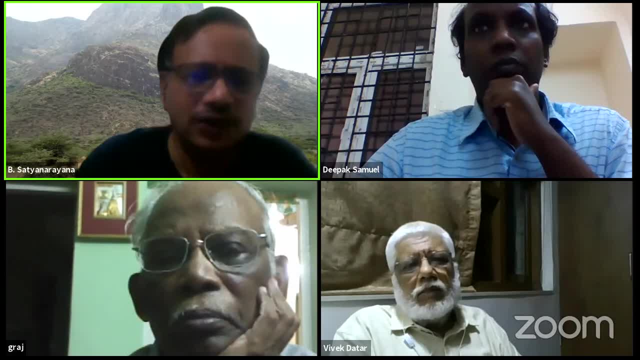 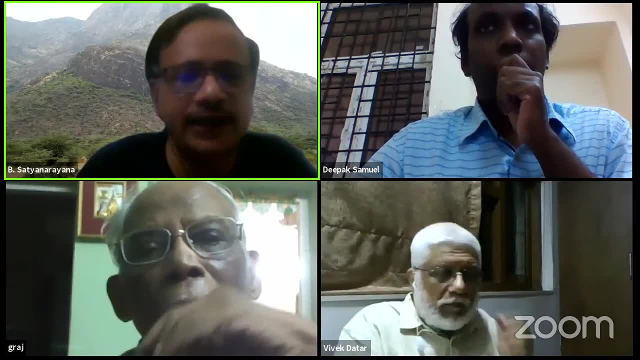 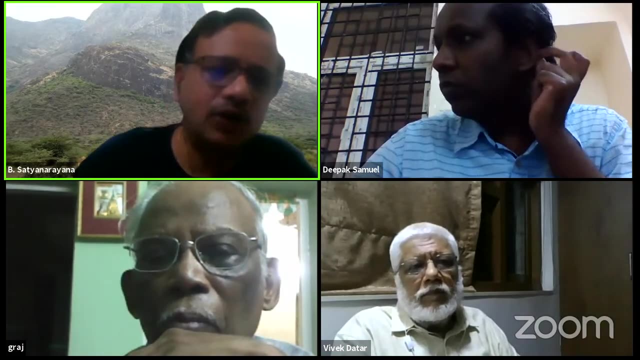 tell you, you go and record the data and send to the backend. So, to summarize, you don't require a very, very big server or in a big storage. Of course we are planning to have the basic system right at the detector and one system in Madurai and also system. 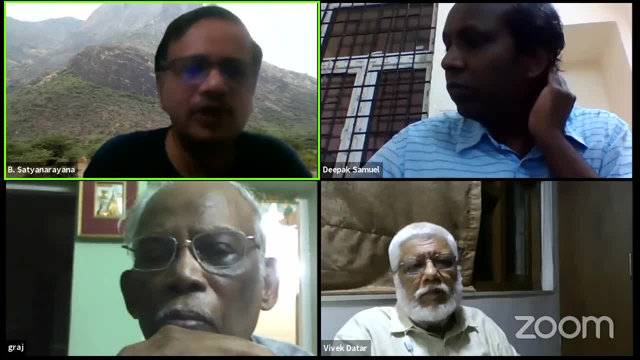 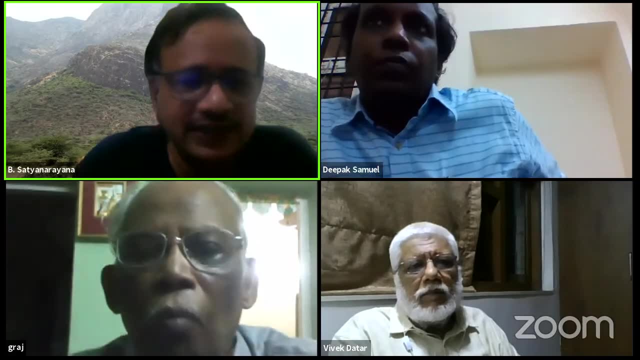 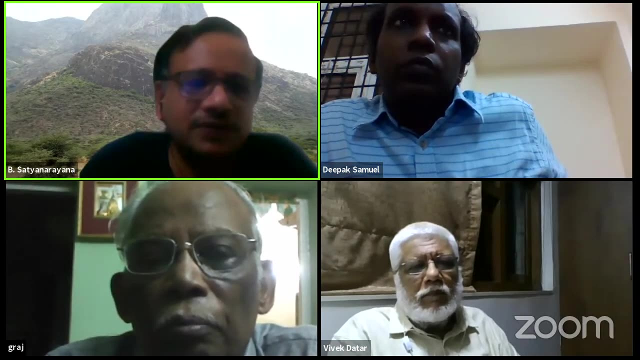 which will allow all the collaborators, where out they are, to be able to access the data. So there will be a sizable amount of computer infrastructure, but nowhere near like let's see or any other experiments, And not at all like what you anticipate in terms of, you know, cloud or very small data. 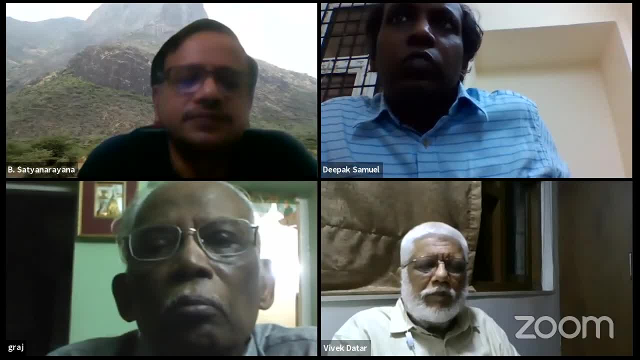 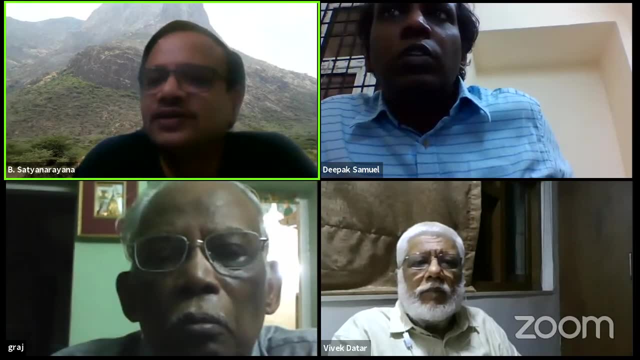 Okay, so thank you. Yeah, All right, So I think we'll go for one last question, or shall we? How many questions shall we take? I see two hands on, So we'll ask Ravindra to ask. Okay, Hello sir, Thank you very much for your very excellent talk. So yeah, I have a general 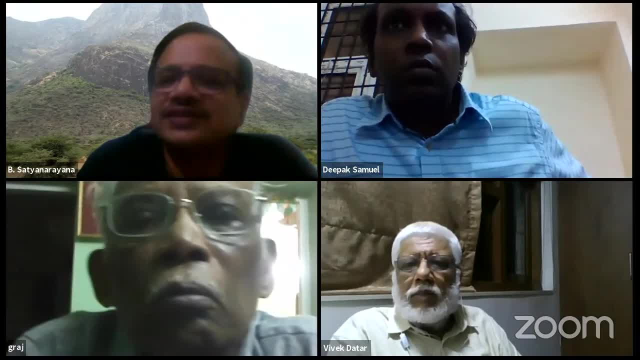 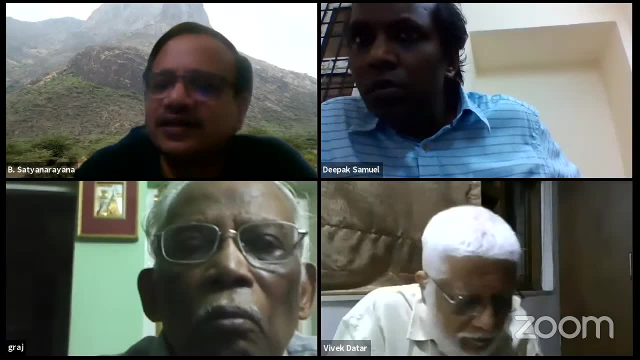 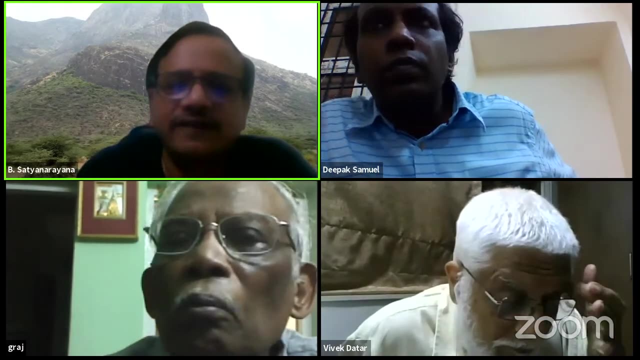 question. Okay, So I have a general question. Okay, So, I have a general question. Okay, So I have a general question- that while we- I mean, since we have discussed about the tracking, muon, tracking in your talk- generally on the surfaces, while we do, I mean, earth. 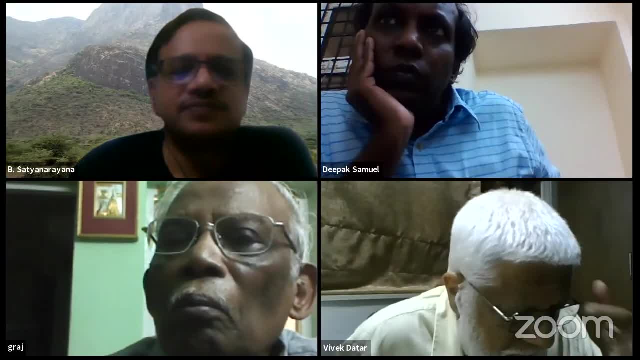 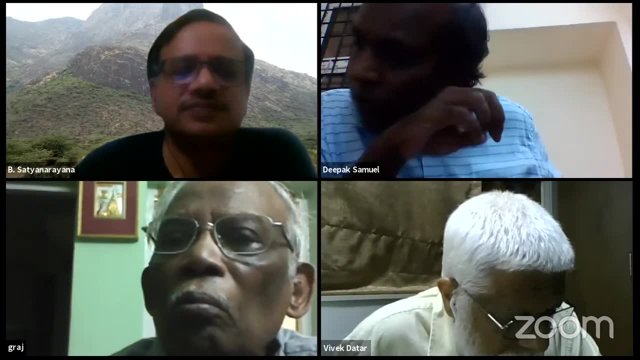 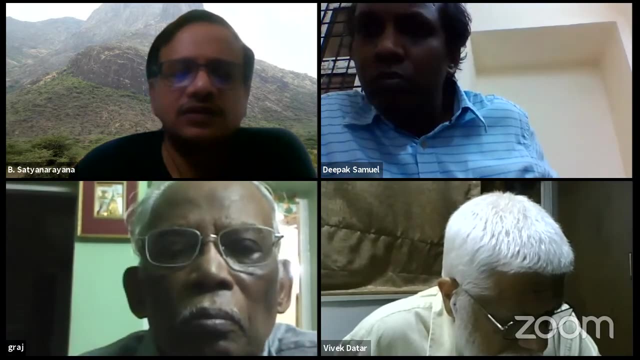 surfaces while we do muon tracking experiments, we have high chances of getting the combinatorial background. Yes, I mean in case of our underground, for example, in case of INO, do we have that combinatorial background chances? And if we have, what we will do further? 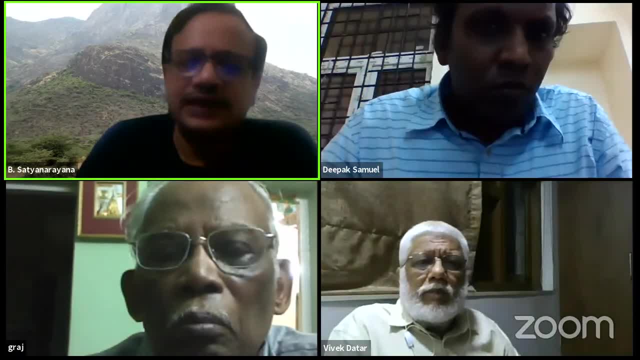 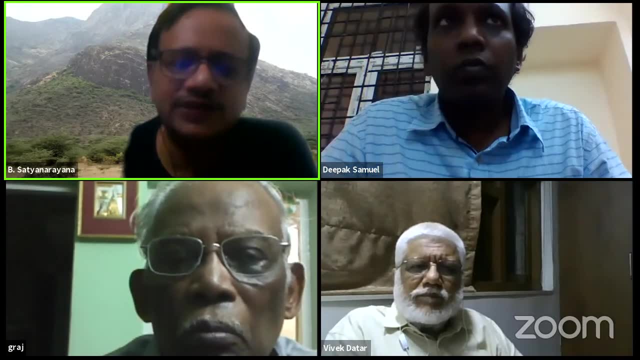 Now I think you're talking about when you say it's like sometimes we call noise rates, sometimes we call background rates of individual let's say strips in this case, which are picking up data from the RPCs. Now, when you see on surface, quite a lot of it also come from 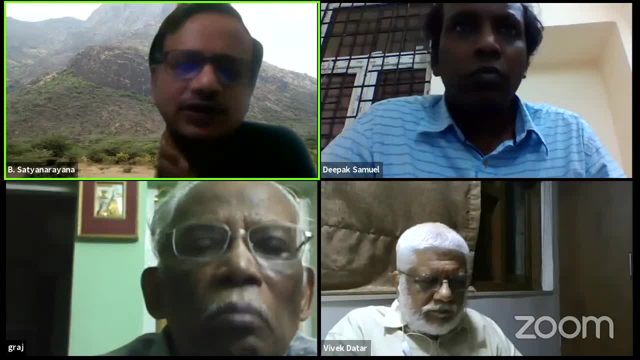 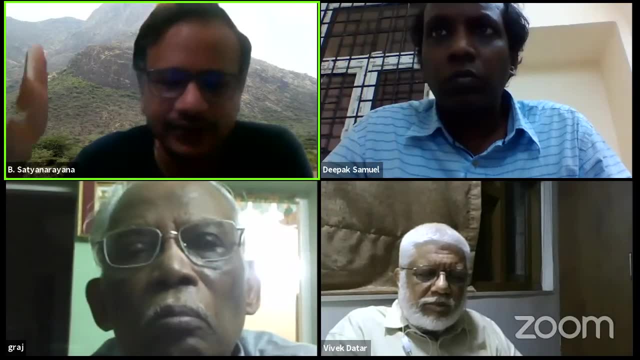 cosmic background And also it comes from all the materials tracer of radioactive material. Okay, There's a lot of radioactive materials around with what you make, the RPCs or anything like that. When you go underground, of course your cosmic- you know flux might come down. 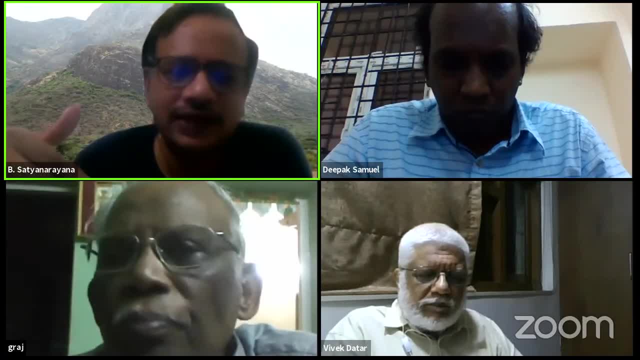 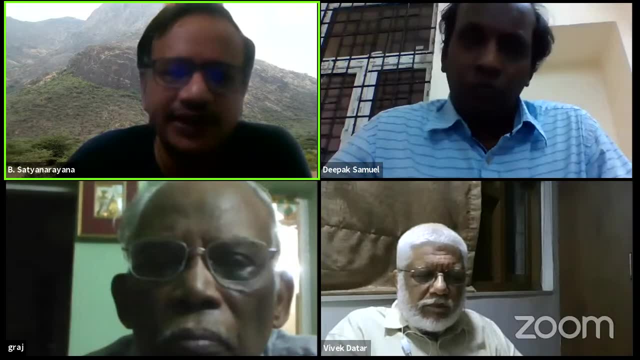 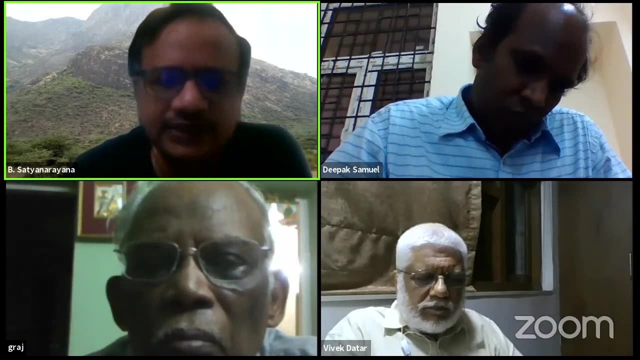 And so those rates might be coming down. but the ones that are produced in the rock are produced within the materials with which you make. that will remain more or less same. That is not going to kind of change, Okay. So when you design the trigger system, for example, which is the one which get affected? 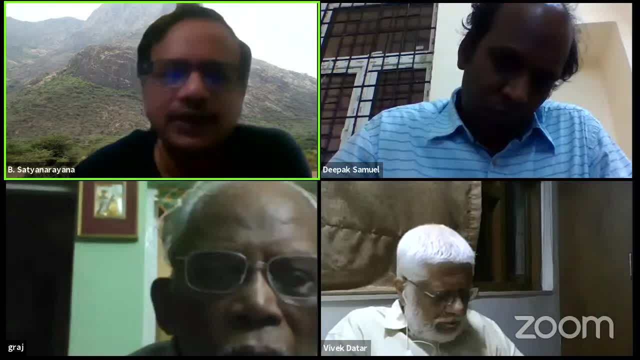 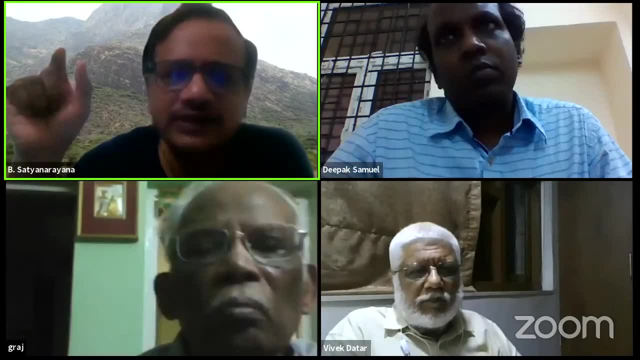 by the combinatorics that you talked about. Okay, So parameters like what is the window that you want to look for, coincidence, What is the coin, What is the multiplicity that you want to ask for and how well you want to segment it, et cetera, that those are the 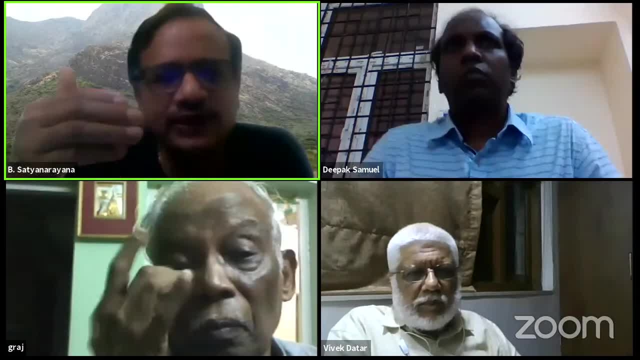 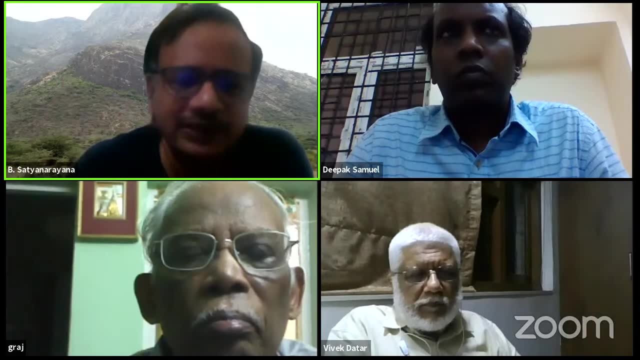 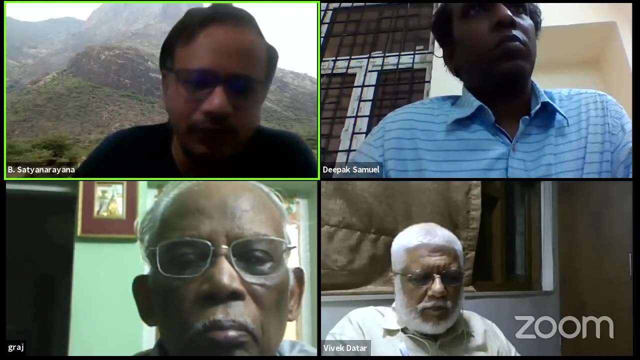 things that you have in your hand to kind of bring down the chance coincidence rate. But again, for experiments like INO or any cosmic, cosmic experiments, this is not too big a problem because you have quite a few such handles to kind of contain the chance. 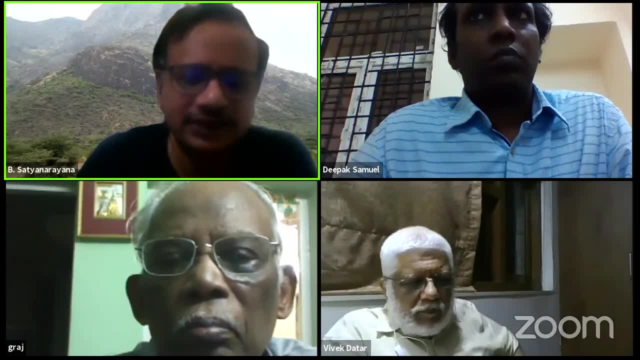 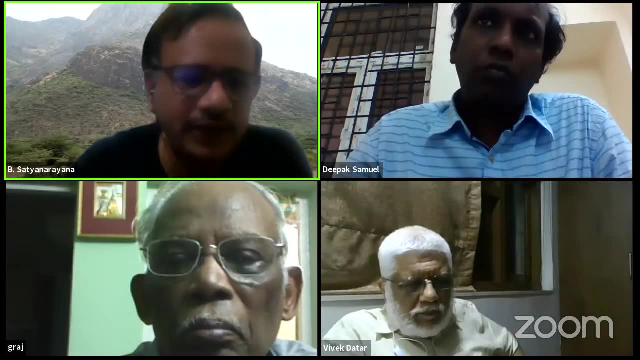 coincidence rates in this case. So only even if, like mini ICAL or engineering ICAL, when you build on surface that trigger rates could be, you know, 8K, 10K, even 8 by 8 meter long area. But when you go underground, 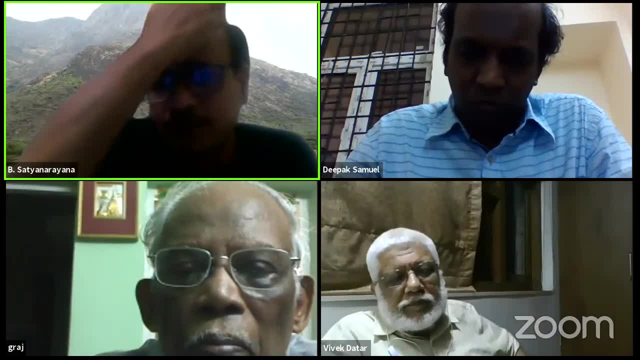 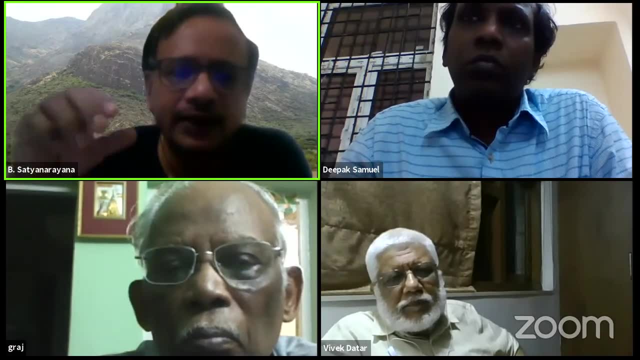 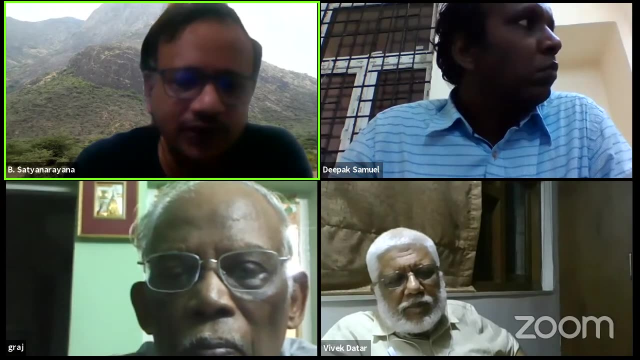 the rates come down and then when you put enough cut, you also will be able to bring down the rate. But see, it's important Also to keep an eye on what is the optimum threshold for trigger. Obviously you don't want to miss an event just because you wanted to reduce the chance coincidence rate, right? 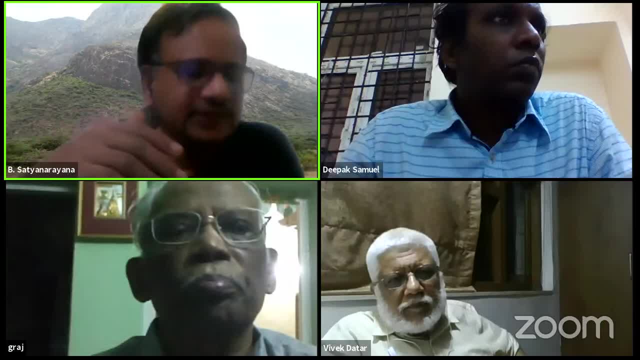 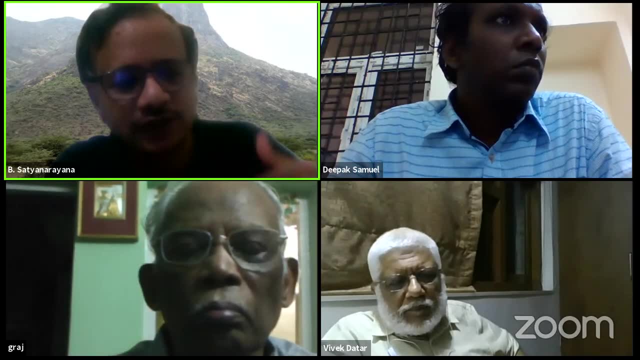 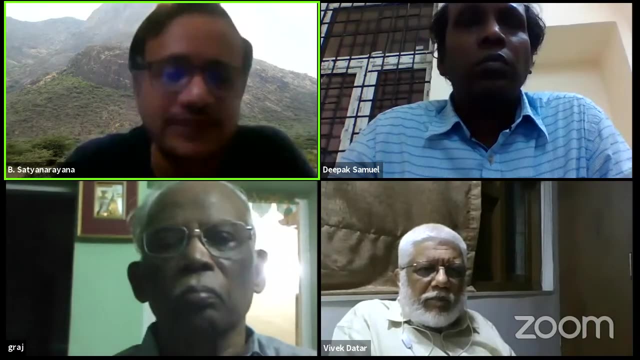 So therefore, sometimes people do say: what is you know data to tape. What is my capacity- Sometimes even use people- is to hit the trigger rate based on that. But nowadays you have plenty of data space So people don't mind actually doing so-called triggerless system. 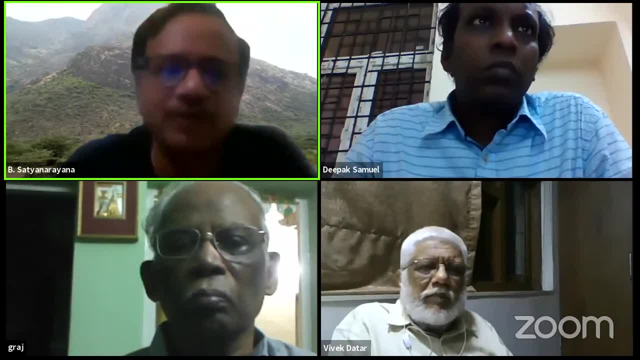 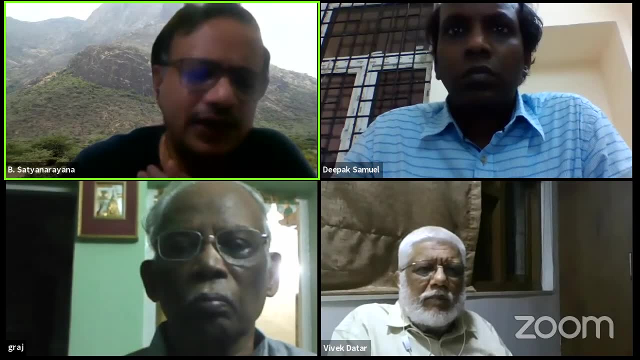 where you take all the data that is coming from RPCs and record everything and do your trigger criteria offline so that you can run whatever you like after that. You don't miss any data. So it is quite possible for experiments like I know. one could also think about that. 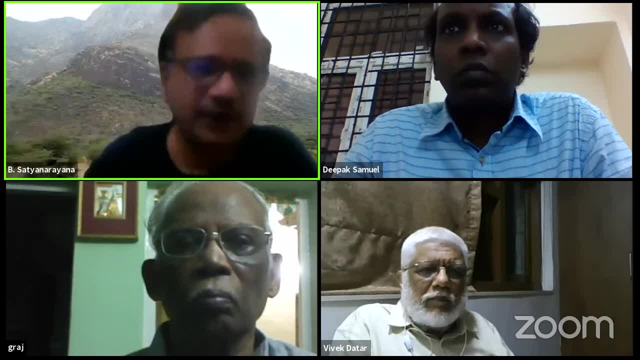 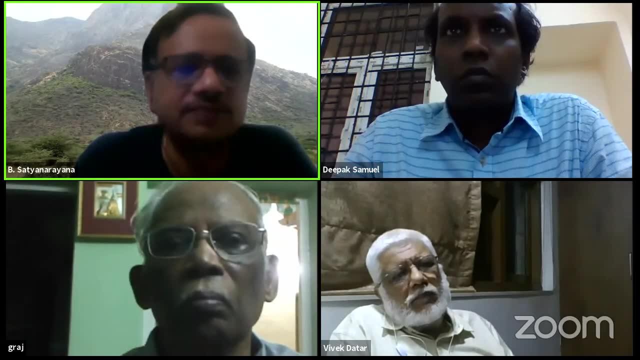 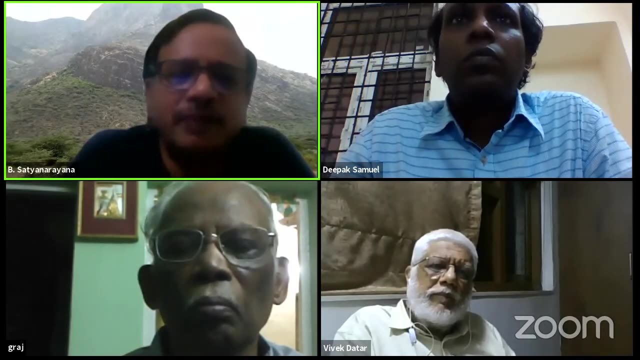 But there are other issues, like you have to have high speed data lines from front end to back end, And the architecture of the DAQ system is entirely different between triggered and triggerless system. Yeah, Okay, sir, Thank you so much, But, by the way, also need certain amount of background rates, what you call, because? 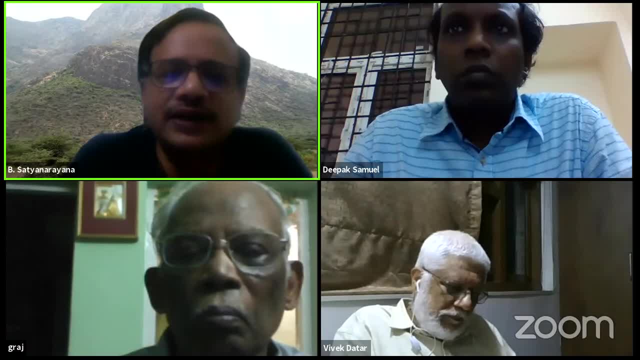 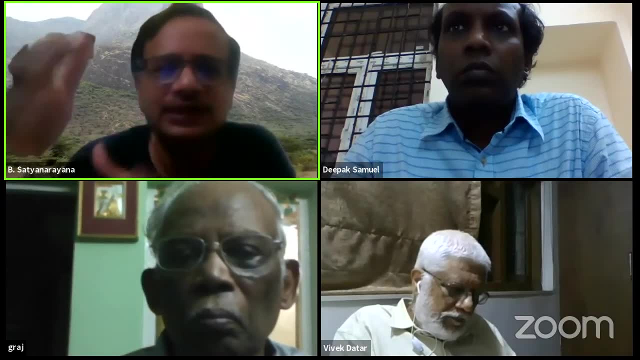 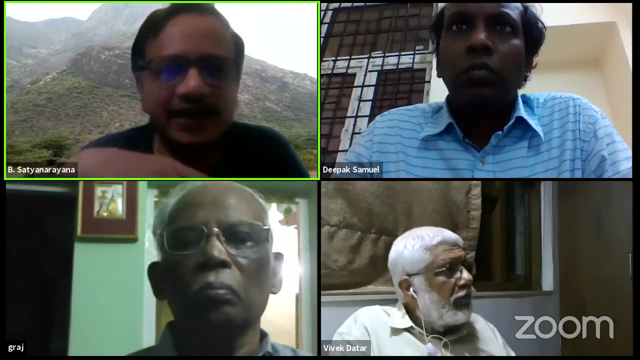 those are the ones through using which you are actually monitoring the gas pressure, the high voltage, the temperature, the humidity, all those parameters you monitor only because there is certain counting rate that you can depend on and get characterization between the rates and affecting these parameters. Actually, if the detectors are all silent, 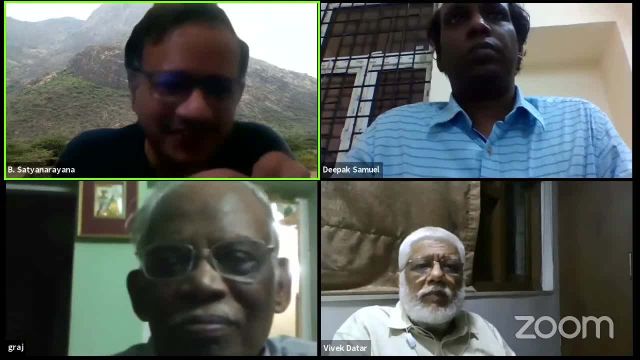 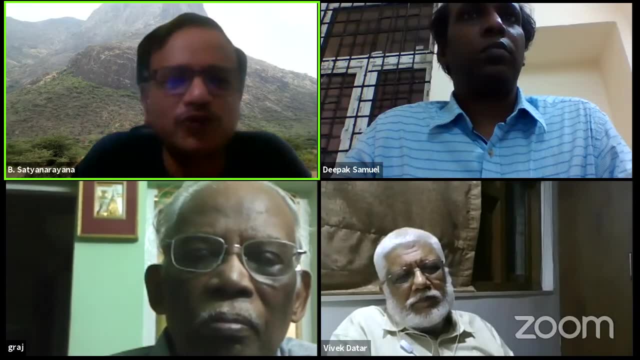 except for neutral interactions, you don't really know what is happening So you can know whether at that time they are sleeping or they're up and working. So you require this Also. it's a very useful thing to have some rates in the background And also record. 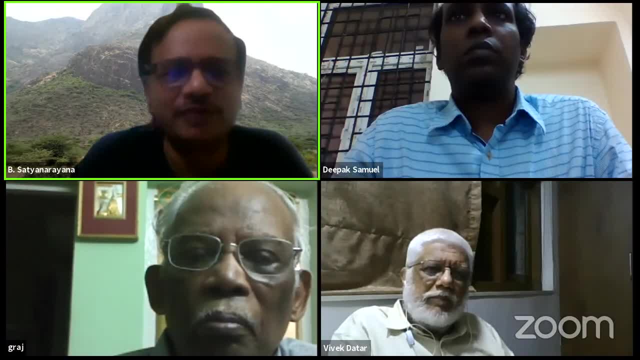 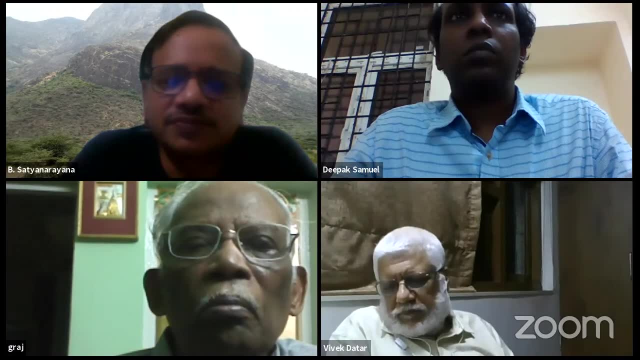 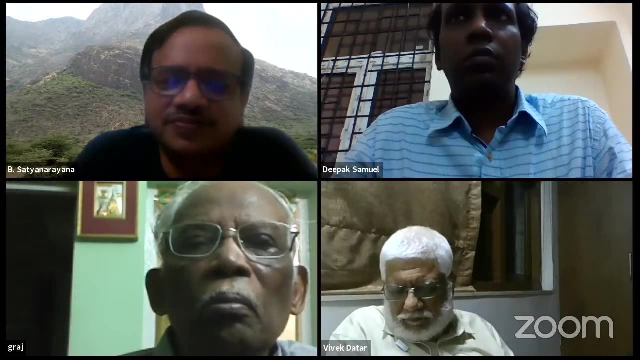 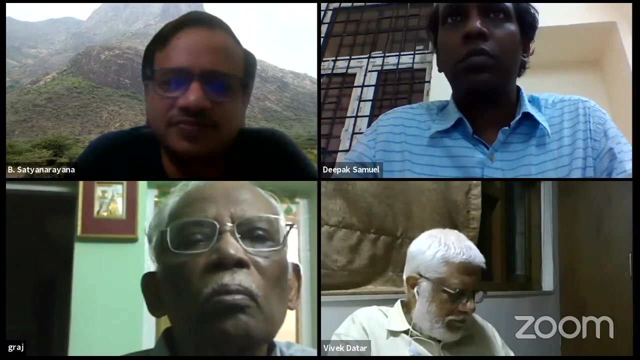 some junk events doesn't matter, You can always throw them rather than missing an event. Yeah, but for example, yeah, I think no. I mean if there is a chance of, if I am looking for the track from one Mian, if I get hit from other Mians in the first track, other. 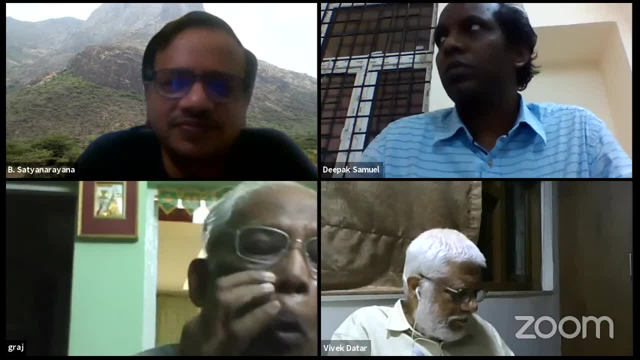 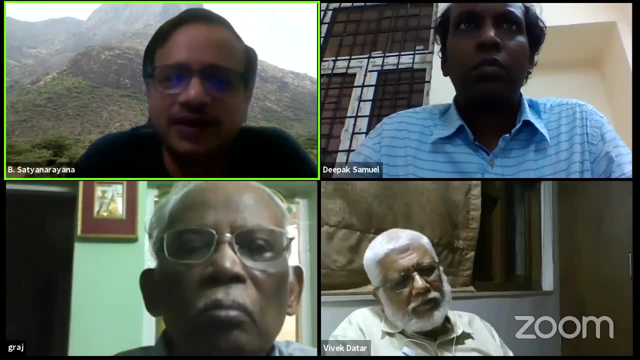 second Mian hit in the first track. so can we remove that? Yeah, you want to record multiple Mian events, right? Why do you want to remove them? I mean, it all depends on your trigger, right? You saw, even in such a small detector, Surya. 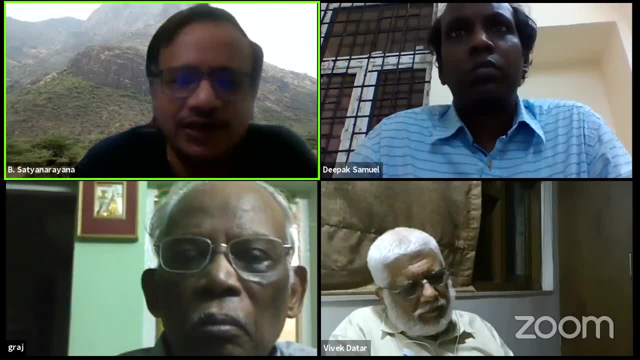 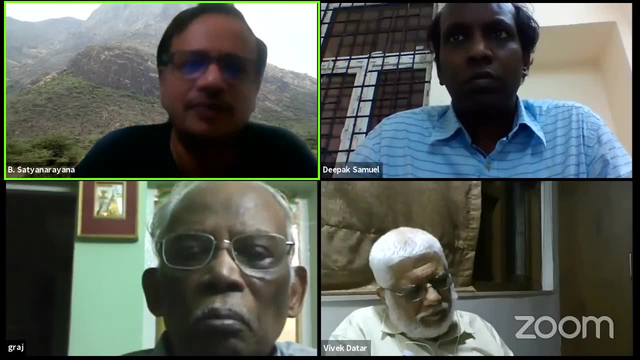 you know one of our students. he actually showed those Multiple Mian events right. So your trigger has to accommodate, Your trigger has to accommodate and it will accommodate Because if the condition is only so-called P into M, by, P into L, by 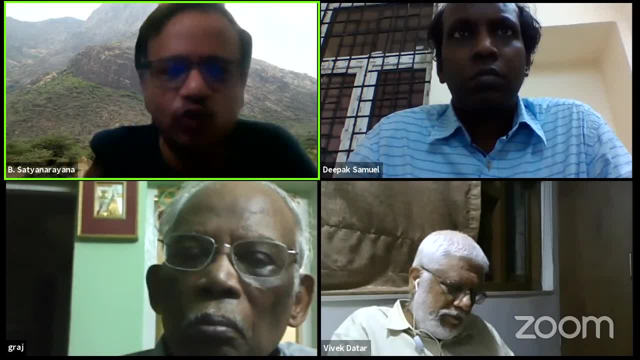 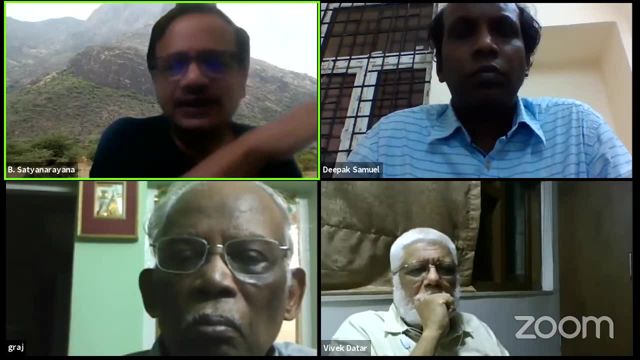 M or whatever. I mean that condition will decide what is your trigger. So if there are two Mians, multiple Mians, two going Mians, hadronic kind of events, large angle events, you have to have, you know, every trigger subsystem looking for this And when you put 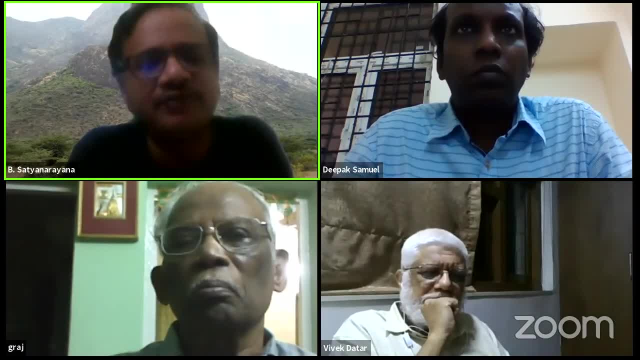 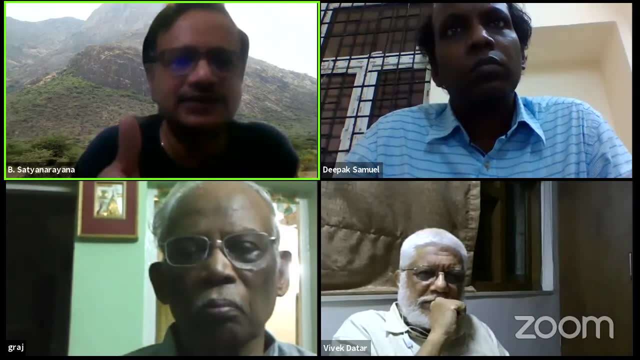 them together. global trigger should take care of all sort of events that you envisage. By the way, modern day people don't anymore, you know. fix the trigger and say: this is my trigger system By using this programmable chips tomorrow, if somebody wants a new trigger, you don't have to go and keep changing the wires. You just send the new lookup tables to the FPGAs. they start implementing new trigger conditions. That is how LHC or any other accelerator experiments do. So you have to have trigger condition extremely fixed. 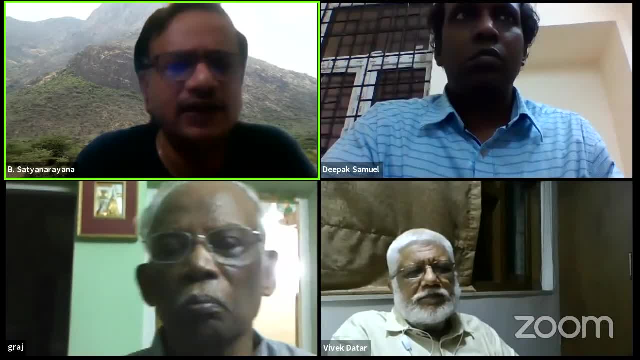 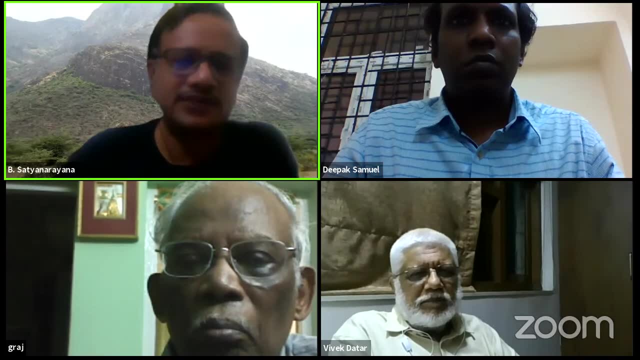 How do you know? After you get the data, the physicist will say yeah, no, no, I think your trigger is too shallow or it is too strict. I would like to change it. You cannot say no, I will change 3 million wires in my system, So it's important to keep that. It's very 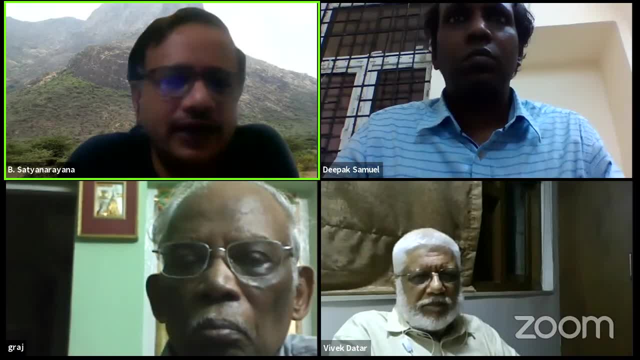 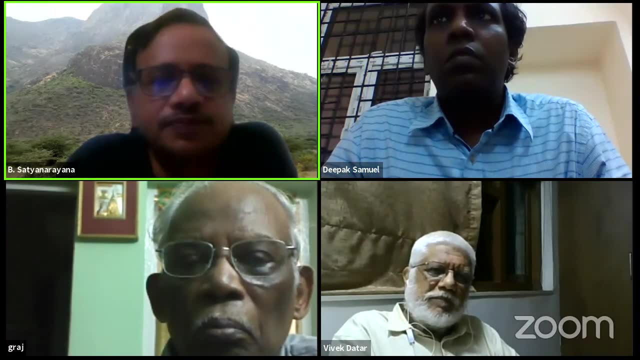 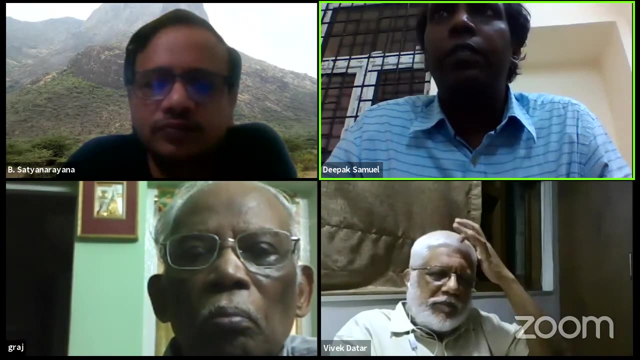 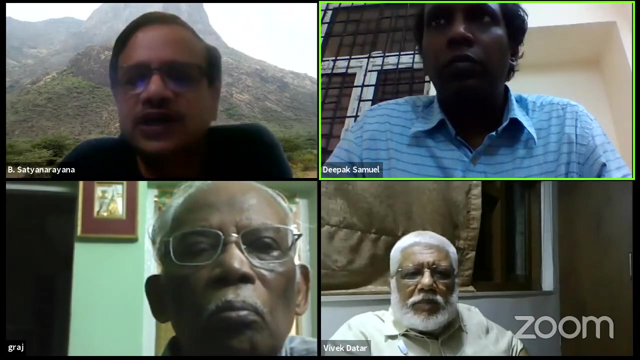 trigger system is the most important system of any high energy, or cosmic or nuclear, whatever- I mean experiments. There's no doubt It's even more complex for accelerators. Okay, Yeah, Thank you so much, sir. Yeah, We'll take one last question from Rohan. Rohan, please go ahead. 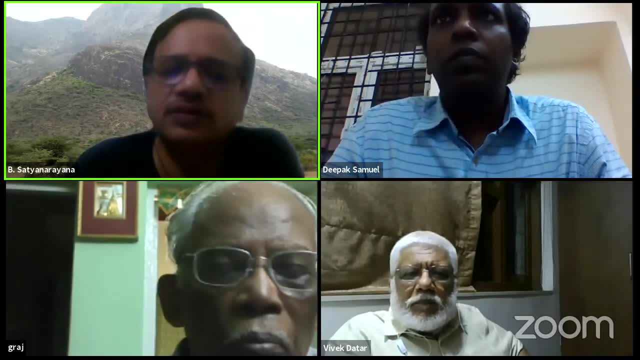 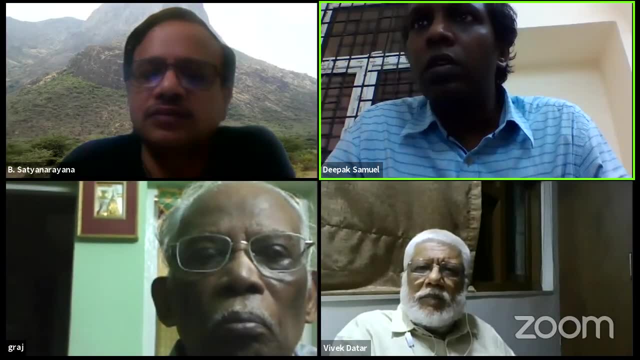 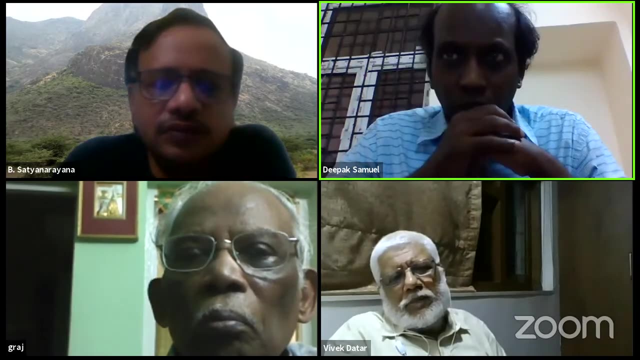 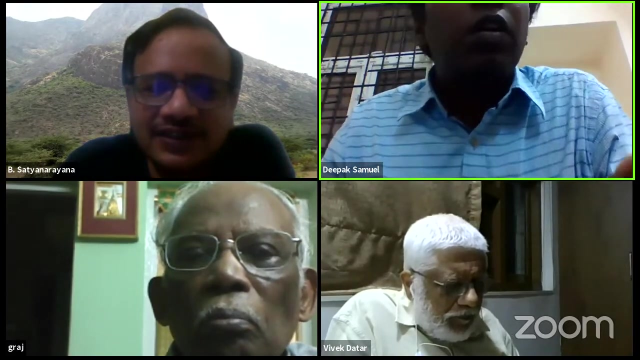 You have to unmute. Okay, He is gone. Oh, yeah, he's there, Rohan. yeah, Hello, Can you speak a little louder please? No, we can't hear you, please, Hello. Good evening sir. 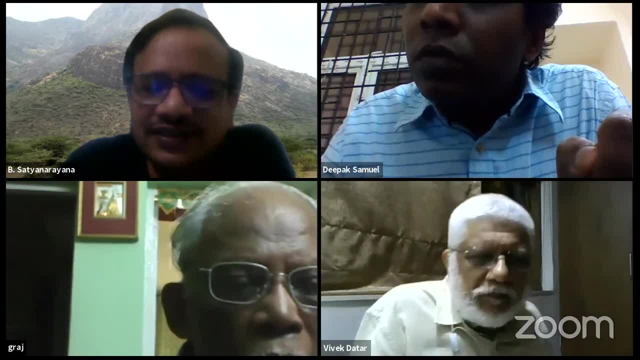 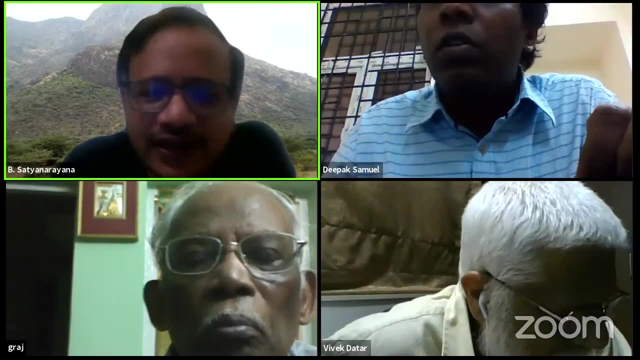 No, it's not clear. still, Some of the experiments are carried out at cryogenic temperature. Can you please type your question so that we can read it? Actually, Deepak, I can hear him. Maybe I'll repeat the question, All right, Okay. 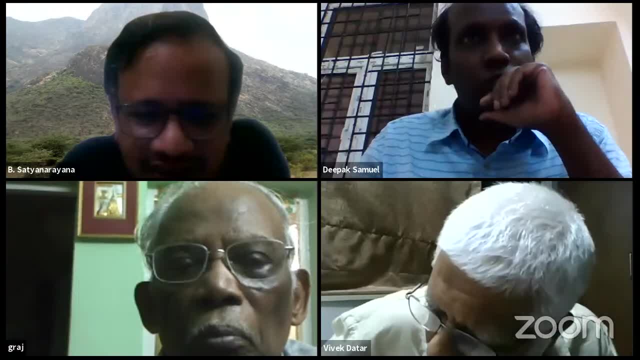 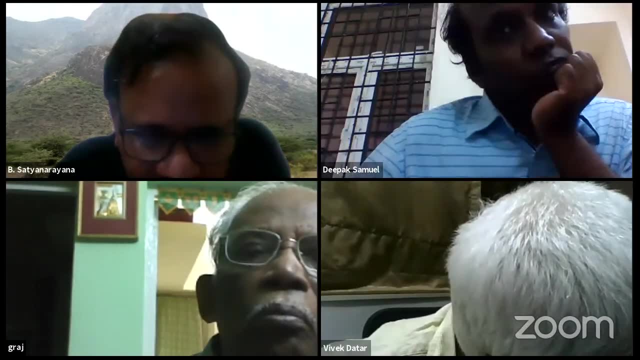 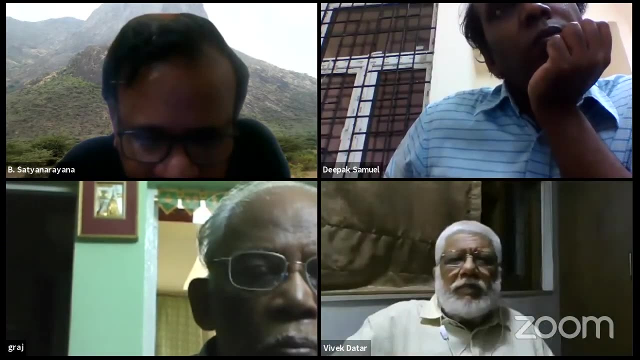 Some of the experiments at Ion-O are carried out at cryogenic temperature. So I would like to know: suppose that in volumetric experiment we are using a preamplifier where JPEGs are used at 120 Kelvin, But if we take a normal JPEG which we are using in our practical labs? 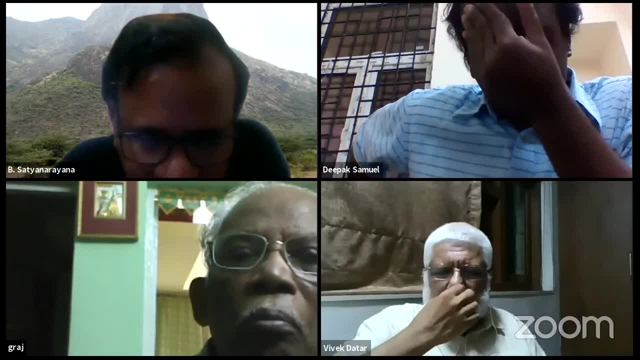 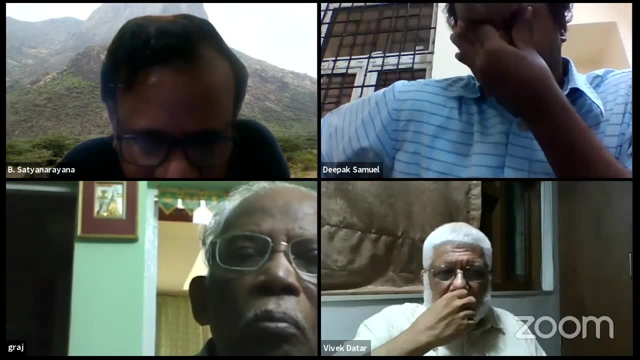 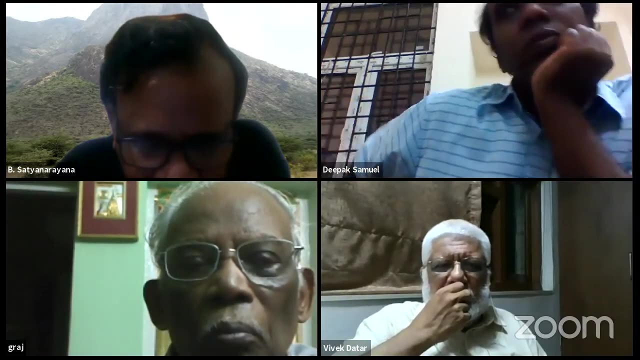 it has a temperature range from minus 60 to 100 degrees, 125 degrees Celsius. So how this chip? so same transistors are used at cryogenic temperature. How do you calibrate or how do you manage with these devices? So do you use a special grade device or the same components? 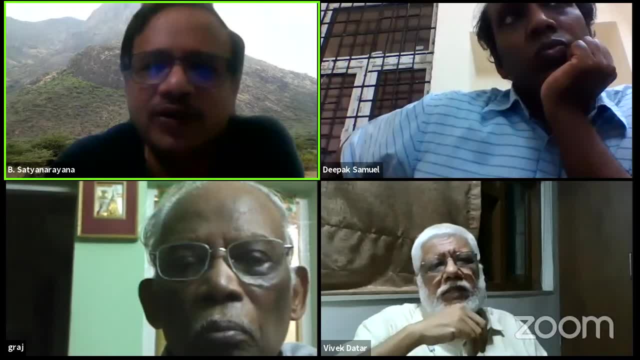 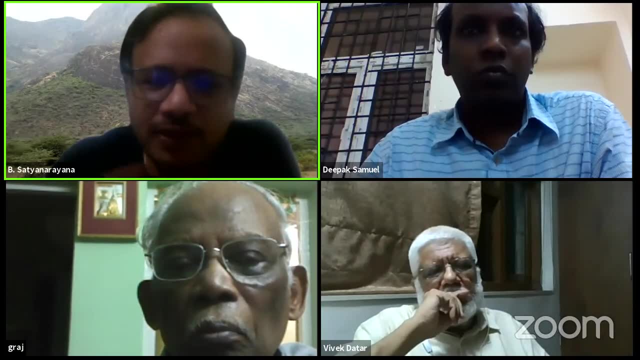 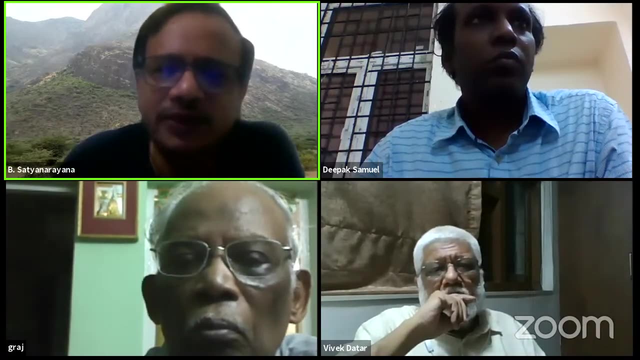 No, no, Okay, So this question is about cryogenic detectors like NDPD or any other futuristic detectors which will also come up in Ion-O. Otherwise, when you develop electronics for that, some front end, let us say, has to be at the cryogenic temperatures. 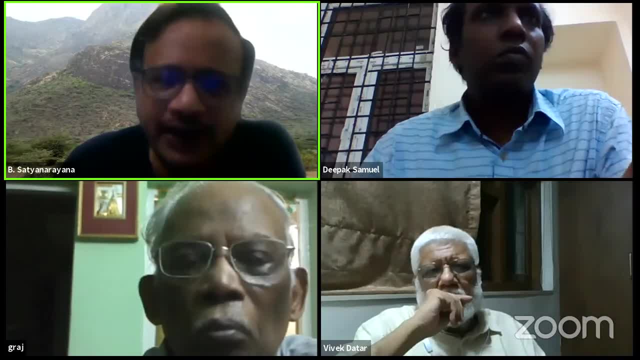 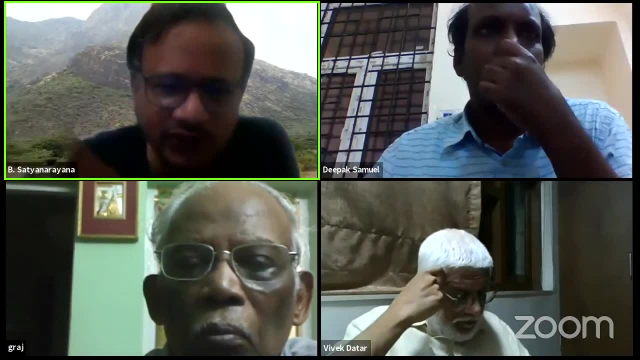 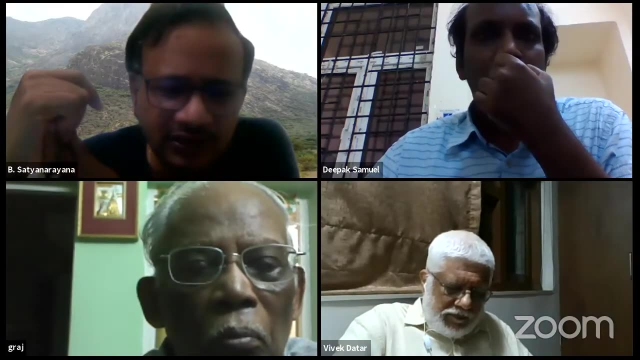 So the FETs that you normally buy, whether or not that will match to the electronics requirements for such a detector? Is that the question? No, my question is very general. like the components which we are using at room temperatures, can the same component be used at cryogenic temperatures? 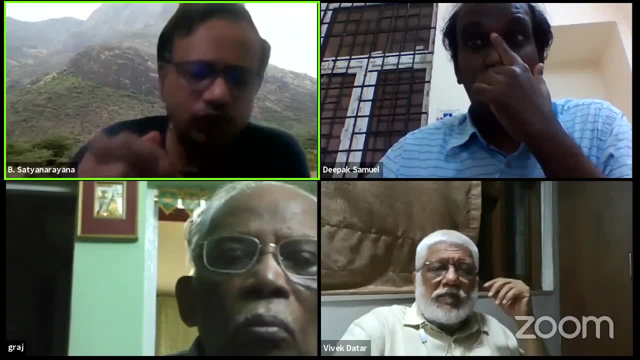 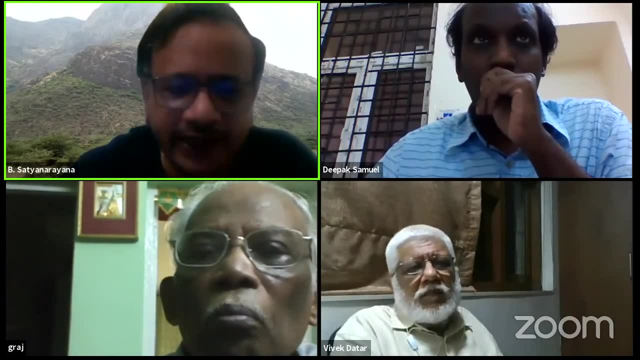 No, no, no, no, I think there are. see, you mentioned about FETs. Once again, I think probably Professor Dathar will be the best, Best person to answer, But let me just start by saying that nowadays there are specific designs of the FETs that were: 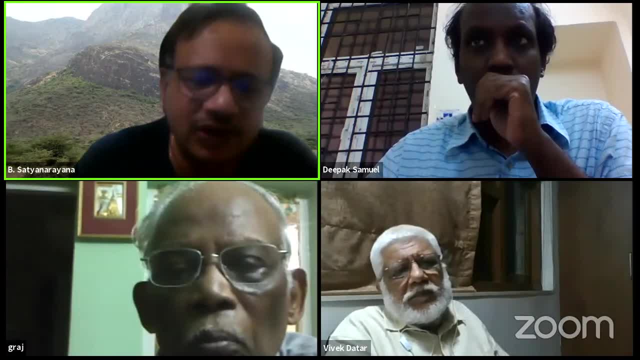 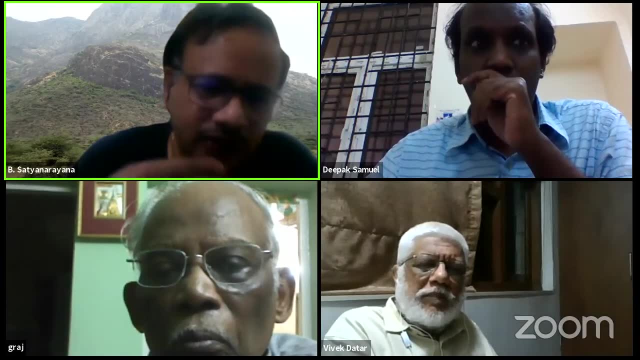 that people make for varieties of applications. It's not like something so-called. you know, any FET will work for any system, Not only for cryogenics. even you know there are FETs which are used for VLS electronics. 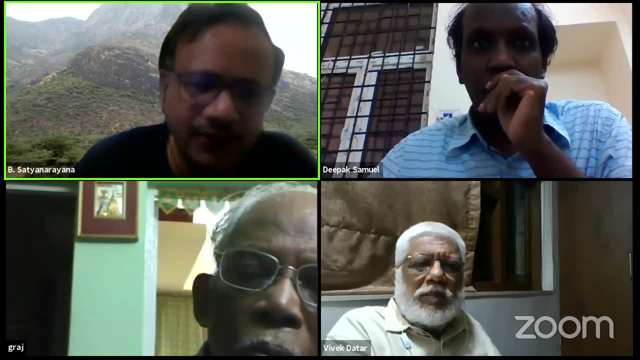 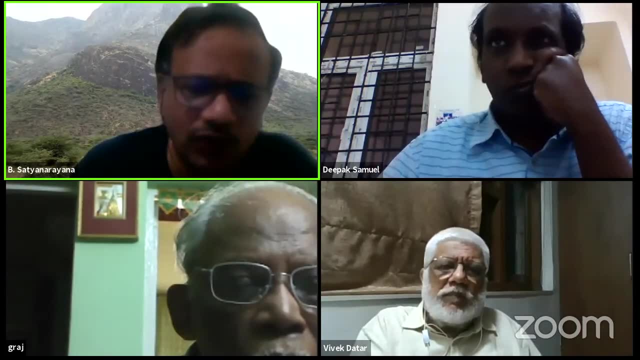 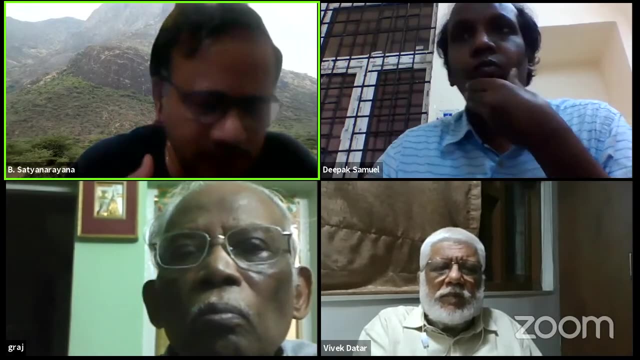 There are FETs, which are used for very, very, you know, electrometer kind of circuitry, very, very high impedances circuitry, Which are required for low current measurement systems, and so on. There are many special purpose, In fact, some of them even the material that is used for making them also. 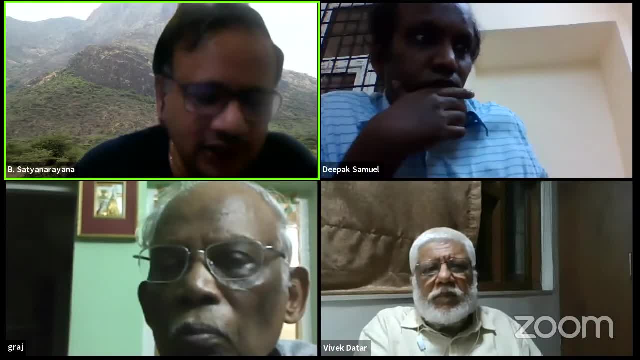 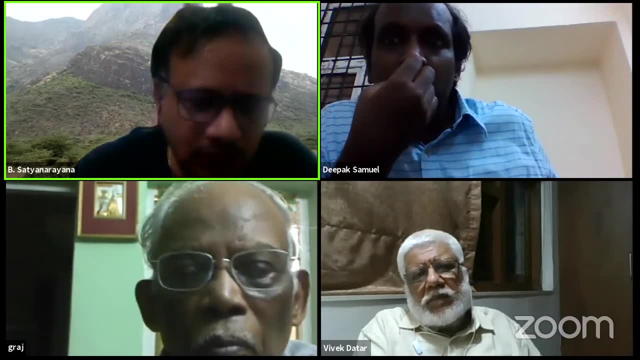 there are companies which make specific FETs for specific applications. I know for sure, But I'm not sure whether. no, if your question is whether ordinary FETs can be used for these applications, the answer is no. The answer is no. 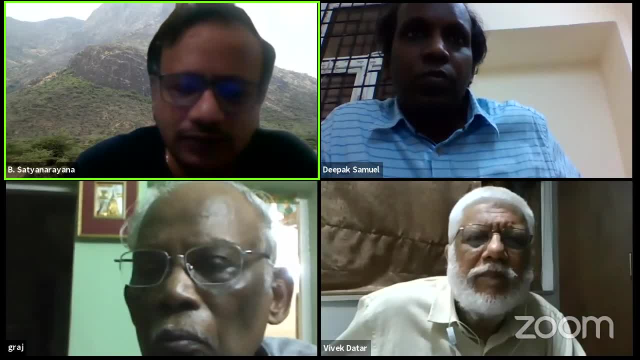 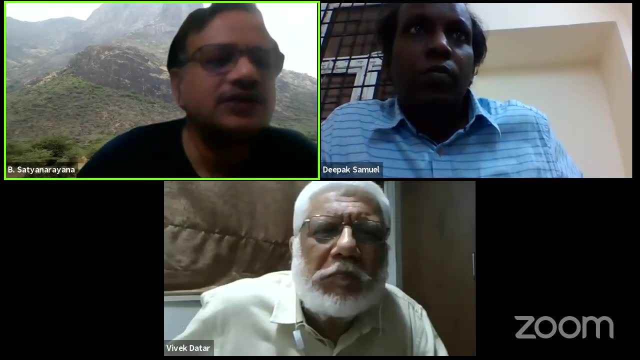 I think Professor Datta probably can give you a more authentic answer, because he also worked on cryogenic detectors. Sir, you have to unmute your mic. Yeah, yeah, Now I can. I think we are allowed to unmute, Okay. 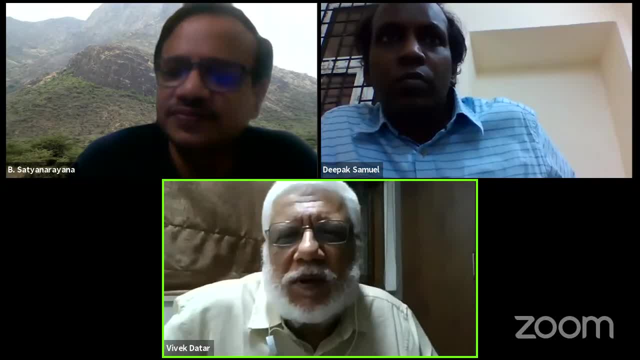 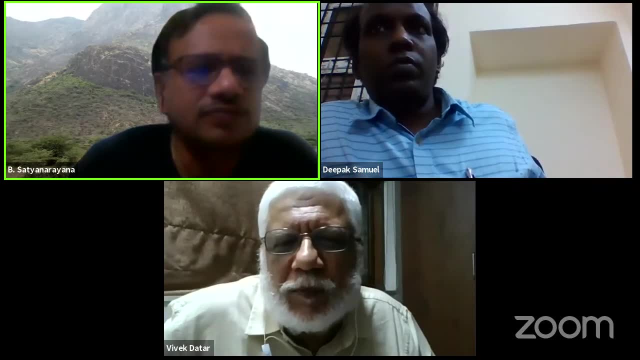 No, no, What you said is correct. Any old FET will not do. It has to be, I mean, a chosen FET and also something that works at cryogenic temperatures. Yes, It's typically. I don't know if you are familiar with the. I mean, I don't know. 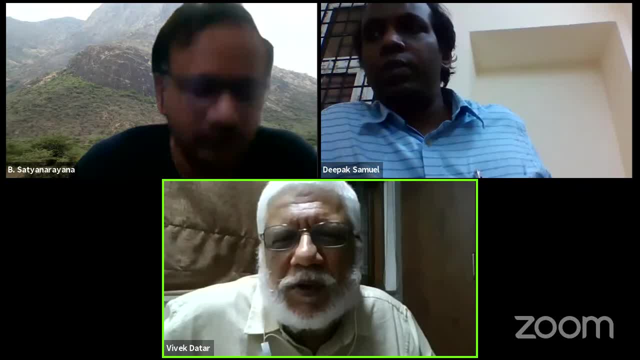 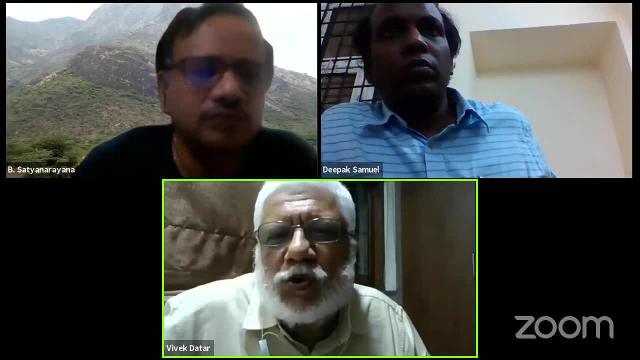 Yes, I mean high purity germanium detectors. They don't operate at Kelvin temperatures, They operate at about liquid nitrogen temperature. But there also you have to choose the right FETs and I mean it's possible to do that. 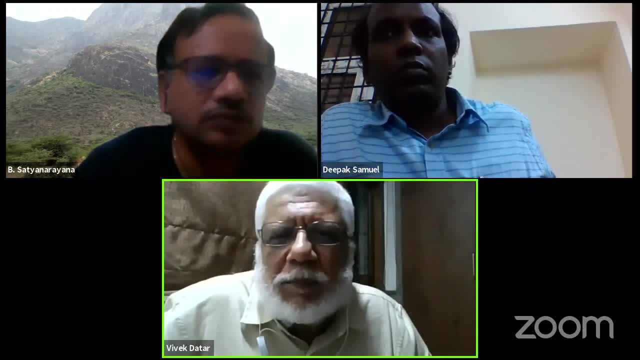 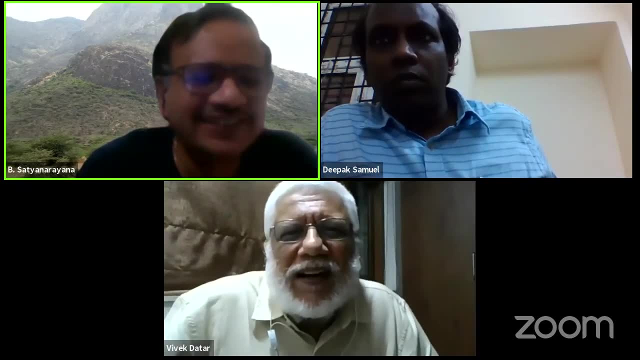 And of course, when you go to Kelvin temperatures or even 110 millikelvin, then there is a different set. I think that has to be used and care has to be taken on various fronts, Not only on the electronic, but also mechanical things. 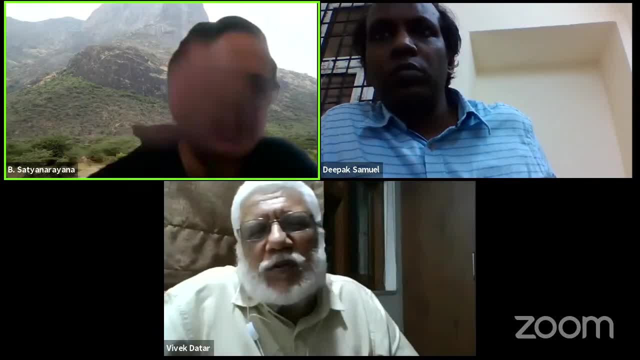 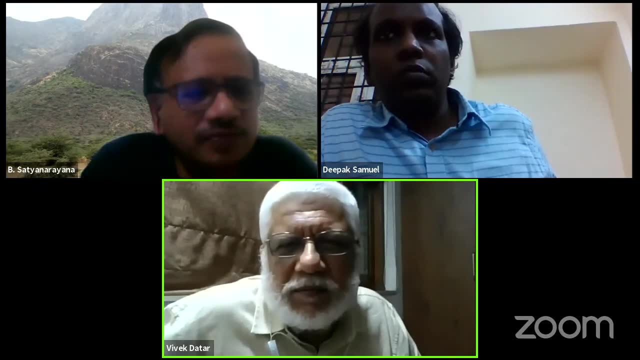 Mechanical Contacts and so on, Also the contacts and wires, and you don't want to use them as thermal antennas, Correct, Correct So. but yes, I mean, there is a sufficient amount of experience nowadays that you can use these Also, I think, for the very low temperature things you also use, you know, superconducting. 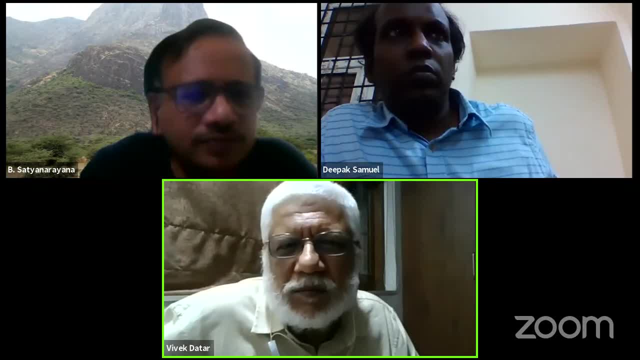 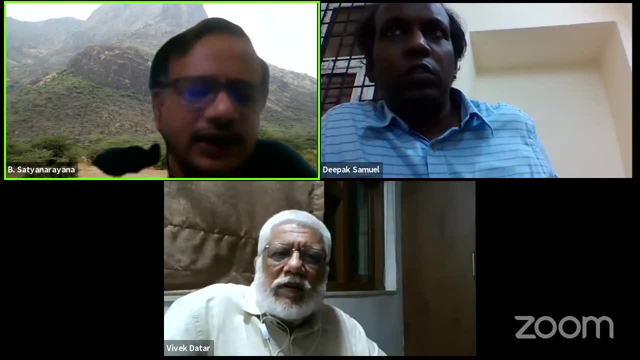 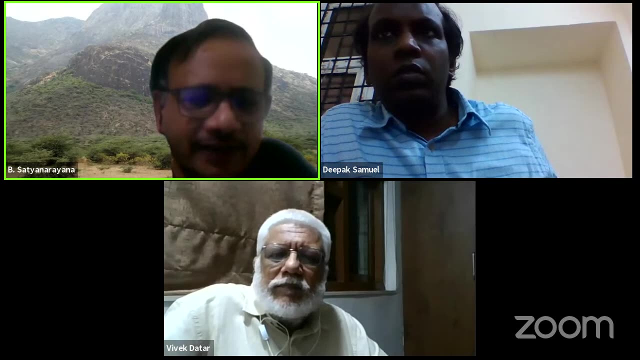 devices to identify and detect signals. This is Rohan. This is Rohan. The question from Rohan. right, You might want to go and listen once to Professor Vandana Nanal's talk. I'm not sure if she described them in that detail, because she gave a talk on the same. 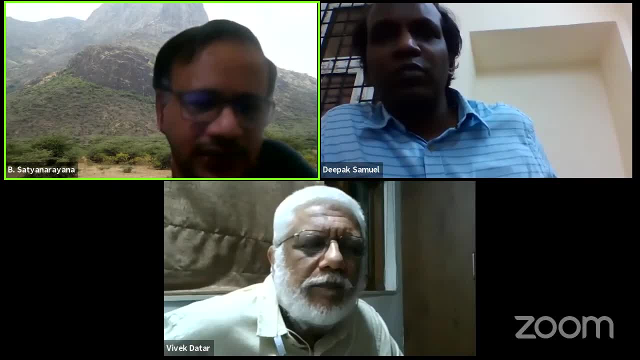 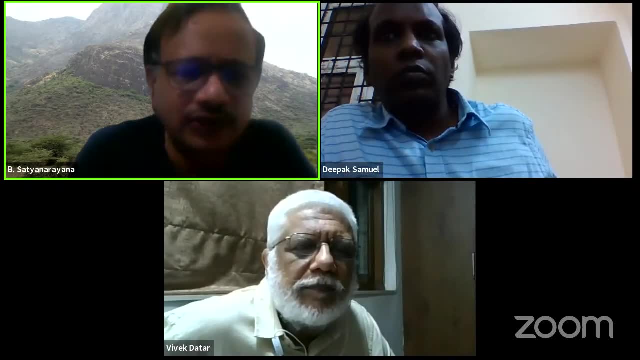 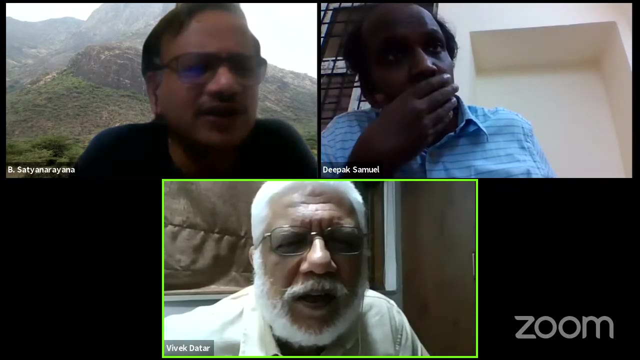 forum about the NDPD detector and the other experimental R&D. But incidentally, one of her students right now is actually designing electronics for the cryogenic. So if you listen to that talk maybe something will come up. I don't think it is there so much in the talk, but he can certainly write to that group. 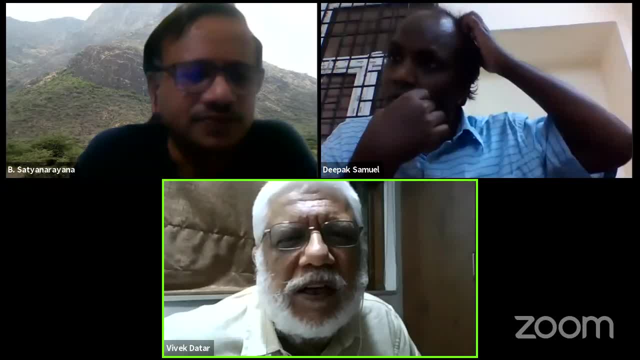 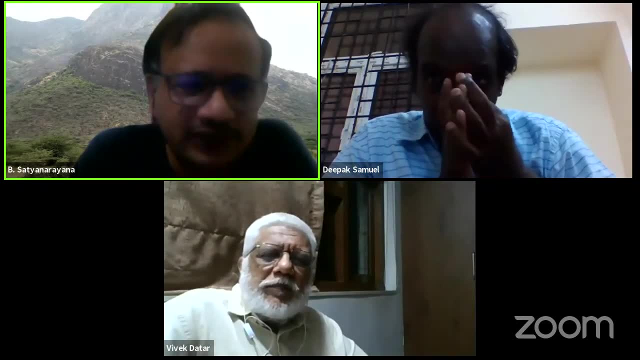 That's there on the TIFR website, The DNAP, or maybe you just…. I can even give the name of the student. His name is Vishal Vatsa- Vishal Vatsa or Vatsa, I don't know. 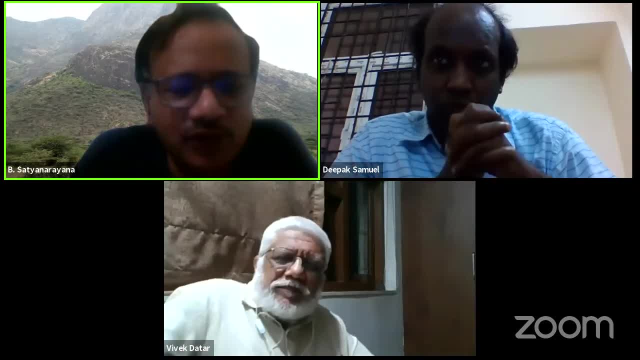 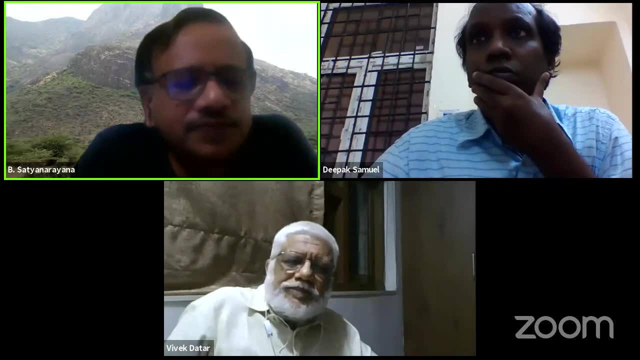 Vishal Vishal Vatsa, So you can write to him. You can see TIFR people's finder. He is the person who is actually working right now for his thesis. Yeah, Okay, sir. Thank you sir. 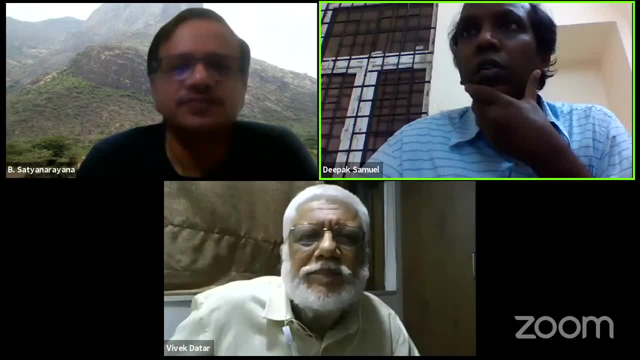 Rohan, do you have any more questions, or is that it Because you are…. Okay, Yeah, He pulled that on, All right. Okay, So I think there are no more questions. So from Zoom, do you want to take questions from YouTube or…. 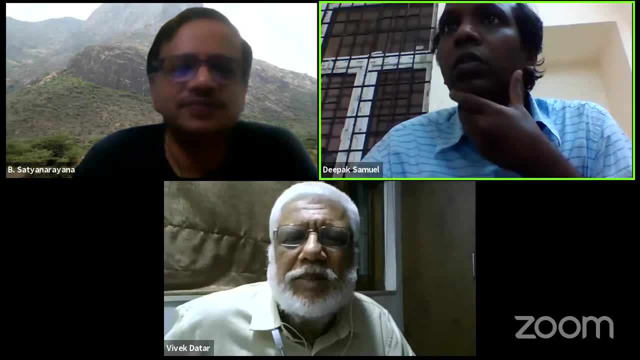 Yeah, I think they are already…. It's already 8 o'clock actually, All right, So I think they are all TIFR students. Yeah, If they are TIFR, we can… They can always…. Yeah, Yeah. 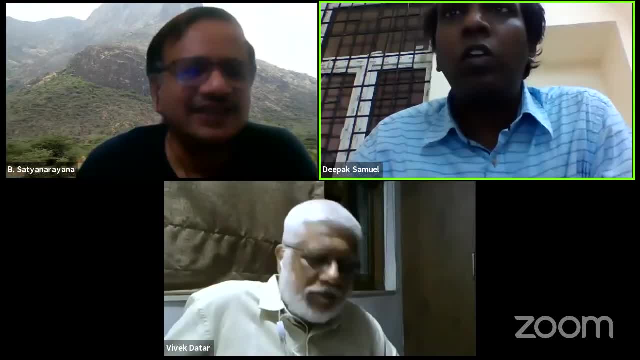 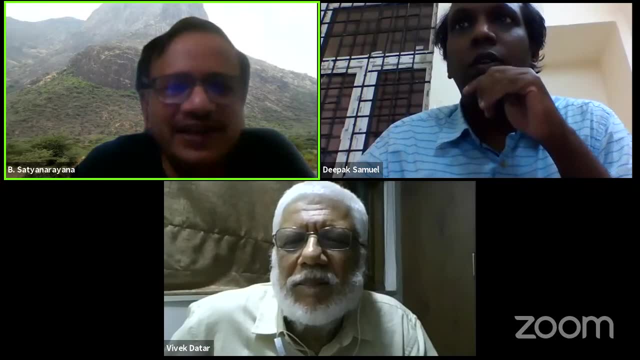 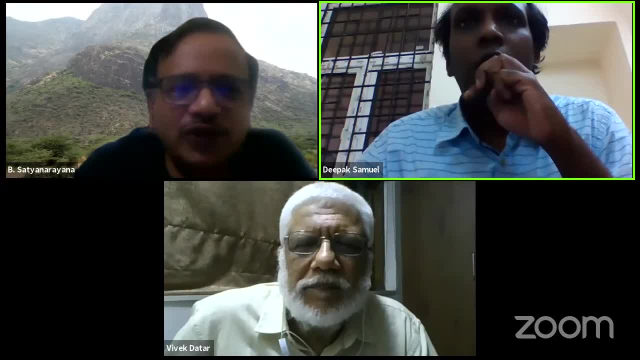 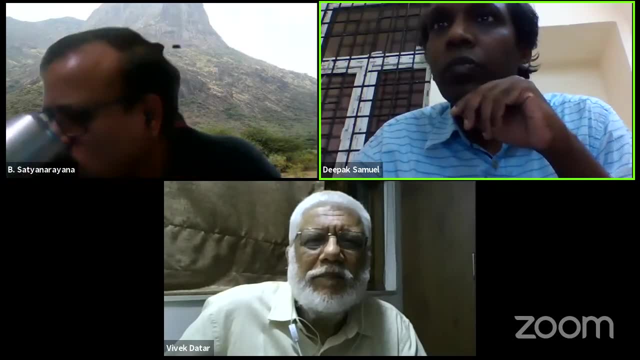 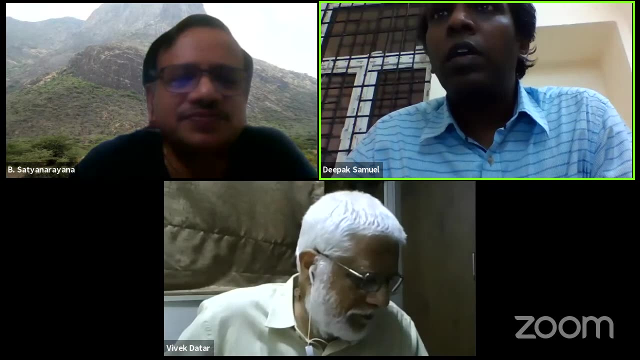 I don't have any problem, but I don't want to keep you holding, So okay, So well, specific questions. I think we can take one and then… Okay, okay, So what is track A and track B in the KGF experiment? 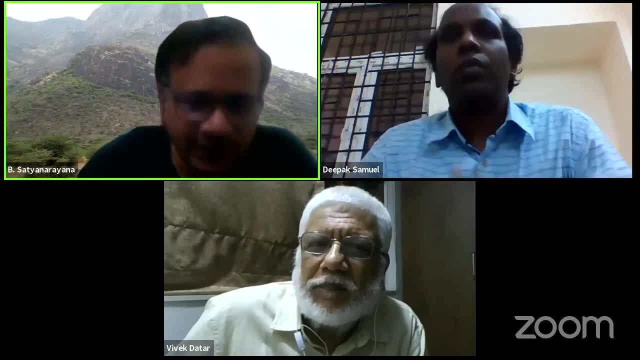 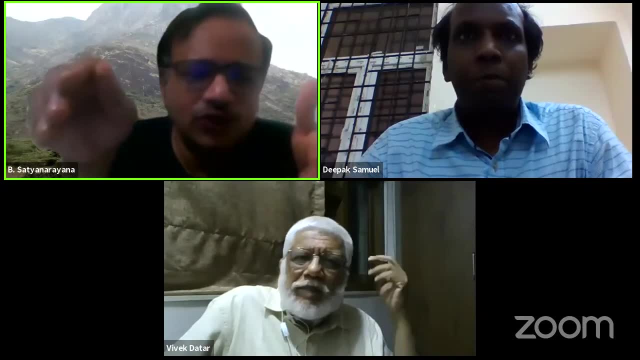 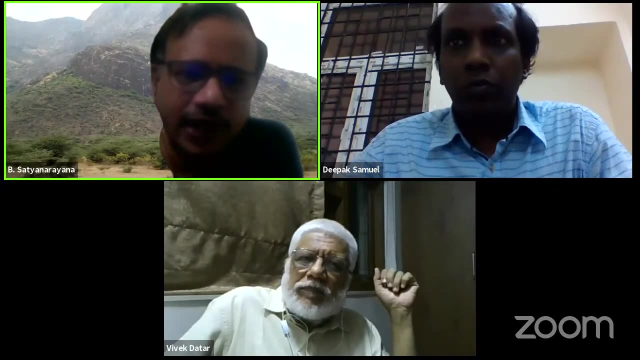 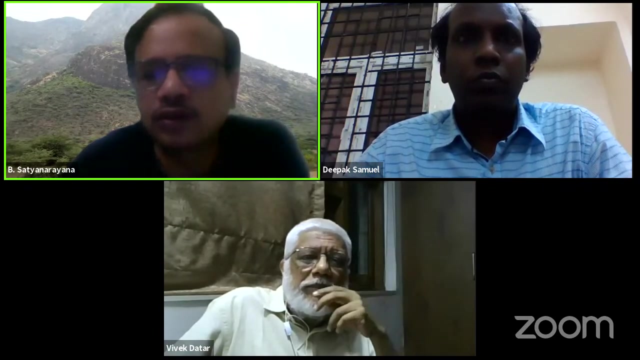 Where is the neutrality? need to know? Okay, So this is. it's coming from the rock which is, I think, a meter or so off. Okay, And the track that you see up, I don't know if I should show. 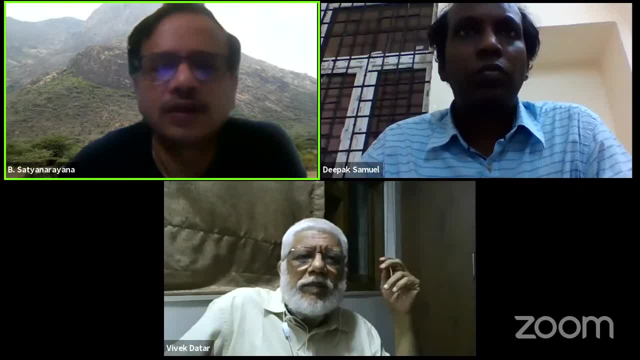 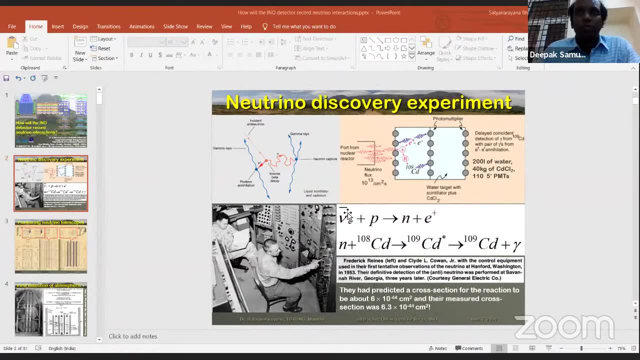 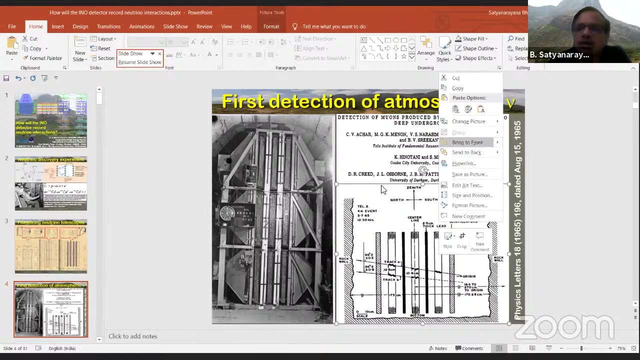 The screen is not shared. Yeah, And you see it now. Yeah, Okay, Okay. So this track here, this track up here, Right? This track is the muon that is present up and 5ة has G intersection. This is the Id. 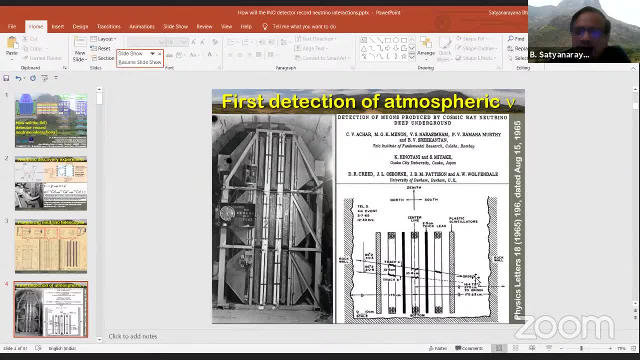 is zeroату and that G intersection is 0 Tik zu. The G intersection is not shared. It is produced in the W production And the origin is expected to be from the rock that is surrounding here, And this track here is supposed to be a muon decay. 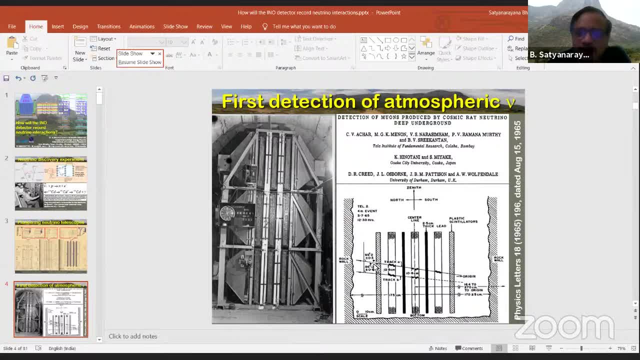 from the domain. So this is the muon. I mean both are muon, but this is the muon that is produced in the inelastic production And this is the muon decayed from W bottom And you can actually see that when they cross these layers.